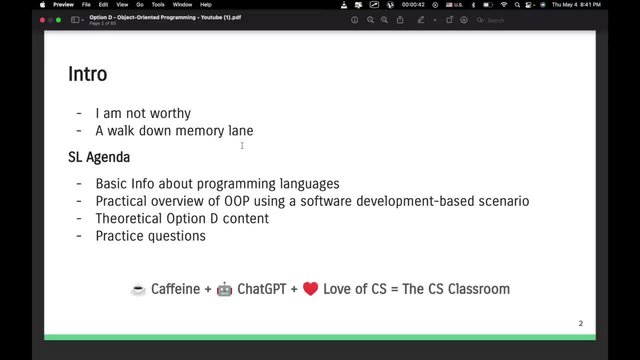 was about 15 years old and I used it in university as well. but it's been about 10 years since I've really used Java, so it's been a walk down memory lane. but some of the concepts, like particularly object-oriented programming, are so poignant and such a defining feature of Java that I haven't 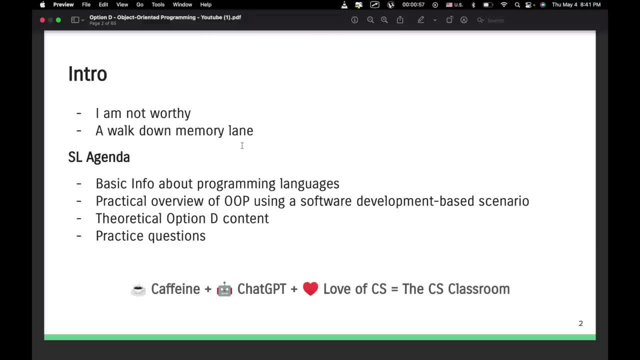 really forgotten them and I hope from this video you get a sense of that and you're able to really get a deep and intuitive understanding of object-oriented programming. Now in this video we're going to start out with some basic info about programming languages in general. Then I'm going to pose a scenario around which we're going to develop a program that makes 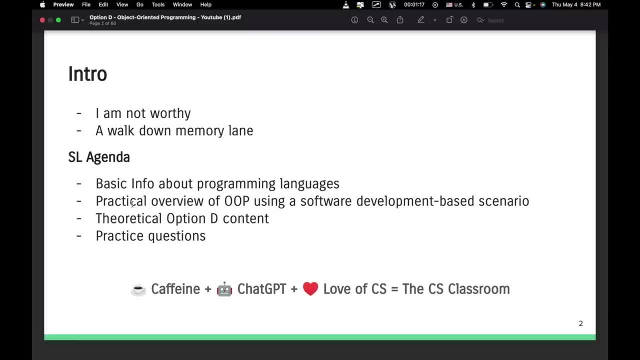 use of object-oriented programming. Part of the reason for this is that I didn't really feel like I understood object-oriented programming until I actually, like, started doing a job with, like a software engineering job where I had to use object-oriented programming, and I hope that you. 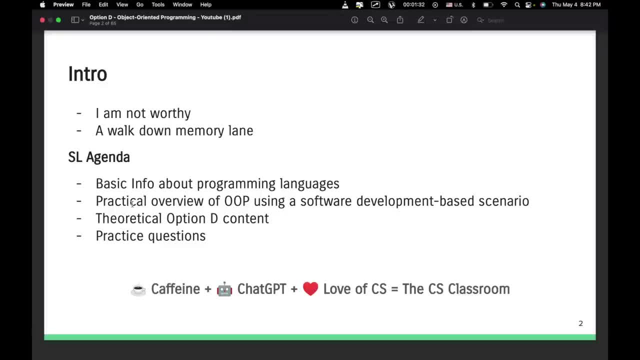 guys can understand it well. before that, In addition to that, we're going to cover some theoretical content interspersed with the coding and finally, we're going to have- we're not going to have- IB practice questions, but I am going to give you a list of basic tasks that you need to be able to accomplish in Java object-oriented. 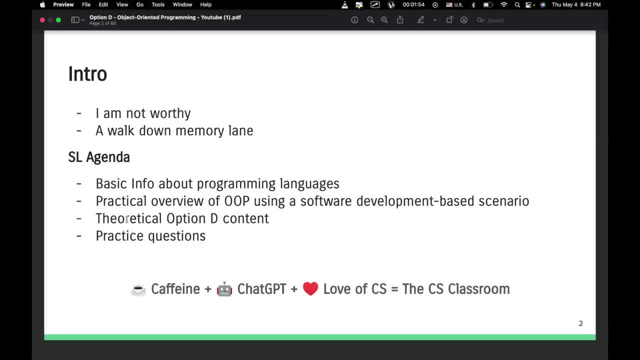 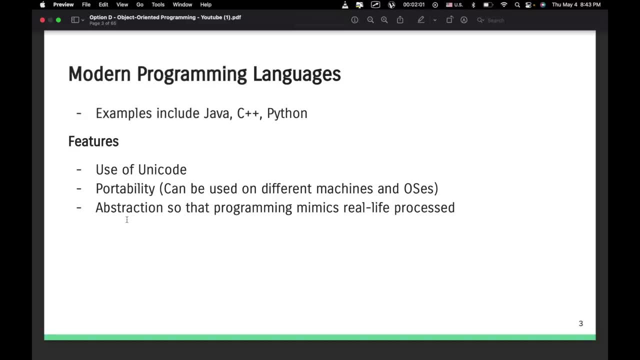 programming to be able to succeed on the exam, and then I'm going to code them and describe what I'm doing. So, that being said, let's go ahead and let's get started. First, I want to talk a little bit about modern programming. 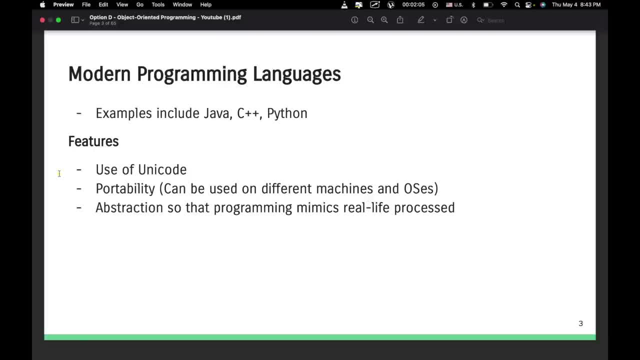 languages. So some modern programming languages include Java, C++ and Python, and they all have certain features in common. Firstly, they use Unicode which, if you remember from topic 2, allows us to basically utilize a bunch of different types of symbols and display a variety of text as output or using the. 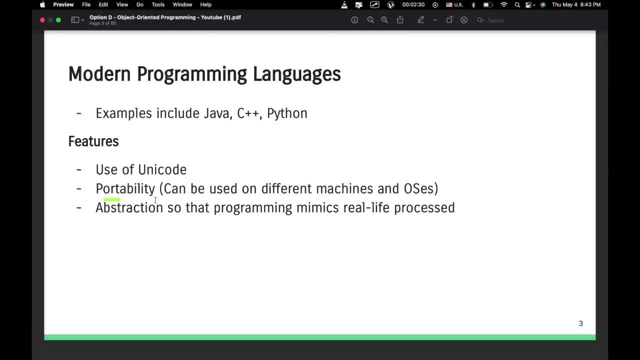 programming language in general. A second common feature is portability, so we can write a program in Java, C++ or Python, take it from a Linux machine and then run it on a Windows machine, for example. And the final feature I want to talk about is abstraction. So abstraction basically allows us to take programming. 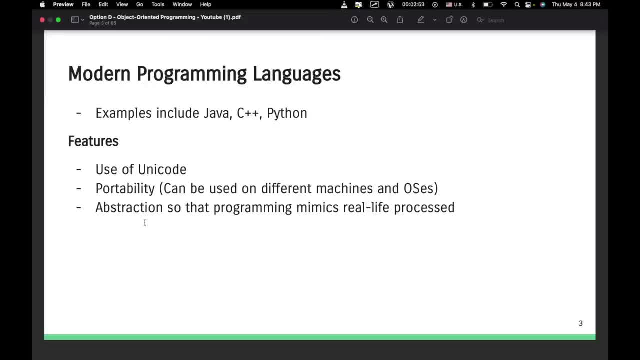 concepts and display them in a more simplified manner. In the case, specifically, of modern programming languages, we can take the underlying mechanics of a programming language and we can take the underlying mechanics of a programming language and we can write code as if we are mimicking a real-life process. So, basically, we can. 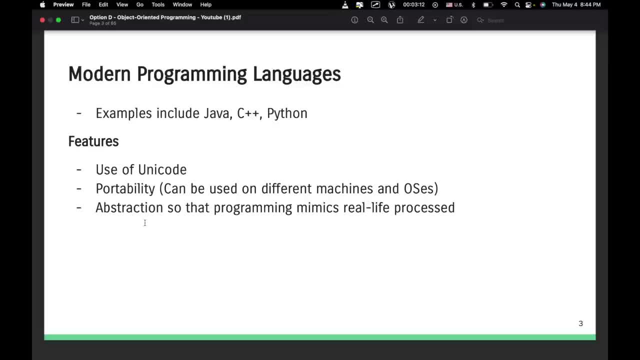 mimic the way that real life works using programming, because the way that is designed And that's kind of a hallmark of modern programming languages. Specifically in Java, object-oriented programming is abstraction, So it basically allows us to kind of not think so much about memory and how the kind of 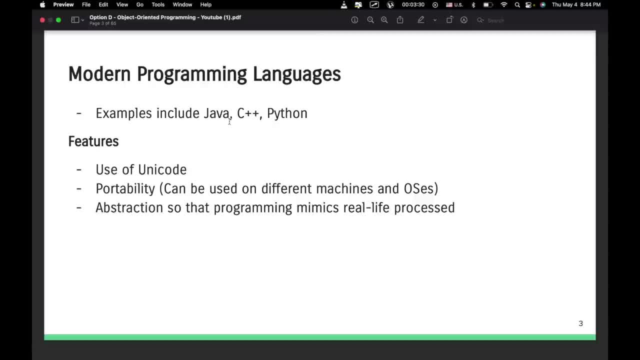 the nuts and bolts are working under the hood and it just allows us to write code that mimics a real-life process. Specifically in Java, object-oriented programming is abstraction, So it also allows us to really generate some logic for everything being able to. 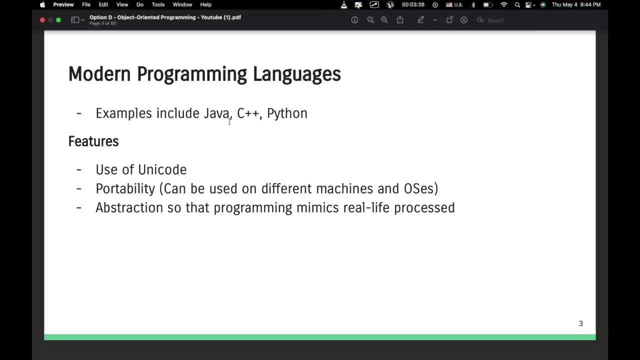 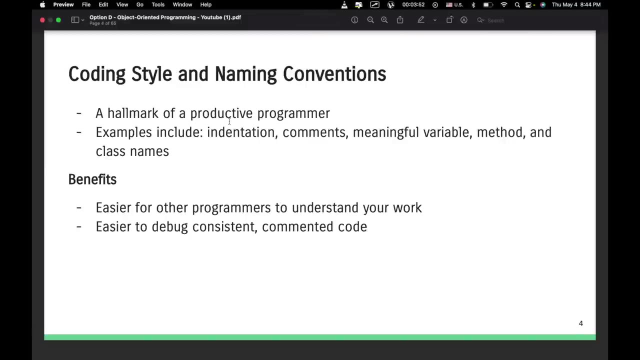 create some formula for photo or visual add-ons that corresponds to each and sort of model in our computer program And I know this is kind of difficult to understand, but when we go through a programming-based scenario, I hope you guys get a better understanding what abstraction is and how modern programming languages fill that role. Now, one thing that we're going to be practicing throughout this tutorial is coding style and naming conventions, And this is basically how to write what is called, in the software engineering world, a frame name is quite an acceptable extreme-spider way. 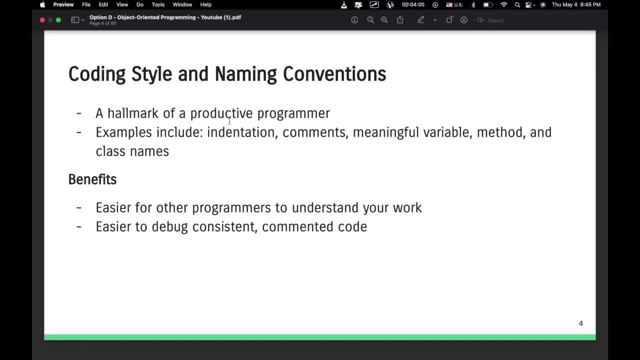 clean code. It's a code that can be easily used by a team and that's easy to understand upon first glance. So some examples of coding style. naming conventions include indentation comments explaining what lines of code are doing meaningful variables. so instead of calling a, 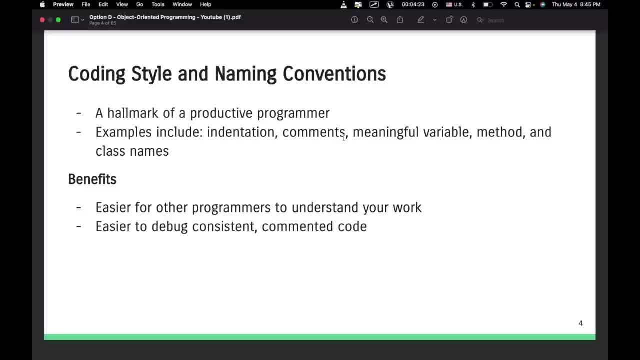 variable x, maybe you give it a name that corresponds to its function, and meaningful names for methods, your functions and class names as well. Now, the benefits of these are that it's easier for other programmers to understand your work. so if you're working in a team, 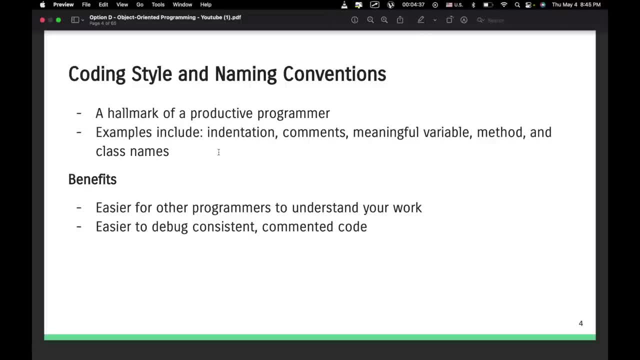 everyone's kind of on the same page And furthermore, it's easier to debug this code because you know what's going on when you just look at the code. So if there is an error, it's easier to identify the flaw in the logic of the code and then fix it. 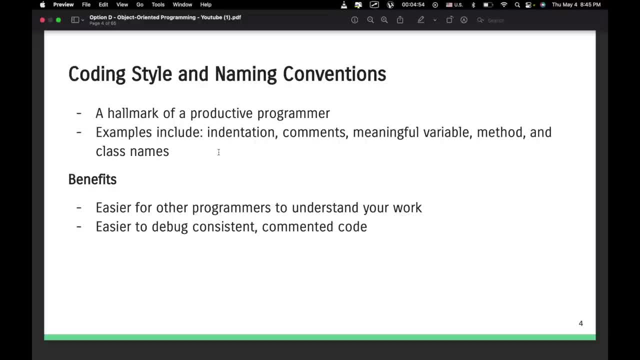 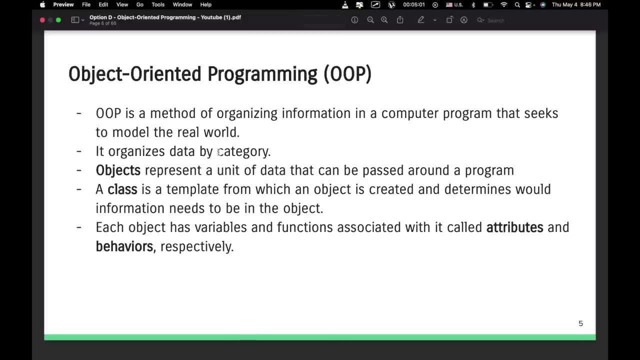 Now, yeah, let's get started with talking about what we're going to be building. So we're going to be using Objective-B, Object-Oriented Programming, to write the programmer programs we're working on today. Now, this is a big topic. Object-Oriented Programming is a method of organizing. 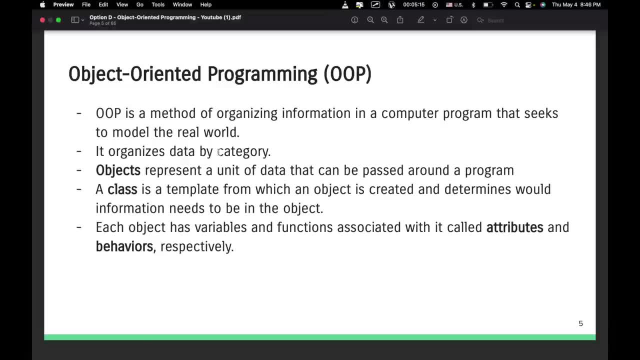 information in a computer program that seeks to model the real world. Now what does that mean? It basically means that we're going to take the data that we want to work with and try to. I mean, first of all, we're going to organize it into categories. 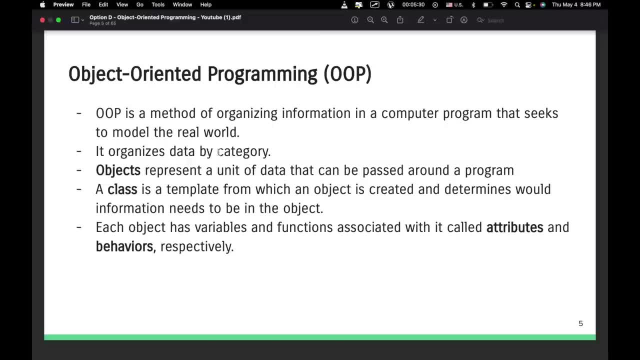 So we're going to take all the data in our computer programs, classify them into different categories and then, once we've done that, we're going to give each of those categories certain methods and certain variables to describe them And using that, that sort of way of organization, we're going to generate a computer. 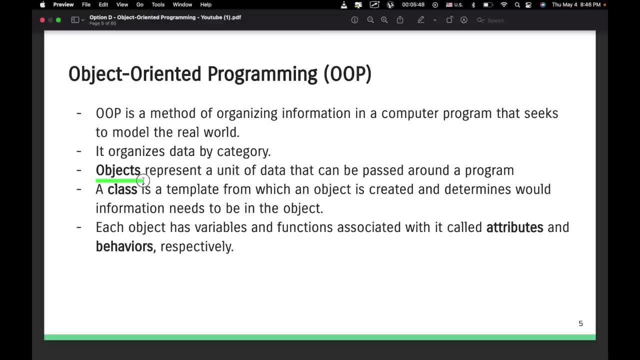 program. So within our programs, we're going to be passing around these things called objects, which are basically a collection of information and functions that manipulate the information, And these objects are created from a class which is a template sort of a plan. 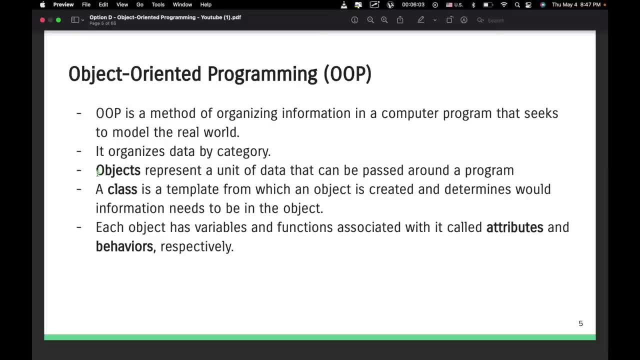 for what our object is going to look like. So we're going to be working with objects and, in order to create an object, we're going to write a class which is sort of like a template or a plan from which an object can be created. 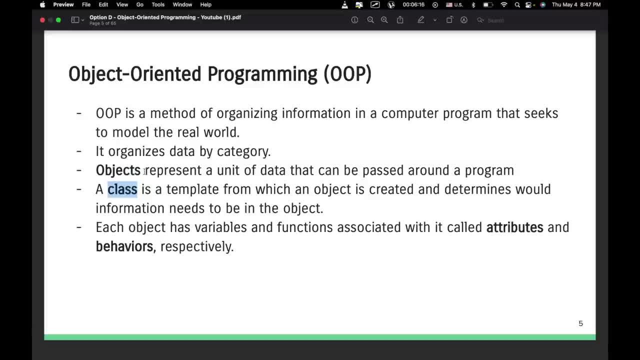 If you think about human beings being created from DNA, I guess a DNA code would be our class and a human being would be an object, right? A DNA code kind of describes everything about us, but it's not actually a human being, It's not a biological being. 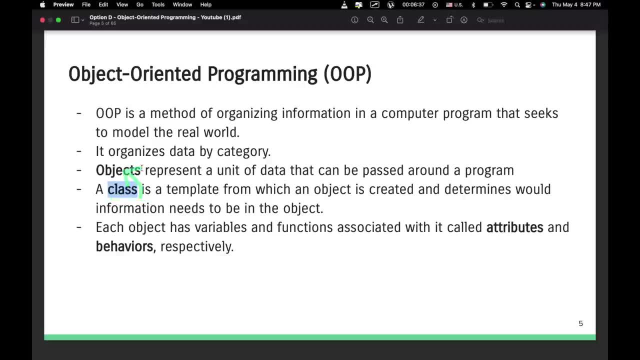 But from a DNA code. we could then create an object, which is, in this example, human beings. Each object will have variables and functions associated with them, called attributes and behaviors. Now, this is just a high level overview. If this doesn't make sense, if this seems too abstract, 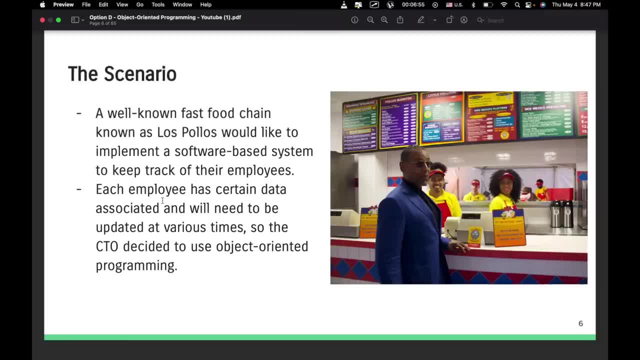 we're going to look at it in a more concrete way. So, in order for us to really understand object-oriented programming, we're going to be kind of playing with a scenario throughout this tutorial. That scenario is a well-known fast food chain known as Los Pollos. 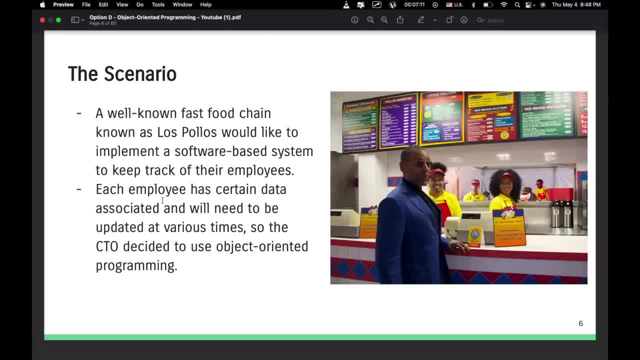 Now Los Pollos would like to implement a software-based system to keep track of their employees. Each employee has certain data associated with it and will need to be updated at various times. So when we were talking about categories of data before, what we're really talking about in the case of this program, 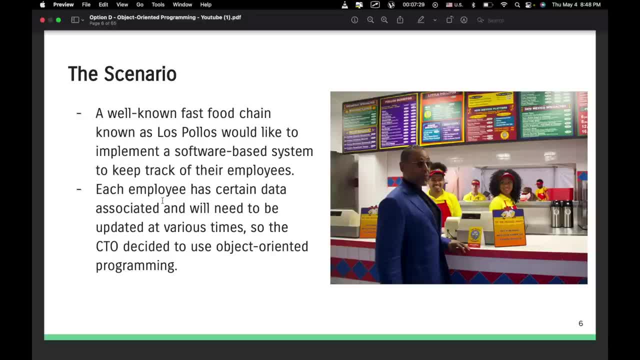 is employees, and each one of the employees is going to be an object. We're going to have an employee class or template. Each one of those objects is going to have certain data attached to it, because each one of those employee objects is going to represent an employee. 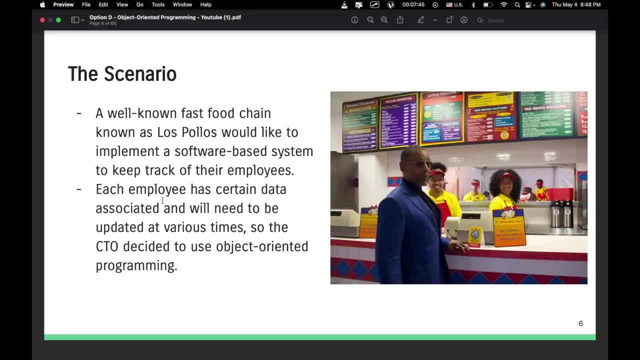 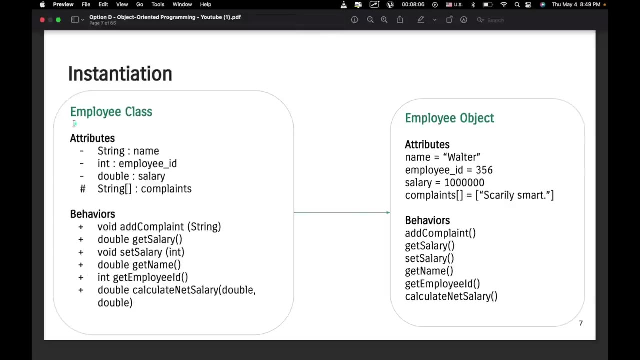 There'd also be other functions or methods attached to an employee object so that we can manipulate or we can carry out certain operations to update that employee's data or a variety of things. CTO, accordingly, has decided to use object-oriented programming. So the first thing we're going to work on is an employee class, okay. 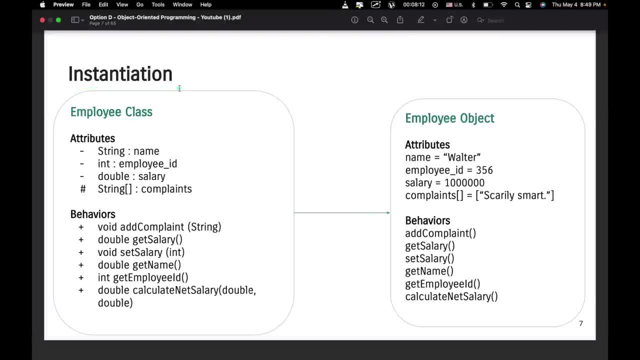 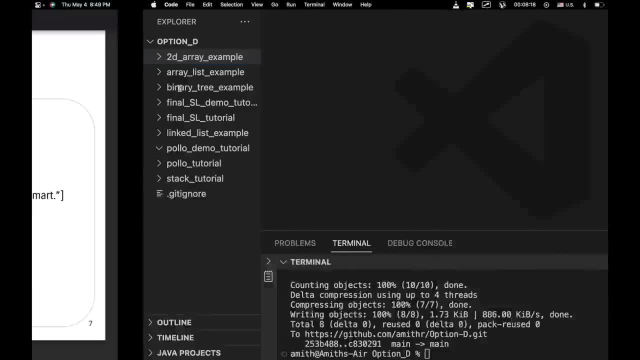 And we're going to be working with a concept called instantiation. But before we do that, we're just going to go ahead and start writing some Java code. So let's go ahead and let's get started. So we're going to be working in this folder: PoyoDemoTutorial. 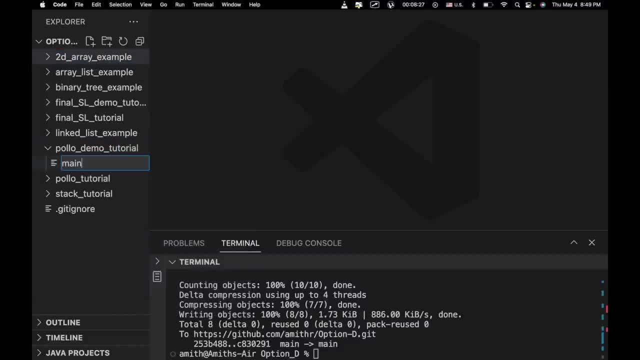 Now I'm going to create a new file called mainjava, And every single Java file should have a name that corresponds to the class that we're working with. So actually, I actually just really want to capitalize this. just for consistency, I want all my class names to be capitalized. 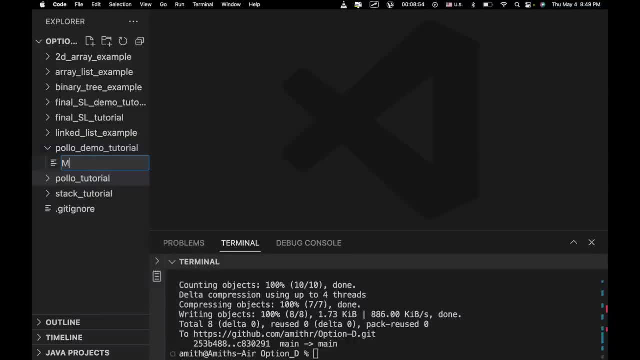 It's kind of one of those things that goes along with writing clean code, So we'll just say: mainjava. Okay cool, All right, just a little thing, But all right, cool. So we've got public class main. 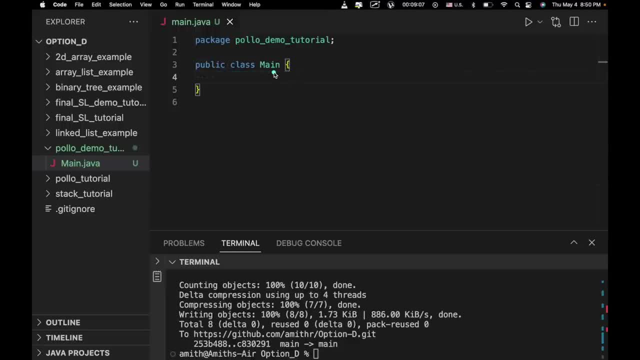 And we're always going to have this main class to execute, to kind of work with our other classes. So this main class isn't really going to be playing a big part in terms of just our demonstration of object-oriented programming, But all of the operations that we do with our classes are going to go through here. 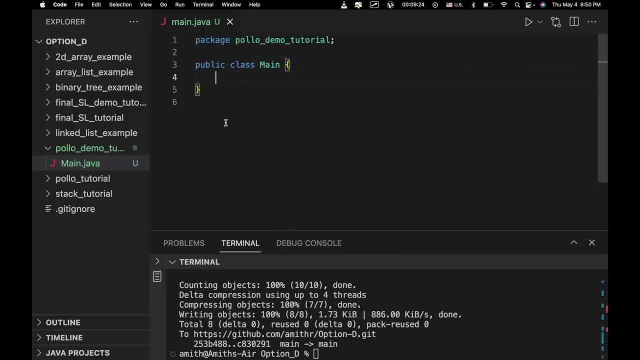 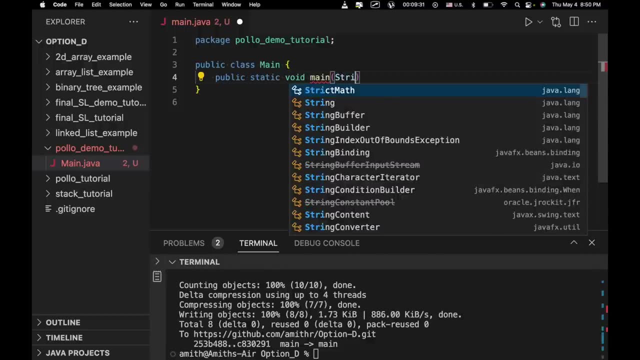 This is sort of like: This is our main staging ground, So we're going to have a function called public static avoid main. Also, this should be pretty familiar with you, because you should know something about Java. I mean, this is meant more to be a review. 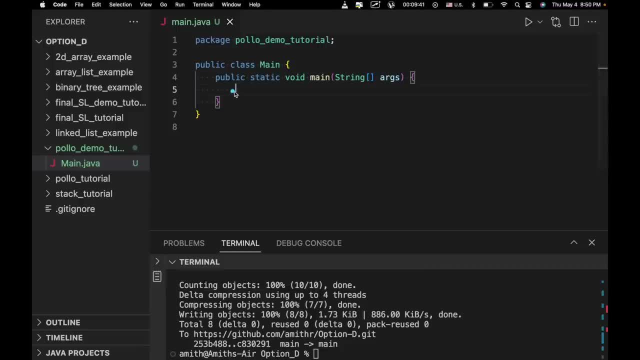 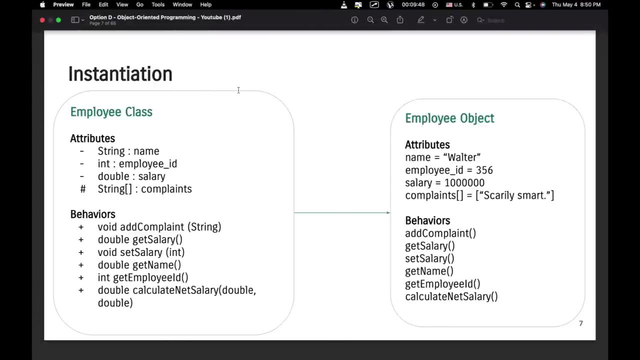 But anyways, we're going to just kind of create this function And we're going to be executing really any of our code in here. So, that being said, what we want to do first is we want to create an employee class. Now, this employee class is going to be: 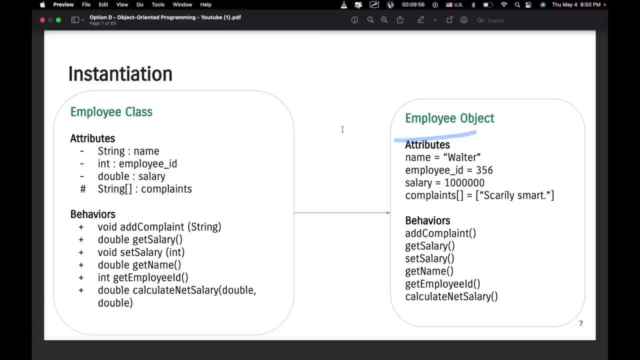 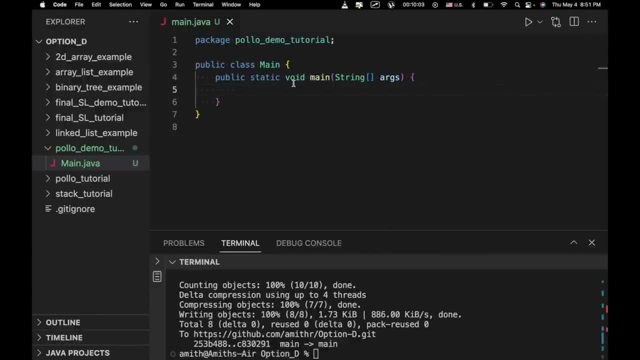 a plan or a template for employee objects, and it's going to be used to model employees in our program. So the first thing we're going to do is we're going to create a new file here called employeejava. All right, So it's going to be called. 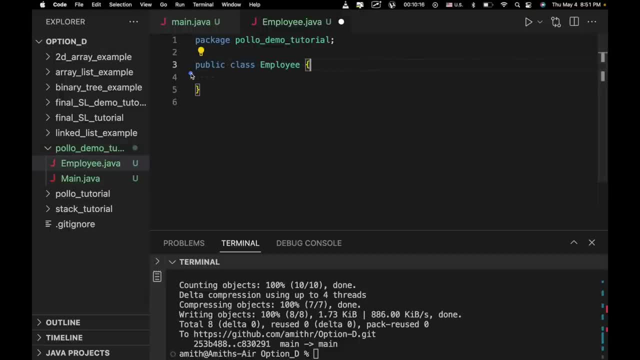 We're going to have public class employee. The public is called an access modifier and we're not going to go into that at the moment, but we will later on in this tutorial. So what I want to do, What I want to do first, is I want to define attributes. 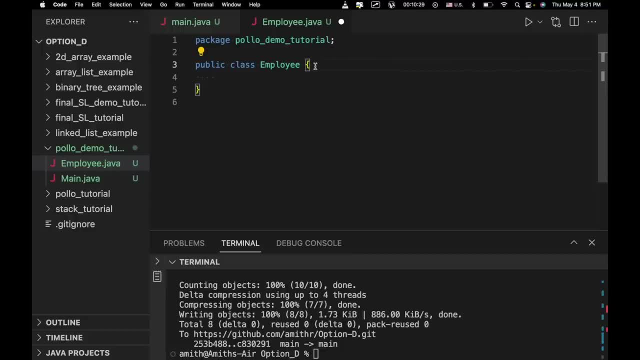 So by that I mean variables that we can be used or that we can use to describe every single employee. So I'm going to start by saying: by I mean, I guess every employee has a name, right? So we're going to say string, name, string being the data type and name being the name of the attribute or variable. 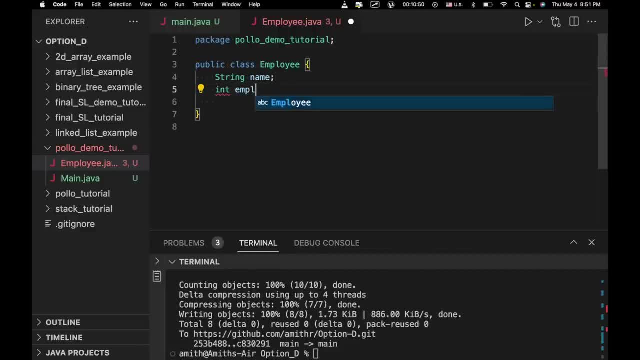 Next we're going to have int employee ID. We're going to have, because every employee is going to have an integer employee ID. Next we're going to have double salary And next we're going to private. Well, we're not going to go with the private quite yet. 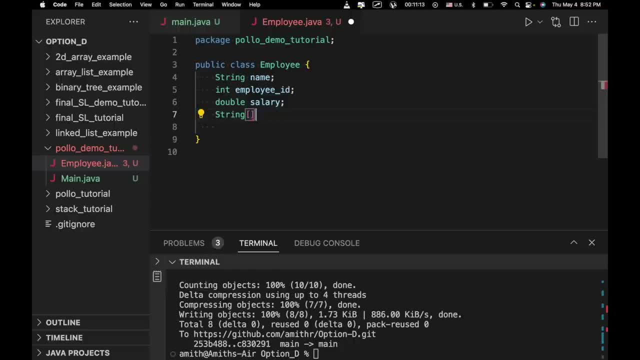 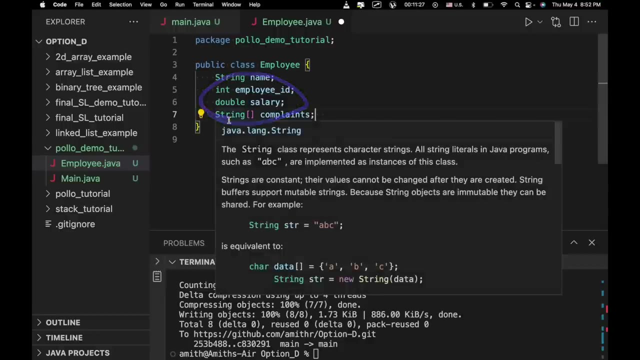 We're going to have string with an array symbol and then complaints. So we're going to have an array of strings and the name of that array is going to be complaints. So right here, these are all the attributes or variables that describe an employee. 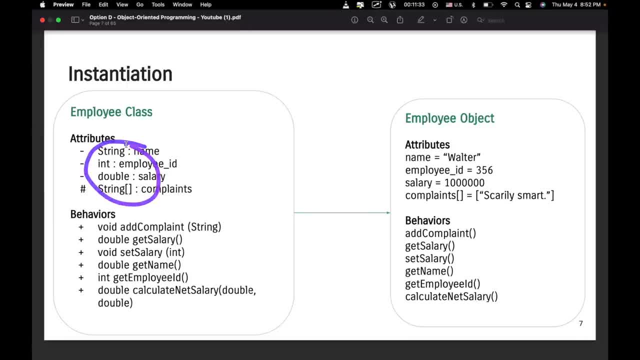 And if you look at our chart right here, we actually specify these right here as our attributes: The data type and the name of the particular attribute. Now, this format might seem strange to you and you may not understand everything on it, but this is actually called a. 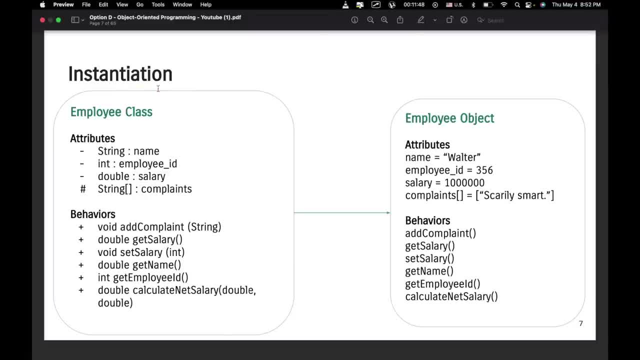 Well, this is actually called a UML diagram, or this is part of a UML diagram And UML diagrams. UML diagrams, which we'll get to later on, are used to basically describe object-oriented programs and be able to give a visual description of how an object-oriented program functions. 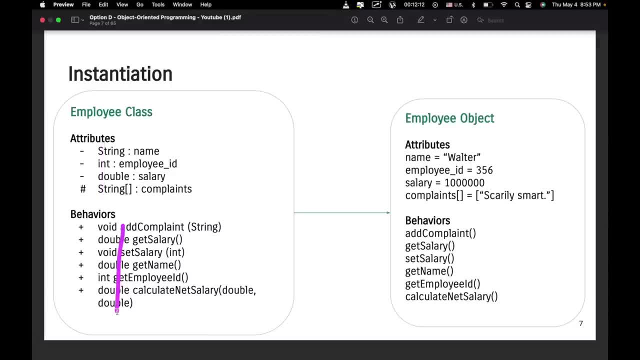 Now we have some attributes, but we also need to have some behaviors as well, And we're also going to need to have some functionality so that we can actually take this class and turn it into an object. So this is the process of instantiation. 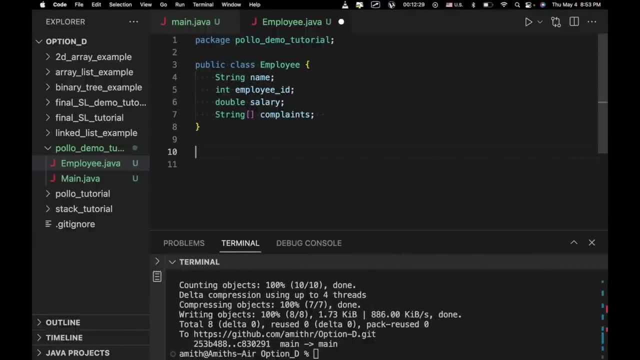 So the next thing we're going to do is we're going to create something called a constructor. So a constructor is a function that we access, or it's a function that we access in order to create, in order to take our class and turn it into a template. 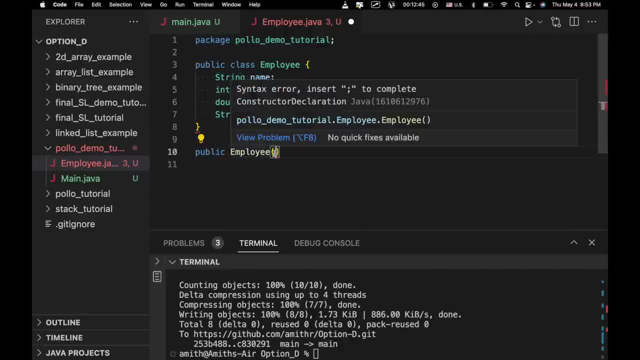 Now I'm going to say string, So I'm going to say public employee string name. We're going to have a parameter for name. We're going to have an int employee ID, an integer employee ID and double salary. Now, this may not make so much sense right here, but just bear with me for a second. 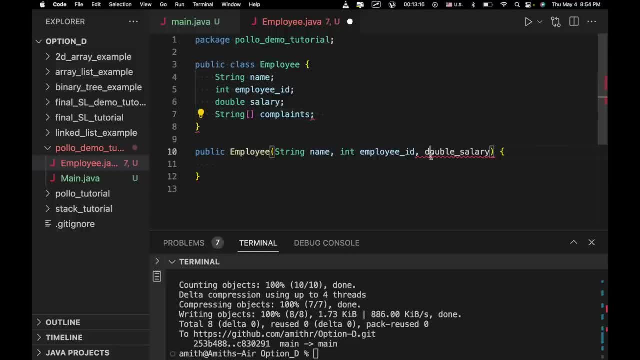 Also, we probably have something we need to fix up here. Oh, okay, We'll get to that in a second. So, double salary. So these are all the parameters for employee And okay, I know what we need to do. 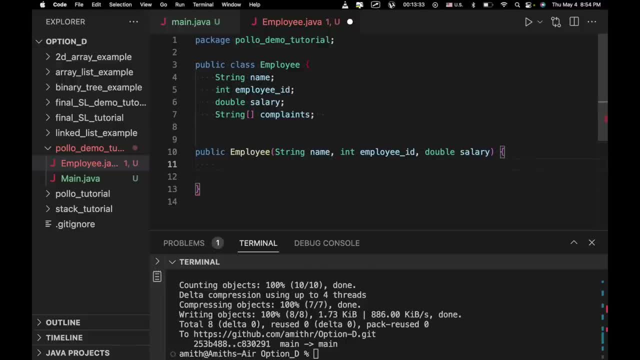 We just need to get our braces right. So we're going to have one brace, or well, we're not going to have any. We're going to have. this is a part of our class. We're going to have braces for our class and then for this constructor method right here. 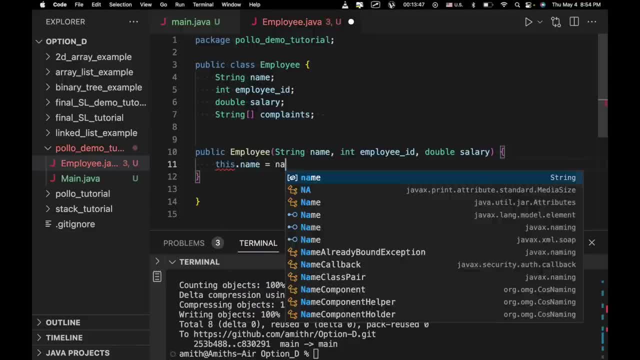 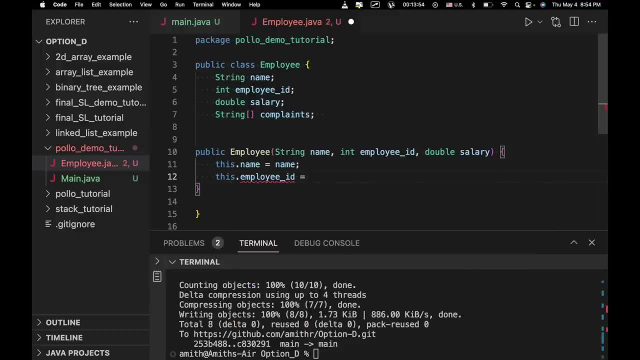 Right, here we're going to say: thisname equals name, ThisemployeeID, Thissalary equals salary And thiscomplaints equals new string 10.. So we're actually going to here: we just created an empty array of complaints. Here we're going to make sure that our complaints is going to be an empty array with 10 positions in it. 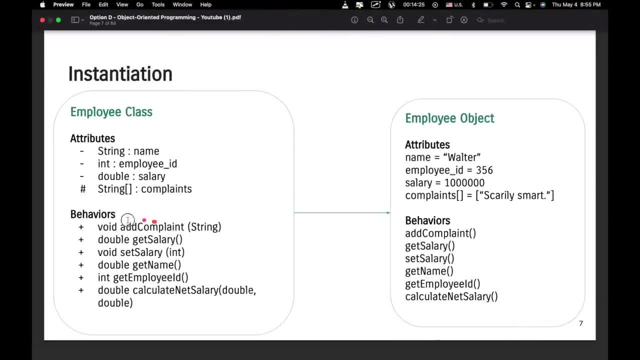 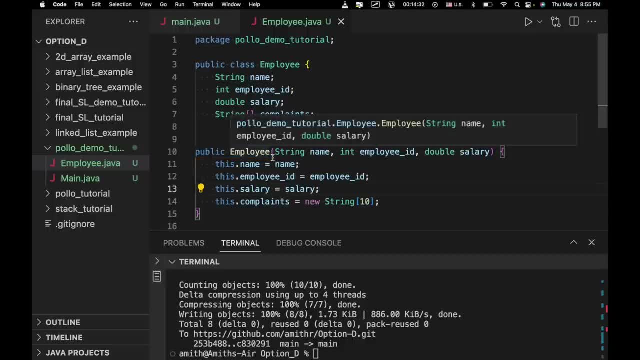 Now, before we go on to all the other methods right here, I'm going to go ahead and I'm going to show you basically what role this constructor plays right here And kind of just give you a better idea of where we're going with objects in general. 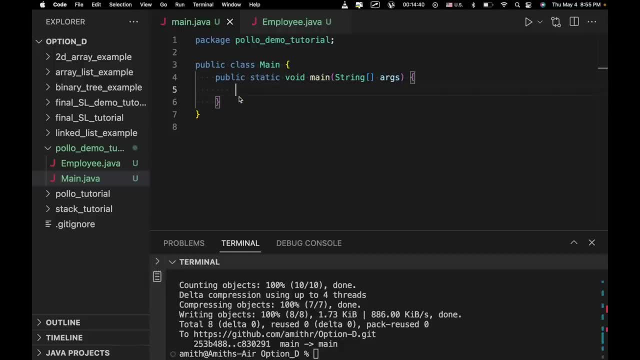 So right here in mainjava, where we're actually executing all of our code we're going to create, we have this employee class And we're going to create a new object from it. Keep in mind that inside this folder, our mainjava- 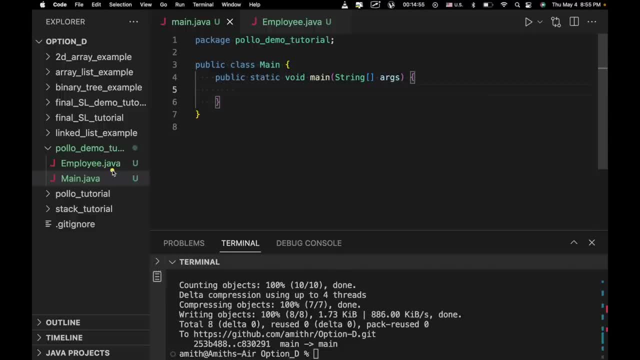 Actually, any file here has access to all of the other files. So what we're going to do is we're going to create a variable called employee1.. We're actually going to give that a data type of employee, because our employee1 is going to be an employee object. 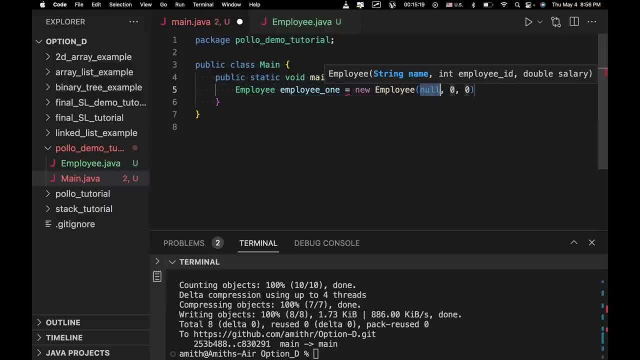 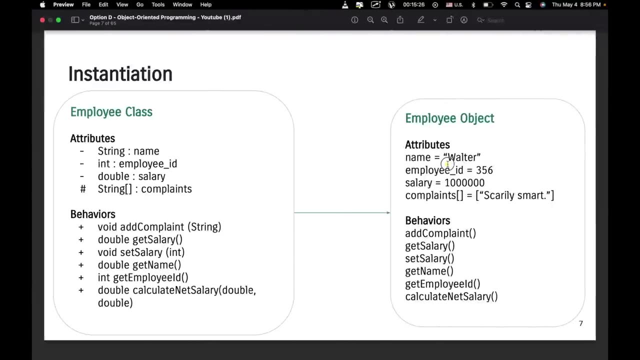 And we're going to say new employee And Right here we're going to create this employee object And we're going to give it a name of Walter. It's going to have, we're going to have- an employee ID of 356.. 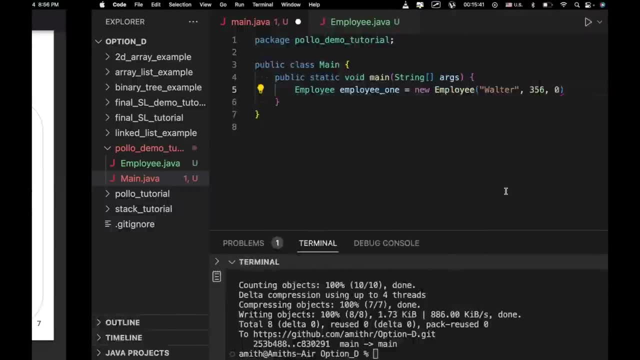 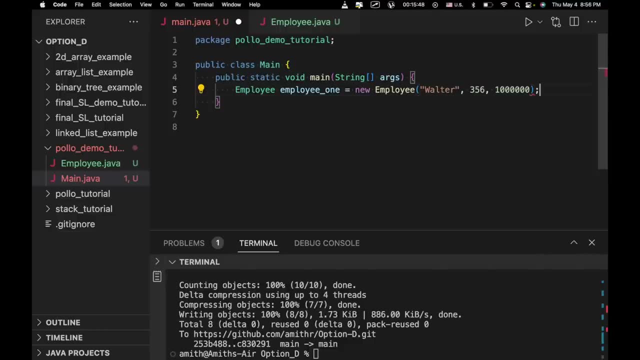 And a salary of it should be $1 million a year. Let's say $1 million, And this is as we are creating A new employee object that represents Walter, with employee ID 356, who makes $1 million a year, And that's going to be employee1.. 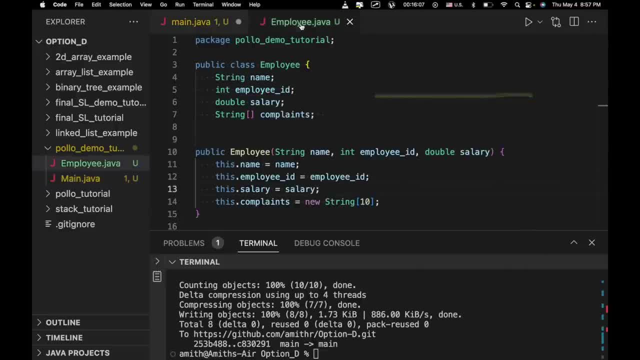 Now right here, if we look at this right here, this matches up to this constructor function we wrote right here. Our first parameter was a name, employee ID and double salary. So in every single class. I'm also actually going to tab this for clarity. 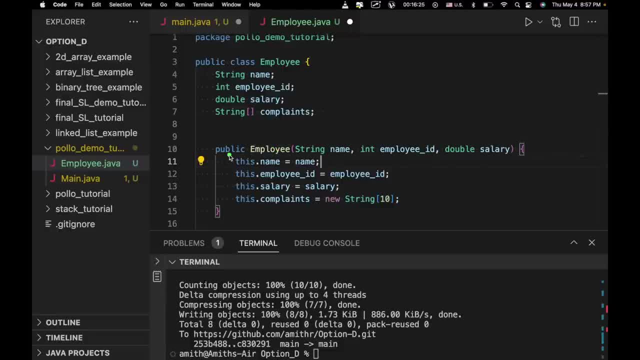 But in every single class we're going to have a function or a method. It's going to be public, which again we'll get to later- It's going to have the same name as the class And it's going to have all the parameters you want to enter in order for us to be able to create this object. 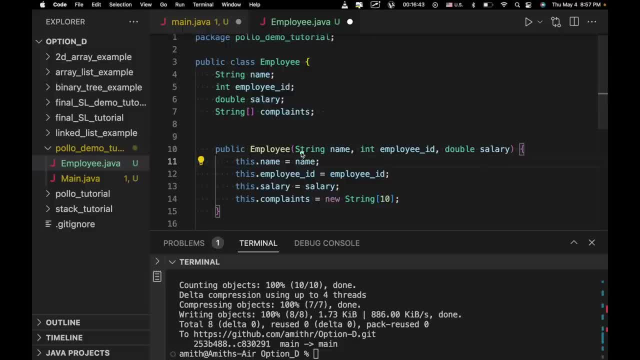 Basically, in order to be able to give the values we want to any attributes. We can also do other things we want when we create this object, Like, for example, create, turn, give an attribute a blank array. So this executes when we actually create an object from a class. 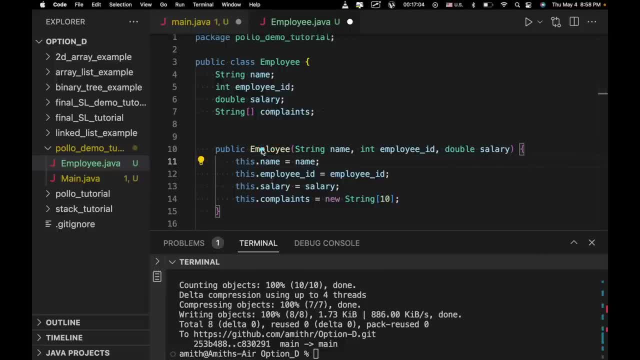 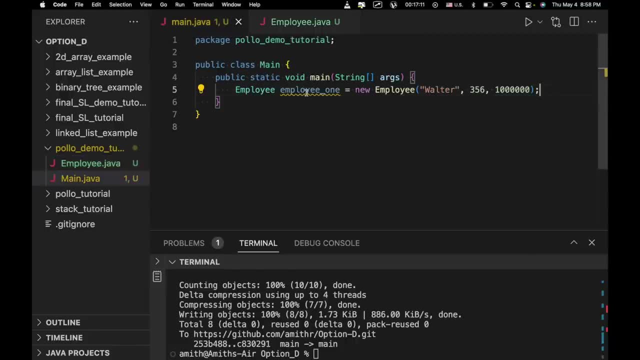 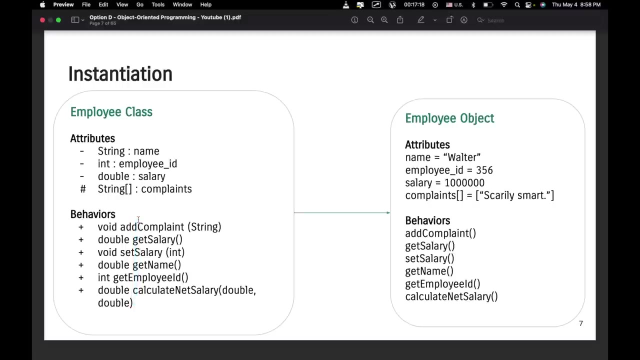 When we go from the classes being a template to it actually being good, actually allowing us to create objects. So that's that right there. So now that we've done that, we can go ahead and add other functionality to our class. So we're going to do a few things. 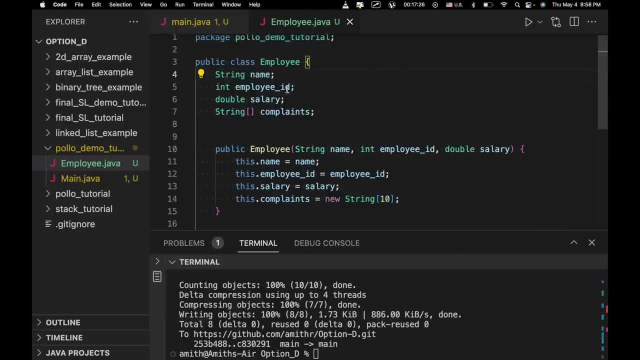 So, first of all, what I'm going to do is I'm going to create what are called mutator and accessor functions. So right here, I'm going to create what's called a mutator function, And that's going to go look like this: 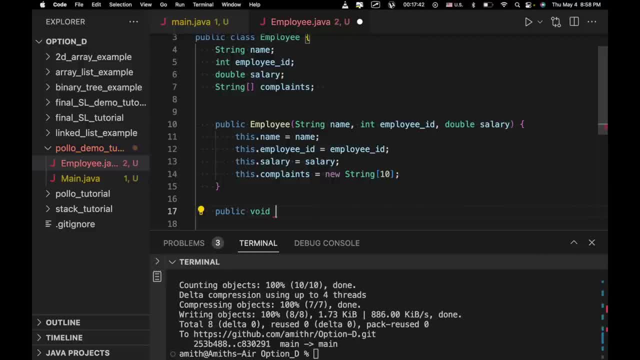 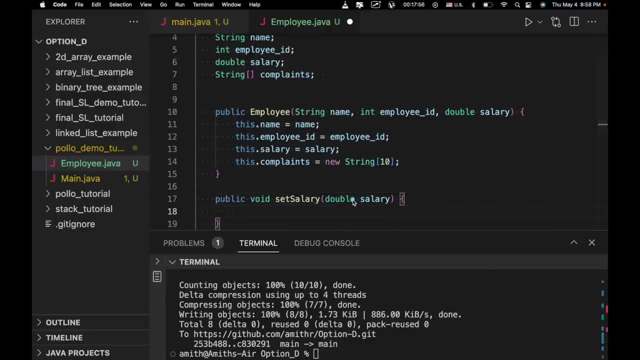 Public void, let's say set salary And double salary. So I'm creating a method called set salary with a parameter, with a parameter of double data type, And that returns nothing, And we're just using this function to change the value of this particular parameter, right here. 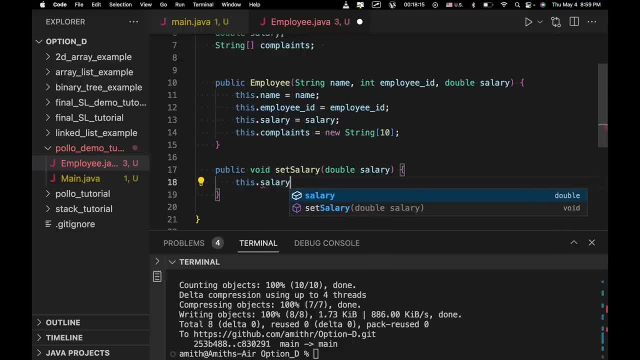 So we're going to say this: dot salary equals salary. Now you might wonder why we used this. So when we're working with classes and methods, we have a concept called scope. So basically, this name, like this name right here. 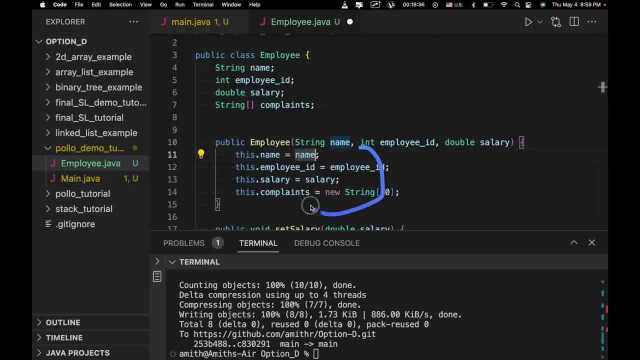 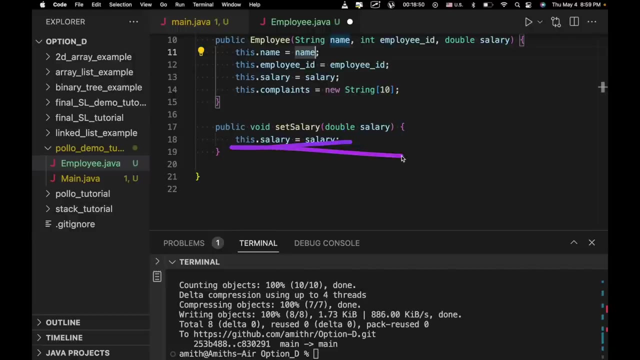 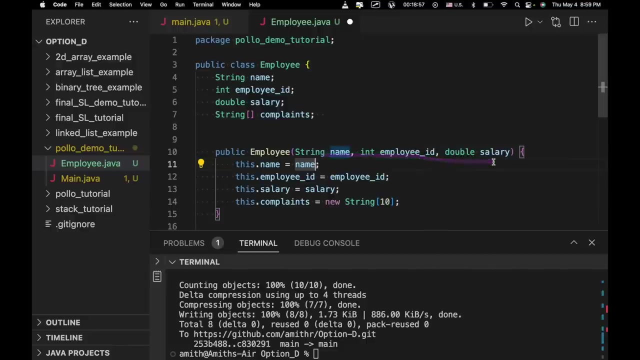 So this particular variable only exists inside this method. So all of these parameters for these methods only exist inside this method, right here. Similarly, this salary parameter We Specified also only exists within this method, right here. However, we want to be able to take our parameters and set and basically allow them to interact with our class attributes, with these, right here. 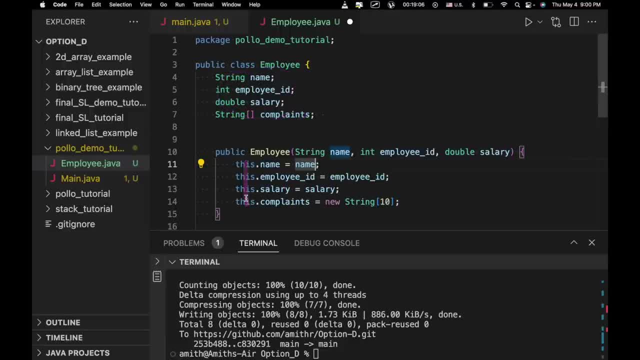 So when we're using this, when we're using this, we're referring to our, referring to the variables associated with our class, Or really it's going to be with our object. So this is so, while name is referring to this parameter, right here. 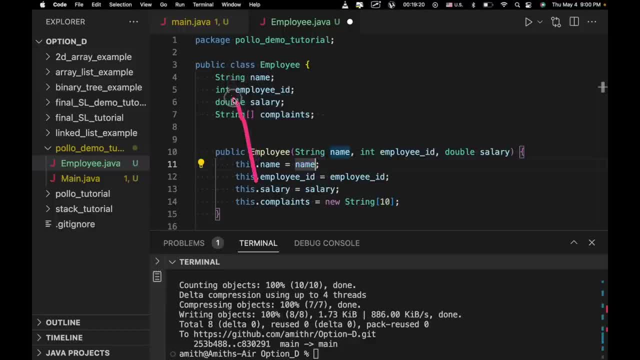 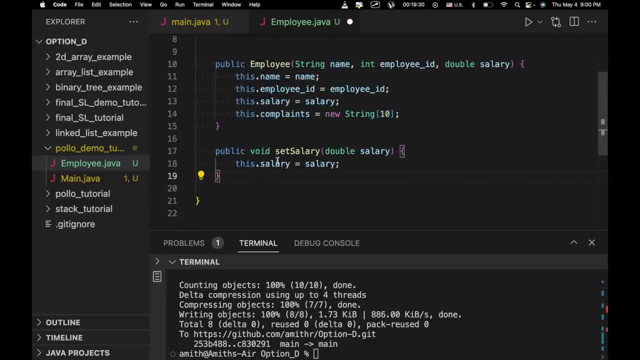 This dot name is referring to what's on our class right here. So we did. we had this right here. We created a function called set salary and we could actually do if we wanted to Employee one dot salary equals five billion, five million. That's how classes work. 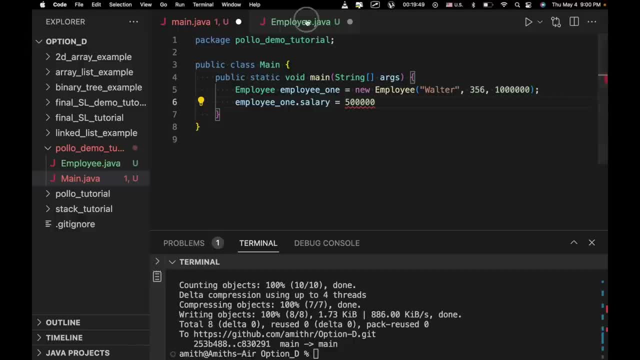 Okay, We could do that Really. Any of these class Attributes we have here we can access in this way, taking the name of the object we created and then just putting a dot and then a period, or we can have employee one dot. employee ID equals five, fifty thousand. 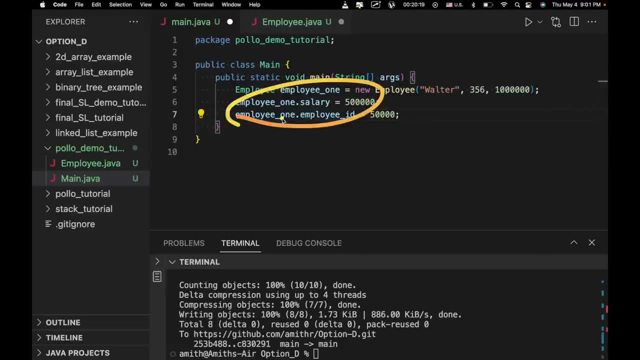 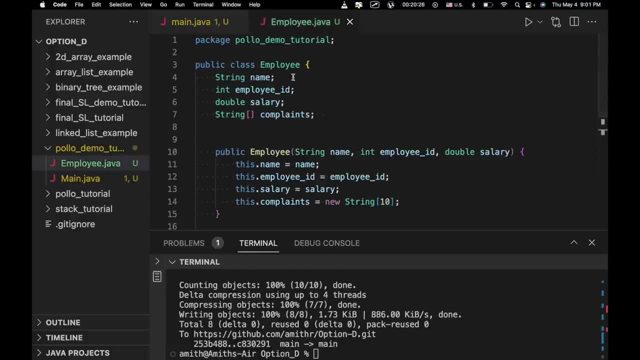 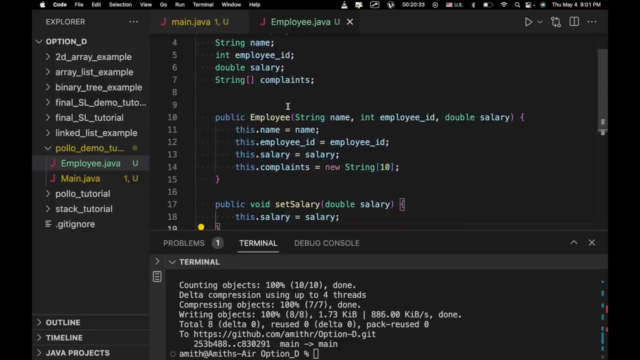 Okay, But we're not going to do this actually. So there's a few reasons for that. So, firstly, we want to force. Well, first of all, the biggest thing is actually one of the most important parts of object oriented programming is that it kind of it's kind of built for us to work in teams. 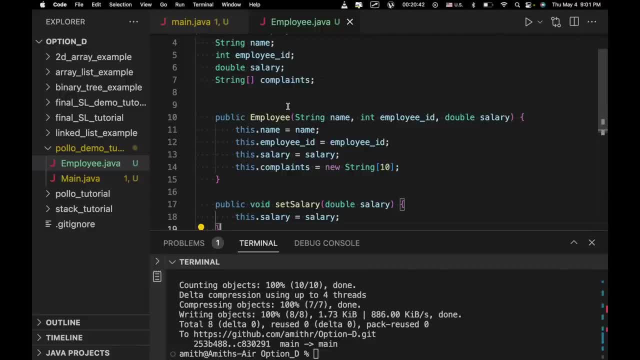 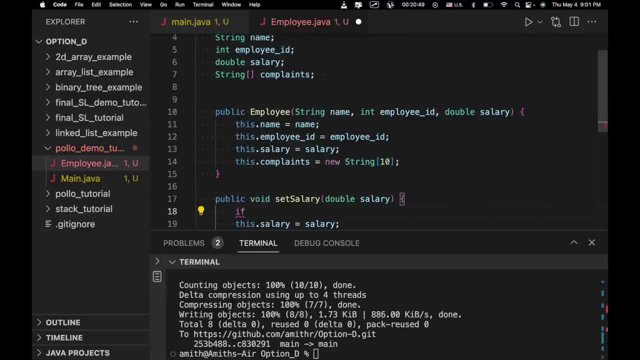 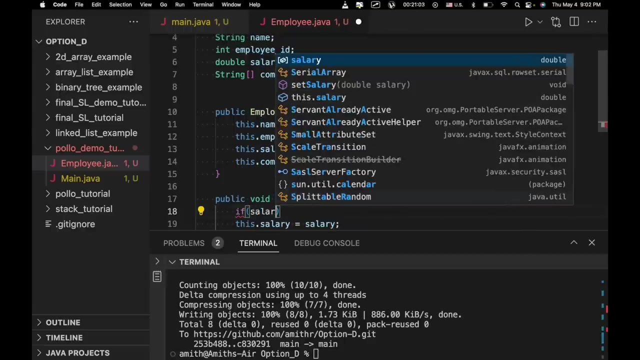 Right. So we want other programmers to only interact with our class in a certain way, So we don't want them to set any salary. We want them to set a salary. We might want them to set only a salary that is greater than, say, if salary is greater than or less is greater than zero. so we may only want them to set a salary that's greater than zero, which kind of actually makes sense. 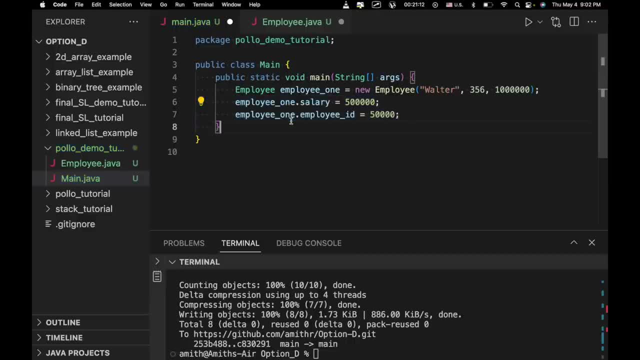 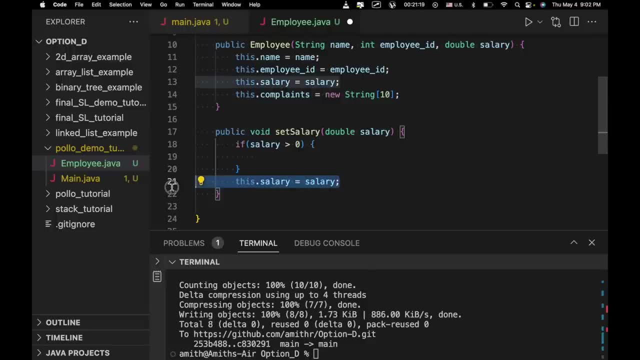 And that's not something we could do right here with our previous example. Okay, That's why we don't do this. So we're going to take this, we're going to put this right in here and we're going to do that right there. 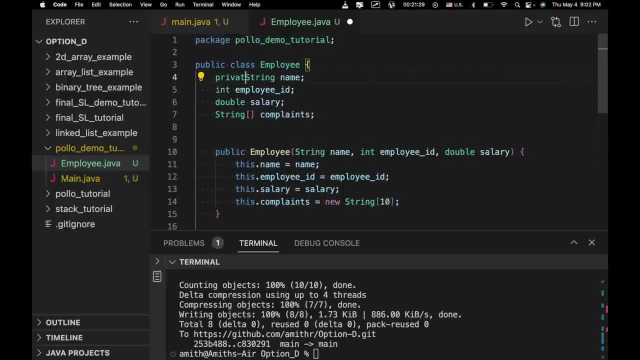 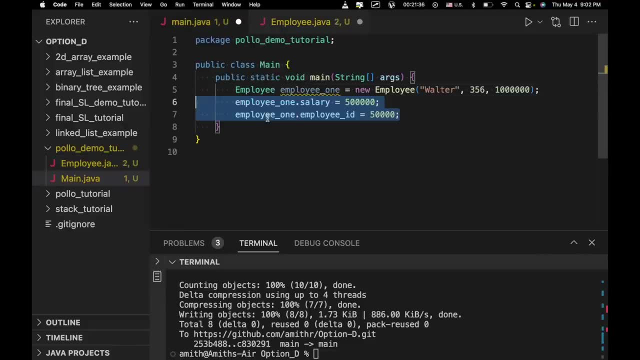 Now we're also going to make these something called private, which limits the access of other classes to them, And private also means that we can't do what we just did right here. So if we give them a private designator, one of the things that happens is: this is not allowed. 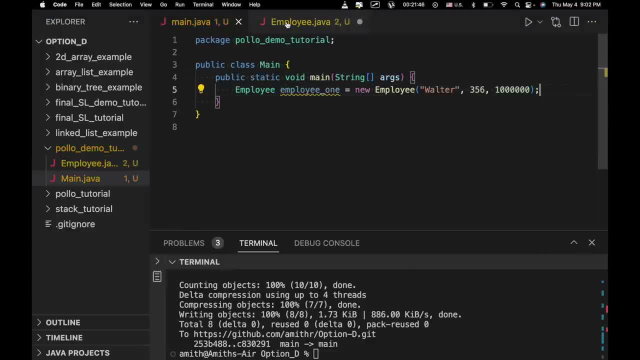 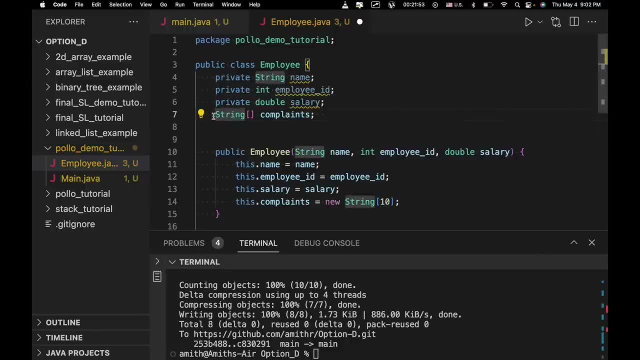 This won't work. So, again, that's so that anyone who's programming and using our classes Has to abide by certain rules, Again with the private and public like. I am doing this right here, but we are going to get into this later on. 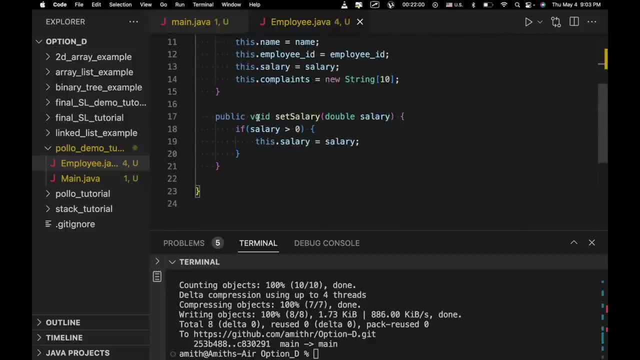 It doesn't play a role in the functionality, but just bear with me. So this is our mutator method right here for salary. Anything that changes an attribute is called a mutator method. Next we're going to do public void, public double: get salary, which is an attribute. 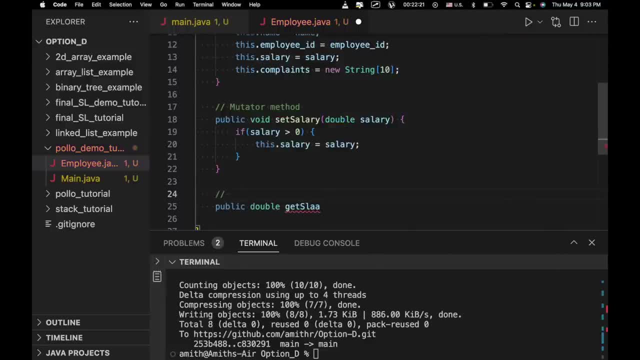 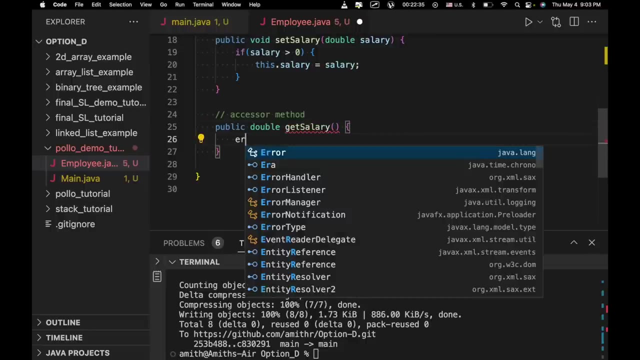 And we're going to do the accessor method And we're going to add a few more methods. We'll go through this a bit more quickly because I've covered a lot of the concepts that I wanted to cover early on. So let's say, get salary and then we're going to return a double of salary. 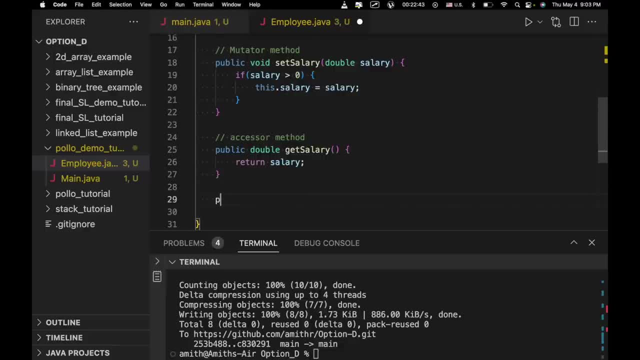 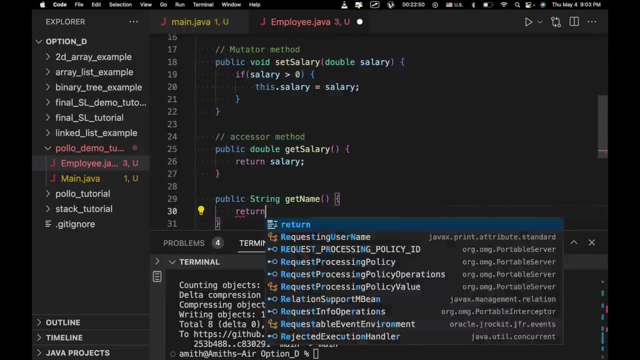 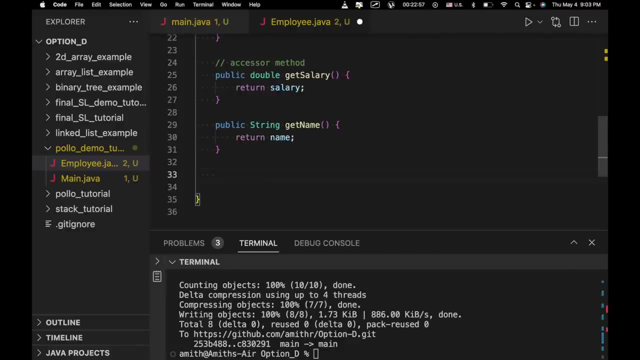 We're also going to do public string get name. We're going to do the same for employee ID because, again, we want to limit access to those. So the only way that someone should be able to get access to this attribute right here in name is by using get name. 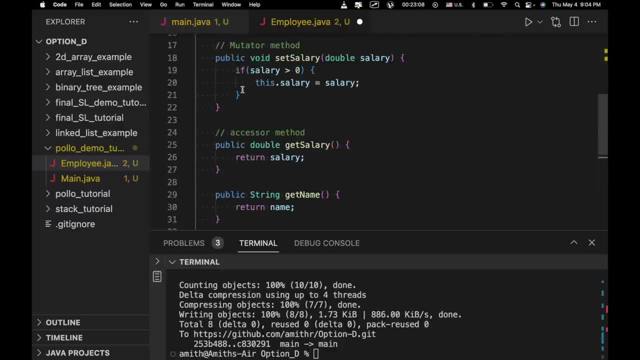 And they shouldn't, particularly since these are private up here. they won't be able to just change them, Particularly because we don't have any set name function. We're not going to have any set name function. Same is going to be true for get. 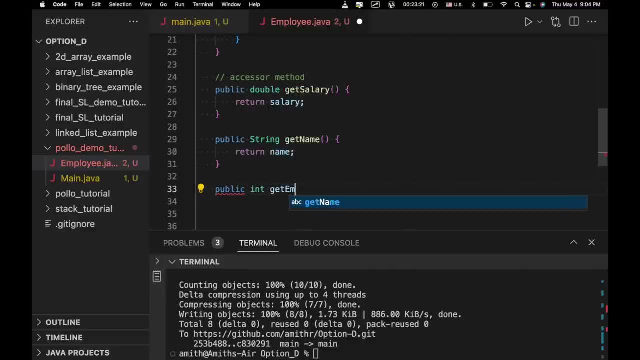 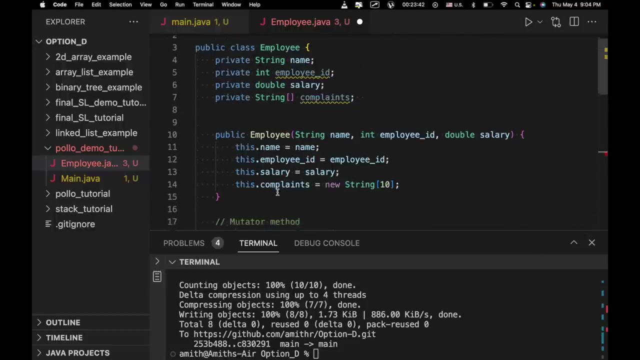 Get employee ID. Okay, cool, I'm just going to return employee ID, which was actually of an int data type. One thing I do want to do as well is I'm going to change these. So one thing, that one mistake I made here is: I want 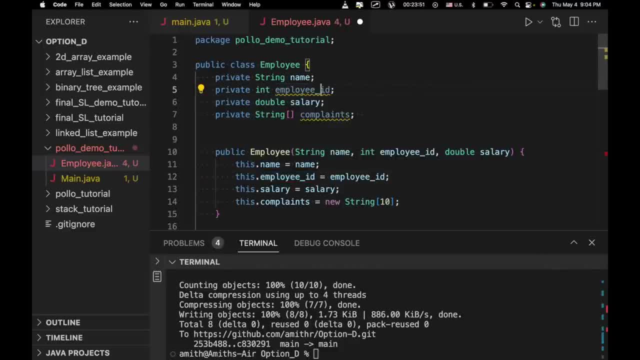 To use something called camel case, which means that we're going to start all of our variable names with a lowercase letter And then the next word in our variable name is going to be uppercase. So if employee uppercase I, and then the rest of the other word. 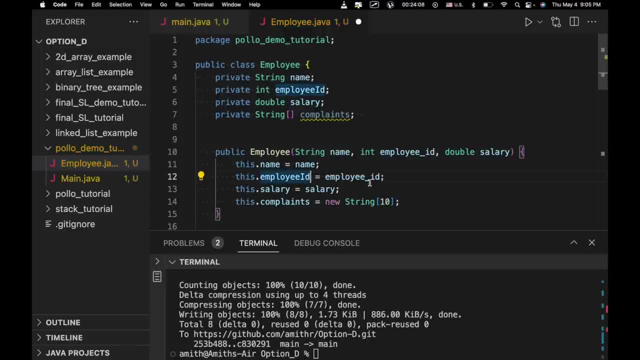 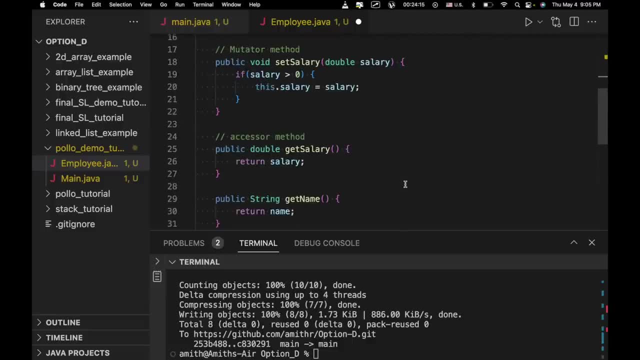 And that's just good coding practice. That's part of those coding conventions that we talked about earlier, So I'm just going to go and fix that before we go any further. That's how I named these methods as well. We have set. 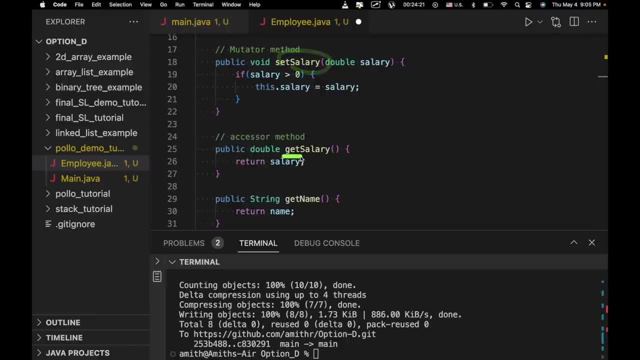 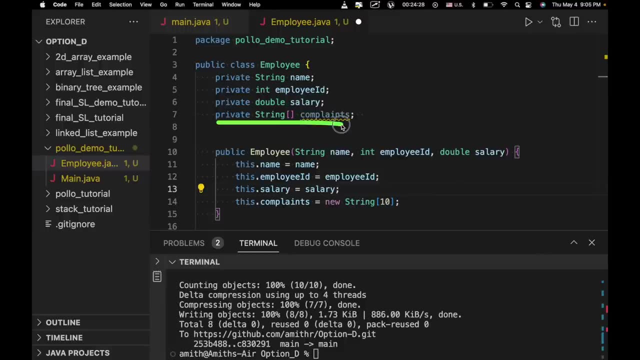 It starts with a lowercase letter and then a capital salary get and then a capital S and then salary, And the last thing we want to do is we want to allow the user to add complaints. So we're going to say we're going to create a way to do that, particularly since this is an array. 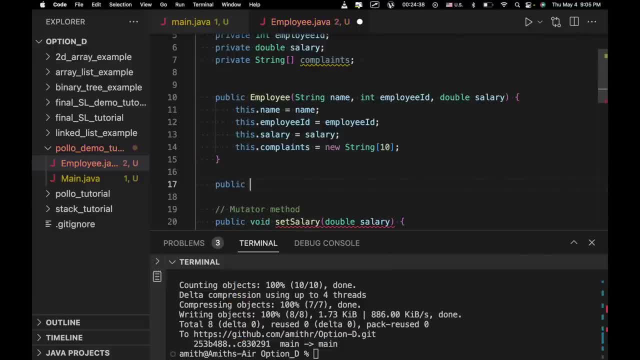 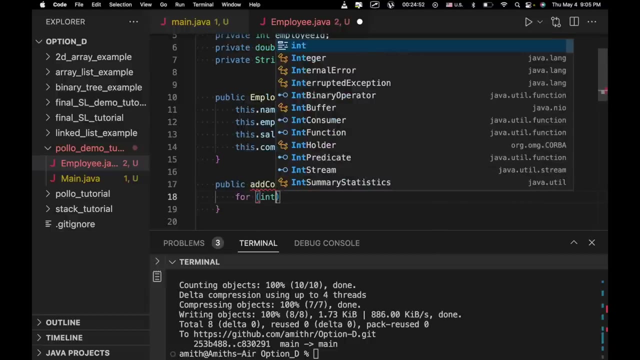 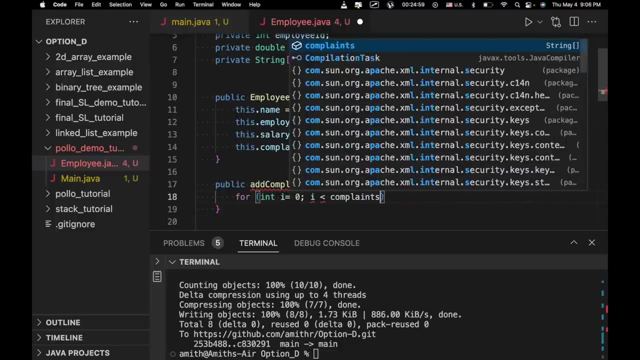 We're going to say public add complaint, String complaint, And then we're going to go through the array using a for loop. So we're going to say: for int I equals zero. Again- I think it's a syntax you should already be aware of- is less than complaints. 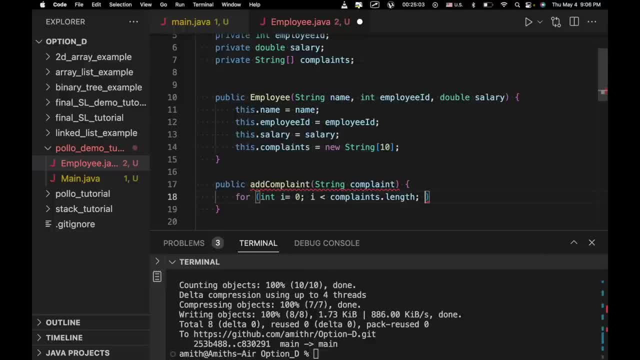 Length and I plus, plus, which is a for loop that allow us to iterate to this array: complaints right here And we're going to say: if complaints I. So we're going to look for the first Blank element in our array And we're going to set whatever complaint we want to add to that right there. 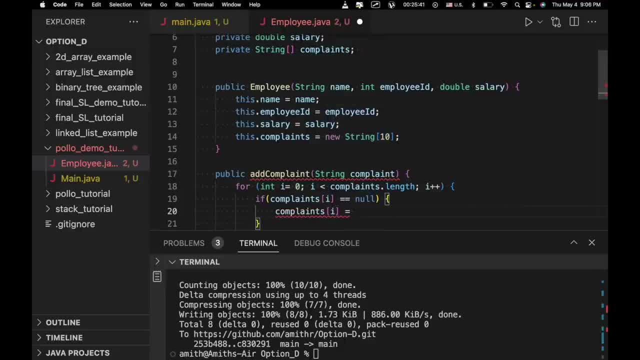 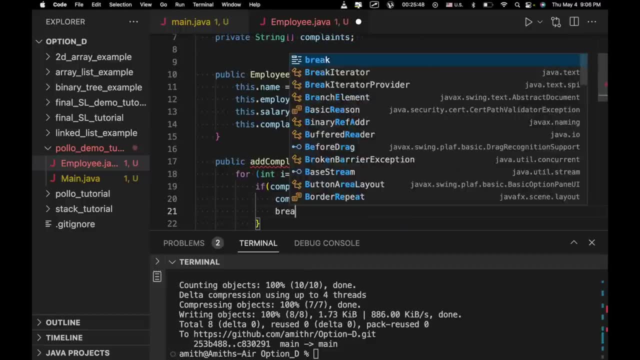 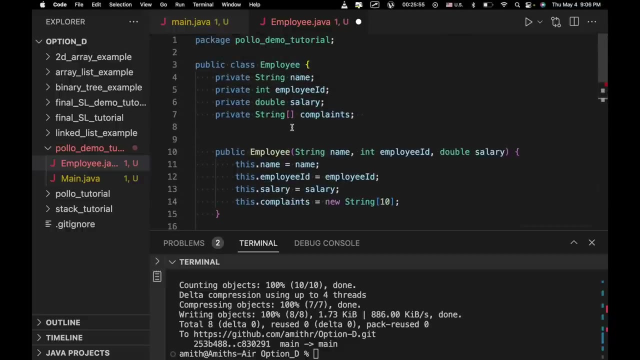 And if you understand the concept of this, if you understand the background behind the scenario, you understand why no one, none of the employees, are likely to have any more than ten complaints. Just doesn't work that way. So this is how we'd be able to add a complaint to our employee object. 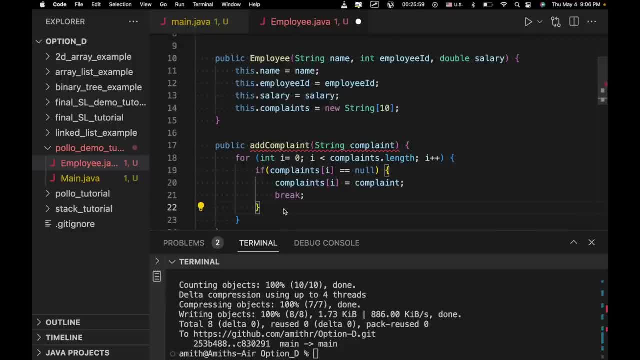 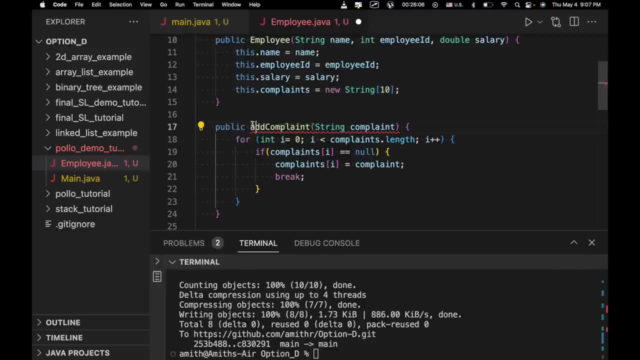 Now, so you can air right here. We have no return type, So we're not really going to be returning anything, So it's going to be void. We're just going to be adding something to the array. Now, now that we've done this, I'm going to give you an idea of how we can actually go about using these methods and what this really means in a more pragmatic context. 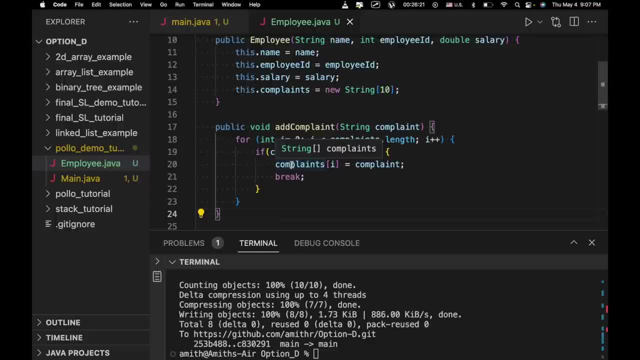 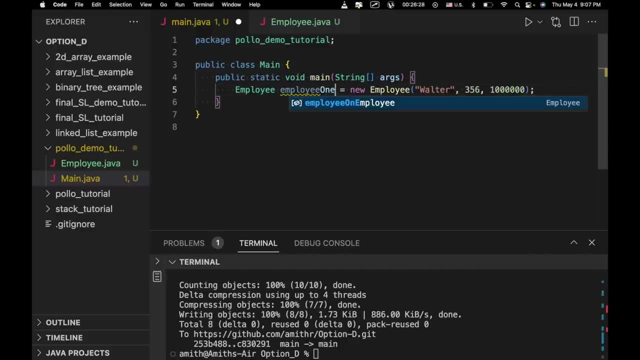 So right here we actually went ahead and we created this object from our class. We're going to give that a more appropriate name. So now some things we can do is we can access information. We can add information to our object. So one of the first things I want to do is I want to add a complaint about Walter. 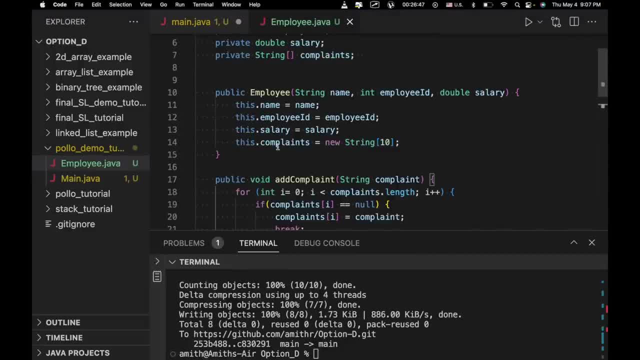 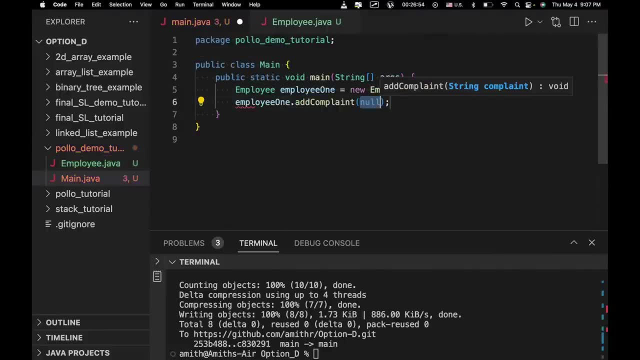 So I'm going to use that add complaint method that we just created right here And I'm going to say: employee one dot, add complaint. And then, yeah, scarily smart It's, I don't know. I don't know if that's a complaint, but I think so. 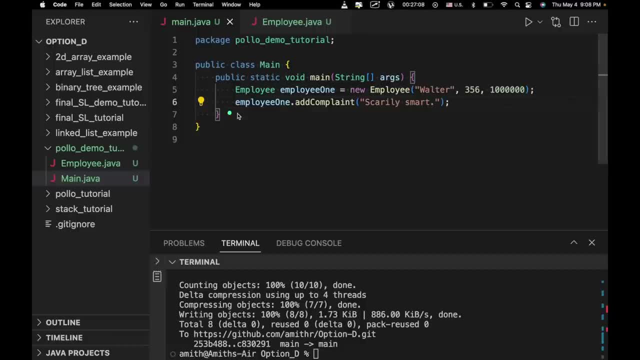 And yeah, I mean that's pretty much as adding a complaint, So we added that complaint. What I also want to do is I want to try to get some information about Walter from this object that we just created. So I just want to get his salary and print it out. 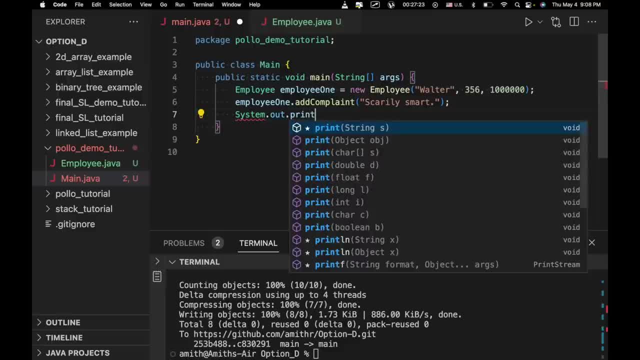 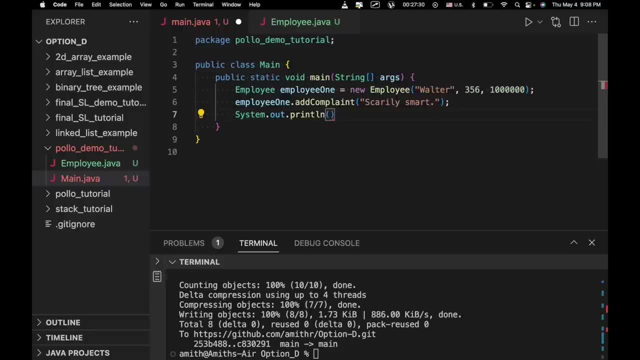 So I'm going to do system dot out dot print line And I'm going to do employee one And then we're going to get our method. We're going to have get salary. We'll just get a salary, see if we can print it out. 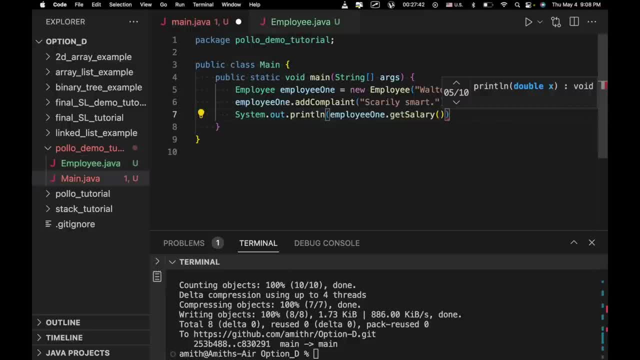 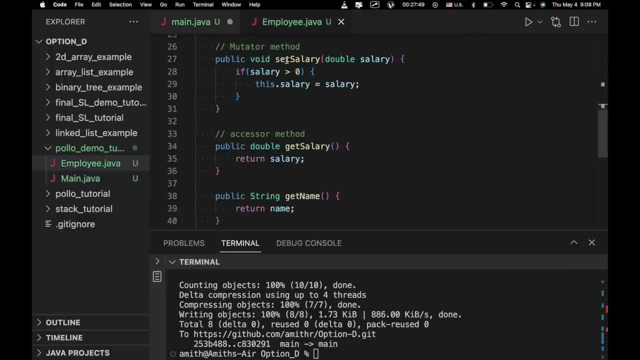 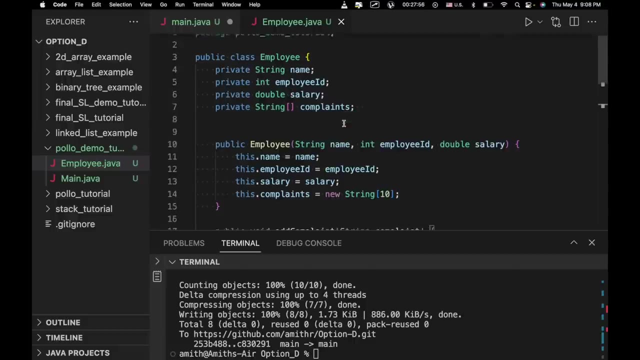 So dot get salary, And I think one of the other things I want to do is I want to write like: so our complaints array is private right here, which I could actually change, But I think I'm just going to add a method instead that is like public void or a public string. 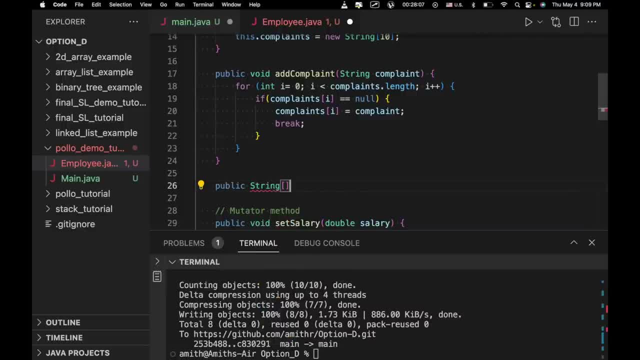 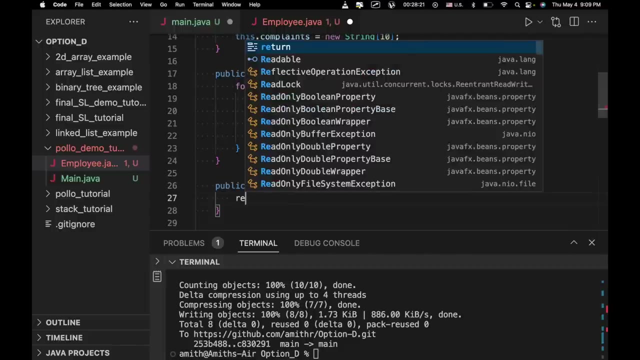 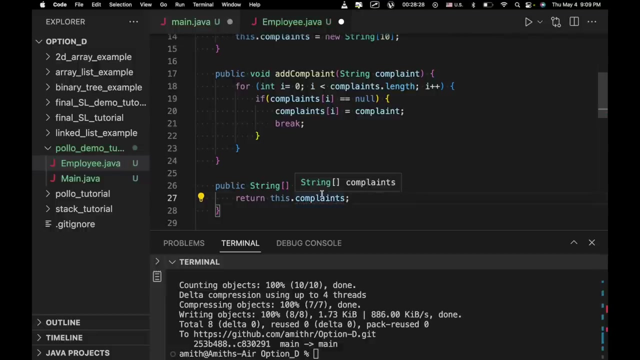 No, I guess be public string, because we're returning a string array, Get complaints- Okay, but then let's return and then I'm going to return this dot complaints. So basically, in the context of this right here, I'm returning whatever complaints arrays attached to the object we're working with. 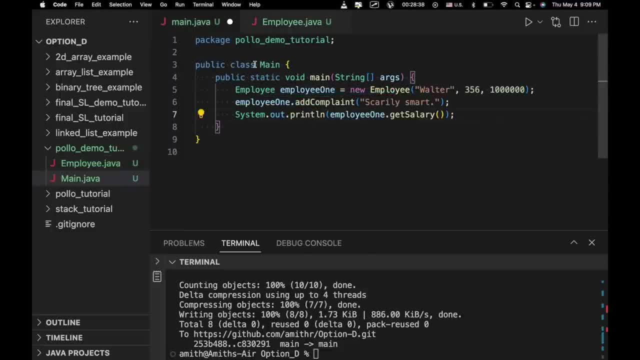 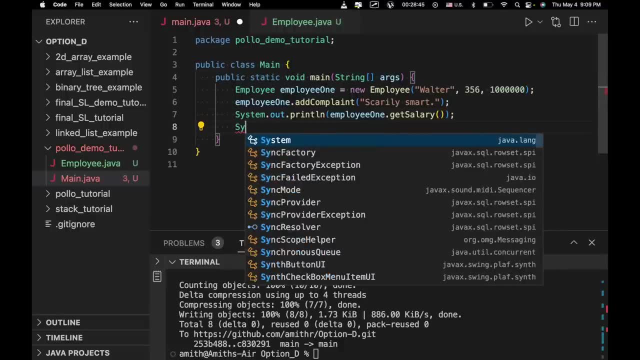 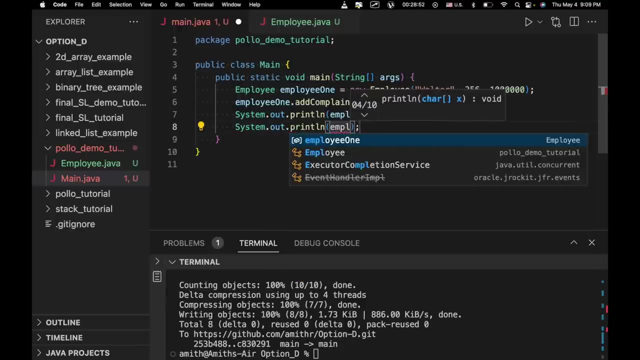 So we're going to see all the complaints for this particular object right here. So probably what I could do is I could also do system dot out, I print line and then I'm going to say: employee dot, get complaints and that's going to just going to return an array. 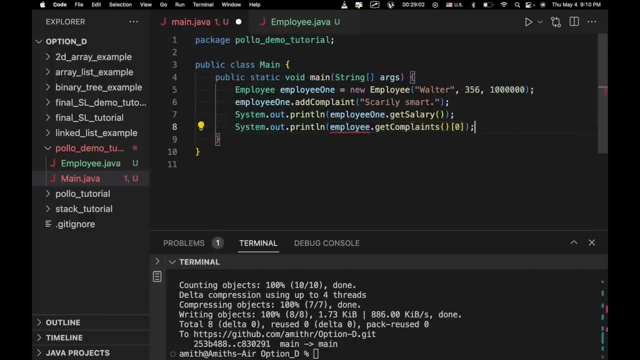 So I'm just going to. if that's going to return array, I'm just going to get the first element in that array. It's going to be employee one. Okay, cool. Now one of the beauties of working with Java and not pseudocode is we can actually like run this in a machine. 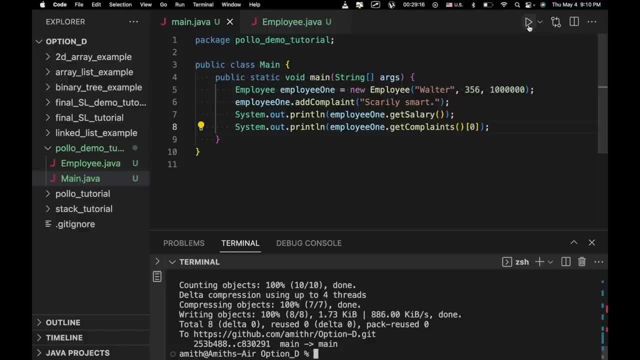 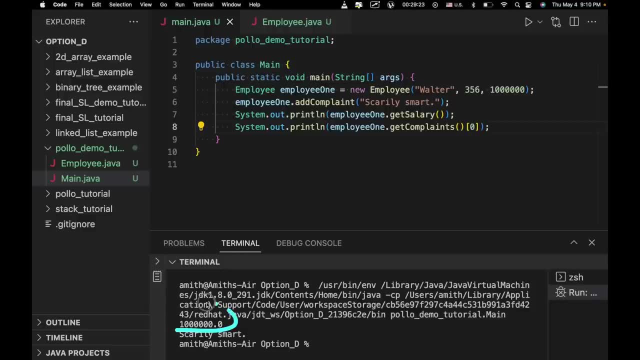 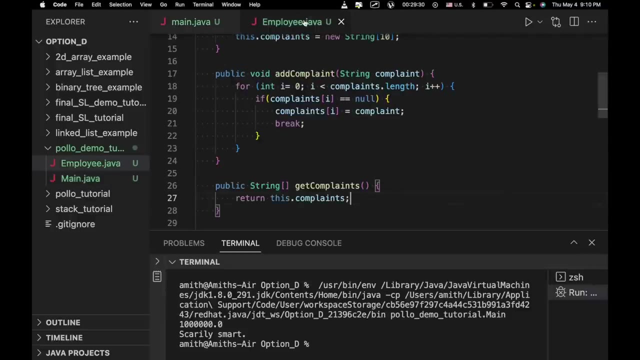 Let's get. so let's give it a try. Odds are there'll be some errors, but that's part of learning. Okay, right here we have 1 million for the salary. We have scarily smart for our comment. So that's a basic introduction to how to write a class. 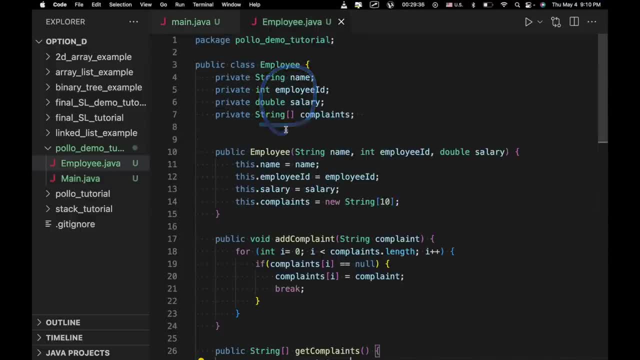 Just to recap, we have our class attributes. We have the pieces of data that will be attached to every object that we create from our class. We have our constructor, which is just a method that has the same name as the class, And that 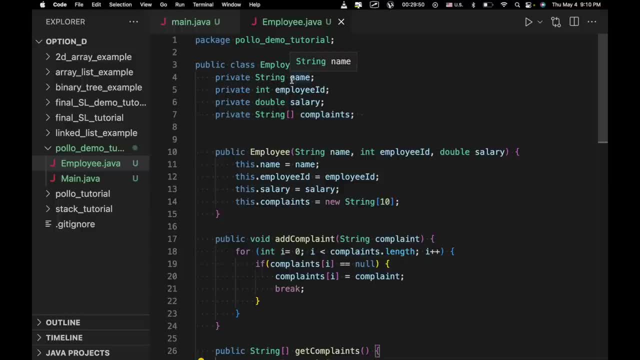 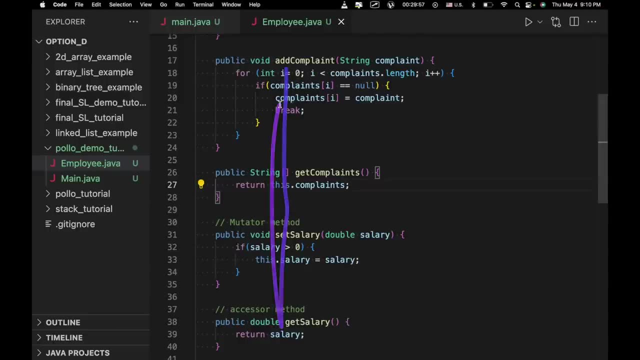 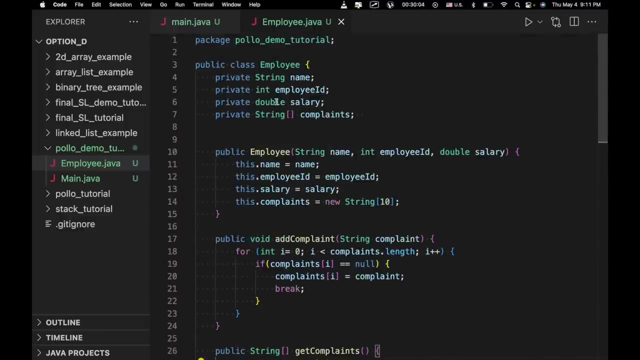 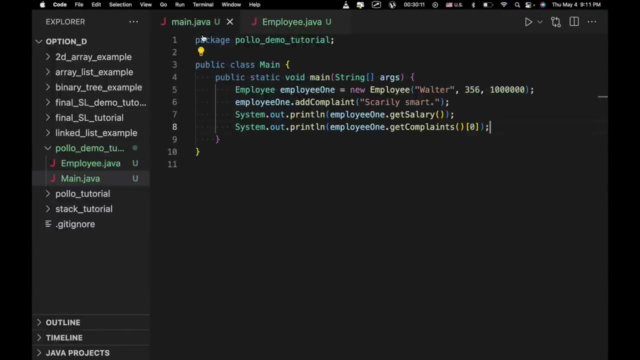 Is initiated or executed when we create an object from a class, and we have we have methods that are attached to our class that allows us to access or manipulate the data on the object that's been created. Furthermore, what I want to say is that this process where we create an object from a class, so what was taking place in this line right here that is called instantiation. 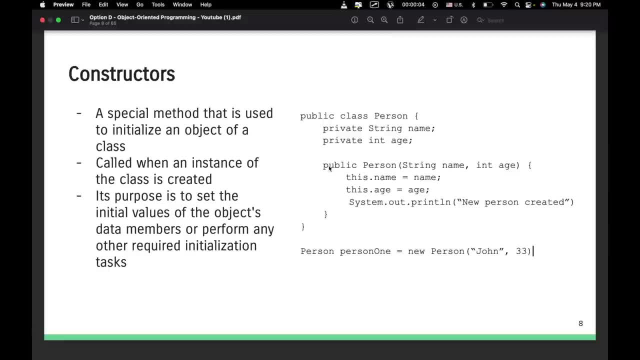 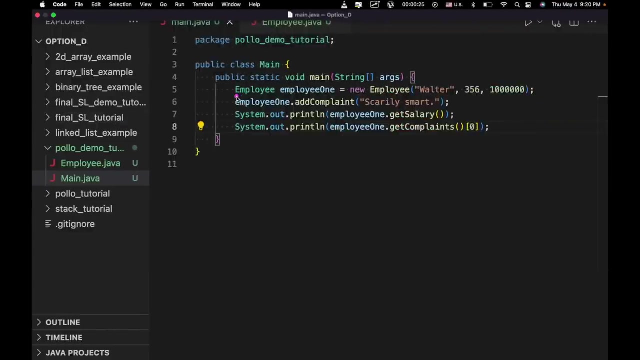 Okay. So Now that we've had sort of a practical introduction to what object oriented programming looks like, let's talk about some of the concepts that we just went over in a more theoretical sense, and we talked about constructors. a constructor is a special method that is used to initialize an object of the class, so when we looked at it in our code, I basically described it as a method that's called when we create an object in the midst of instantiation. 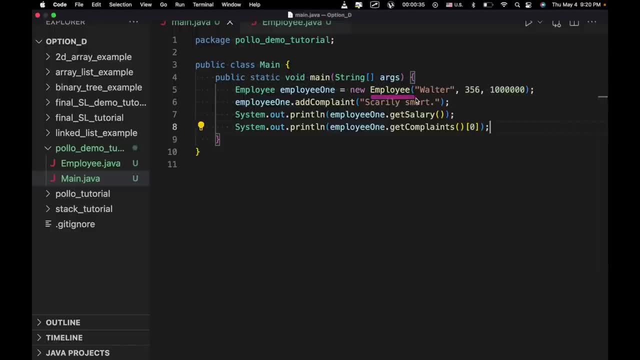 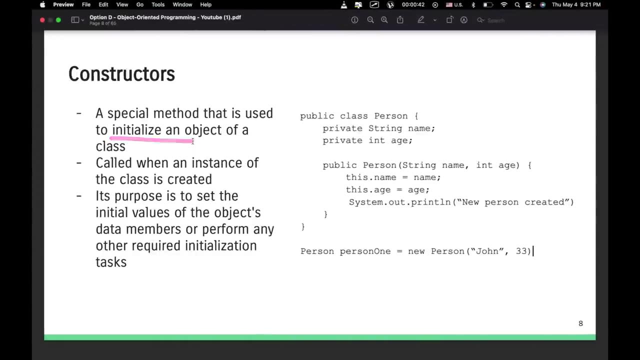 In the midst of creating an instance of an object from a class, And that is basically what we mean when we're talking about initializing an object, basically creating or starting an object. Now it's purpose to set the initial values of the objects, data members or perform any other required initialization tasks. 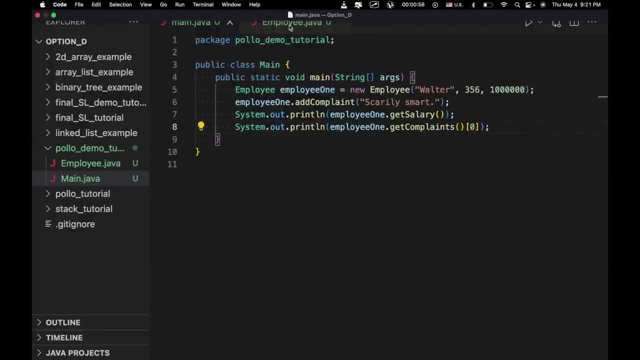 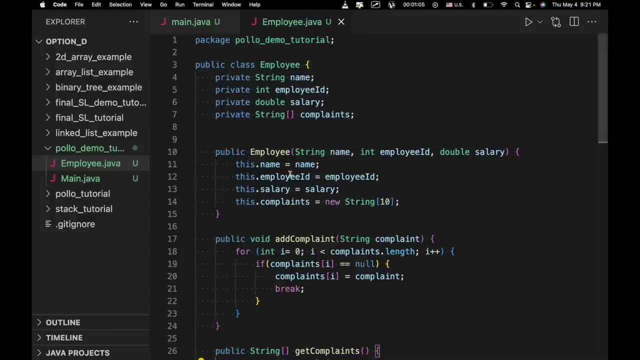 So in our example, right here we- if I can just fix this window- right here We did actually set the attributes, the initial data, members of an object. so, for example, when we created this Walter object, right here we set the name equal to Walter, the employee ID equal to whatever it was and the salary equal to whatever it was. we set complaints equal to an empty string array. 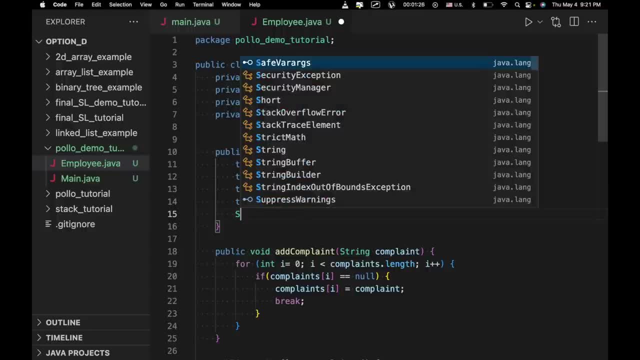 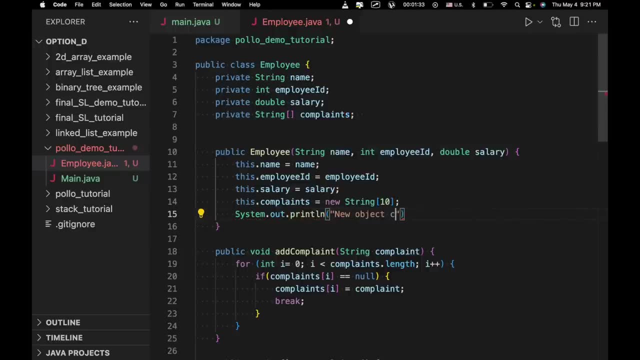 We could have also done something else, like we could have done systemoutprintln and say: new object created, And this is a function that would take place any time, or this is a line that would be executed any time we create a new object from an employee class. 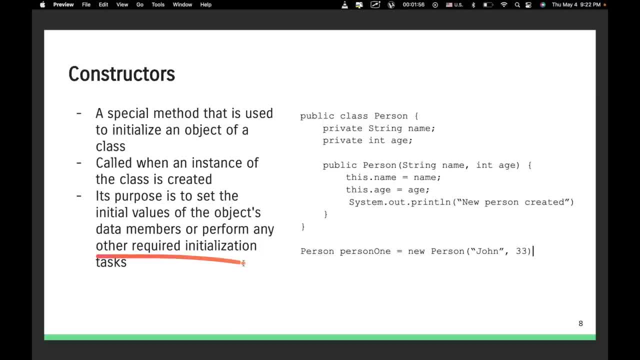 And that's an example of what we mean by any other required initialization tasks. So if you look at this example right here again this is kind of a repeat of what we just looked at- We have a class called public class person. We have two data attributes, or you can call them class variables as well. 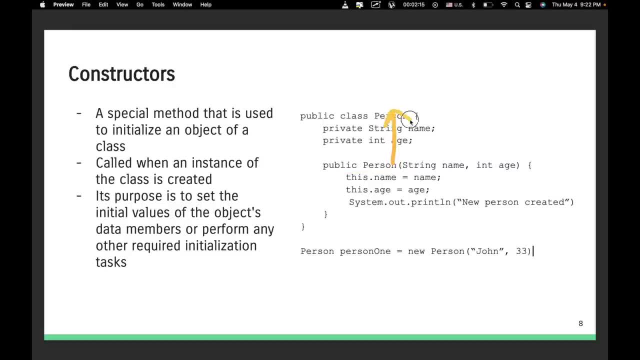 We have our constructor right here. notice that it has the same name as the name of the class. We have two parameters for that particular constructor And we are setting our class attributes equal to whatever parameters were entered or whatever input there was to that constructor. 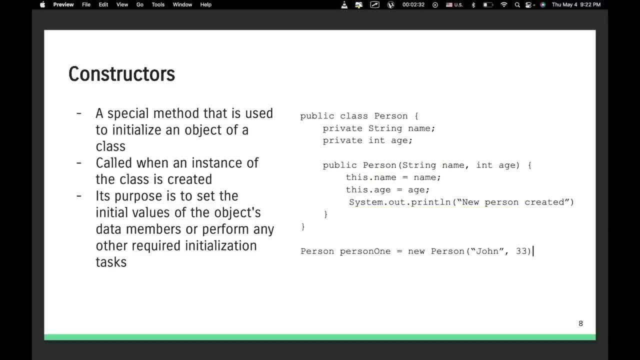 And we also have another line of code that we're just running And this is how we would go through with that process. So this constructor right here is exactly what's being utilized right now. This constructor right here, John, would become name, 33 would become the age, or 33 would be the age, and so forth. 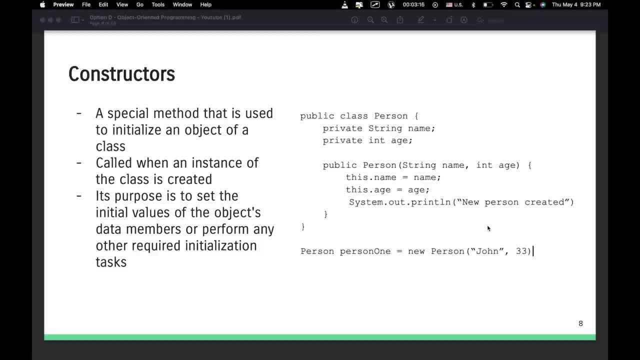 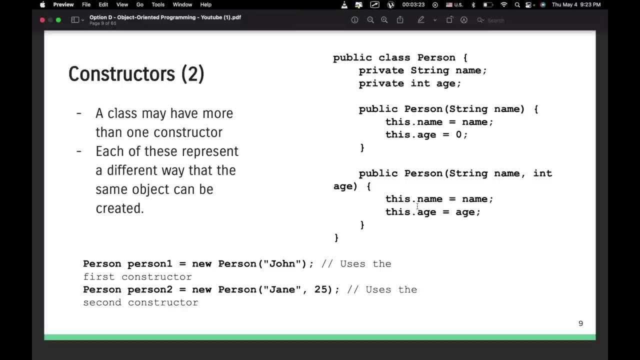 So then? so that's basically an overview of how we use constructors and what the role is in instantiation. Now, next, this is just another example. So one thing that you should know is a class can have more than one constructor, And these can both be used to create a new object. 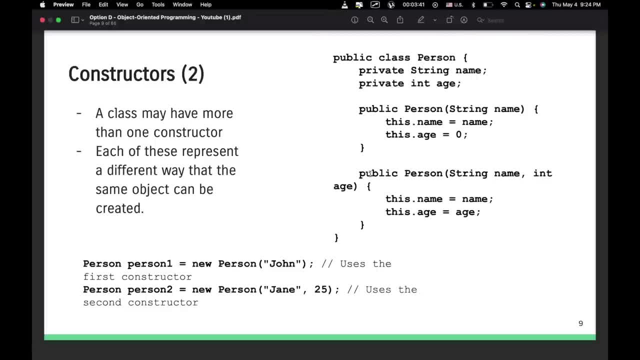 But which one is used is dependent on the parameters that are entered in when we're instantiating or creating an object. So right here we have person. person one equals new person, John. We have one parameter, which is name. So we're going to use this constructor right here, which has a parameter. it just has one parameter. 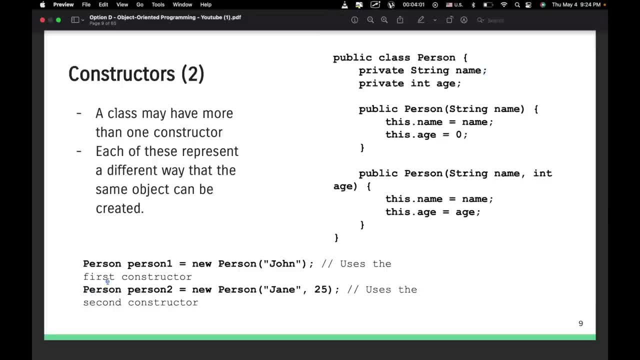 All right Now. right here we said person again. same Same class, same object. person two equals new person. but here we have a string as input and then we have an integer matching this constructor right here. So this is the one that's going to be used. 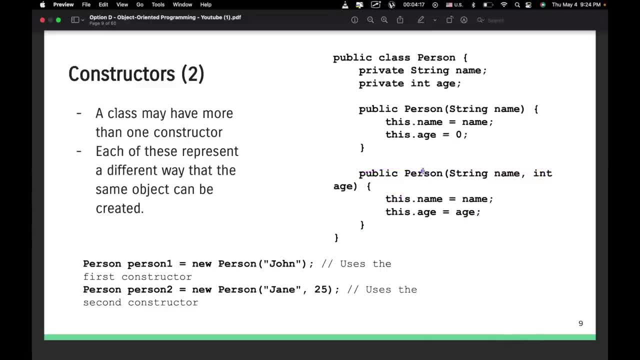 So both these constructors look the exact same, Their their method, the name is the same as the class, but they have different types of parameters, And that determines which constructor is being invoked or used. Now, this isn't. this is. 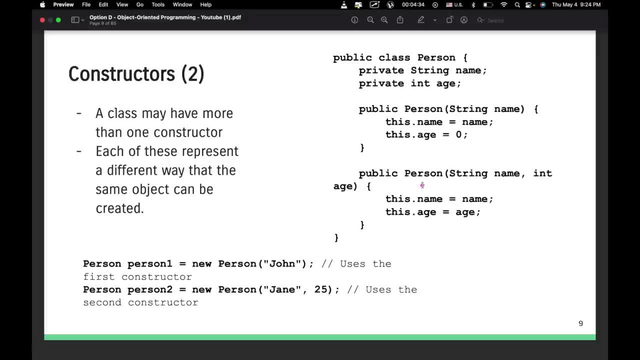 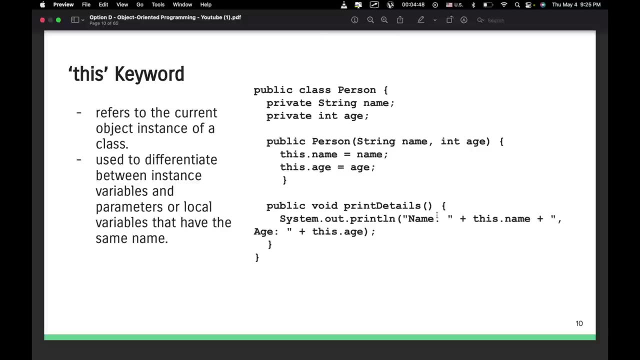 This is also an example of something called method overloading, this idea of having methods with the same name but different parameters, and we're going to go over that in a letter in a later slide. And the next concept we want to talk about from a theoretical sense or a theoretical perspective is the this keyword: 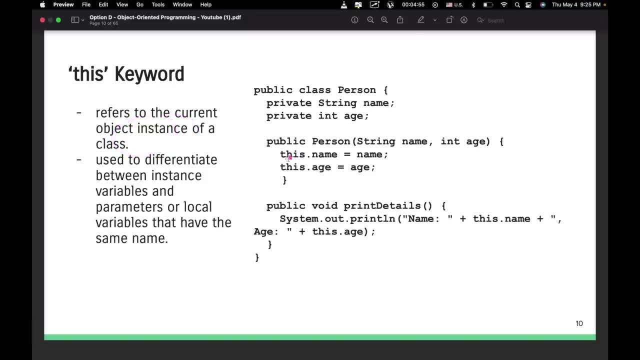 So it refers to the current object instance of a class. So right here we had: this dot name equals name and this dot age equals age. So this is referring to the attribute That's associated with a given object. And these names right here are just, are just parameters in this method and don't exist outside of this constructor method. right here. 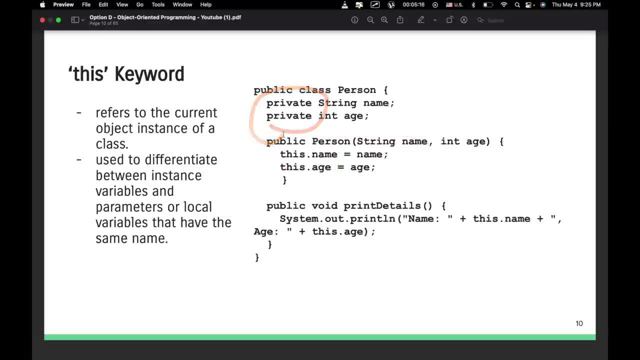 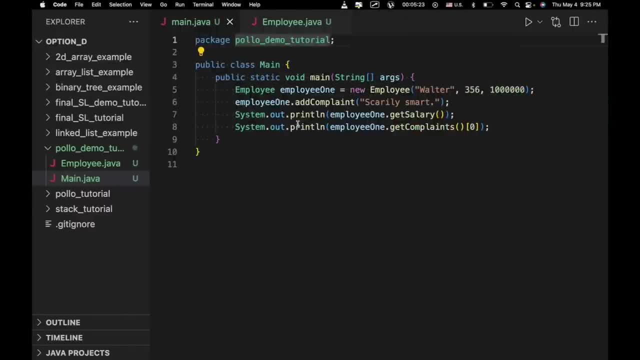 So now we're using this, we're talking about these attributes that are specifically associated, um with the uh object, or with the class or with the object that's been created. So, for example, for this object right here, um, this dot name would be Walter. 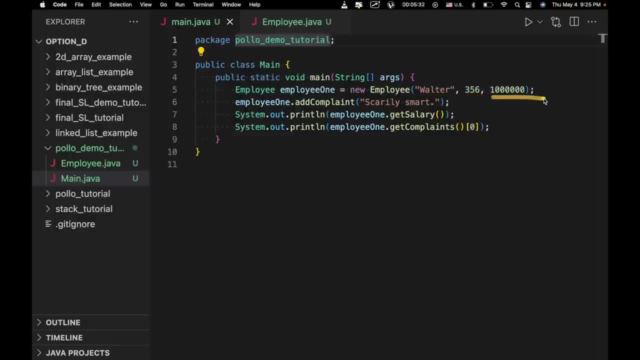 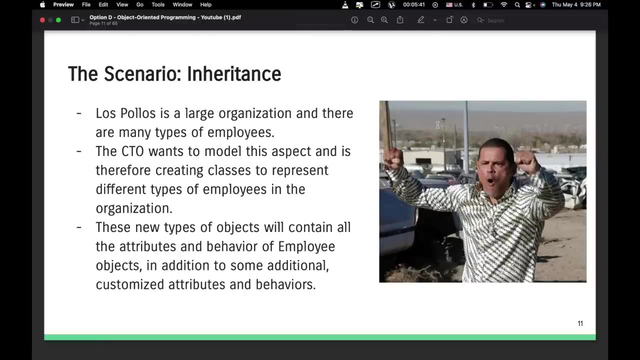 This dot employee ID would be three, 56. And this dot salary would be 1 million. Now let's look at the next step in our scenario. So this is going to involve a con, a concept called inheritance. Now, Los Pollos is a large organization and there are many types of employees. 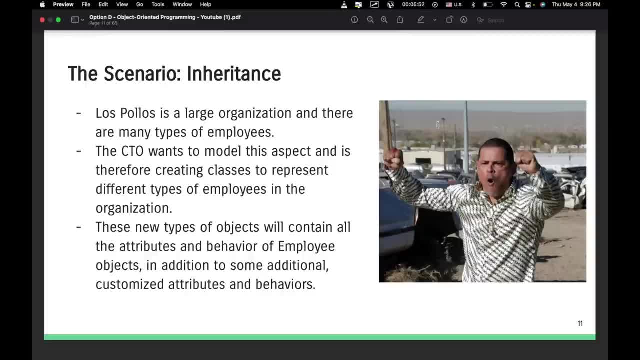 The CTO wants to model this aspect and is therefore creating classes to represent different types of employees in the organization. Now these new types of objects will con will contain all the attributes and behavior of employee objects, In addition to some additional customized attributes and behavior. 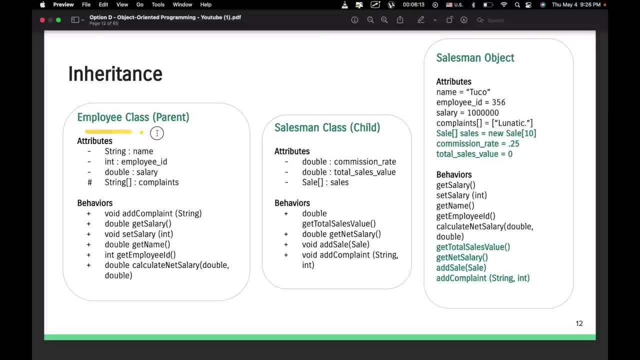 So, right, here we initially had the employee class. Okay, now we're going to create what's called a subclass or a child class of our employee class. So that refers to a class that has all of these in addition to its own, to its own distinct attributes and methods. 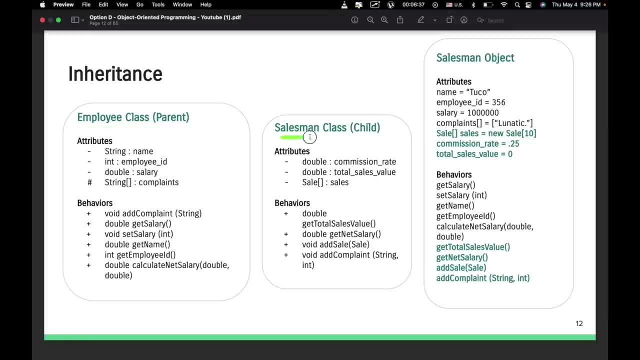 So if employee class is the parent, we're going to create a new class called salesman class. That's going to be a child, and a child is going to have these attributes and these methods, in addition to everything on the employee class. So here, when we create an object, a salesman object, this is what it's going to look like. 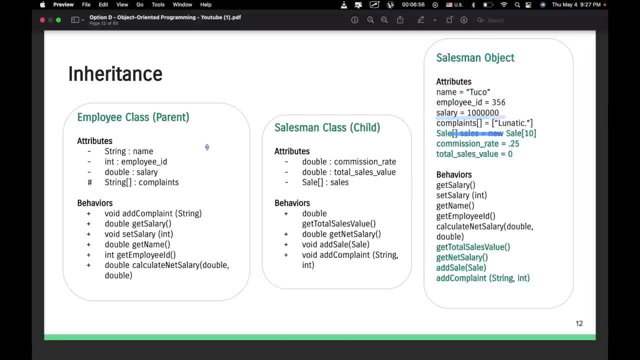 We're going to be able to set our name or employee ID, our salary and our complaints from our employee class, but we can also um set our uh, a sales array, A Commission rate and a and total sales value, because those are associated with the salesman's class, salesman class, and there are salesman object. 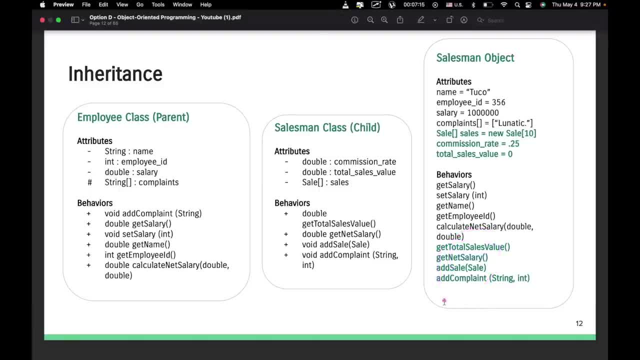 We'll also be able to access all of these methods, or we'll also be able to use all these methods with our salesman object that are on the salesman class, In addition to all these methods associated with the employee class. So let's go ahead and let's write some code so that we can see what that, see what that really looks like in practice. 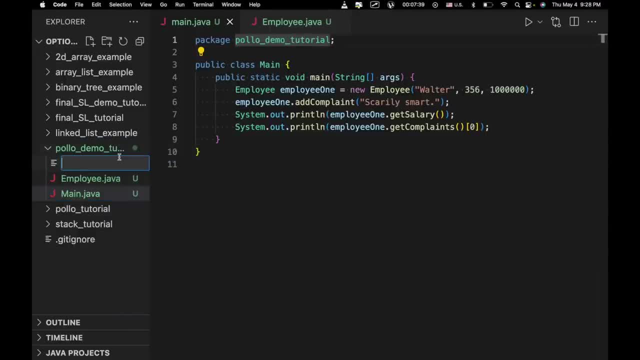 So what we're going to do is we're going to create a new file called salesman dot Java, because we're going to have a class called salesman And in this class, right here, we're going to have a double uh variable called commission rate. 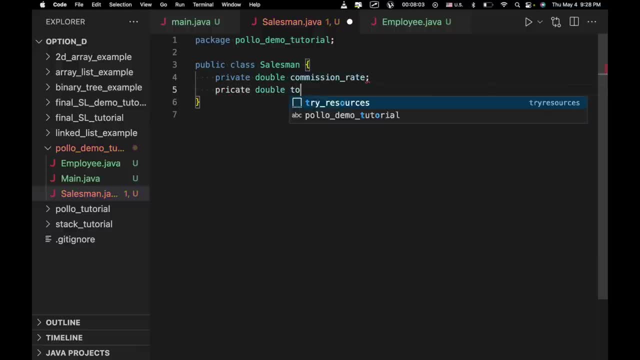 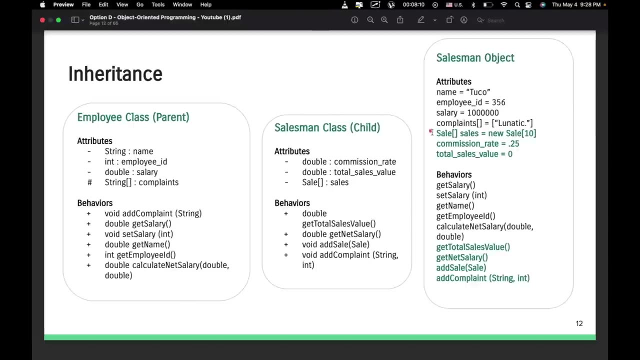 We're going to have a uh double variable called total sales value, And we did actually have this sales array, but I think we're going to leave that off for now. We'll get to that in a second. So we're just going to have these two for right now. 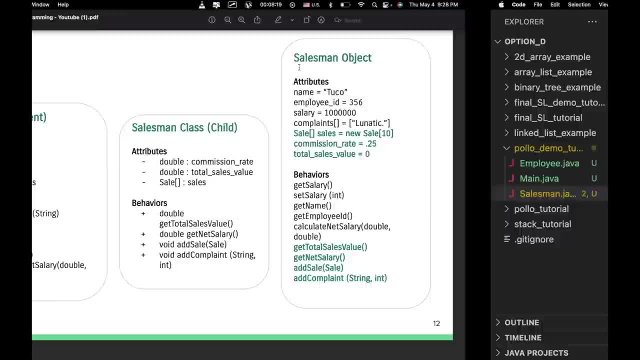 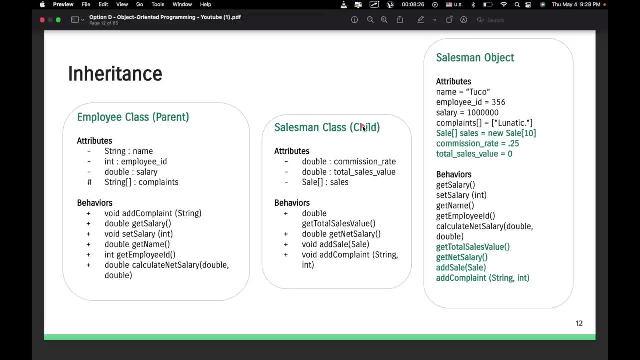 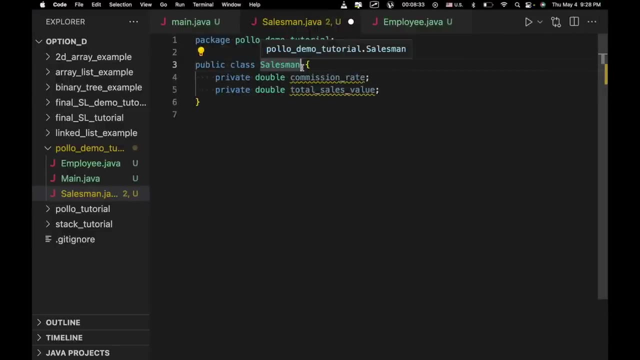 Um, and in order to establish this relationship between our parent employee class and our child salesman class, so that salesman gets all of the methods and attributes of the parent In addition to having its own, we're going to do public class. salesman extends. 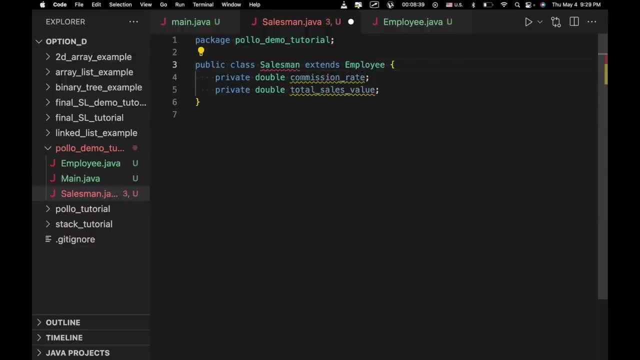 And then we're going to have a public class salesman, And then we're going to have a public class salesman. So we're going to have a public class salesman And then we're going to have a public class salesman. Now that's weird. 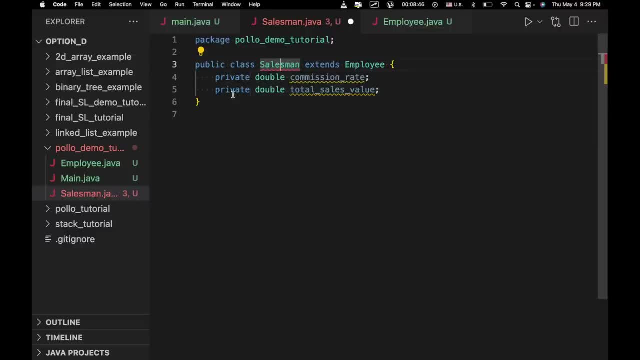 Why does it have a red line over it? Okay, Yeah, It doesn't have a constructor. Okay, So next thing we're going to do is we're going to create a constructor. So that's always going to happen in a class. 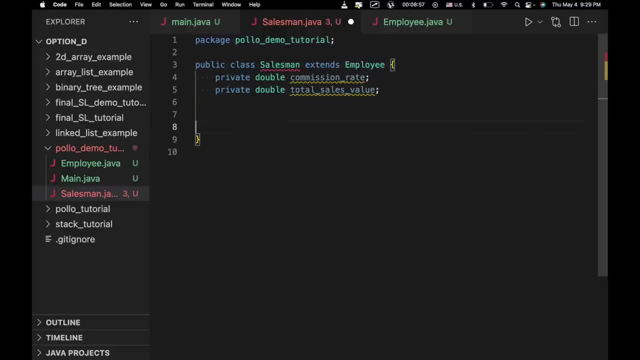 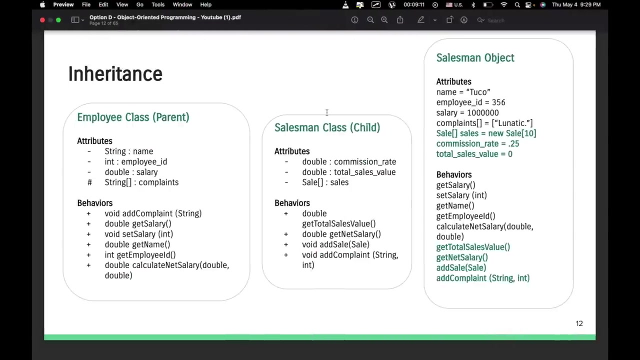 So we're going to say public class, our public salesman, And we're going to have several inputs. So when we create a salesman class, we're going to have a public class salesman. We don't just want these three, but we also want an additional input for our commission rate. 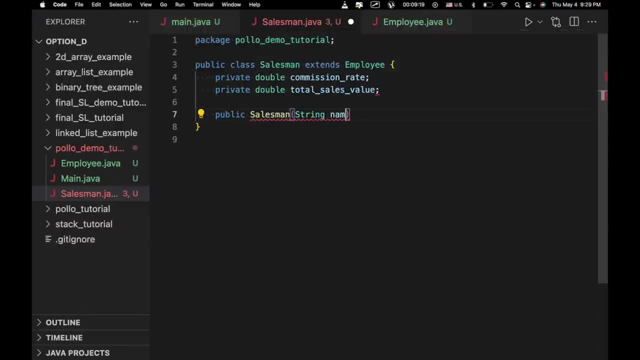 So we're going to have a string name: int employee ID. Actually, I want to change the style of these, So we're going to make that commission rate and total sales value. Anyways, we're going to have int employee ID, double salary. 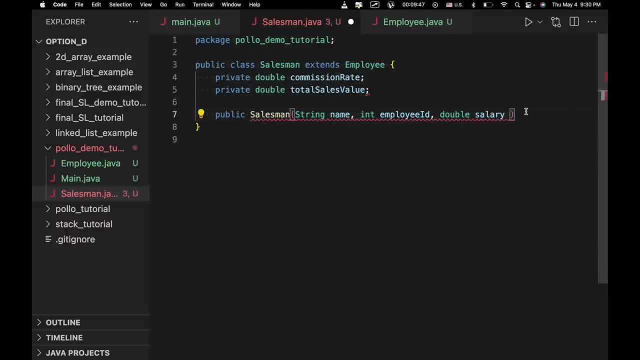 And we're going to have double commission rate, And I'll just do that right there, And then we're going to actually create that method. And why is this all red? Okay, And what we want to do first is we're going to do super, which actually represents employee. 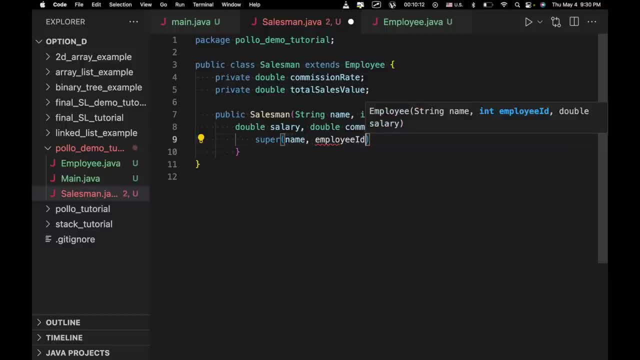 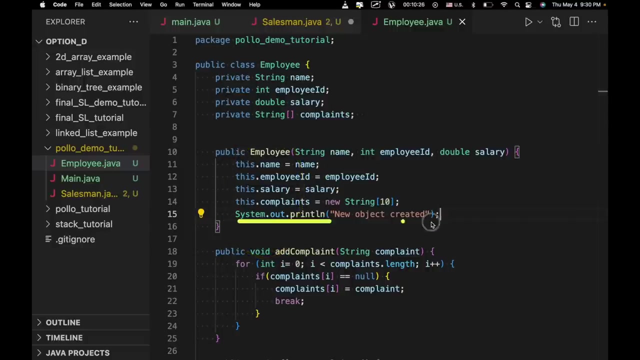 our employee class name, employee ID and then salary. And what this line does right here is this: actually invokes or uses the constructor from the parent class, So this constructor right here, which means we're also going to have this line of code. 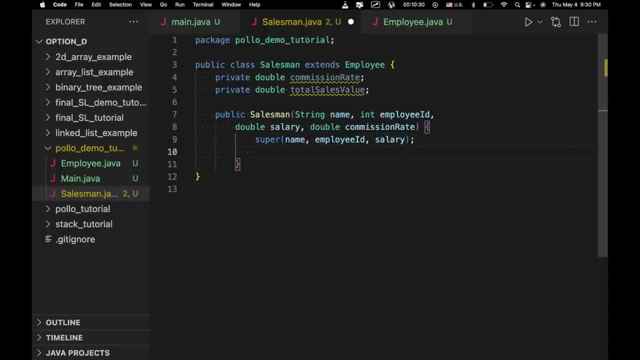 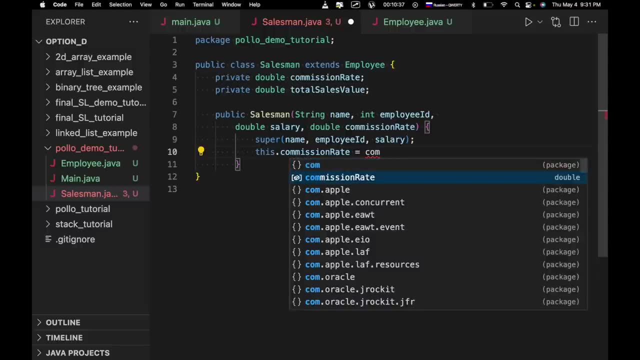 right here. So we're going to do that. And then we're going to say this: dot. commission rate Equals commission rate, So whatever has been entered. And then we're also going to do a few other things. So we're going to say this: dot. total sales value. 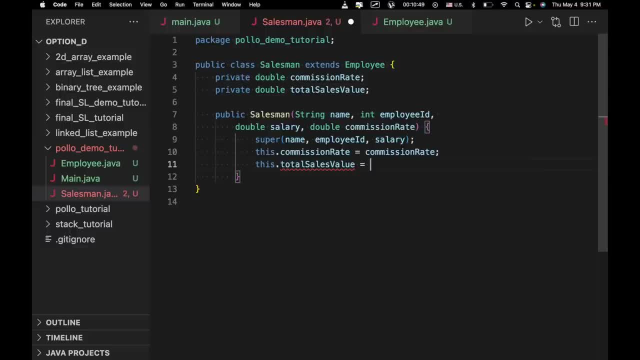 So, remember, this is a salesman, So they're going to have a total amount of money that they brought in. It's going to be zero, And for now that should be good. Now we're also going to write some unique methods, which we specified right here. 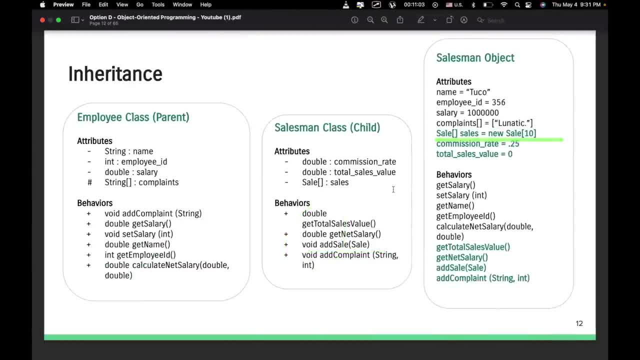 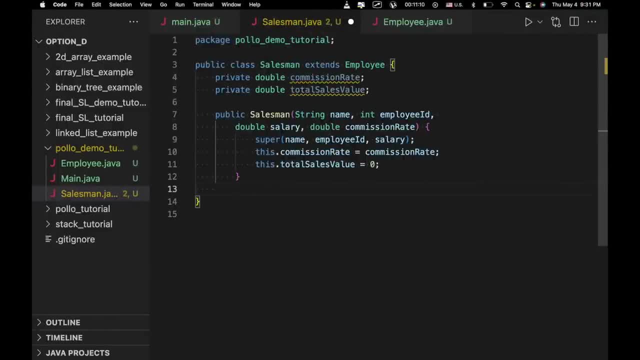 Again, we're going to leave the add sale one off. that corresponds to this array, Everything else we're going to add. So we're going to get out of our little OK. so we're going to have like double get total sales value. 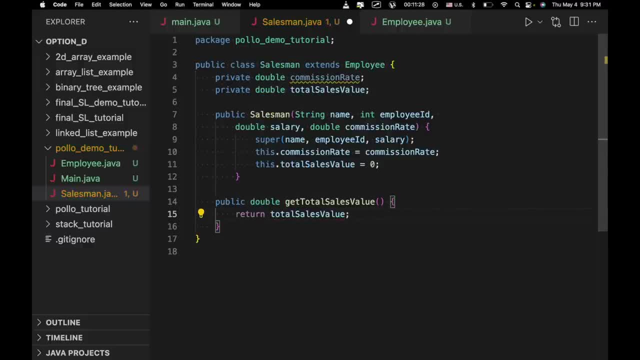 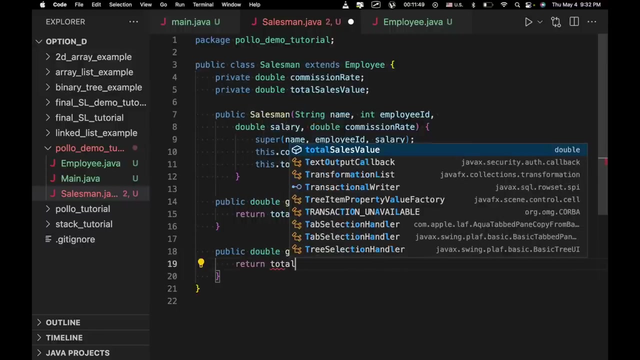 Return total sales value. We're going to have public double. we'll get net salary. that's gonna be kind of a unique one, because that doesn't actually correspond to either of our attributes. that's going to do is return the net salary, so that's going to be returned total sales value. so how? 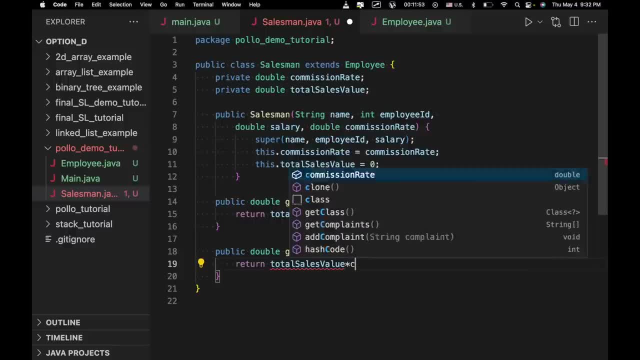 much they've brought in times, whatever their commission rate is, because that's really going to be the amount of money they're taking home and next we're going to have. yeah, we should probably have a method in order to be able to get the commission rate. so we'll say right up here: a public double get commission rate. 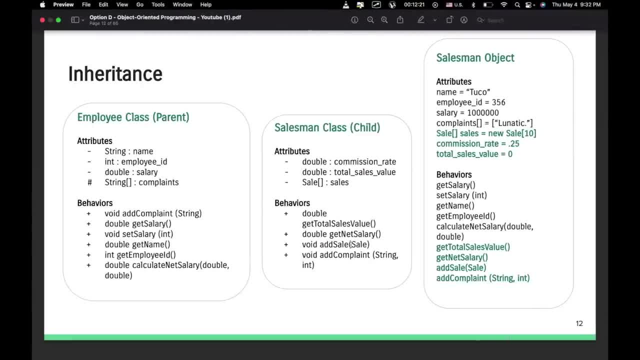 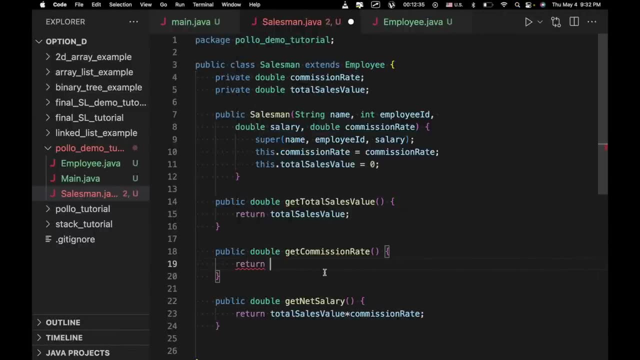 now, actually, looking right here, there are a few other methods that we all have access to, like add complaint and add sale, but we're gonna get to that a bit later because that refers to some concepts that we haven't gone over yet. okay, so, yeah, that's gonna return. yeah, Commission, right, cool, okay, so what I? 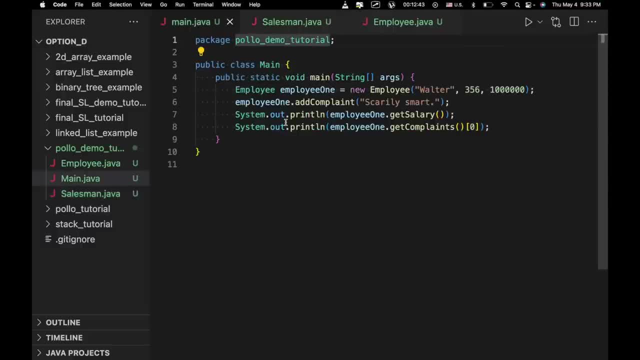 want to do now is I want to show you, like, how this actually works when we're executing some code. so so right here we're going to create a new object. we're gonna say it's gonna be a salesman type. so we're gonna say: salesman, salesman one. 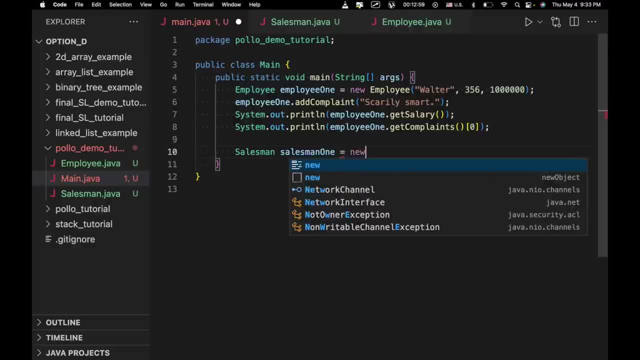 equals new salesman And we're going to input a name, so that's going to be Tuco. Well, I suppose Tuco never really worked for Los Pollos. but whatever His employee ID is going to be 666, for obvious reasons. 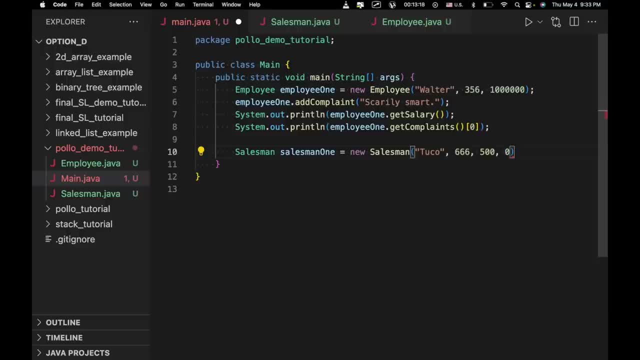 He has a salary of $500,000 a year- I don't know, I just made that up- And then he has a commission rate of 0.75.. Seems appropriate for a complete lunatic, And okay, So now that we've done that, we can access this as any other object. 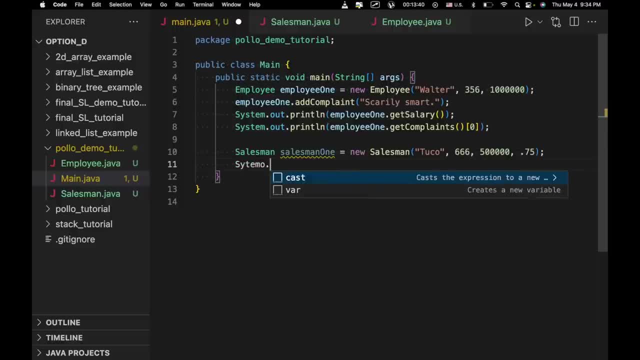 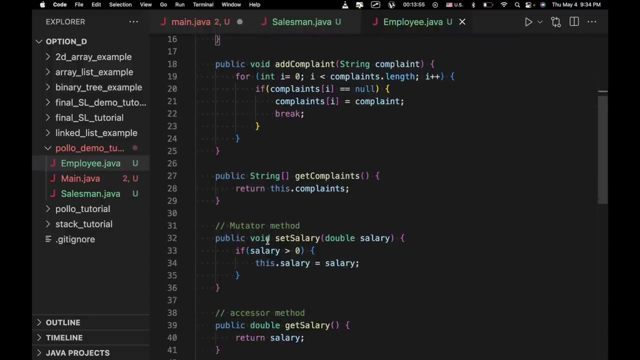 So we're going to start by just accessing a. So this is a Salesman object. But just to demonstrate that this is a child class of Employee, we're going to access a method from the Employee class, So we're going to access getSalary. 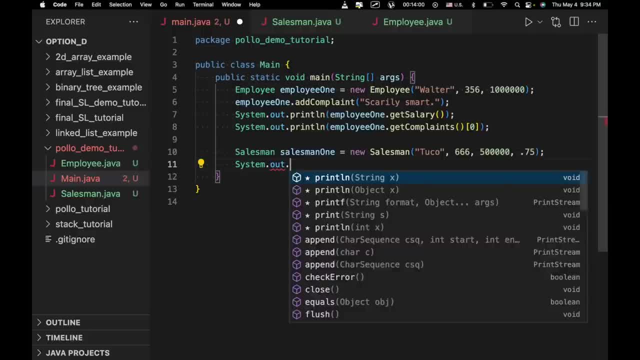 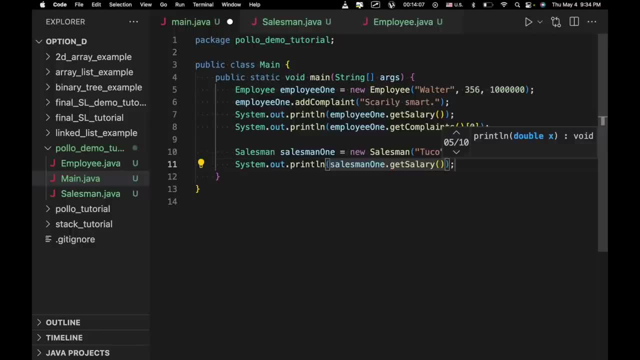 So we're going to do SystemoutprintLine, just so you can kind of see how it works, And then we're going to do Salesman1.getSalary, And then we're also going to use a method that's Salesman-specific. 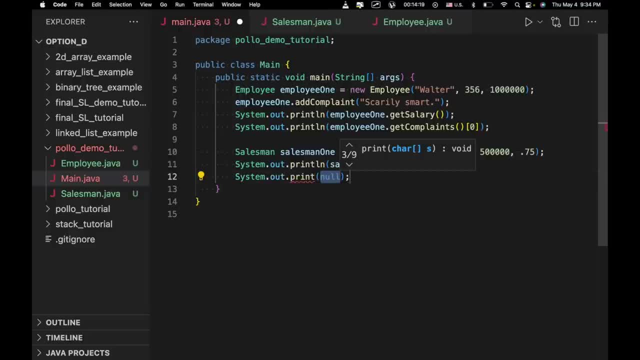 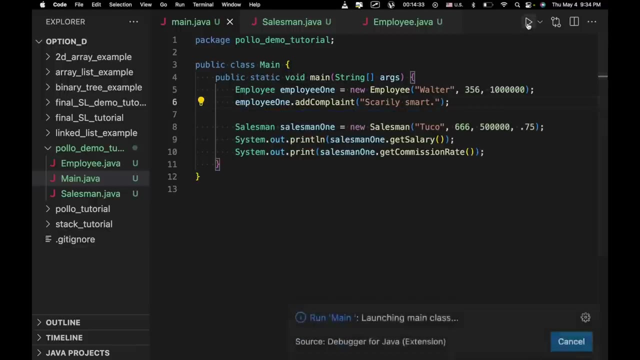 And we're going to say Salesman1.getCommissionRate- All right. So we're going to backspace these because that's not really that relevant to us right now. So let's go ahead and let's run this, All right. 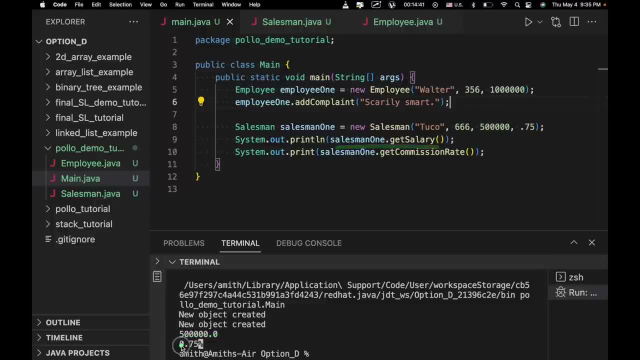 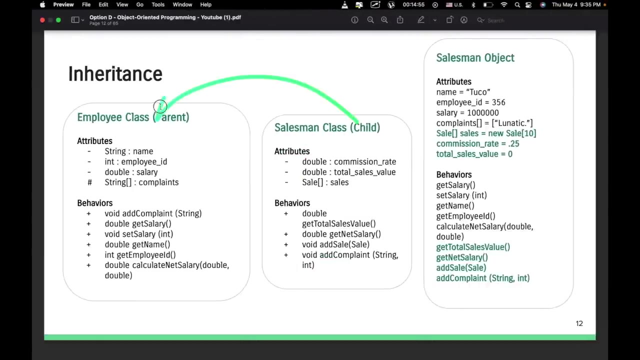 So we got 500,000 for Tuco's salary And we've got Tuco's commission rate right here, And that is a basic application and demonstration of inheritance, a concept called inheritance. Now, Salesman class was a subclass of our Super class. 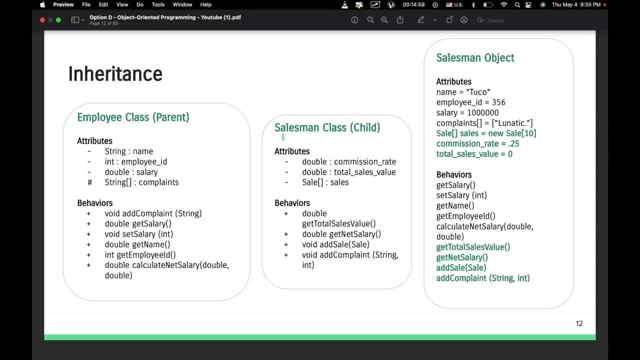 So we had a single employee, Salesman, inherited all of these attributes and these methods so that we could use them in a Salesman object in addition to the methods and attributes specific to the Salesman class. That's a demonstration of what we call inheritance. 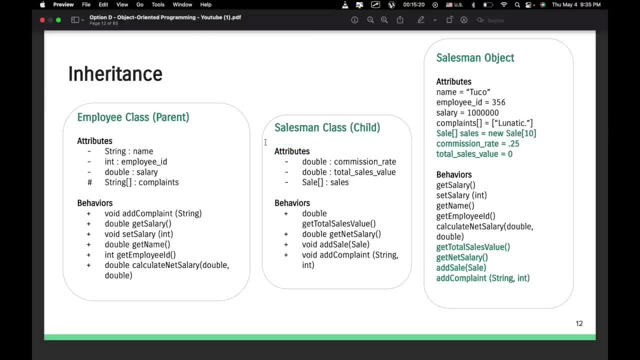 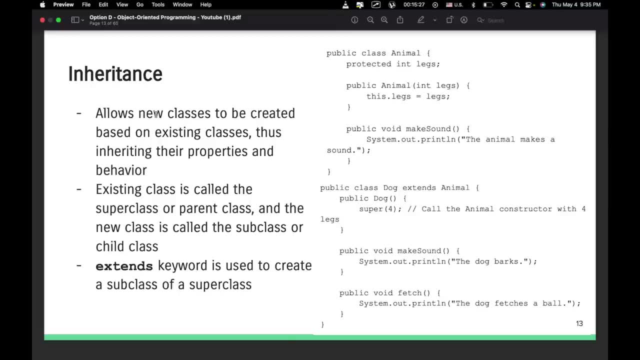 thinking about a child inheriting the traits of a parent. The best of both worlds. So, in order for us to again look at sort of the the theoretical definition, we can say that inheritance allows new classes to be created based on existing classes. 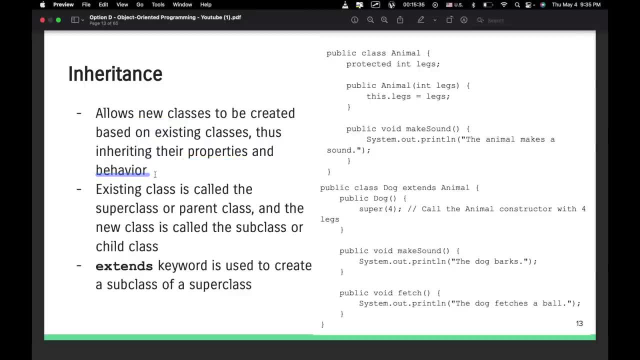 thus inheriting their properties and behavior. This term behavior refers to methods And this term properties refers to attributes. There are different names for practically the same thing, So an existing class or a parent class is also called a Super class, And the subclass can also be called the child class. 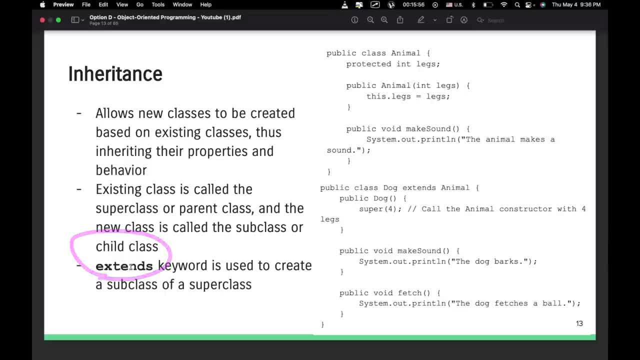 And the extends can also be called the child class. So the subclass is used in order to establish that relationship between both those classes. Now here we have an animal class. It has an attribute called legs. You have a constructor right here, And then we have a function called makeSound. 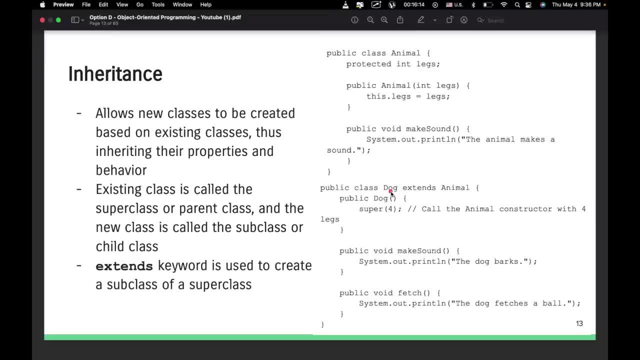 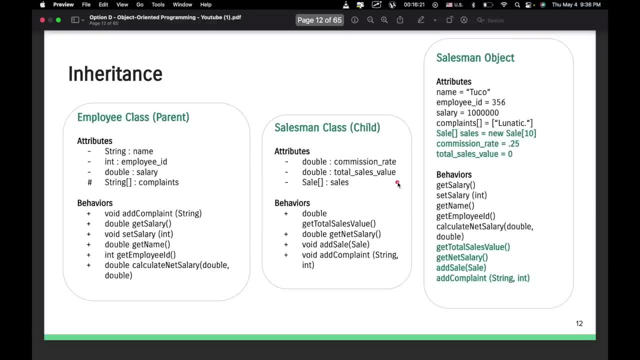 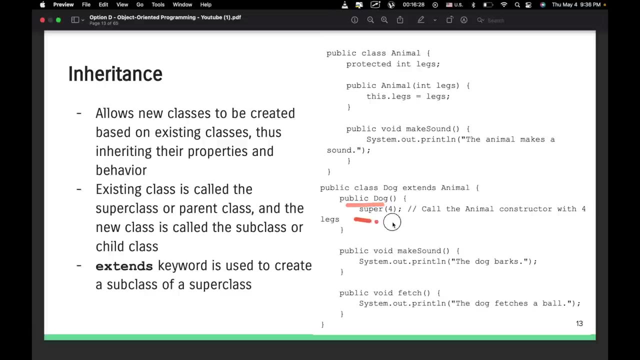 And it just prints out. the animal makes a sound, And we have dog, which inherits from animal, because dog is a specific type of animal, Similar to the way that a Salesman was a specific type of employee, And in public dog we have the super keyword. 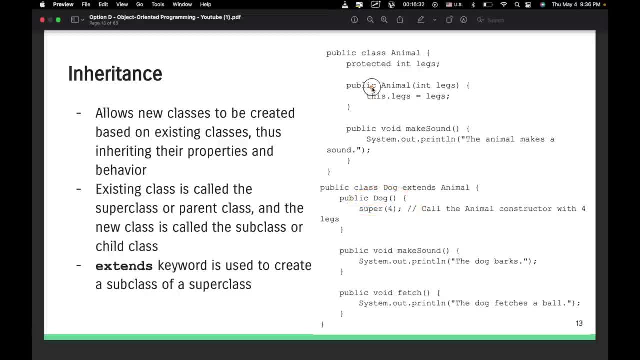 which we talked about Basically doing this right here, invoking this constructor. We have makeSound which we're going to use this makeSound. If we do dogmakeSound, we're using this one instead of this one, because we're using the dog class. 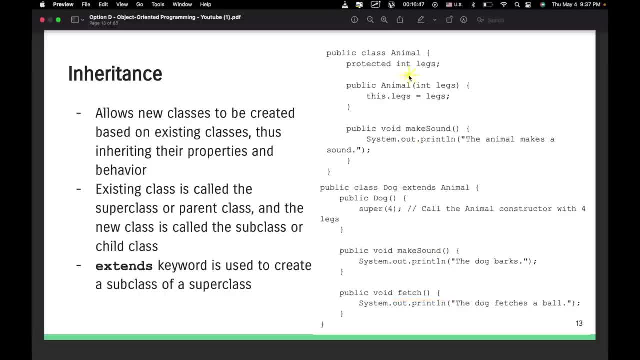 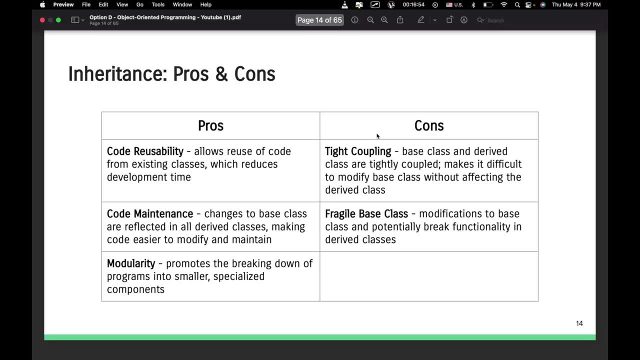 We also have a function called fetch That wasn't on the animal class and the parent class, but is here Now. this is another example of inheritance. Now, there's some pros and cons to inheritance, like everything, And this is something you do need to know for the IB exam. 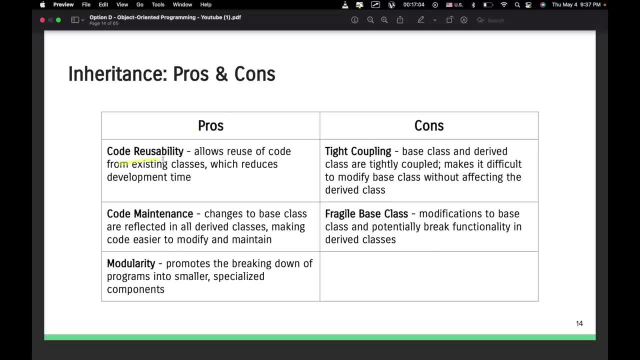 One of the pros is that it allows for code reusability. So if we want to create a new class and it has very similar behavior to a class we've created previously, we can use inheritance to allow our new class to inherit from the old class. 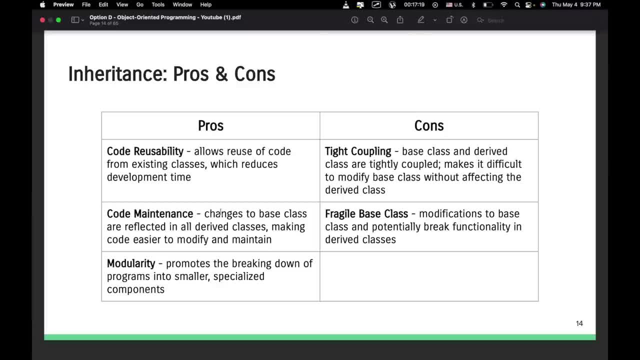 which reduces development time. Next, it makes code maintenance easier, because if changes to a class, like a base class or a super class, are reflected in all derived classes, you just need to change that one class instead of like eight different classes. So, for example, if we have an animal class, 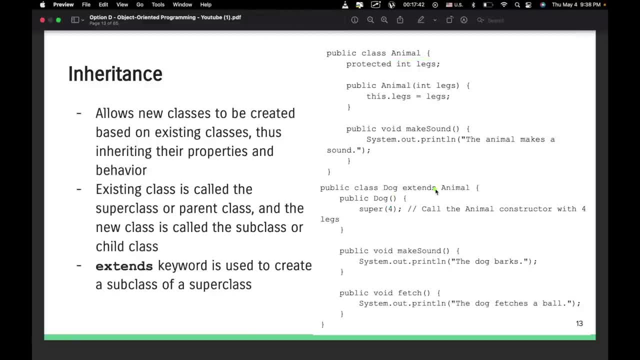 and we have a dog class, a cat class and a raccoon class. you want to make a change to a makeSound function that all of those classes inherit. You only need to edit that on the animal class instead of all three or four of those classes. 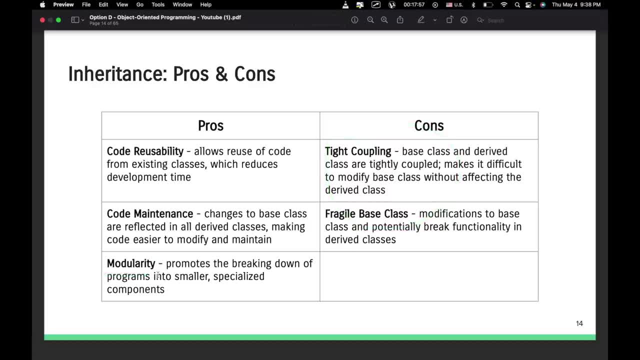 Next, we have modularity. Modularity is an advantage of inheritance, And this means that we can break down our programs into smaller specialized components, Our smaller specialized components being those subclasses, each with their own particular, each with their own specific attributes and functionality. 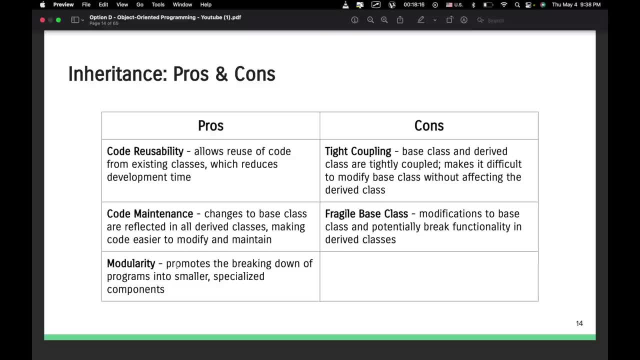 Now some of the concepts or some of the cons are tight coupling. So the problem is that when you do inherit from a base class, you are kind of stuck with that functionality And you can't modify that class without it affecting all of the classes that inherit from it. 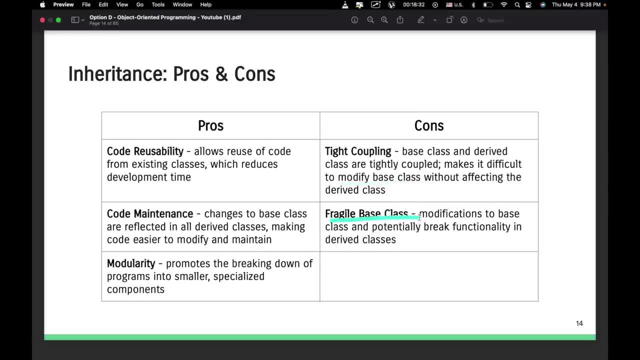 And kind of hand in hand with this particular con. if you make a certain change in your base class or superclass, you could break functionality in your child classes as well, because they make use of that. So those are kind of the same thing, but two cons, we could say, of inheritance. 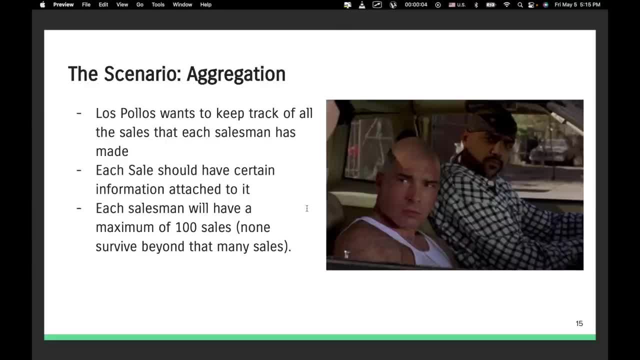 Okay, so the next concept we're going to cover is called aggregation, And let's see how that fits into our scenario Now. Los Pollos wants to keep track of all the sales each salesman has made, So each salesman needs to have information about each sale. 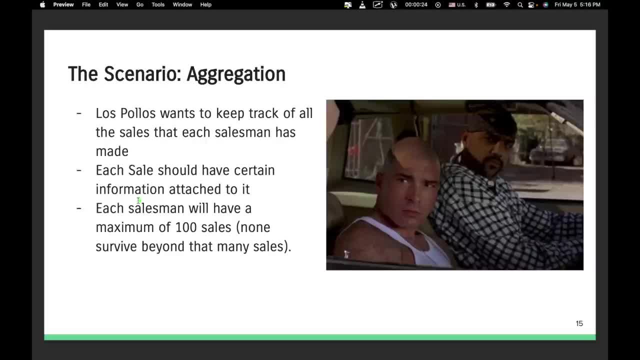 that that salesman has made attached to it. Now each sale should have certain information, as I just said, attached to it, And each salesman will have a maximum of 100 sales. To be honest, in this scenario salesmen don't really survive more than 100 sales. 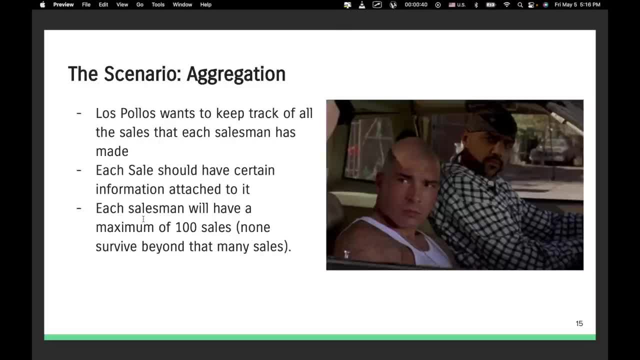 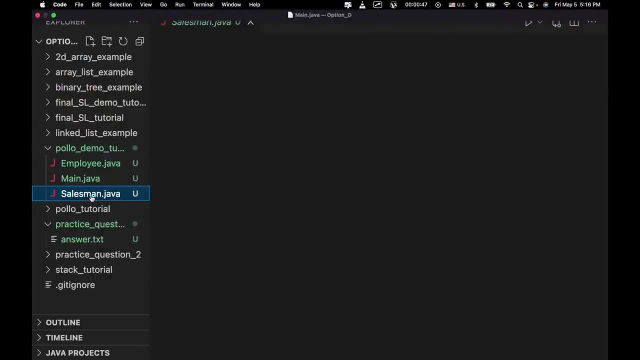 if even that, It's a rough business. So, in order to do that, what we're going to do is we're going to take a look at our salesman class. So right here, we've got our salesman class. We want to attach sales to it. 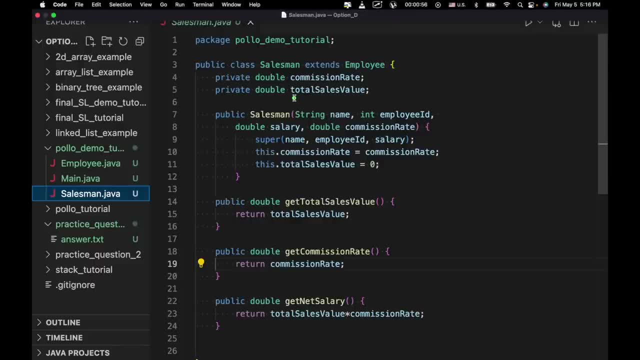 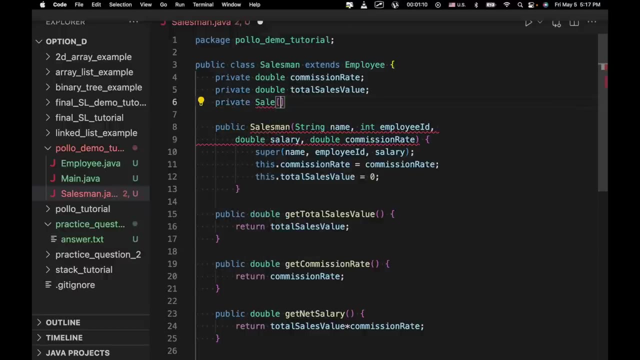 And by that we want to have a collection or an array of sales objects that are attached to this particular class. So what we're going to do first is we're going to create that, We're going to see what that looks like. So we're going to have private sale sales. 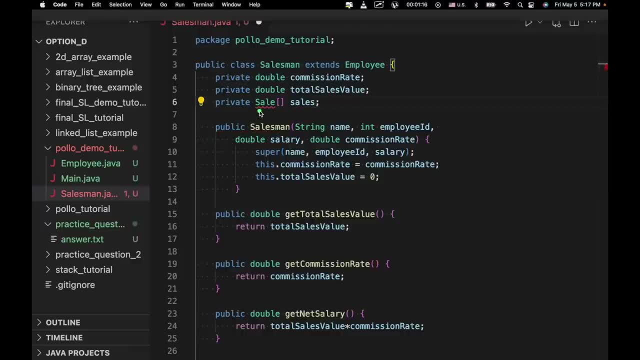 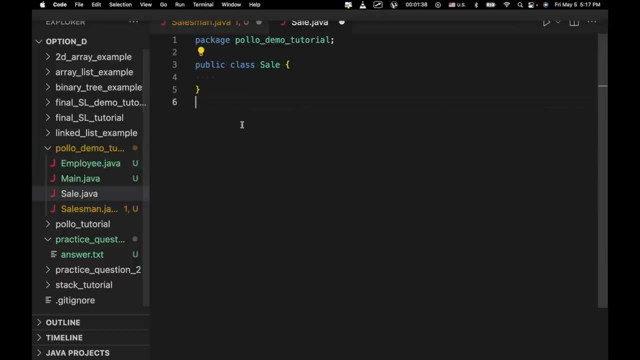 Okay, And we haven't created the sale object yet, So let's go ahead and do that New file, salejava. Okay, so now that we've got that right here, what we're going to do is we are going to give it some attributes. 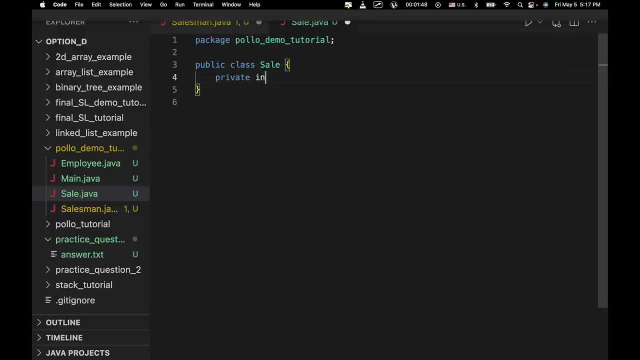 So, for example, we're going to have private int transaction ID, similar to our employee ID, just a way to kind of keep track of that sale in the system. We're going to have private double sale value. So how much was that sale for? 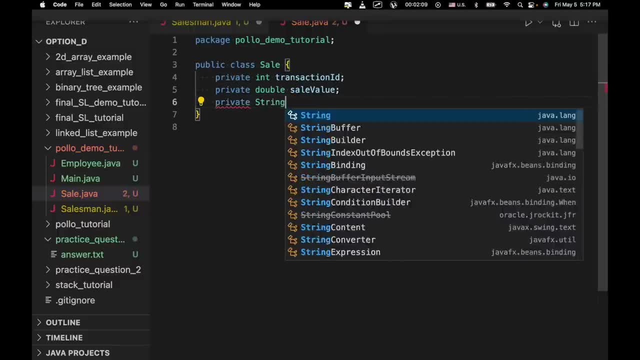 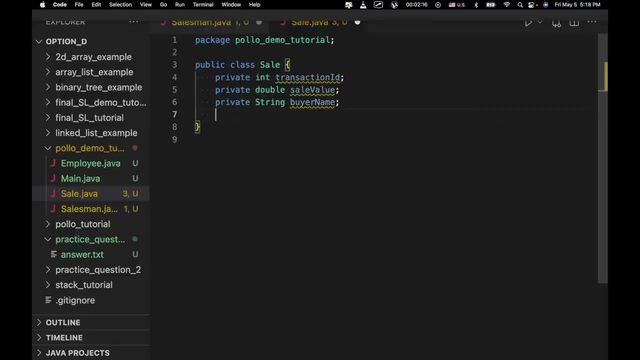 We're going to have private string buyer name. So who bought that? Probably not the best thing to keep track of, but whatever. So we're going to have a pretty typical constructor. We're going to say int transaction ID, sale value and buyer name. 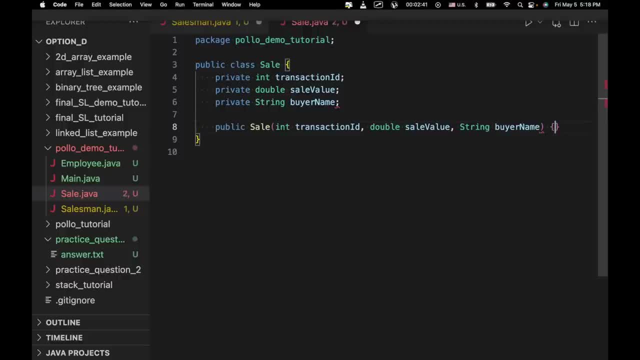 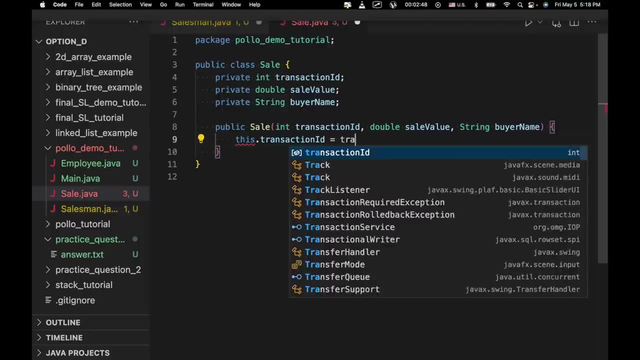 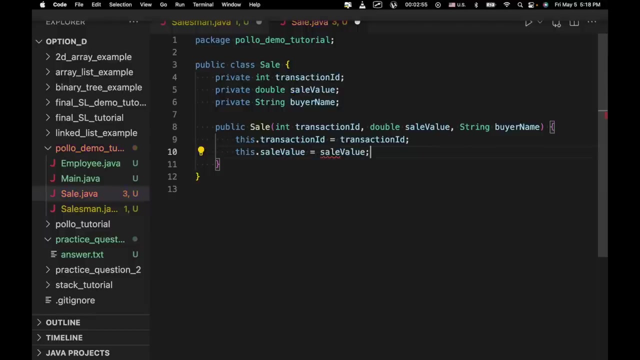 And that one should be a string. And then, in order to make sure that we're setting our class attributes, we're going to use: this: equals the transaction ID that's been entered as a parameter. Okay, cool, That's our constructor. And then we're just going to have some typical mutators and accessors. 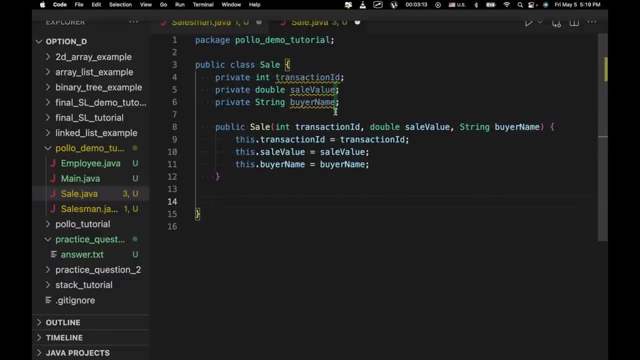 Although I don't think I really want to change any of these, I think that once we create a sale, once we instantiate with this information, that's all we're really going to do with it. If we want to edit the sale, we're just going to have to create a new one. 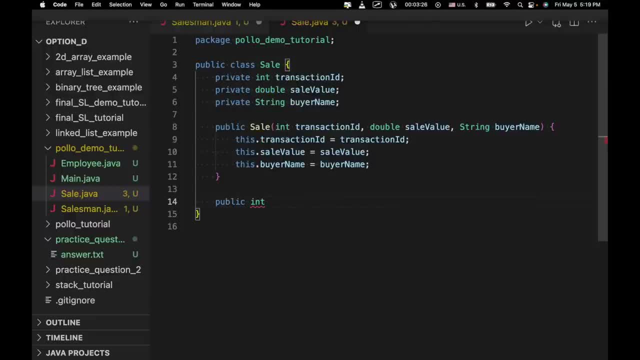 So in that light, I'm just going to say: public int- get transaction ID: It's going to return this dot transaction ID. Public int- get sale value: It's going to return This dot sale value And, Oh sorry, That's going to be a double, I think. 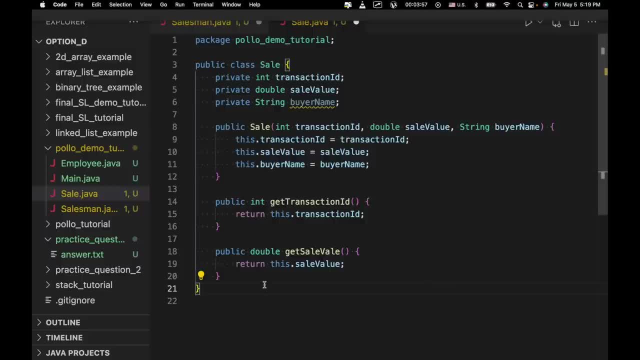 All right, Double return type And then we're going to have public string return buyer name. Now, generally, particularly when you have scenarios on the IB exam, you will have both mutators and accessors, So both gets and sets. But for this one, 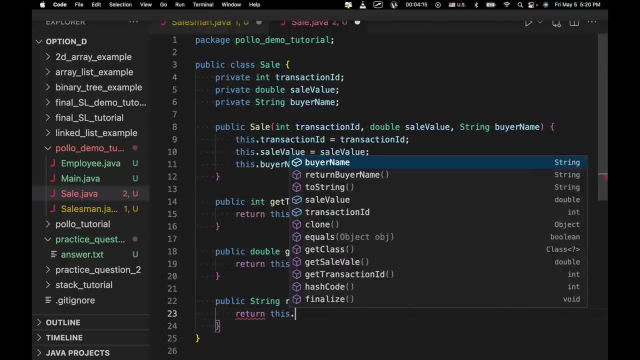 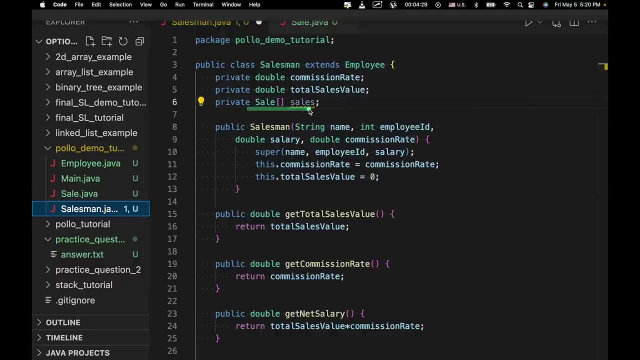 we're just going to- We don't really need to do that- This dot buyer name: Cool, Okay. So we've created a sale class, Okay, And in our salesman object, our salesman class, we're going to have an array of sales objects. 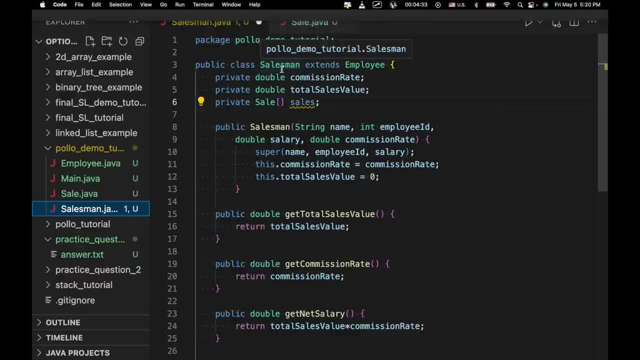 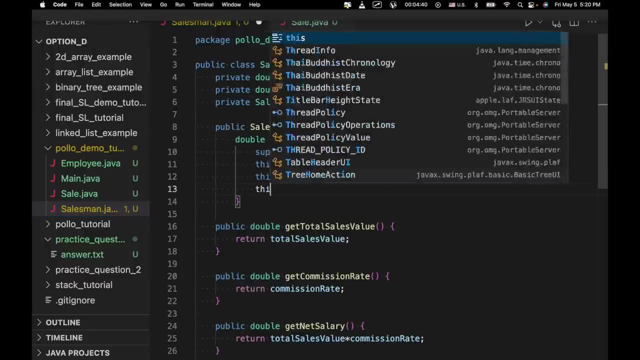 attached to the salesman class. Now there are a few things that we need to do to modify our class to deal with these sales. The first thing we want to do is we want to initialize it. So we want to say this: dot sales equals new sale 10,. 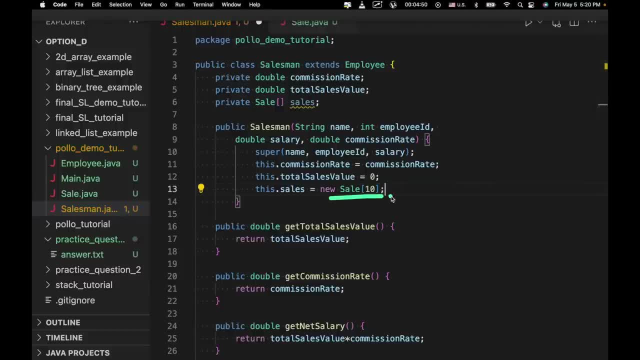 which is basically creating an empty array with 10 spaces for sales objects. So basically, we're basically adding an array. So this already has a type of array of sales, but we're initializing it and we're making sure that it's equal to an empty array. 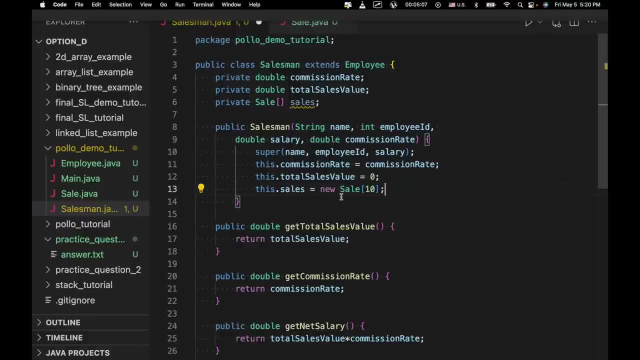 with 10 spaces that are reserved for sale objects. Now we could also put this right up here. It doesn't really matter whether it's a constructor or up here We could just say: sales equals new sale. We can do that for any of our attributes. 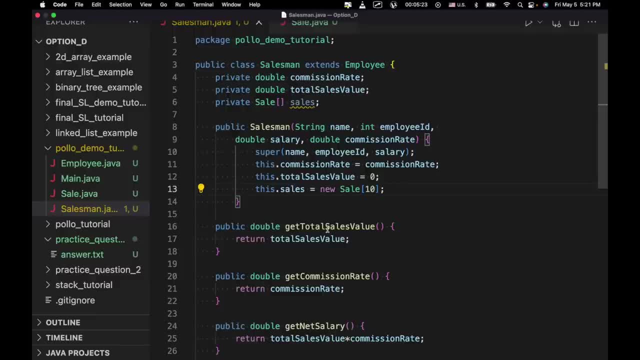 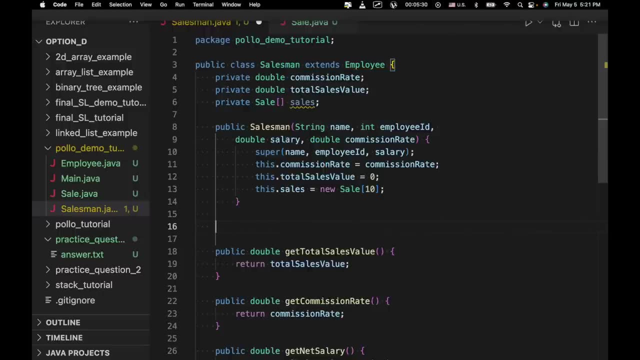 Now that we've done that, we also want a way to add sales. So we're going to create a function right here called public void, add sale, And we're going to have a sale object as a parameter. So we're going to have sale. 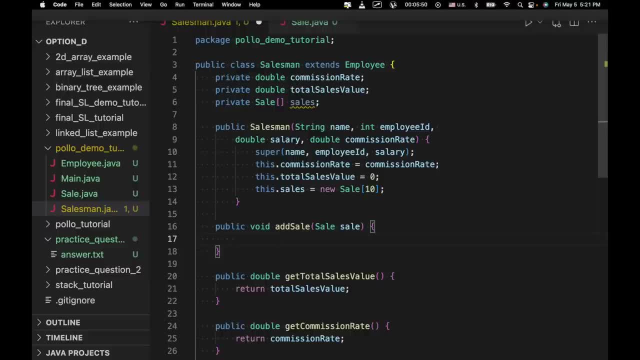 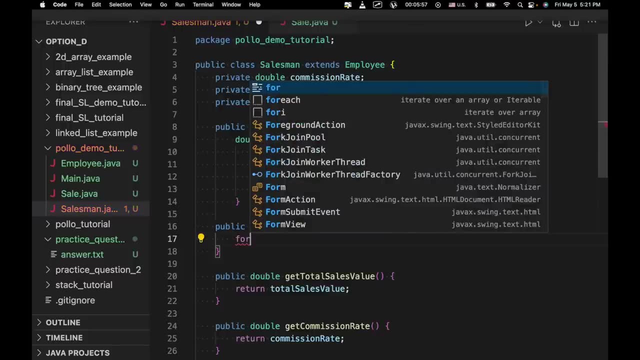 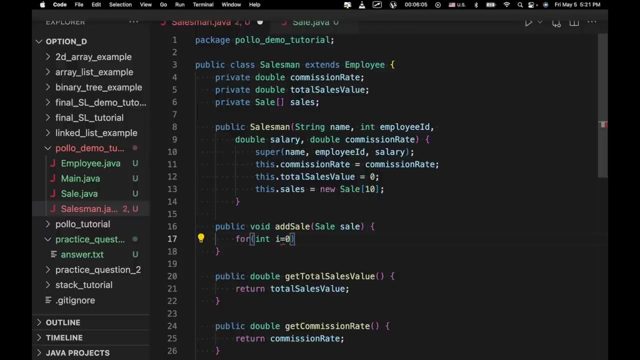 sale. And then what we're going to do is we're going to say we're basically going to find the first empty space in this particular array and then put our sale there. So we're going to iterate through it. We're going to say: for int i equals 0. 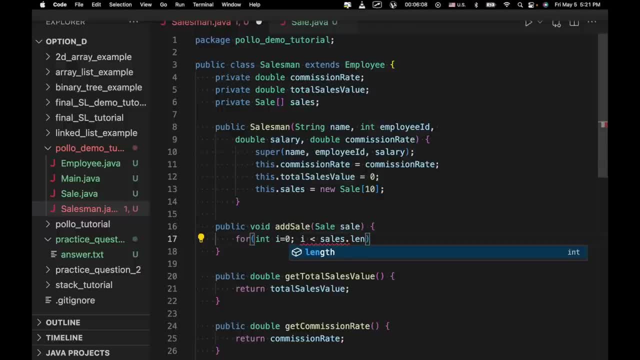 times i is less than sales dot length, and then i plus, plus, And then we're going to have: if sales i equals null, Then sales i equals sale. So we're going to go through the array and if we have the first element that we find that is null. 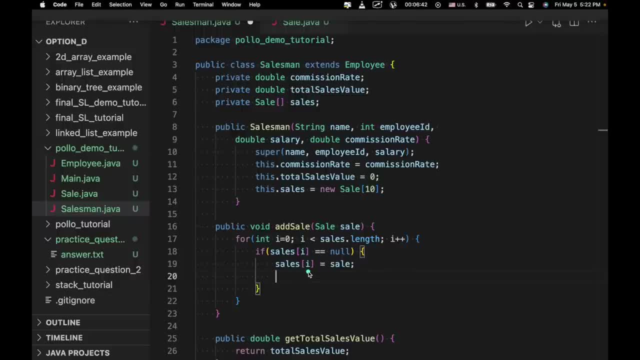 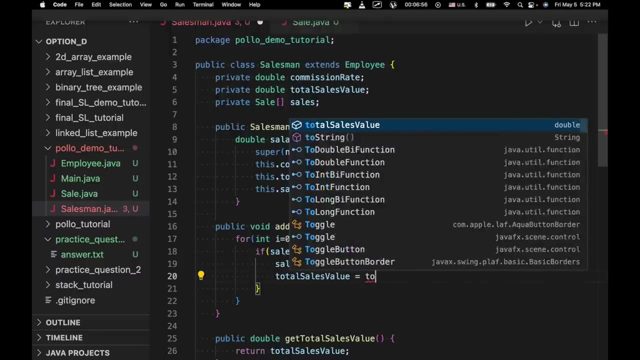 we're going to set our sale, We're going to put it in that particular element And then we're going to say total sales value equals or plus equals, Or it's going to be equal to the initial value of total sales or initial total sales value. 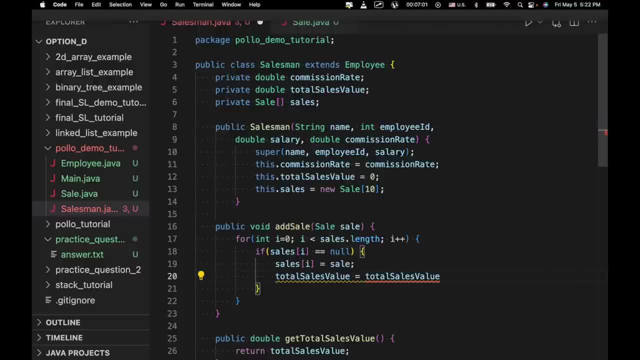 Or actually we can say total sales value plus sale dot get sale value And then we can just break. You don't need to go through the array any longer. That's how we're going to add a sale And we can also do something like public. 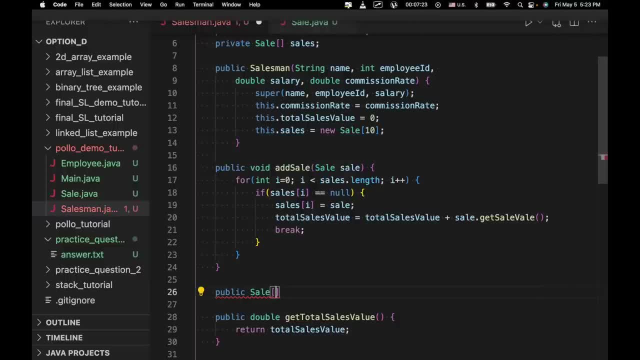 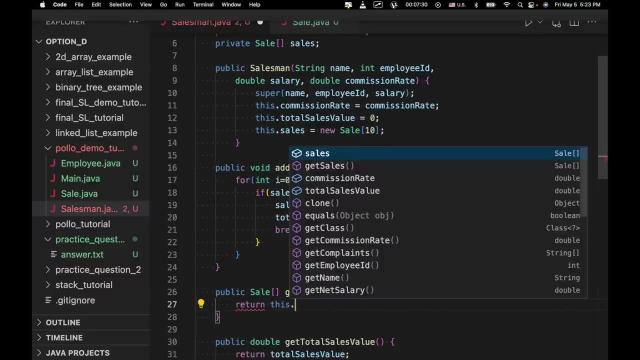 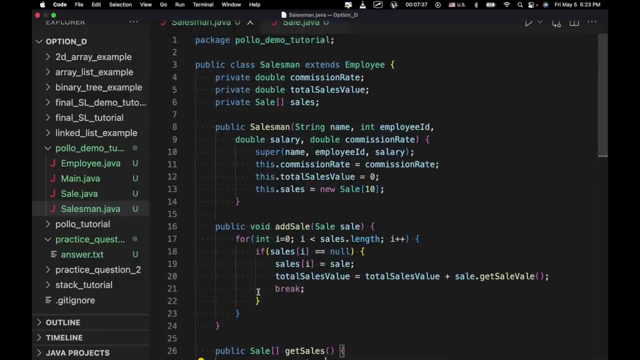 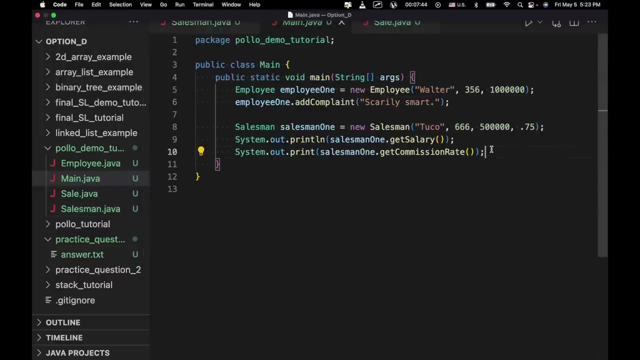 well, it's public sale, get sales, And then we can just return this dot sales. So this can be our accessor, our mutator and our accessor for that particular array. And now let's go to our main class And let's see how we can work with that. 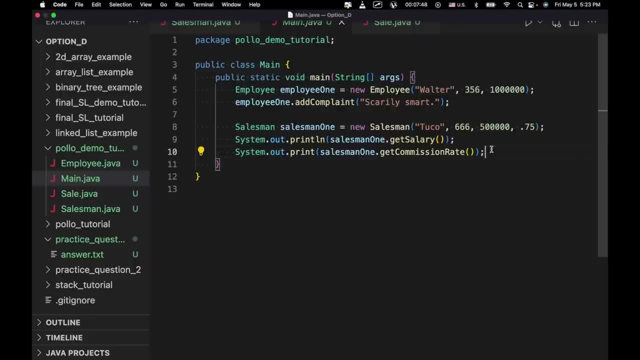 and how that looks like in practice. So basically, what we can do is we have this right here. We can say: we'll create a new sale. We'll say: sale equals our- remember our transaction ID. we'll just say 988790.. 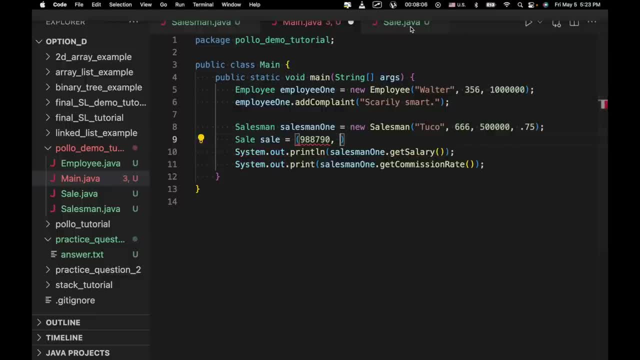 Our- I think it was actually sale, yeah, sale value. So we'll say that was a- I don't know if that was a big one or a small one, I guess a big one $1,000.. And the buyer's name was Emilio. 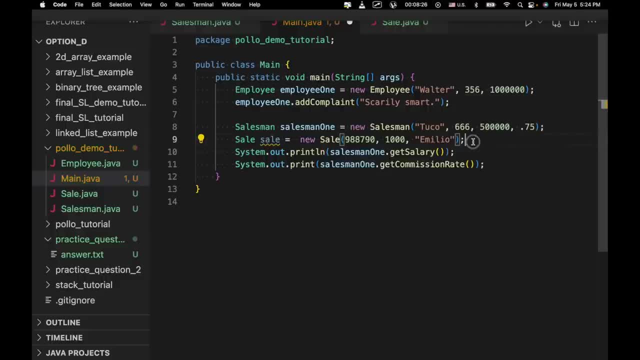 Oh, and we got to do new sale. my bad, Okay, cool. So now that we've done that, we want to go ahead and add this sale to our particular salesman object. So we're going to say salesman1.addSale and put that in there. 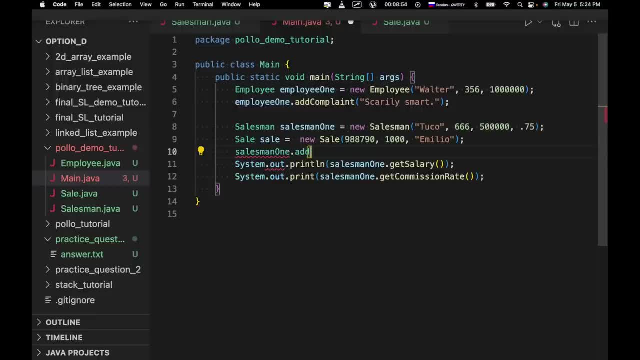 Oh, my bad. Okay, so we've add sale and then sale, And that pretty much does what we want it to do. We'll just run this to make sure that everything works, But what that would have done is that would have added a sale. 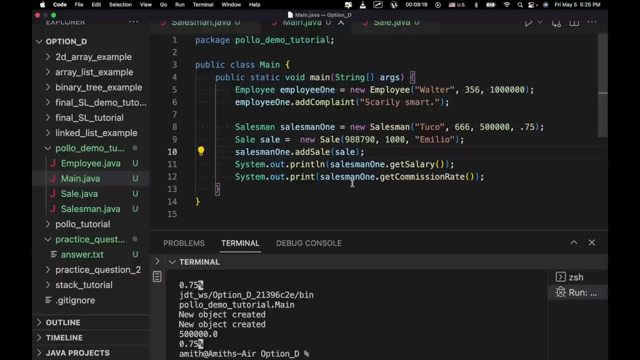 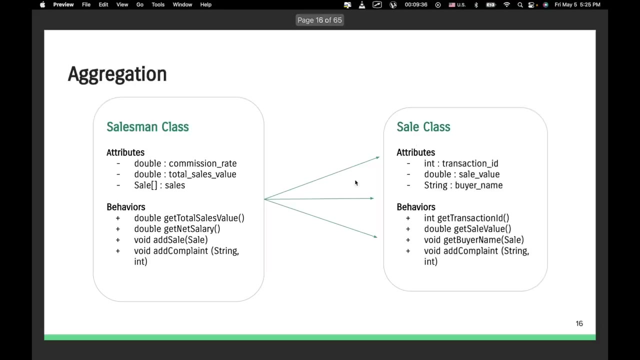 to the salesman1 object, And that's pretty much it. If we got the array and we went to the first element, we would be able to see the details of this particular sale, And that's an example of how aggregation works. Now, right here, 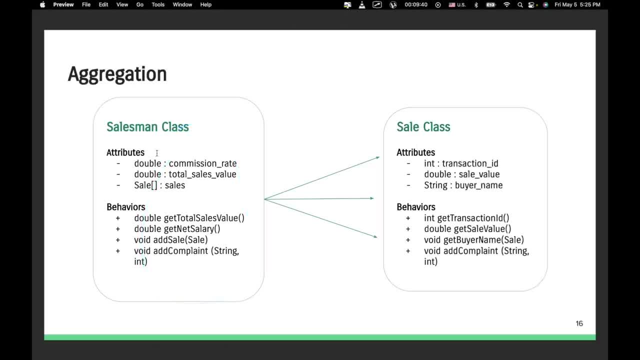 this is a chart that illustrates basically what we had done in our program. So right here we had a salesman class and we had our array sales and we had multiple sales objects, or we had the possibility of having multiple sales objects that are created from the sales class. 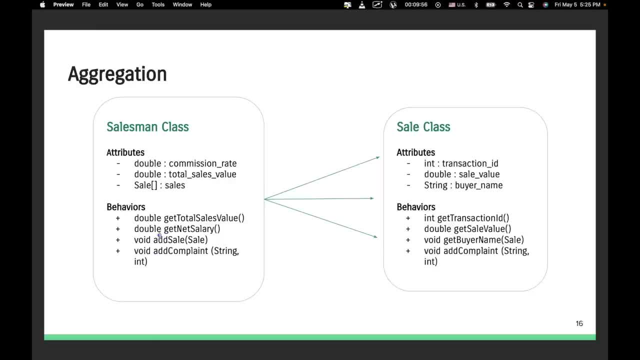 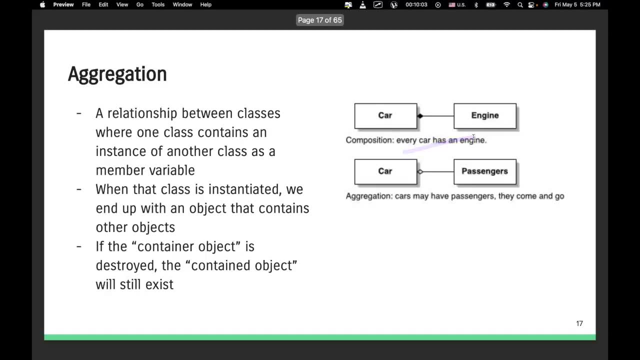 associated with our salesman class. We also had our addSale method and then we had the accompanying methods right here on our sale class. Now, an aggregation is a relationship between classes Where one class contains an instance or an object of another class as a member variable. 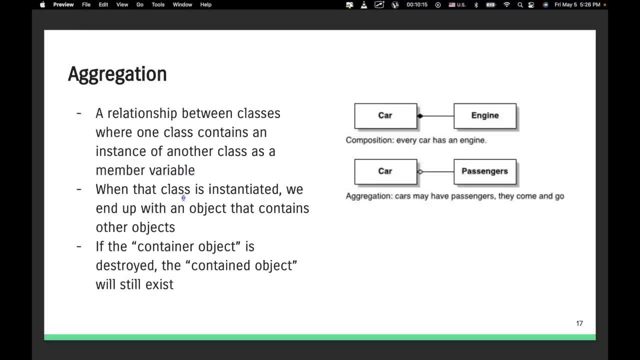 When that class is instantiated, we end up with an object that contains other objects. So aggregation means an object that contains other objects. If the container object is destroyed, which in this case would be the employee object or the salesman object, then the contained objects 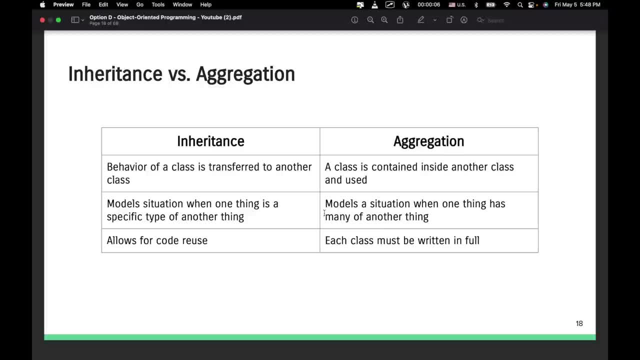 which are the sales objects, would still exist. Okay, so now that we talked about aggregation, let's compare it to inheritance. So with inheritance, the behavior of a class, meaning the attributes and methods, are transferred to another class. So, for example, from our salesman class, 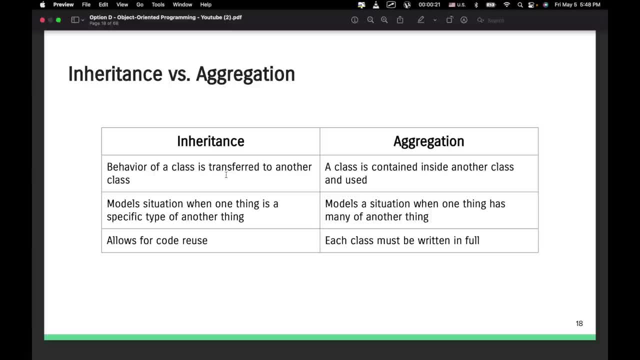 we can also use the methods and attributes in our employee class And with inheritance we're modeling a situation where one thing is a specific type of another thing. Again, the salesman is a specific type of employee And because the behavior of one class, 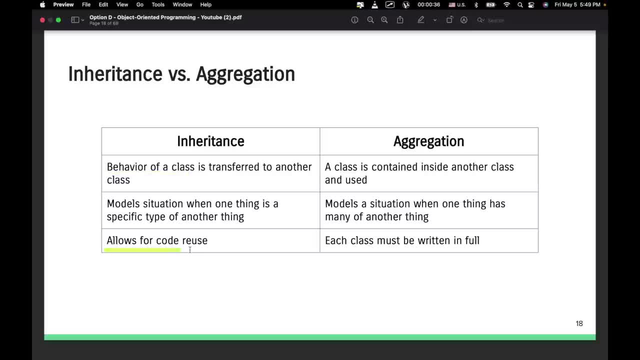 is usable from another subclass, we can actually reuse code, meaning we have to write less code. Now, with aggregation, a class or an instance class is contained inside another class. So in our salesman class we had instances of the sales of sales. 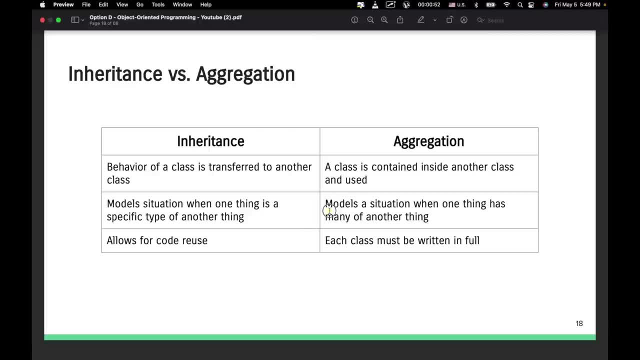 So basically it's sales objects And we're basically modeling a situation where one thing has many of another thing. So salesmen have many sales. Each class has to be written in full. Here we have more of a relationship, a one-to-many relationship. 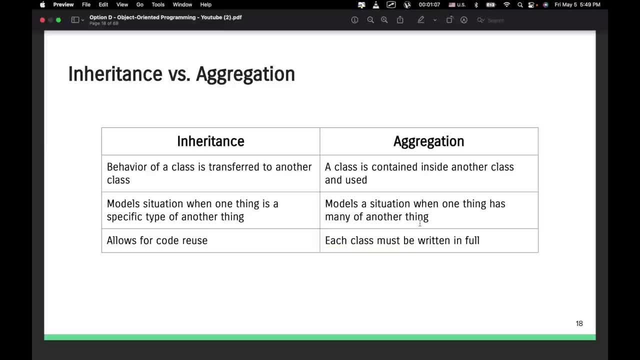 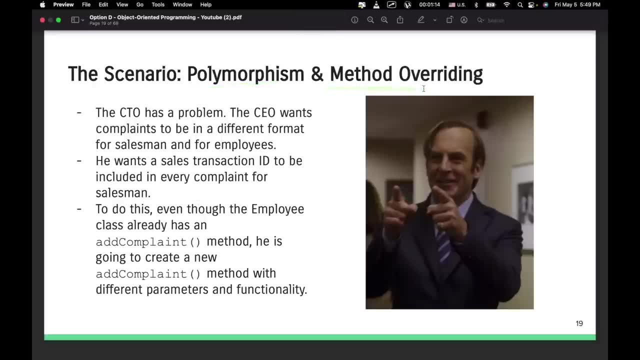 rather than actually sharing code, And the next concepts we're going to talk about are going to be polymorphism and method overriding. Now the CTO has a problem. The CEO wants complaints to be in a different format for salesmen and for employees. 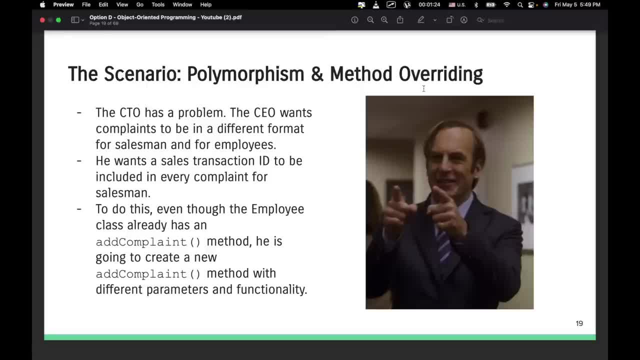 So, for example, that means that Tuco is going to have complaints in a different format than Walter is. He wants a sales transaction ID to be included in every complaint for every salesman. Now to do this, even though the employee class already has an add complaint method. 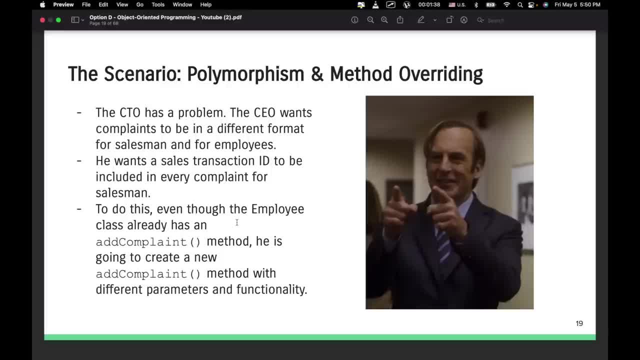 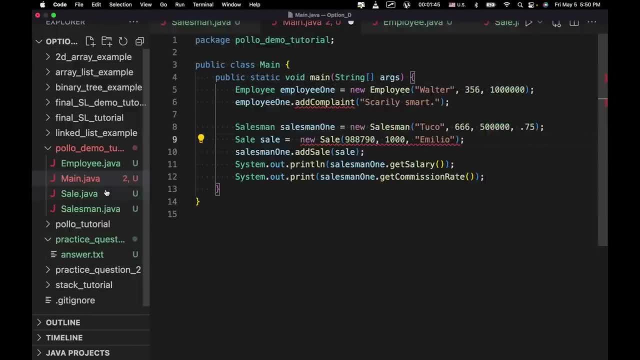 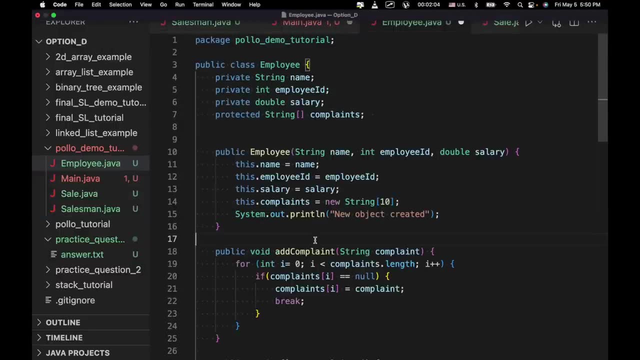 we're going to create a new add complaint method in our salesman class, different parameters and functionality. Now what I want to do is I want to go to sale right here, Or I want to go to employee rather. So I have our add complaint. 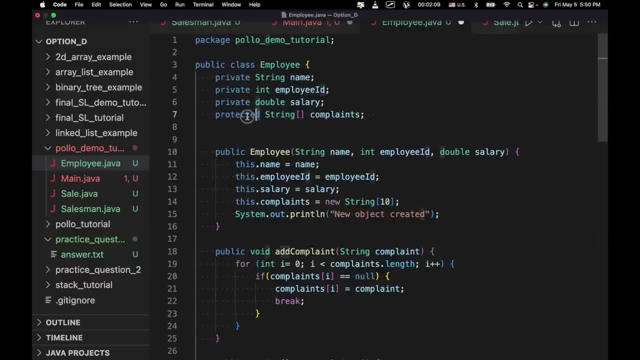 our add complaint class right here, And this is actually should be private for now, But I have our add complaint method right here And we're just going to go ahead and copy this And we're going to stick this in our salesman class right here. 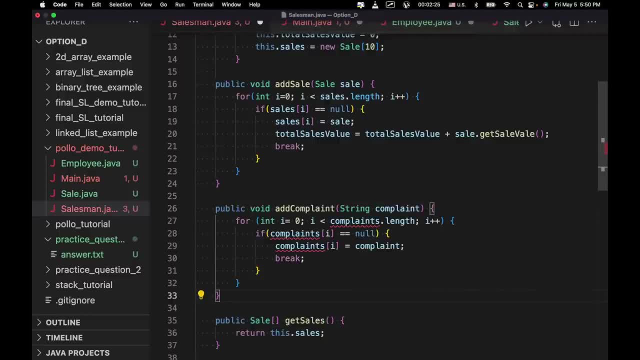 Now you might think there's a problem, given that both of them have the same parameters and same name. But what we're going to do is we're going to add a parameter, We're going to say string transaction ID. Now, just to avoid problems with casting. 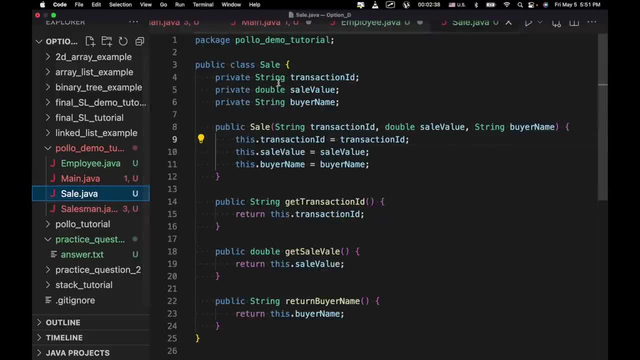 and using different data types. I actually want to go to sale and change the transaction ID to a string, which I've already done right here and right here, And I'm also returning a string. And if we go to mainjava right here, I'm going to input a string. 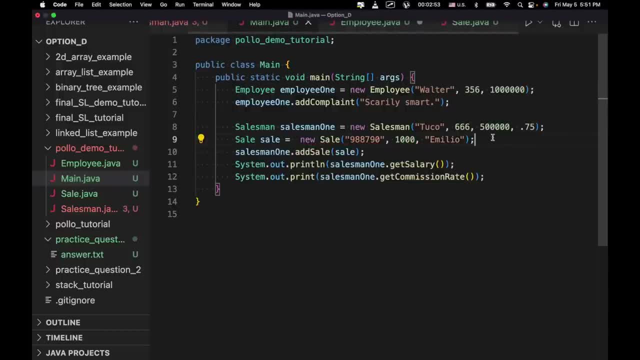 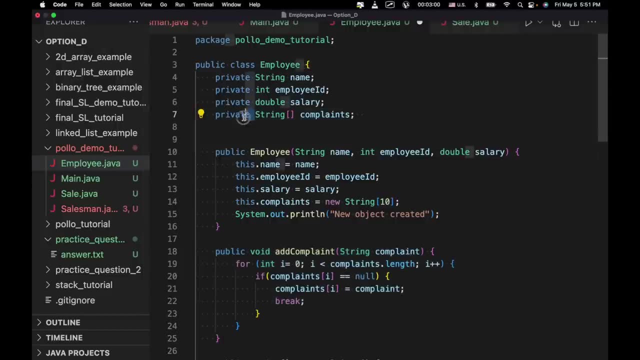 as the input for transaction ID. Now, one last thing I need to do. right here is right here. this private string complaints. It was previously protected. I'm going to change it back to protected, Because protected means that we can access this array both within this class. 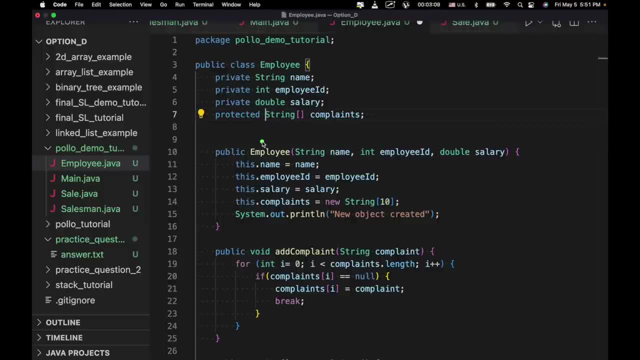 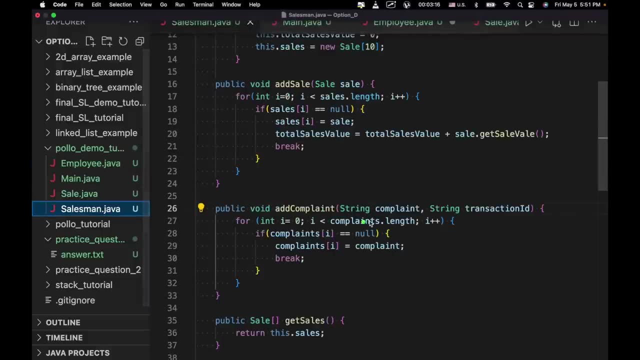 and within our salesman subclass. Otherwise, it could only be accessed in the current class, which is employee. So we're going to go to salesman right here And we're going to have the same method but with different parameters, which is the only way this works. 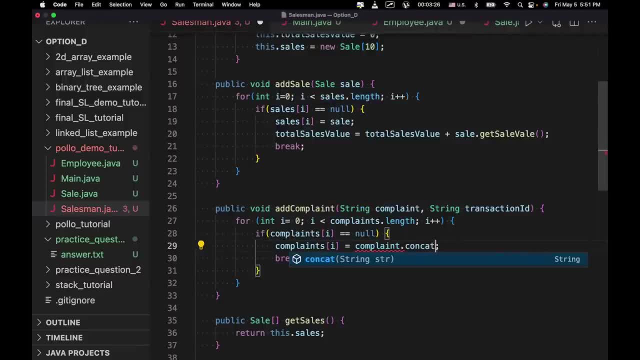 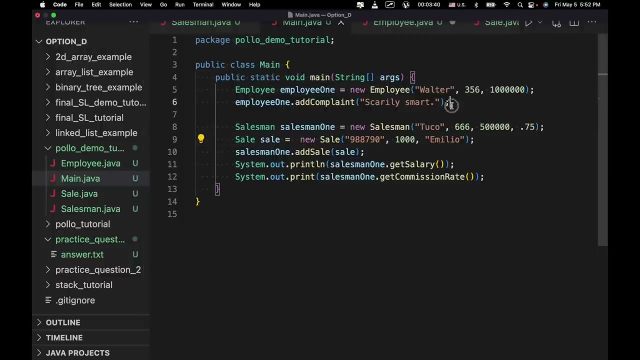 And we're going to do complaintconcat and we're going to have transaction ID. So how this is going to look in practice is we're going to go back to mainjava And so right here we had add complaint where we had one parameter. 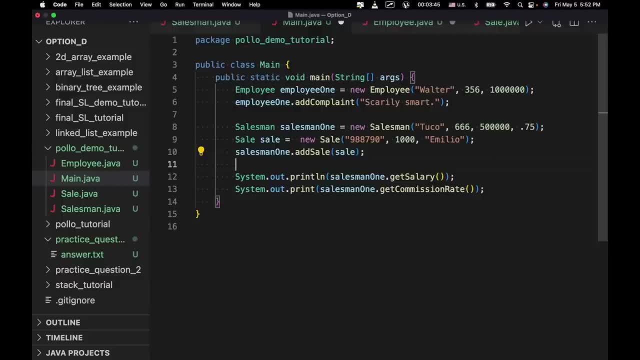 Now what we can do with our salesman is we can say salesman1.add complaint and we have two options, So we can actually do the one we previously had. So we can do add complaint and we can say: insane, I mean, we're describing Tuco. 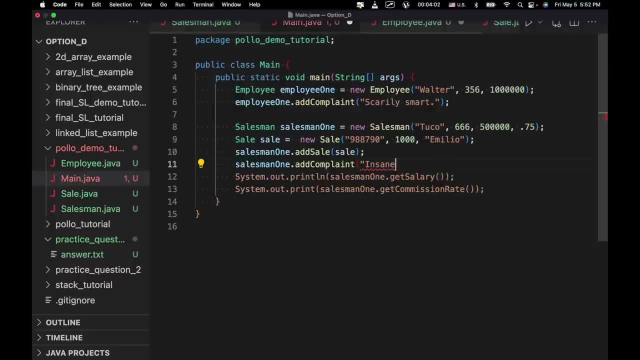 Or we can use the other option, which is to do salesman1.add complaint and we'll have insane but with the transaction ID, Because this may be the transaction ID of the complaint. I don't know, It probably is. We're just going to get rid of this one. 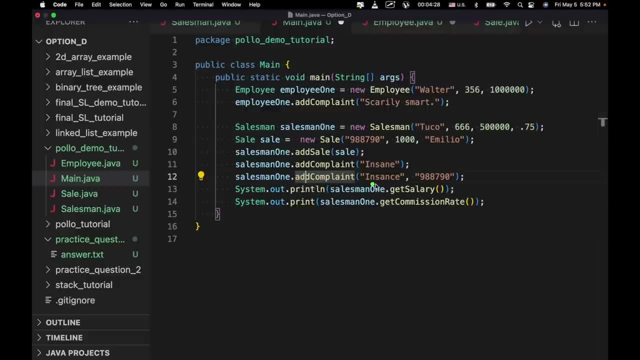 But either of these are possible, And the main differentiator here is the fact that this has different parameters. So which of these functions- whether we use the one on the employee class or on the salesman class- is dictated by what the parameters are. 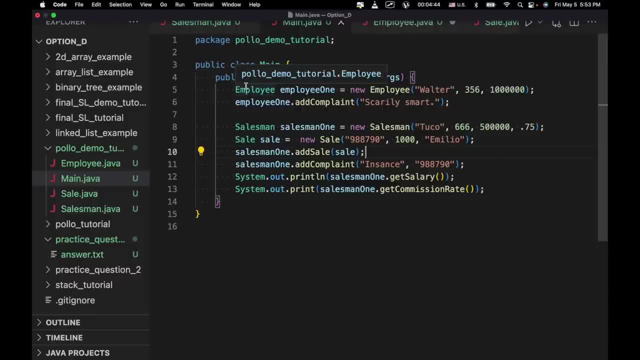 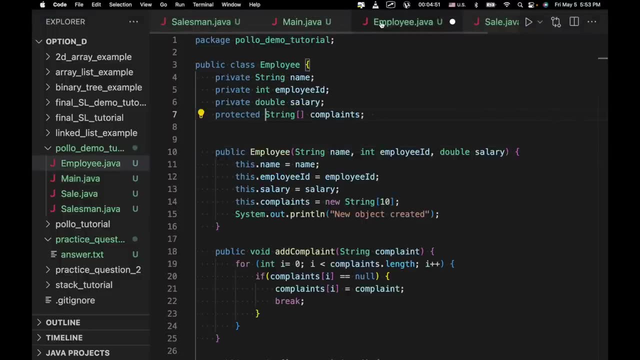 And that's basically how method overriding works. Now, another concept I want to talk about is method overloading. So, right here, let's go back to our employee class, right here, which we just saved, And let's say that, rather than having this be an option, 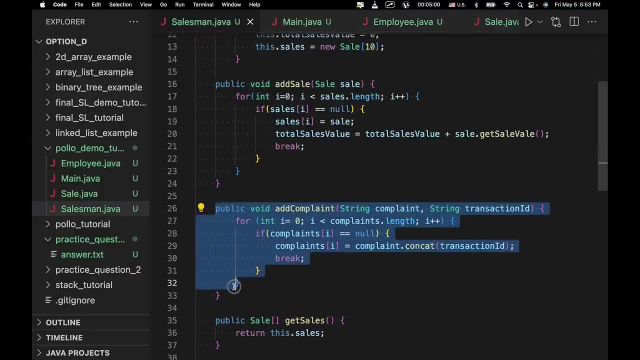 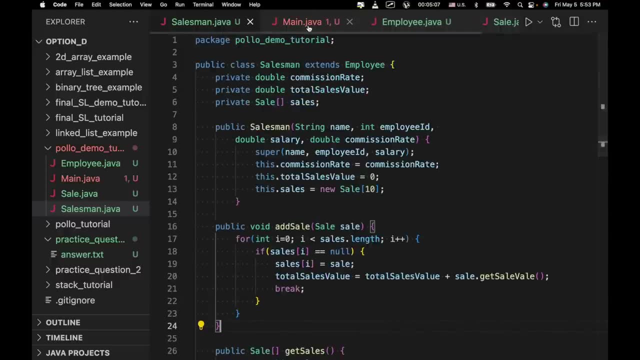 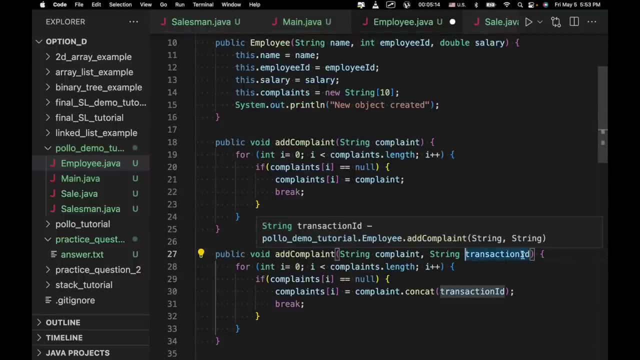 just for salesman. we want it to be an option for everyone to use that transaction ID. So, instead of having this in salesmanjava, what we're going to do right here is we're going to put it in our employee class And, instead of having a transaction ID, 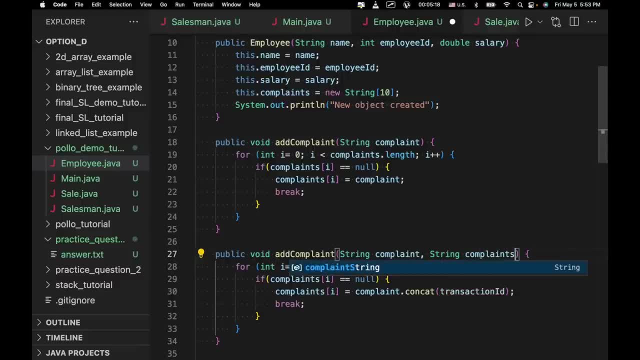 let's say we'll have a complaint ID of some sort. I don't really know why, but we're going to do that, So this also works. So we have two methods with the same name in the same class, which is employee, but they have different parameters. 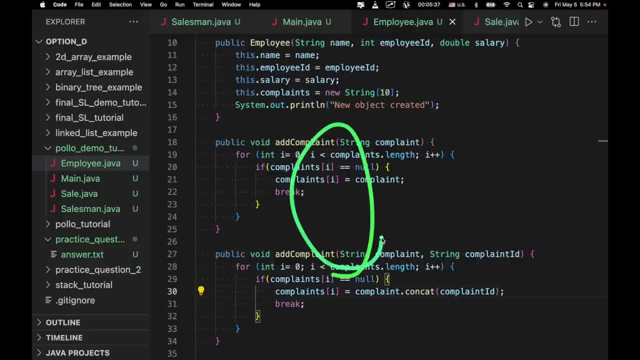 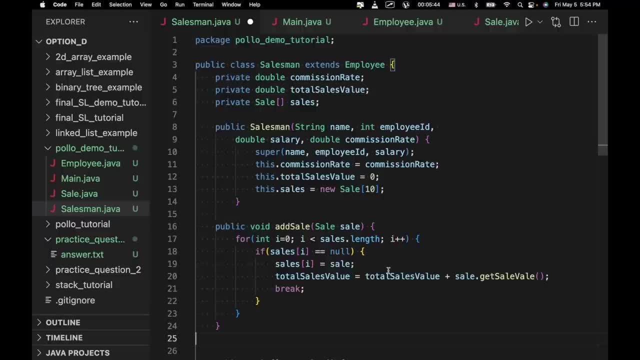 So we can use either one of these. Now. this is called method overloading, When we had a method with the same name in our salesman class. I guess I might as well just put that back here. This is an example of method overriding. 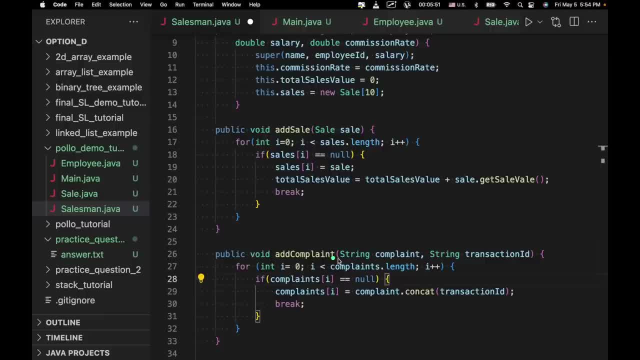 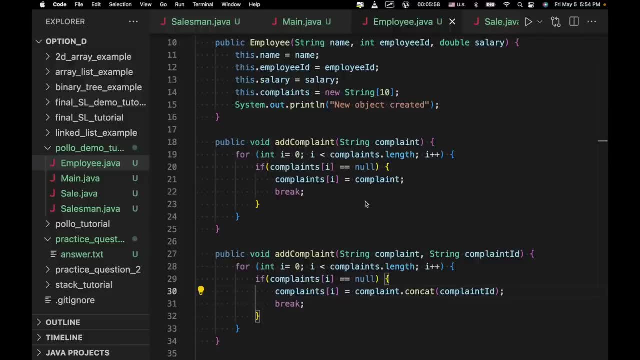 We have a method with the same name in a subclass and in a superclass and they have different parameters. That's method. overriding This right here, where they're in the same class but have different parameters, would be method overloading, And both of these are an example. 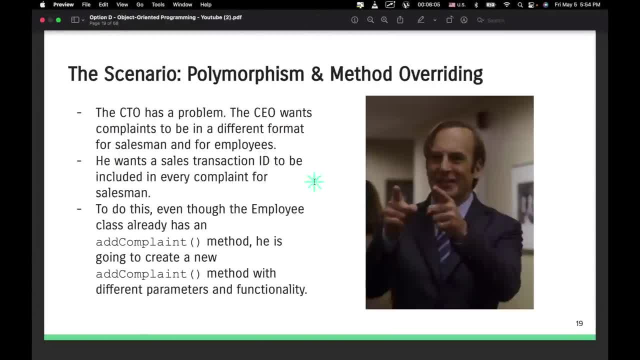 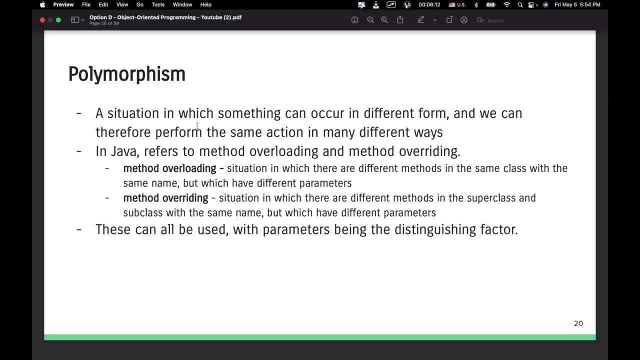 of what is called polymorphism in Java. Now, polymorphism just in nature, just in generally, is a situation in which something can occur in different forms and we can therefore perform the same action in many different ways. So thinking about a donkey kicking and a human kicking. 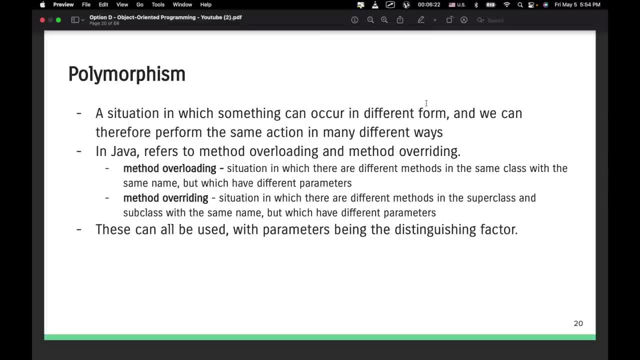 It's a weird example, but anyways, And in Java, this is really referring to method overloading and method overriding, which we just went over, Method overloading again being a situation in which there are different methods in the same class with the same name. 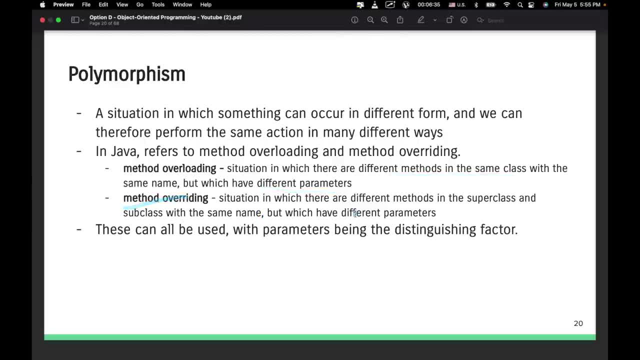 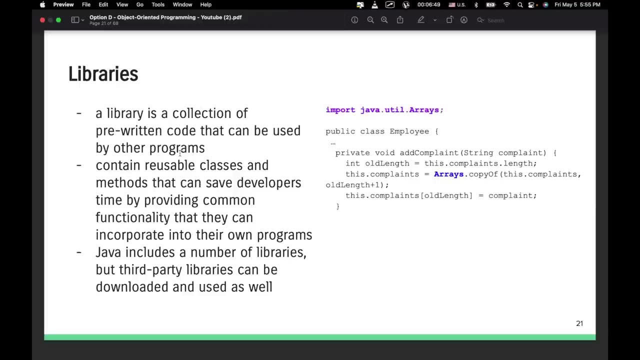 different parameters, Method overriding being a situation in which there are different methods in the superclass and subclass with the same name but with different parameters. In all these cases, the number of parameters is a distinguishing factor, as we saw before. The next we're going to talk about libraries. 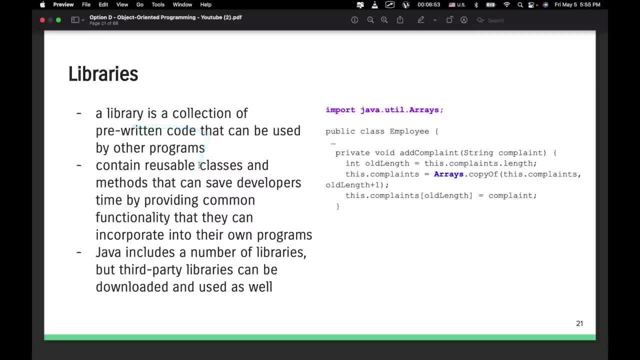 So a library is a collection of pre-written code. It's kind of like an addition or an expansion pack. It contains reusable classes and methods that can save developers time by providing common functionality they can incorporate into their own programs. Java includes a number of libraries. 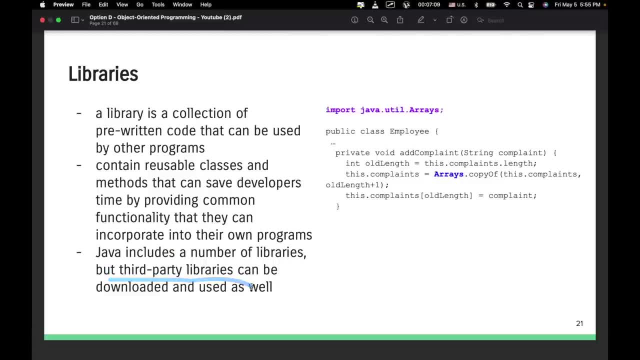 but third-party libraries can be downloaded and used as well. So here's an example of how we would use a library. Now, if you wanted to manipulate arrays in a certain way- that's not part of the standard Java- you could go to employee right here. 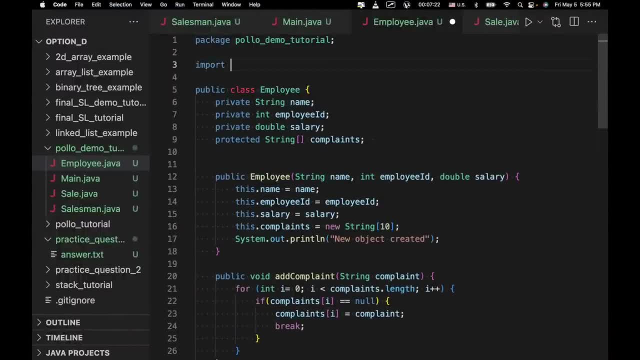 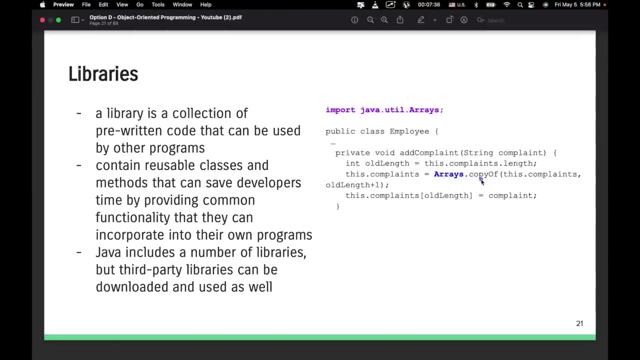 and we could do import javautilarrays. Then we'd have access to some additional functionality which, in this case, allows us to make copies of arrays. I'm not going to do that right here, but this is some additional functionality we didn't have before. 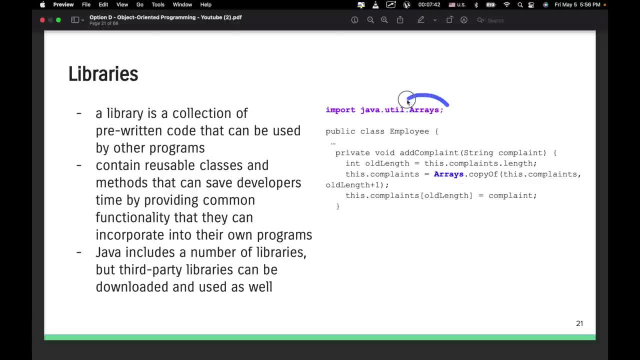 that came from this library. And we know it did, because here the last string is called arrays. So we're using this down here to access the functionality on that library. Now, mainly in the SL exam, you're not really going to use libraries. 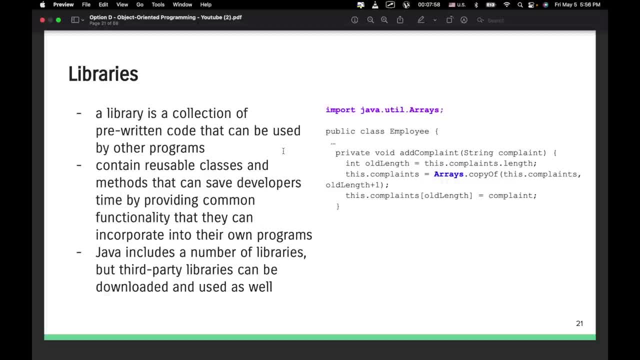 You will extensively on the HL exam, but on the SL exam, you just need to know that these exist and the fact that they contain reusable classes and methods. Now, later on, we will look at an example involving the use of libraries. that should help you. 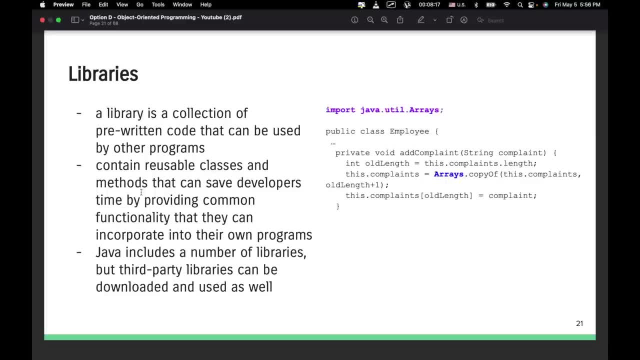 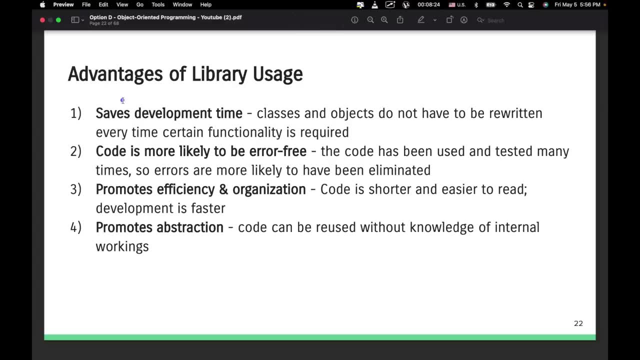 regardless, get a better understanding of how object-oriented programming works and give you a little bit of a bridge into the HL content. Now, some of the advantages of library use are that they save development time because actually you can download libraries off the internet. 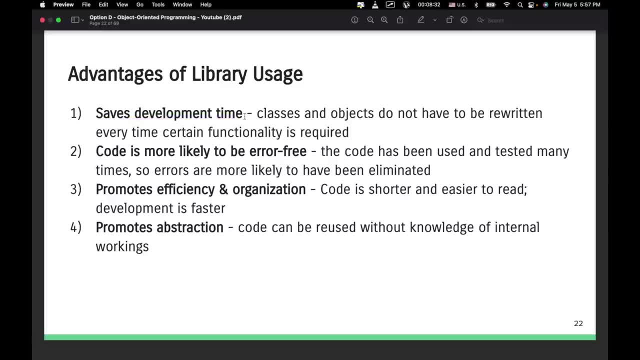 that take care of certain functionality so that you don't have to rewrite it. So classes and objects don't have to be rewritten every time certain functionality is required. A lot of times these libraries are shared and used by multiple programmers, so they're more likely. 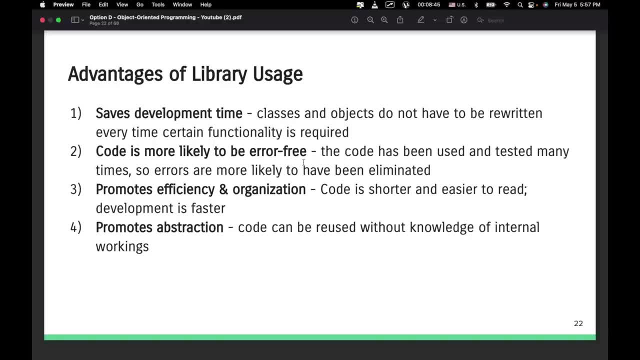 to be error-free, because if there was an error, even how many programmers have used it, it's likely to have been found, And many times these are tested before they're used. Moreover, because you're not implementing the functionality in these libraries, 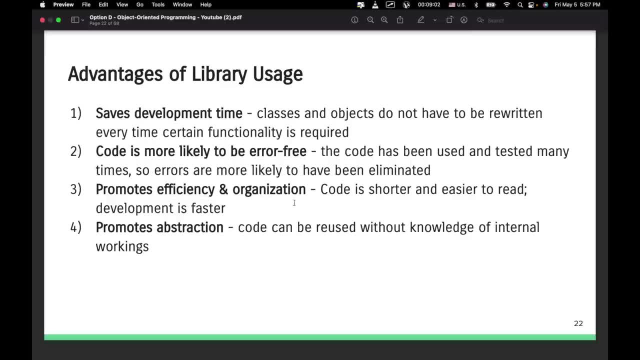 your code is going to be shorter and easier to use, making development faster. And finally, we can promote abstraction through library usage. Now, abstraction is basically hiding away the internal workings of a particular piece of code. Now, if you're using a library, 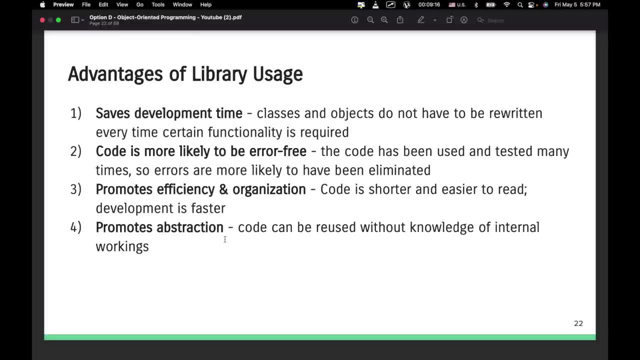 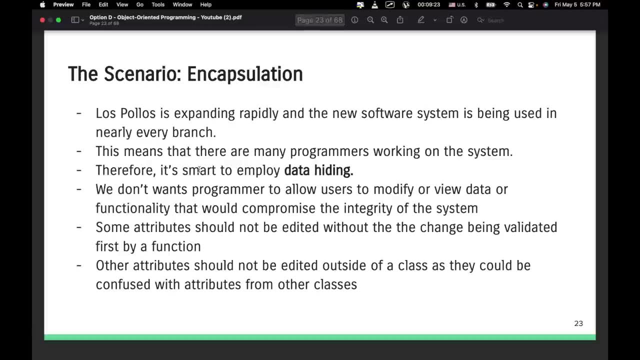 you don't have to understand how it works, You can just use it. And that's an example of abstraction which just makes coding a lot faster. It reduces development time. Now the next concept we're going to talk about is a big one. 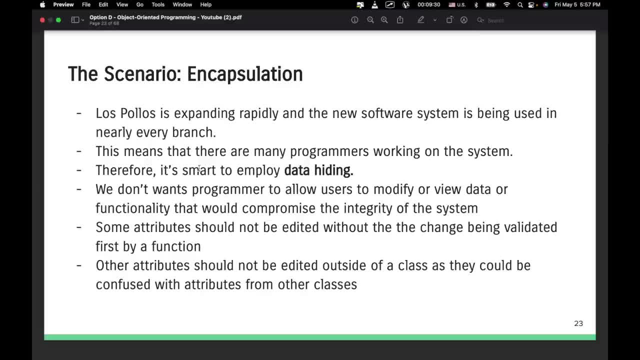 It's called encapsulation. Now, to go back to our scenario: Los Pollos is expanding rapidly and the new software system is being used in nearly every branch. This means that there are many programmers working on the system. Therefore, we want to do something. 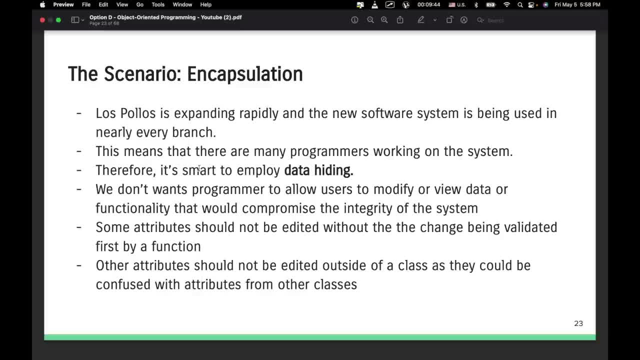 called data hiding. We don't want programmers to allow users, We just don't want programmers in general to be able to modify or view data in a way that would compromise the integrity of the system. So some attributes should be edited and some attributes. 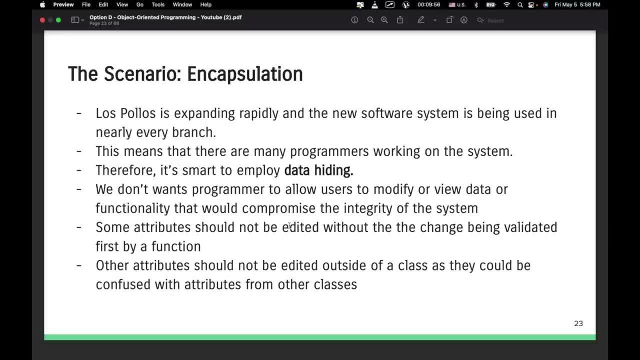 should not be editable. So we want some attributes that can be edited outside the class and some that can be edited only inside the class or in subclasses. Now, encapsulation refers to the practice of hiding the internal details of an object from the outside world. 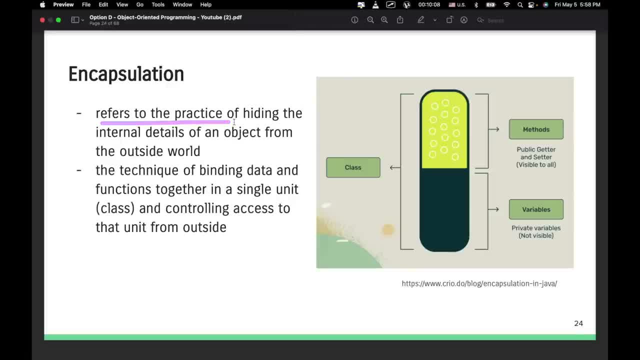 And really it's referring to the technique of binding data from the outside world. Now, encapsulation refers to the practice of hiding the internal details of an object from the outside world, And really it's referring to the technique of binding data and functions together. 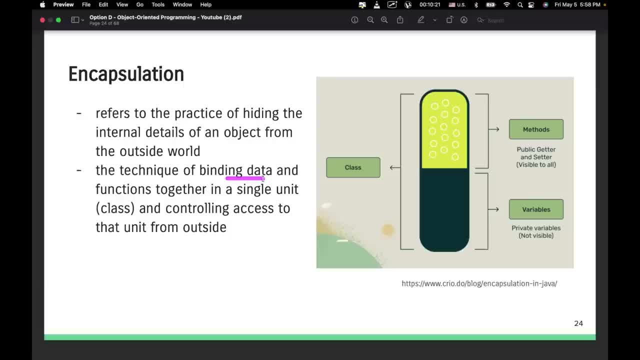 in a single unit and controlling access to the unit from the outside. So there are two components: just the fact that we have attributes and methods in the same class- an object- and then the ability to control access from the outside, But without further ado. 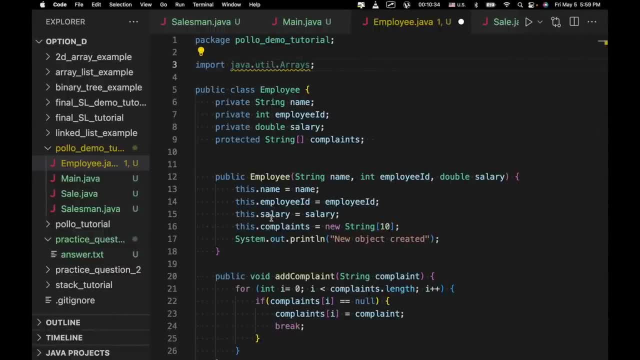 let's see what this means in practice using something called access modifiers. So if you look at our code right here, we basically have private, private, private and protected, And private means that these attributes are only accessible within the employee class. 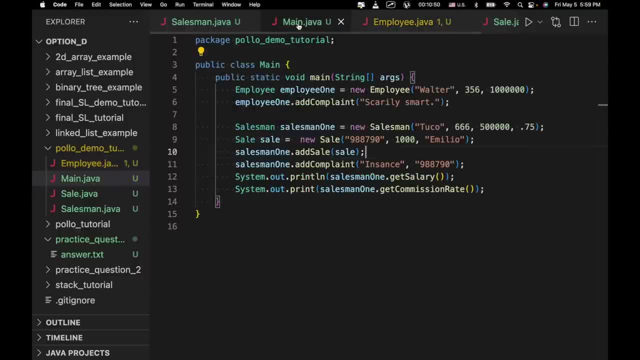 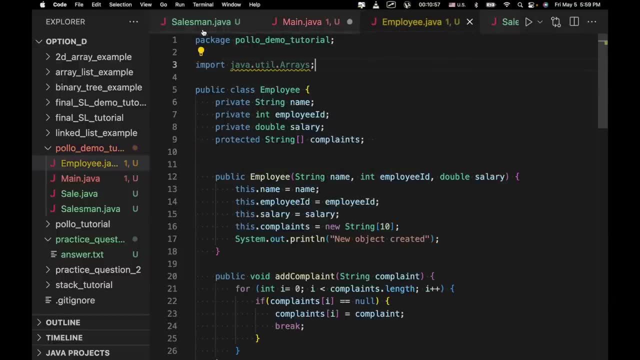 So, for example, if you go to mainjava, we want to just access employee1.one of these attributes, which is, let's say, name. That just doesn't work. Okay, Right here it says that it's not visible. 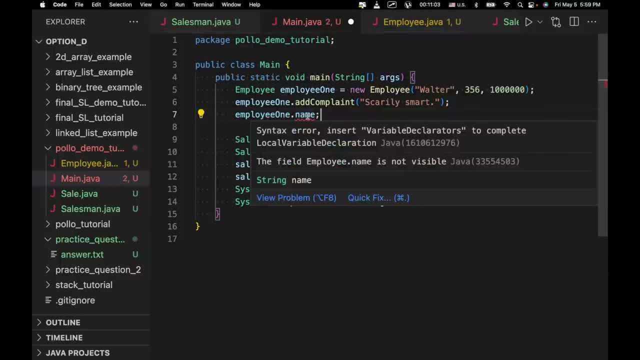 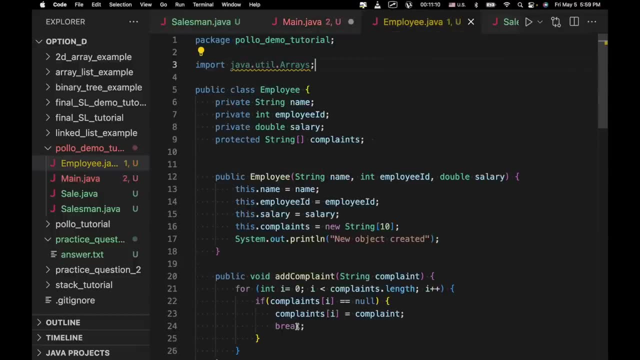 However, inside here, if you want to access name, we're free to access it using this or just in general. The same is true for this. So if you go to mainjava, the same is true for employee ID and salary. 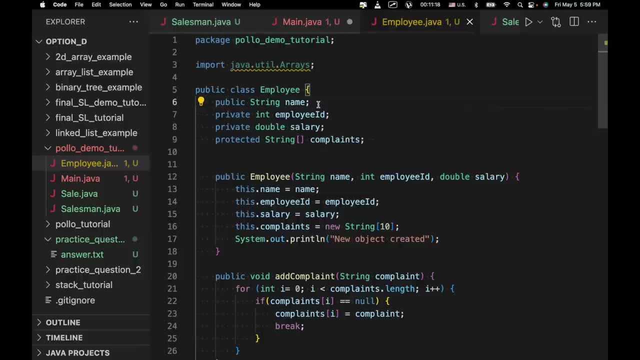 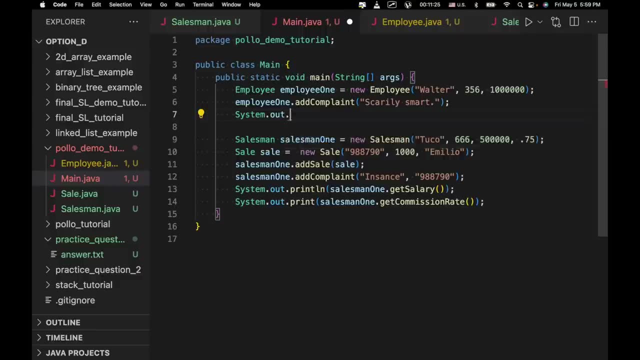 However, if we change this to public meaning, we can access it outside our immediate class or subclasses. all of a sudden there's no error right here And we could just go ahead and do systemout. Actually, well yeah, systemoutprintln. 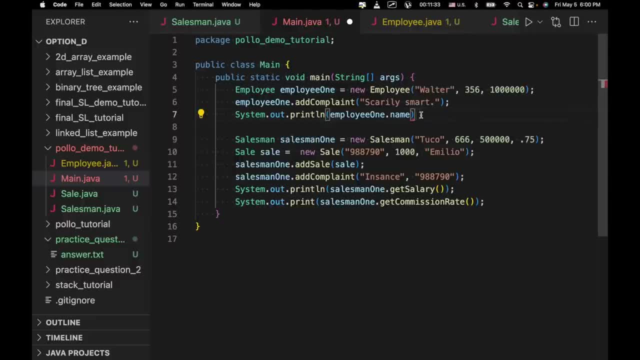 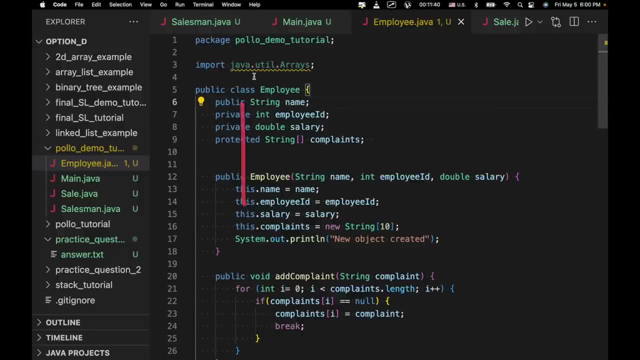 employee1.name, and that would work. So public allows us to access this attribute anywhere, and private means it can only be accessible within this class, And we're going to change it back to private because that's the way we want it. Now. private. 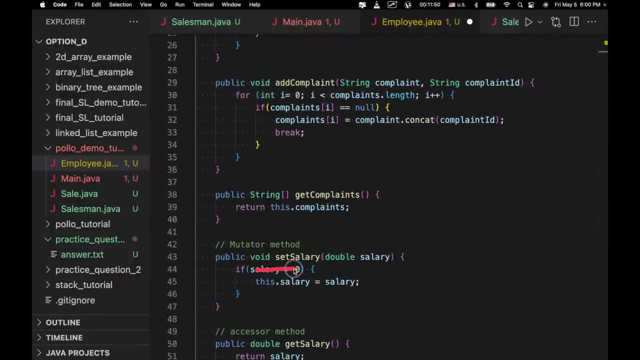 with private, we can. within the class, we can use mutators to change the value of the salary and accordingly we can control, like what the salary is. We can put some limitations and some validation on that. This means that through using accessor methods. 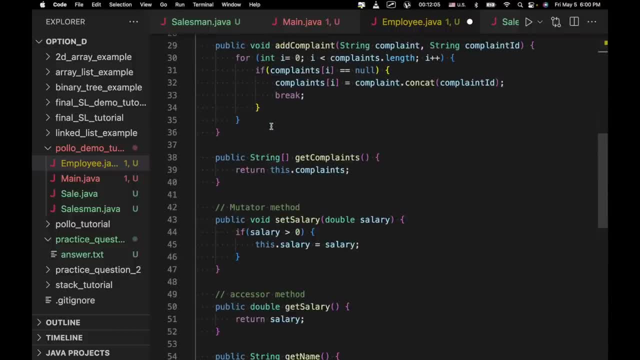 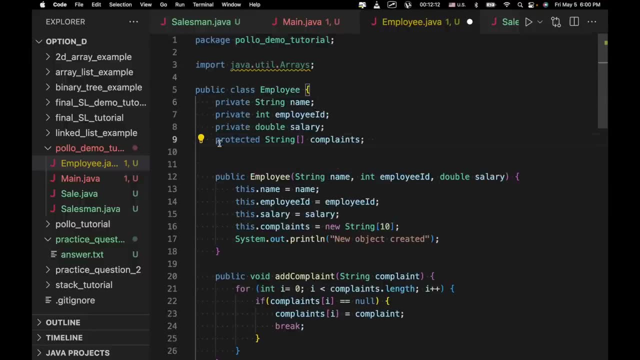 like private, we can control how those methods are modified. Hence the reason access modifier, or hence the reason it's called an access modifier. With protected, we can only access or we can only modify this complaints array in our in this class, in our main class. 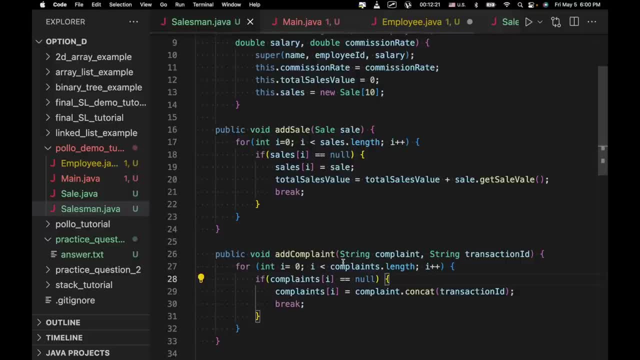 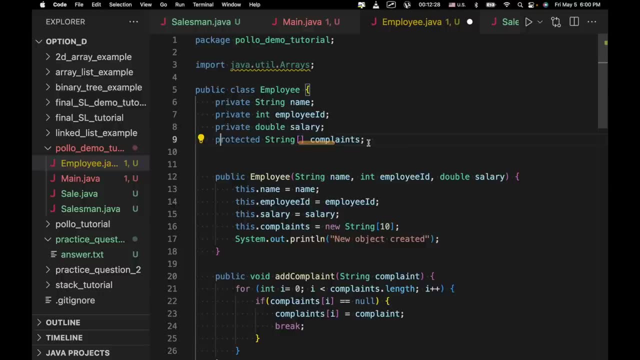 or in a subclass, So, for example, in salesman. right here we're modifying complaints and that's why we have to change this from private to protected. Protected only means that we can edit this within our class or subclass, or object or subobject. 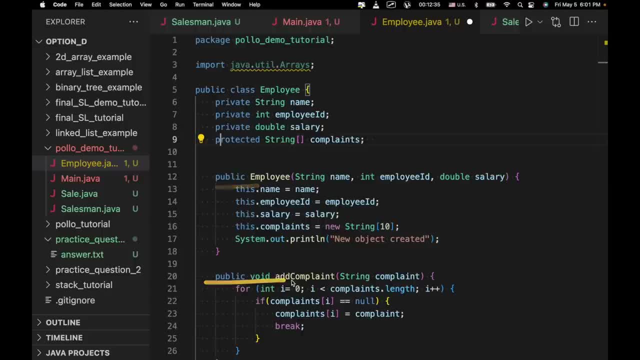 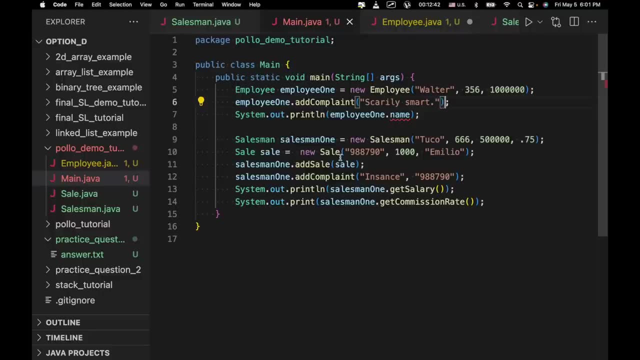 if you're thinking in those terms, If something is public, that means it can be accessed anywhere outside the object, anywhere outside the object. So anything that's public we can access outside of it. Hence, like these methods like add sale, 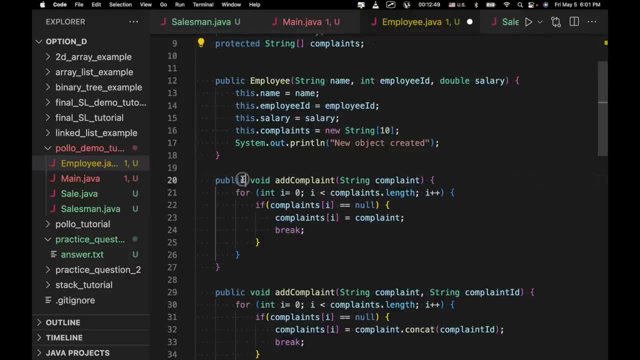 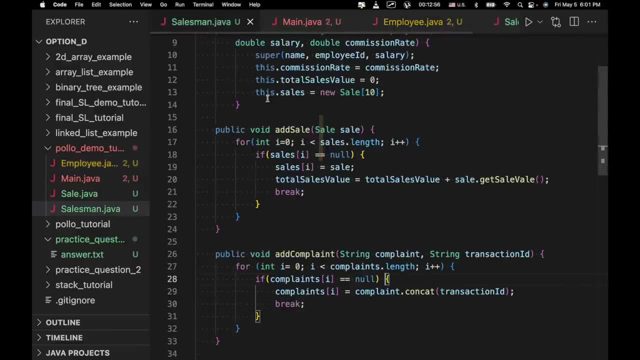 add complaint, add complaint, which are all public methods. If we change add complaint to private, it wouldn't really serve any purpose. but that just means that we can only really change it within this class, which just again makes no sense, and then this doesn't work. 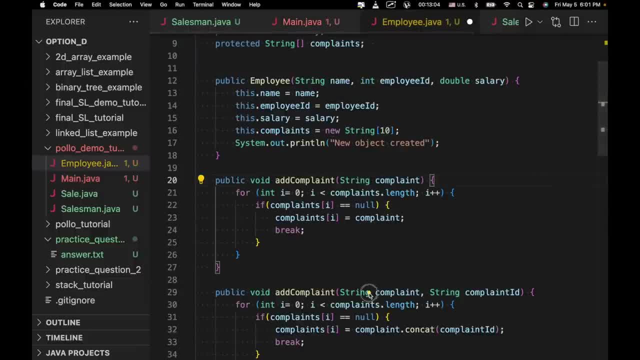 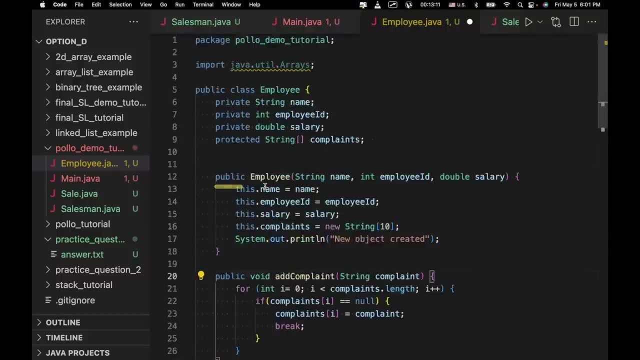 right here, Unless we're using it in another function inside inside of this class. there's not really any use in any reason to make this private. but any methods and attributes can be changed, can have their access modifier changed to either private. 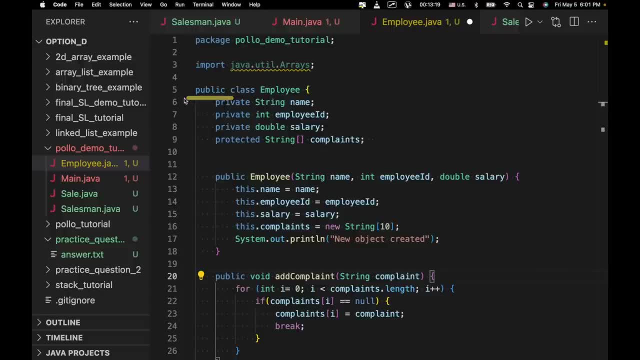 public or protected. Now we can also change the access to classes, but we're not going to get into that. You're never going to see that on the SL content and it's just. there's just no point covering it right now. 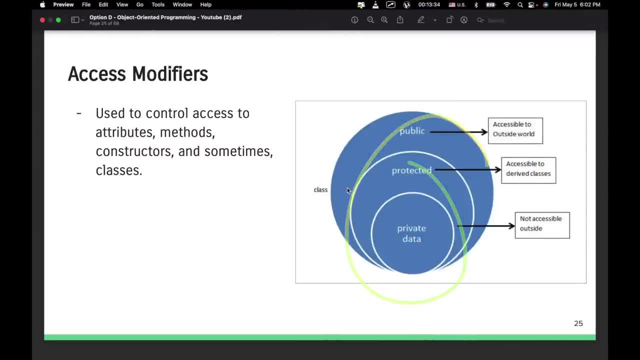 Now here's a little graphic. So private data is not accessible outside of a class. Protected is accessible to derived classes or subclasses. Public is accessible to the outside world. Actually, methods can be made private, public or protected as well. 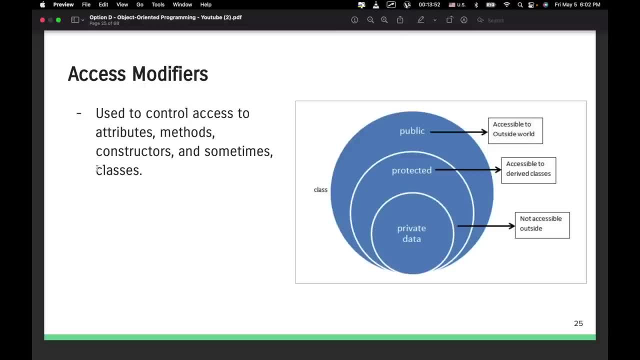 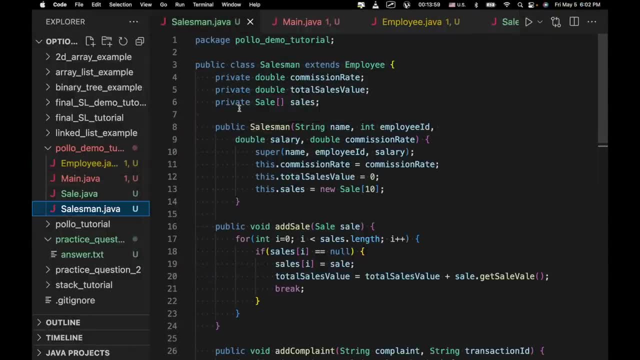 depending on how and where we want to be able to instantiate methods. So, for example, in our Salesman class right here. if we just only wanted to be able to create a sale, well, actually that's not a great example. 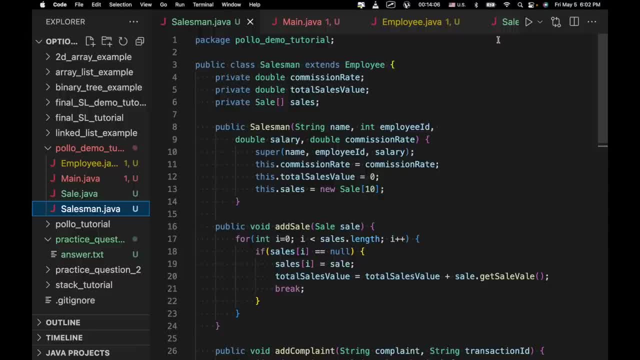 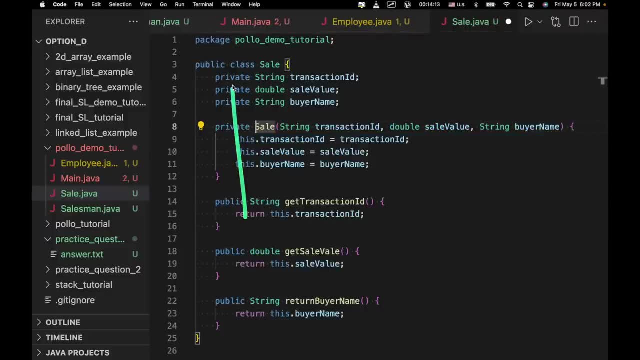 Never mind. Well, I would say well, I guess, if we made this private right here, that means that we'd only be able to create a sale inside this class, which doesn't make any sense. It's almost like a recursive situation. 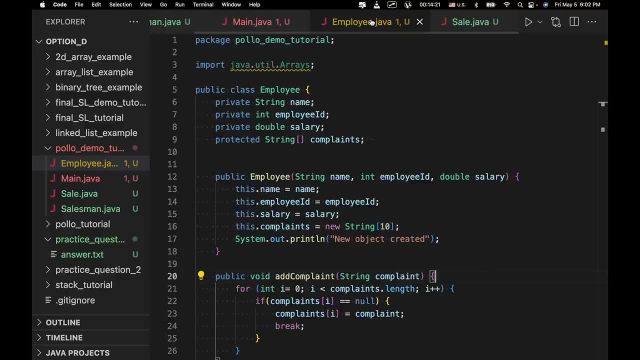 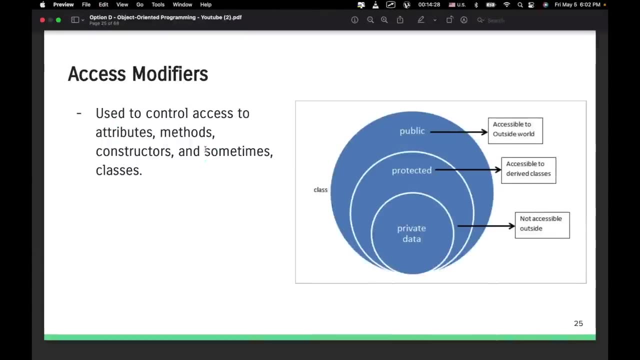 So that doesn't really make that much sense, But anyways, that can be done in a constructor, though there's not really a point to doing it. Anyways, so going back to this right here, public, protected and private. 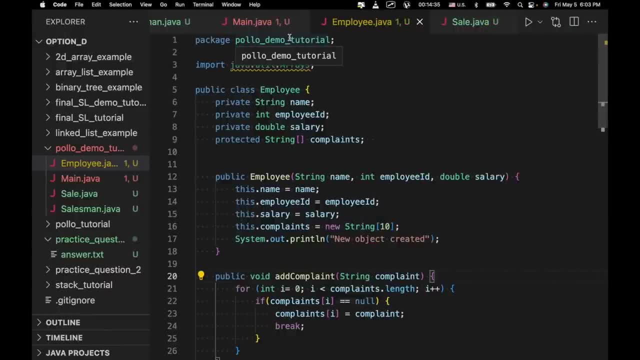 And yeah, so basically what? like? the reason that we're doing all of this is so that when we're working with other programmers, we don't want them to do anything they're not supposed to right. So if you want, 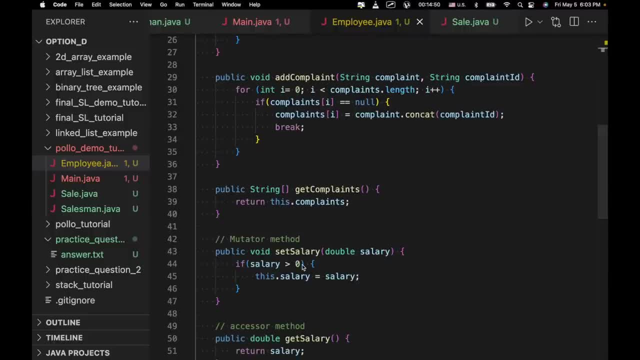 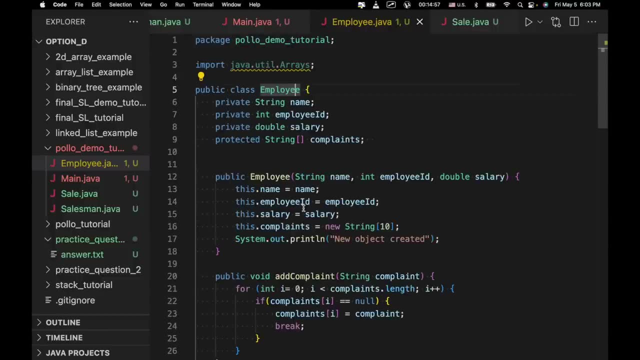 them to directly modify name. if you want to force other programmers to have to use this method, like get complaints or sorry, like set salary or set complaints or whatever. add complaints if you want to force them to use methods and play by our rules. 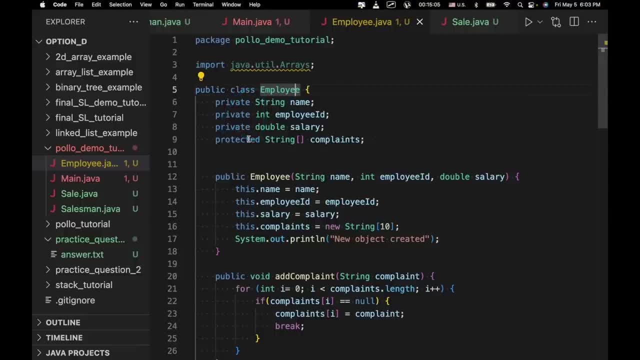 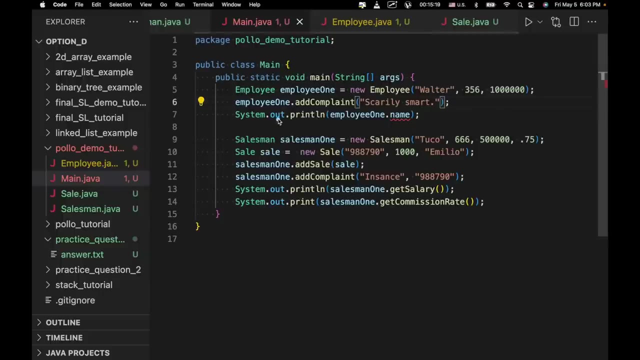 we can make them private And generally you're asking: okay, why couldn't those programmers just change this code? And you know, if we want to make sure that the code is in the class and subclass protected public means, we can just 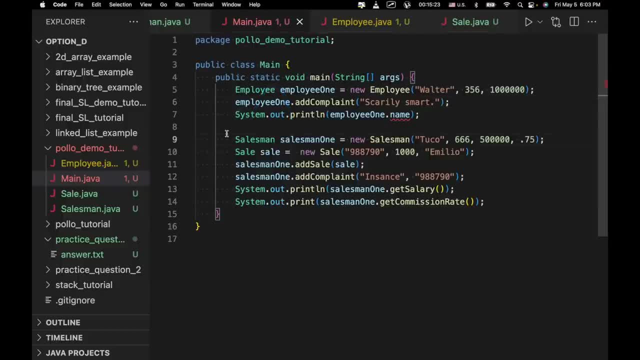 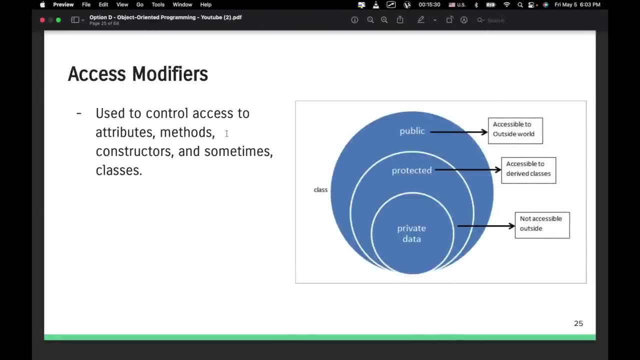 access these anywhere. Public is what we're leaving open to other, basically the main class and other aspects of our program. So access modifiers are used to prevent unauthorized access from other from code, from other programs, in order to make sure, in order to retain 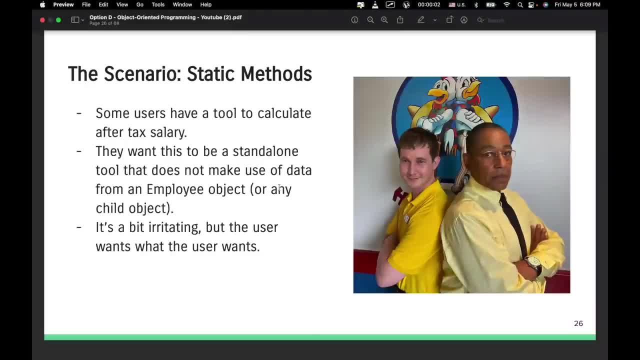 the integrity and maintain the functionality of our classes. Okay, let's talk about static methods. So, in our scenario, some users have a tool to calculate after-tax salary. Now, they want this to be a standalone tool. It does not make use. 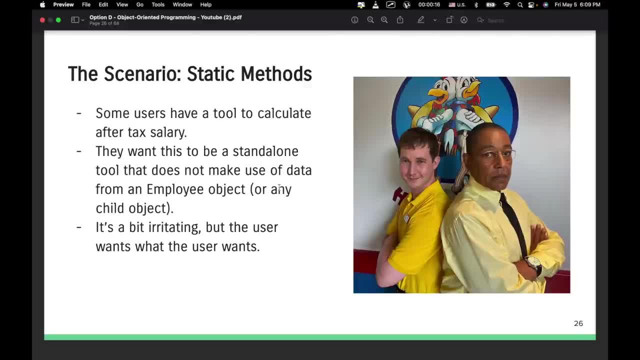 of any data from an employee object, but it's still a piece of functionality that's related to the employee object. Now it's a bit irritating, but the user wants what the user wants, So we're going to use something called a static method. 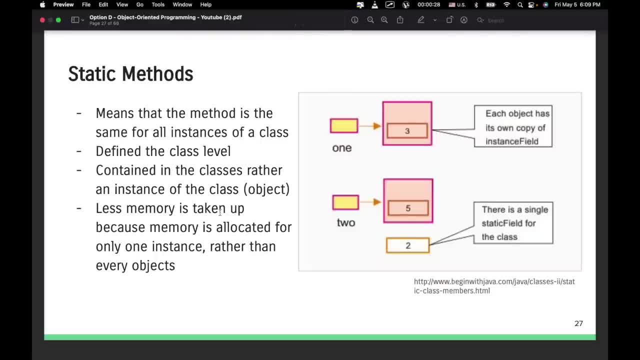 in order to implement this. Now, what a static method means is that the method is the same for all instances of a class, And before we get more into the theoretical underpinnings, let's go see what this looks like in code. 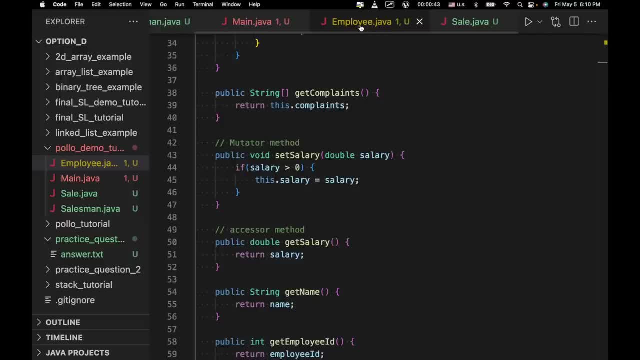 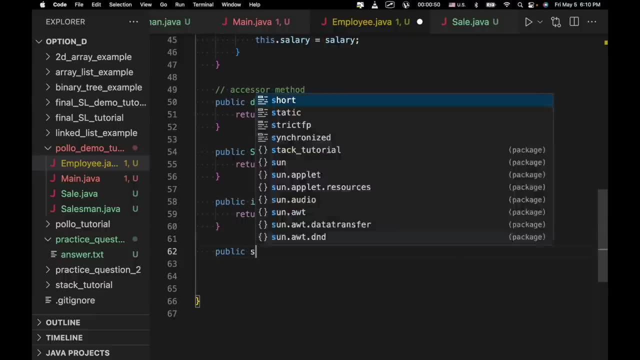 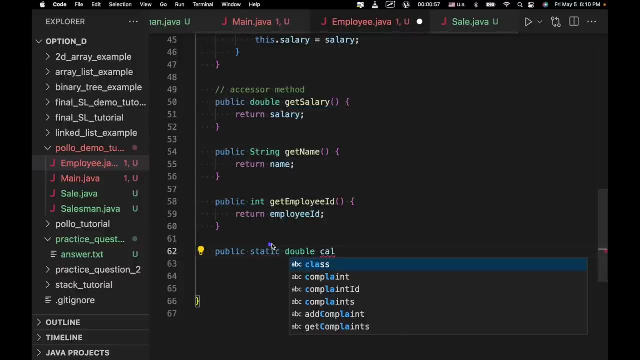 So what I'm going to do is I'm going to go to employeejava and I'm going to do- I'm probably going to go all the way down here- I'm going to do public static double calculate. Notice: the main difference: right here is static. 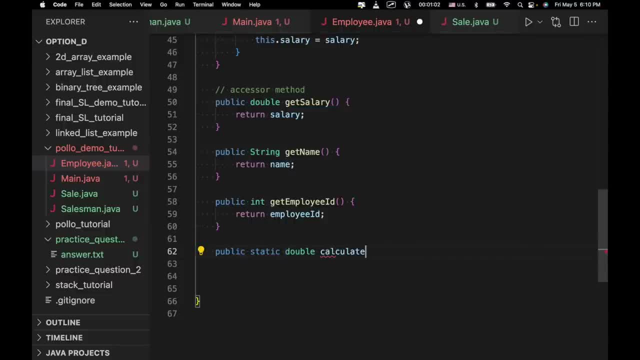 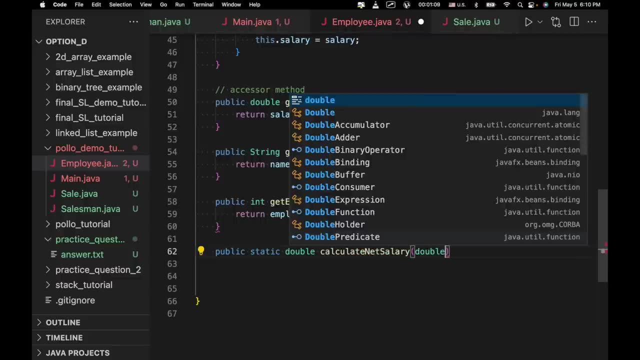 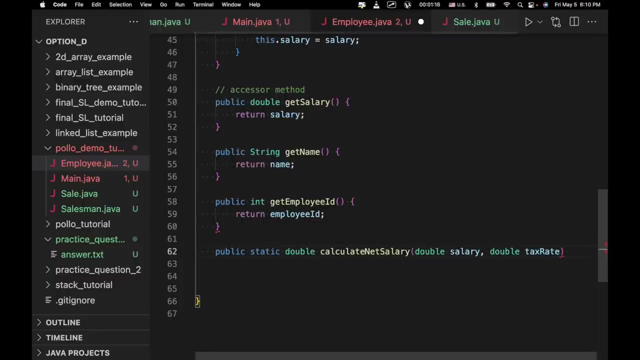 I'm using the static keyword Calculate after after calculating net salary, And my parameters are going to be the salary and the tax rate. So now that I've done that, I'm going to say: double taxable income equals salary times 1, minus tax rate. 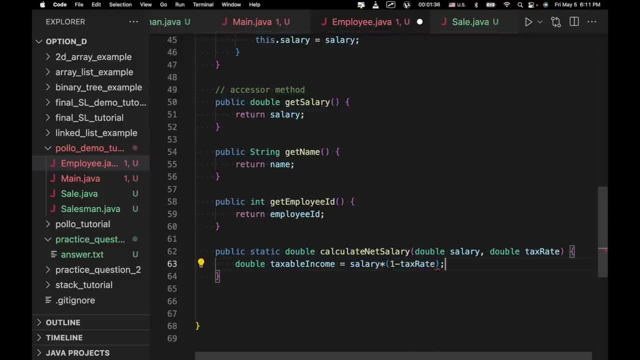 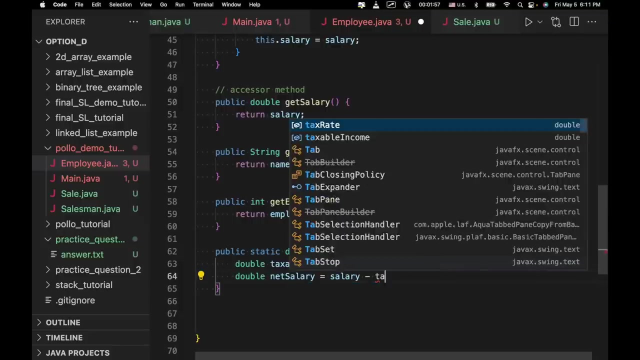 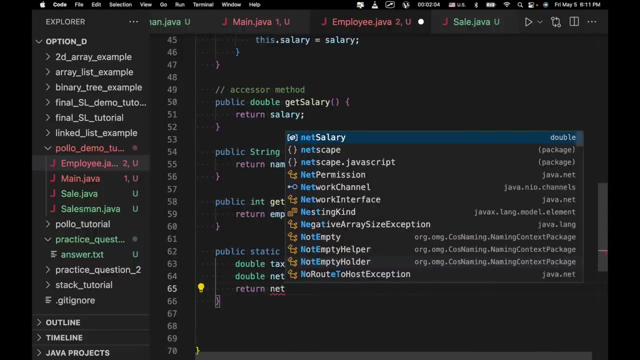 Now we can say: double net salary equals salary minus taxable income. Does that really make sense? Let's see salary times. yeah, okay, I guess that kind of makes sense. Oh well, And then we can just return the net salary. 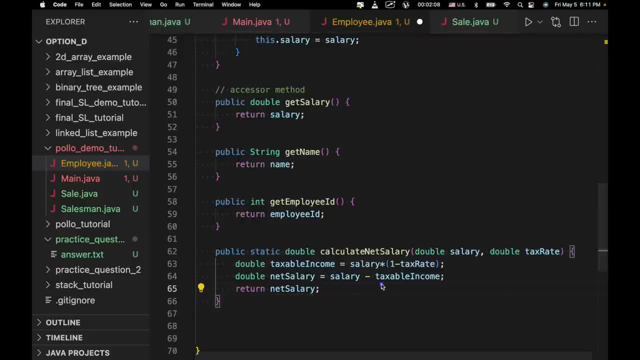 which is going to be a double. So keep in mind that in the body of our method right here, we're not using- we're not using any, anything from our class, So we're not using anything that would be in our object. 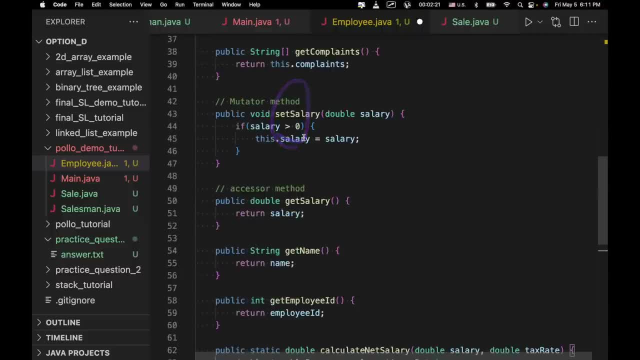 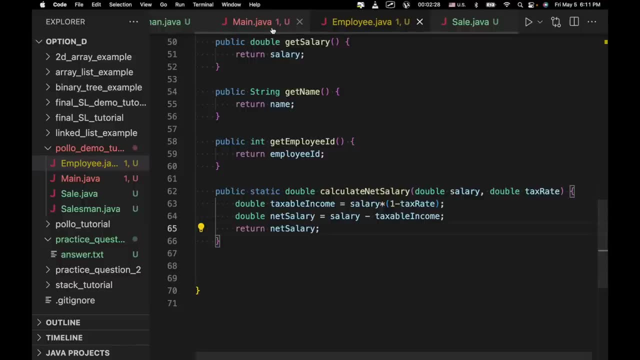 There's no this. there's none of our attributes that are being used here. This is kind of just a function that is its own thing and relies only on the parameters that have been put in, And once we do this, what we can do is: 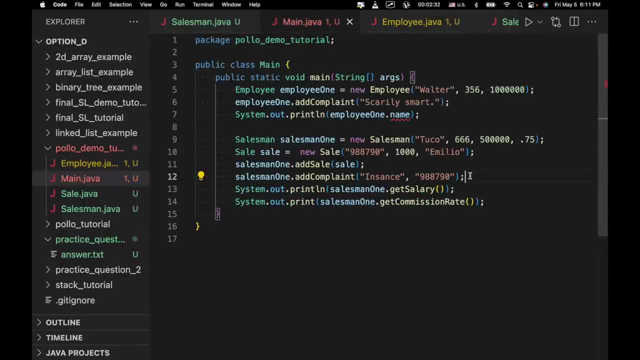 we can go to mainjava. The way we can make use of this is we can say: what we've issued right here, Oh yeah, we can't do that anymore. Anyways, what we can do is we could say, for example: 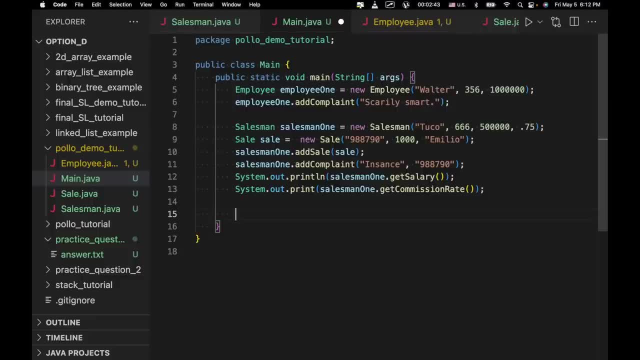 employee. we're not instantiating it at all. We're just going to say we could say: just say two cos after tax. Eh okay, Let's just choose a different character. Let's say sols, We'll say double. 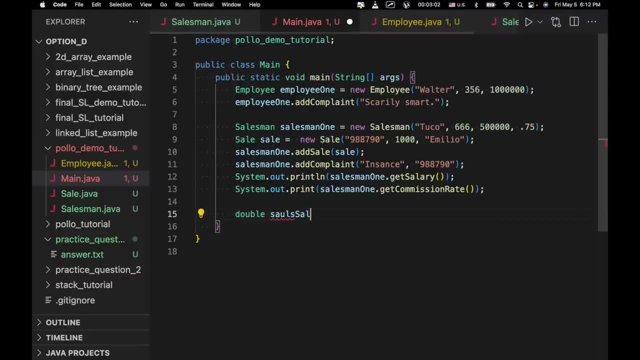 equals double sols salary. equals employee dot calculate net salary, and his salary is 40,000.. It's the old days and the tax rate is 0.25.. So then what we could do is we could just say: print sols salary. 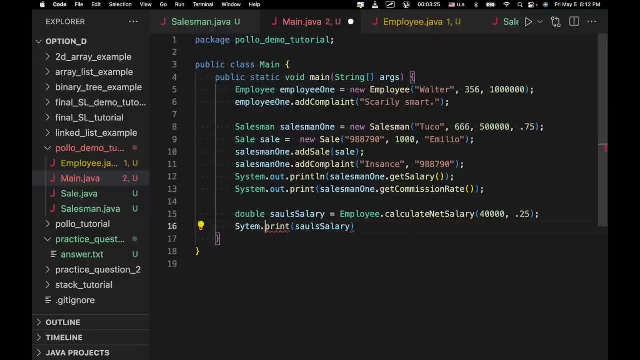 and sorry, not print. still thinking in terms of Python out dot print line sols, salary, and that should work. actually, Let's go ahead and get rid of these right here. I guess that should be insane And save it. And we have new object created. 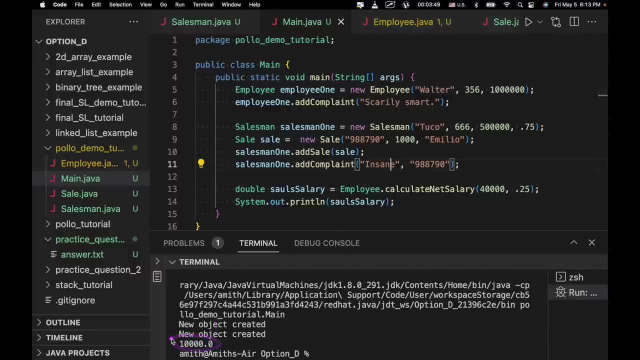 but we also have 10,000 right here, which makes sense, I guess. Kind of Well, maybe not. I guess I got the arithmetic wrong, But you get the point- Rather than having to instantiate an object and then call a method on that object- 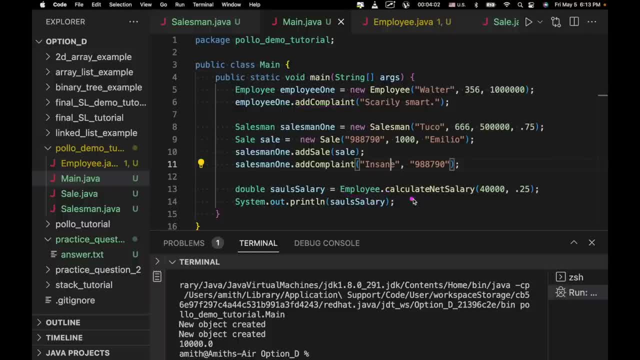 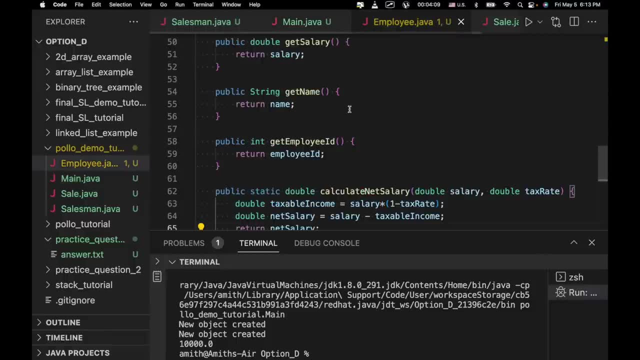 we can just call the method directly from the class. just do employee dot, calculate net salary, And that's basically how a static method works. We can also have static attributes. So, for example, if we did, we could say static. let's see static. 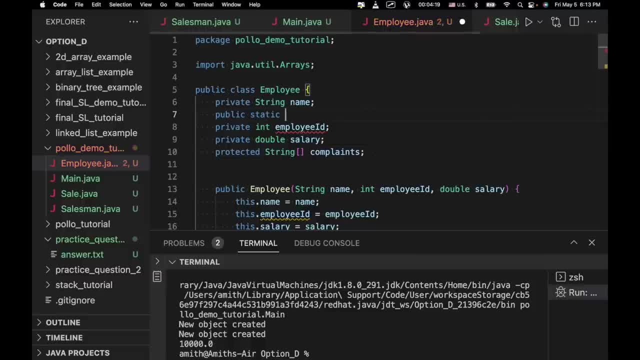 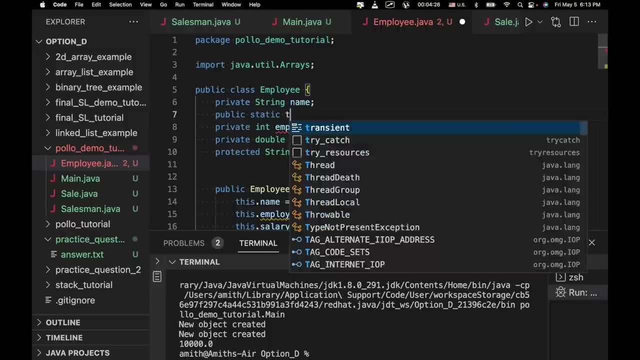 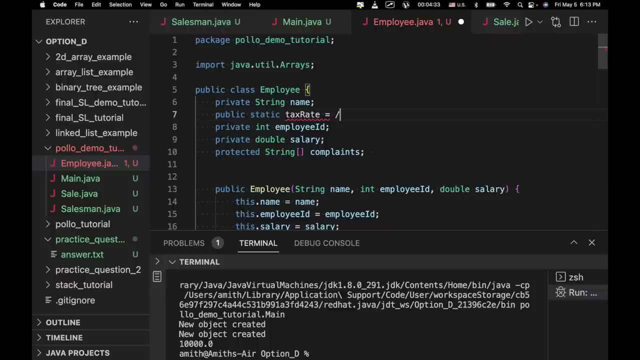 we could say public static, I'd say tax rate maybe, And we could set that equal to 0.3. Or just initialize that to 0.3.. Okay, so that's weird. We got to set a double and then 0.3.. 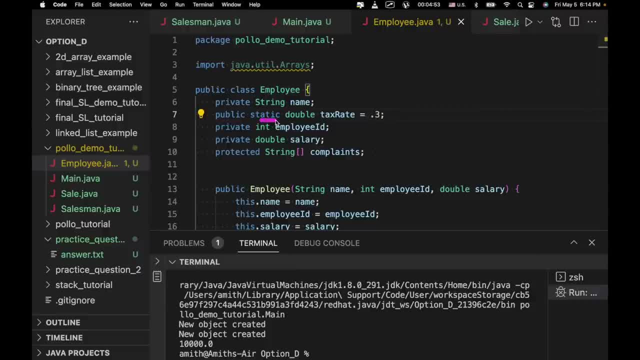 And we're not going to get into what the combination of public and private and static does, because we don't need to do that for the SL exam. But, safe to say, this is accessible anywhere outside of the class. If it was private then we would just do. 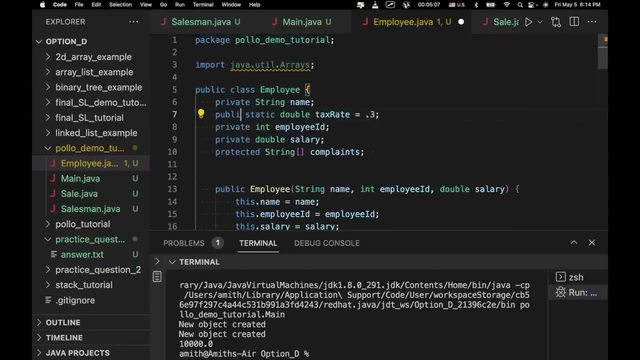 we would probably just do employee. So if this was private, for example, we would have to do. we'd have to do employee dot name. No, that's not going to work. Anyways, I'm not going to get into that at this point. 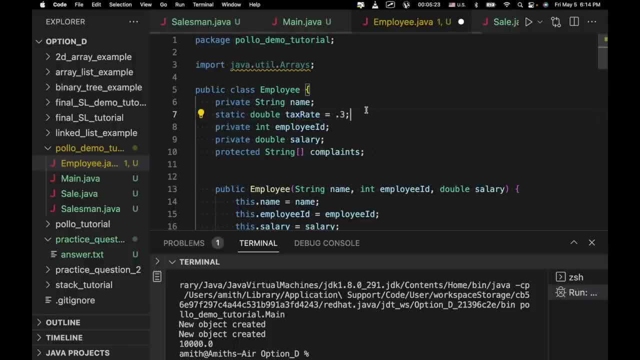 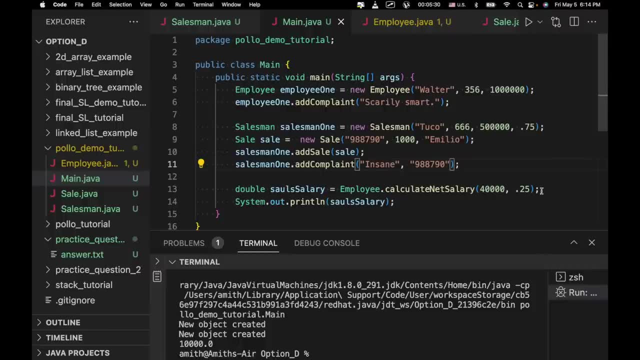 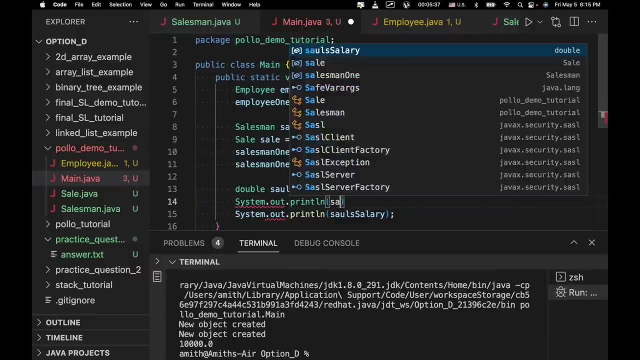 But we could even just leave it like this static double and it would do what it's supposed to do. In that case, we went to mainjava, We would just do SolveSalary, We could do systemoutprintln And then SolveSalary. 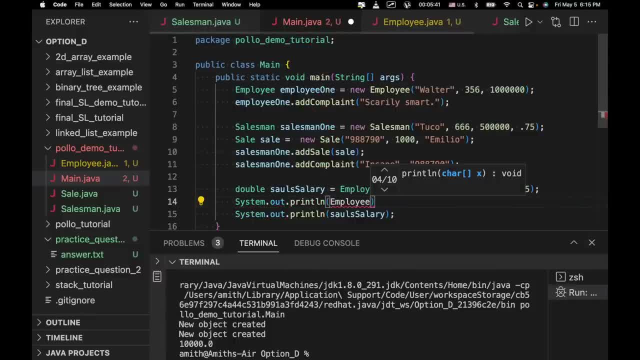 Actually not even SolveSalary. We could just do employeetaxRate. And again, we're not instantiating anything, It's just directly from the class. Now, static methods are the same for all instances of a class And it's defined at the class level, as we saw. 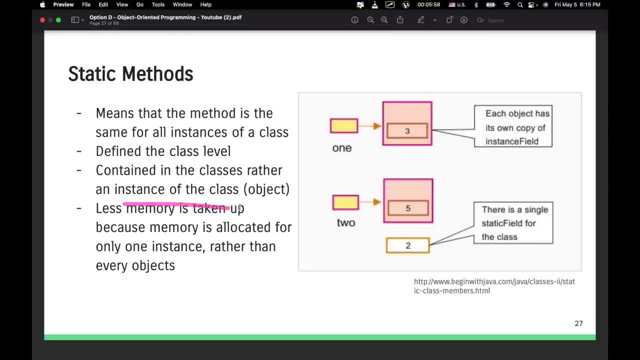 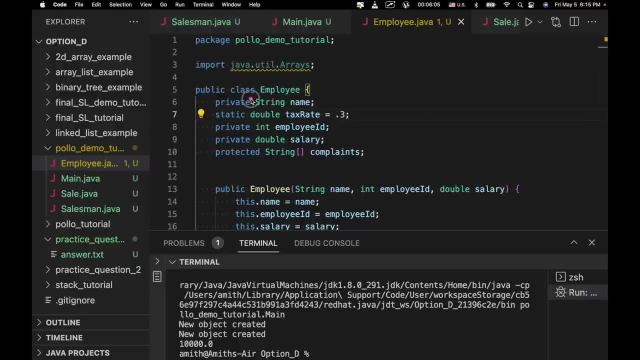 So it's going to be contained in the class rather than an instance of the class. So this isn't something that's attached to an object, like these other attributes that aren't static right here. So all of these non-static attributes besides this one, 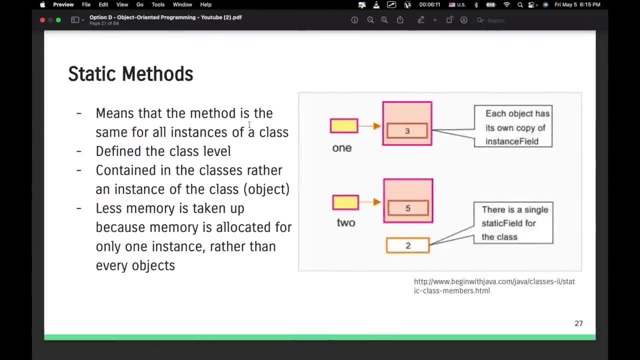 are attached to a specific object instance. So you're going to create an object and then you're going to give these all values. However, with the static method or attribute, it's just attached to the class And because it's only allocated- 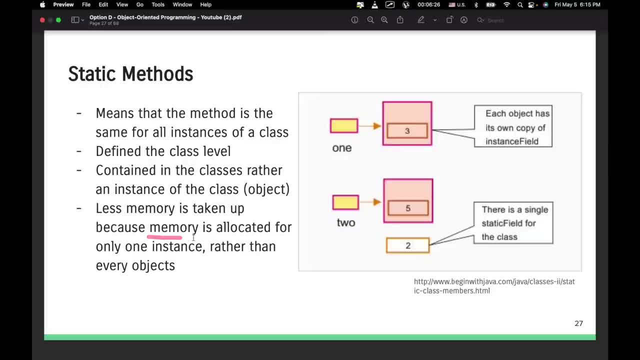 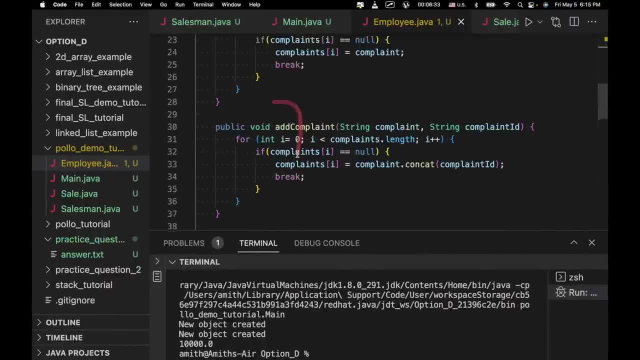 and because it's only attached to the class. we only need to allocate memory for one instance rather than for every single object, Because otherwise, every single time you create an object, we're using memory to store the attributes, the methods, et cetera. 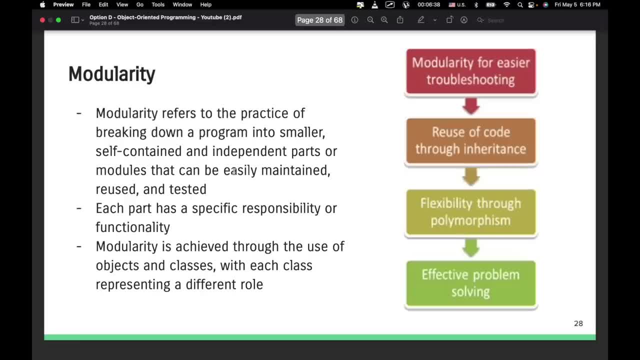 So it's actually more memory efficient. And the next concept we're going to cover is going to be modularity. So modularity- this is just something you need to know. It's kind of representative of what we are doing when we're doing object-oriented programming. 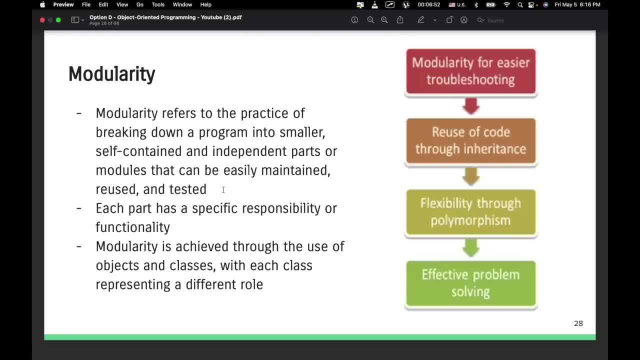 or what we're trying to achieve Now. modularity refers to the practice of breaking down a program into smaller, self-contained and independent parts, So basically taking a large program and breaking it down into smaller parts that can work together but that can be individually maintained. 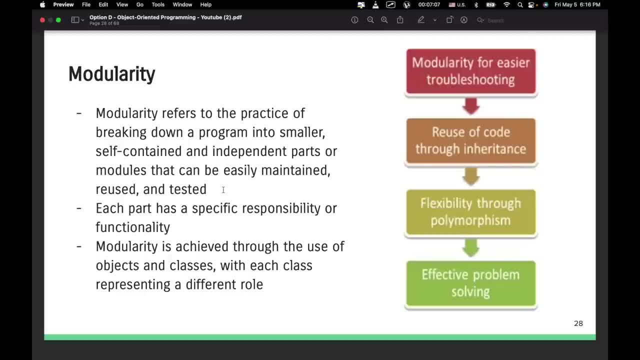 reused and tested. So every single part has a specific responsibility, like every single class in an object-oriented programming, and an object-oriented program has a specific responsibility or functionality. So, obviously, modularity is achieved through the use of objects and classes and the use of objects and classes. 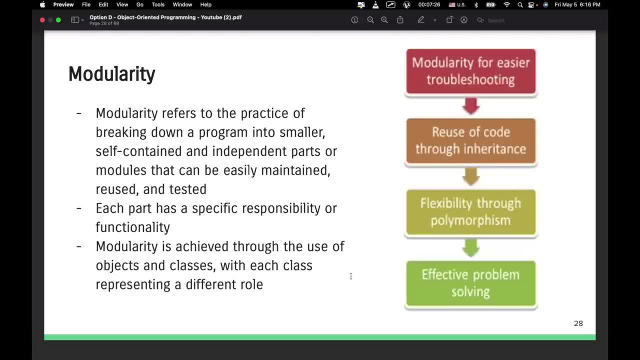 in a class representing a different role. I say obviously because this is literally repeating what I just said. So, if we're talking about object-oriented programming as a concept, we have flexibility through polymorphism, reuse of code through inheritance, and we have good organization, maintainability. 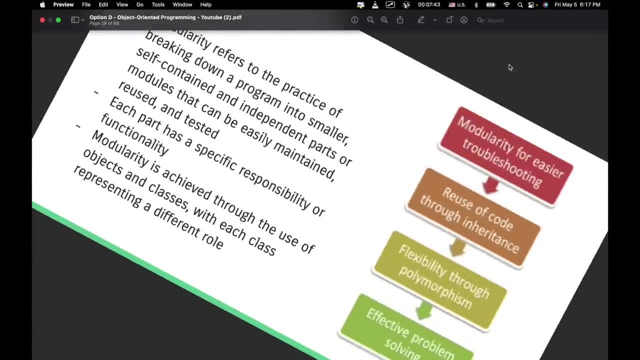 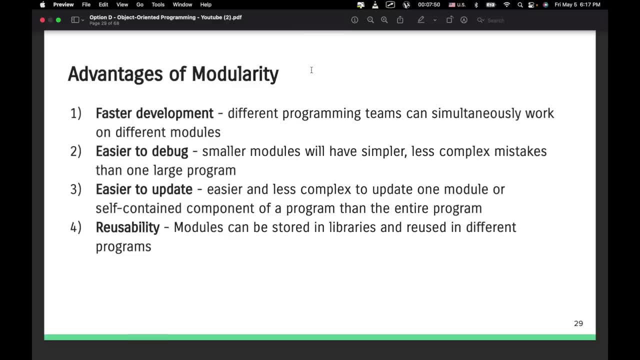 and easy debugging through modularity And those kind of all lead to effective problem solving. I don't know why I just did that, Okay. So some of the advantages of modularity are that it's easier to debug and faster development, So different programming teams can work. 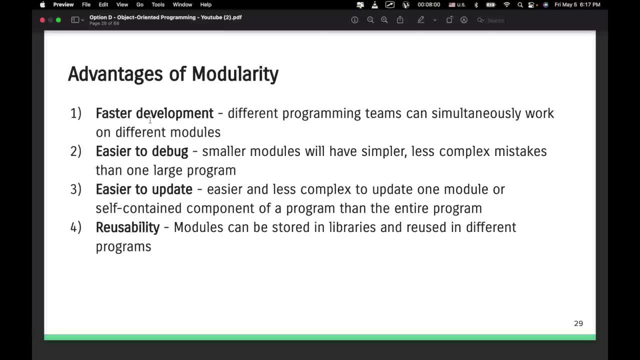 on different components separate from each other, and they can put them together because they're working on modules. It's also easier to debug because if you want to find a problem, you can look at each individual module or you can see which module failed, rather than trying to have to look at the program as a whole. 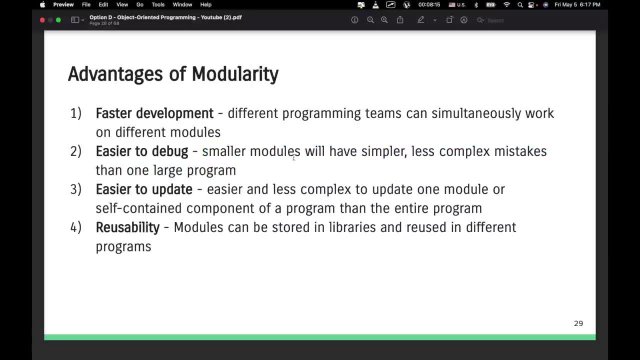 And smaller modules, because they have less code, will lead to simpler, less complex mistakes that are easier to debug, Easier to update. So it's easier to update just one module or one piece of a program rather than the entire program itself. 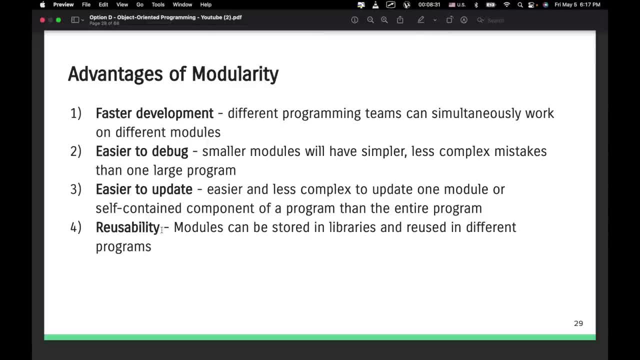 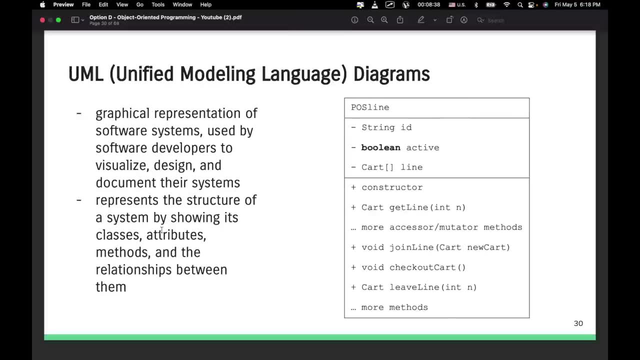 Reusability: You can take modules from libraries or from one program and use them in another program. Now one of the final concepts we're going to go over is just how to graphically approach object-oriented programs. And now the most common way. 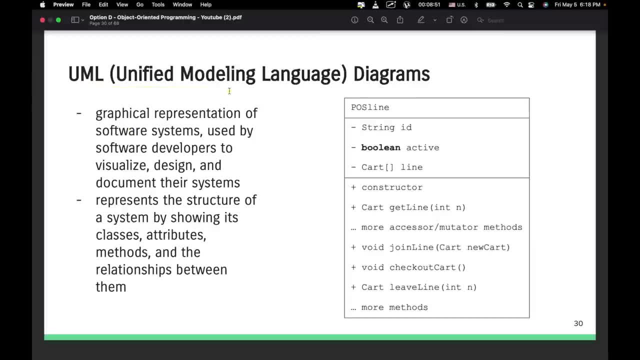 is by using UML diagrams or unified modeling language diagrams. Now, these are graphical representations of software systems used by software developers to visualize, design and document their systems, And through those we can see classes, attributes, methods and relationships between the classes. 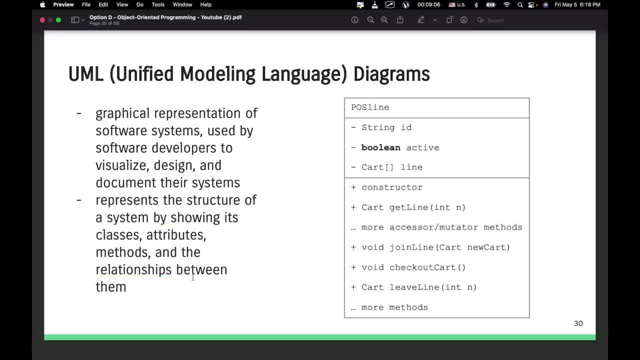 Although, weirdly, in the IB, like in the IB exam in general, we don't use UML to illustrate relationships. They have their own weird way of illustrating them, which we'll go into here in a second, And this is an example class. 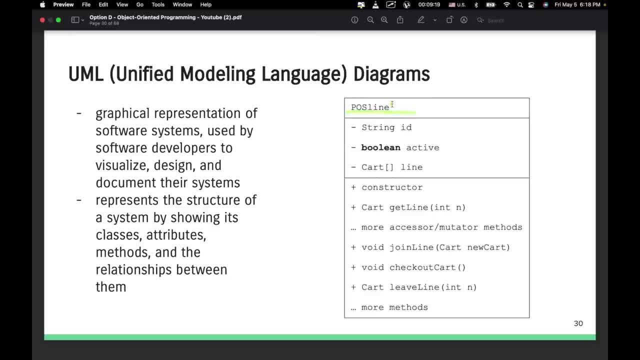 or an example UML diagram for a class called POSLINE. So at the top we're going to have the name of the class, Then we're going to have the attributes in the second portion and then all the methods in the third portion. 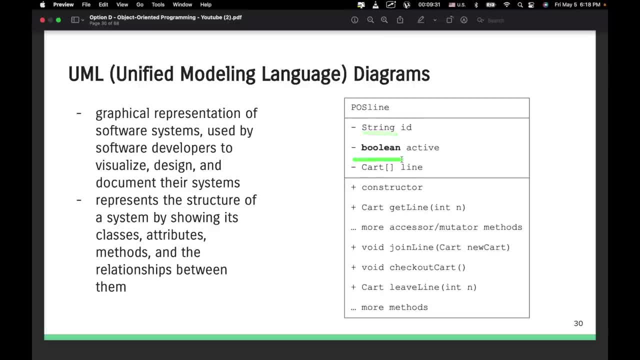 And with all of the attributes, we're going to have the data types And then, with all the methods, we're going to have the return types, as well as the parameters, with their types as well. Now, these minus and plus signs stand for public and private. 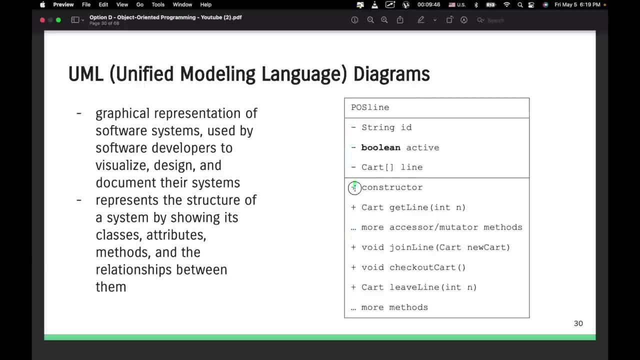 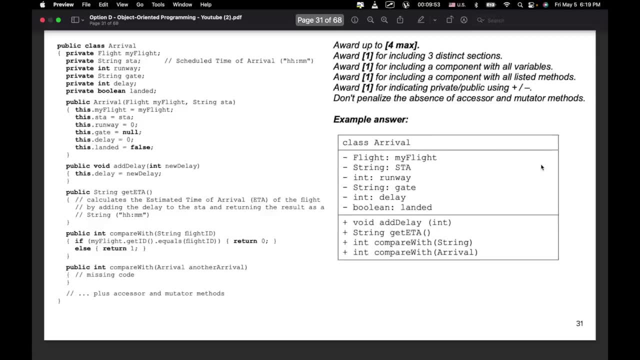 So minus means private and plus means public, And then an ampersand, so like an, and sign generally means protected. So right here- sorry, it's not an ampersand- a hashtag means protected. So right here we have this class. 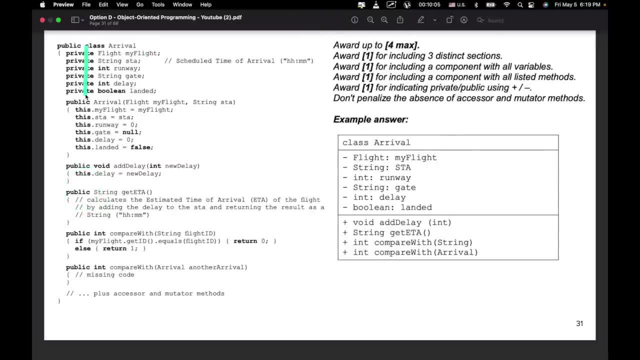 It may be difficult to see. We've got a bunch of private attributes, So these are all minus and we have all of their data types as well, with a colon and then the name of the variable itself. So right here we have flight myFlight. 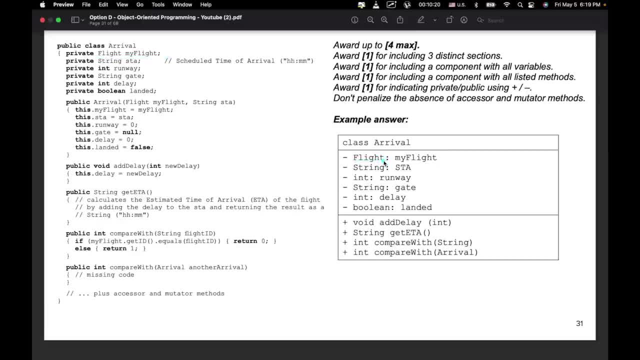 So we have flight, the data type, followed by the colon, followed by colon and then the name of the variable. Actually, if you went back here it wasn't exactly illustrated that way. I don't think it makes a difference on the IB exam. 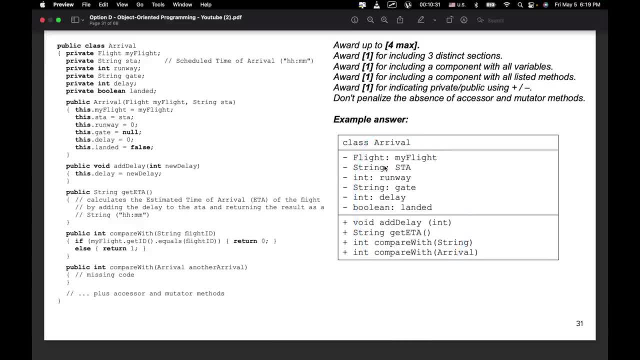 but this is taken directly from mark scheme, So this is probably best to go with having the colon in between. And right here we have our methods, which are all public right here, And we've got our return data types as well as our parameters. 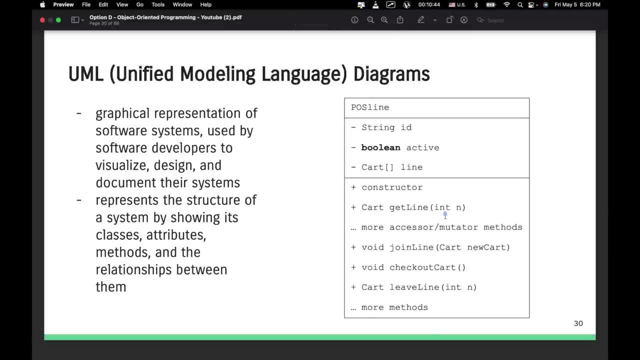 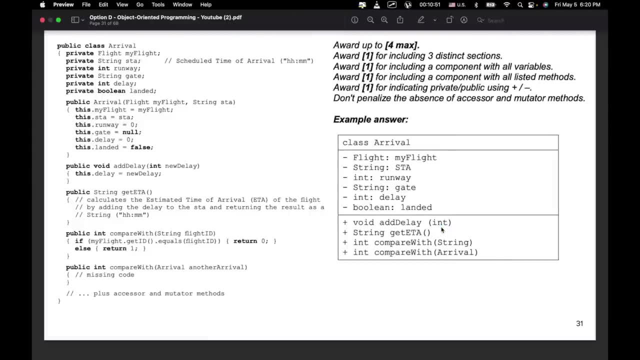 Here we actually don't have the parameter names. Here we have the parameter names like int, n and then u, cart. Here we just have the data types of the parameters, but I'd actually recommend including the names of those variables as well. 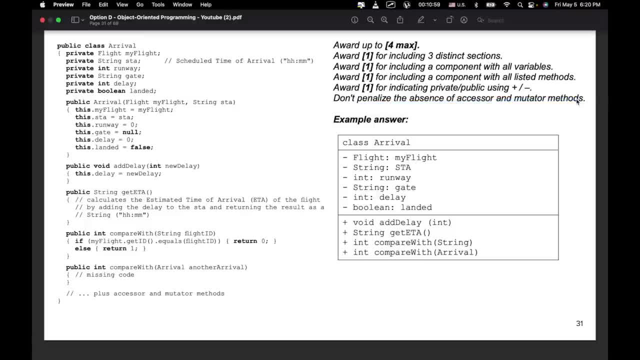 It says: don't penalize the absence of accessor and mutator methods. So remember, accessor and mutator methods are like set runway, get runway, set gate, get gate, And you don't necessarily need to put those if they're just accessors and mutator methods. 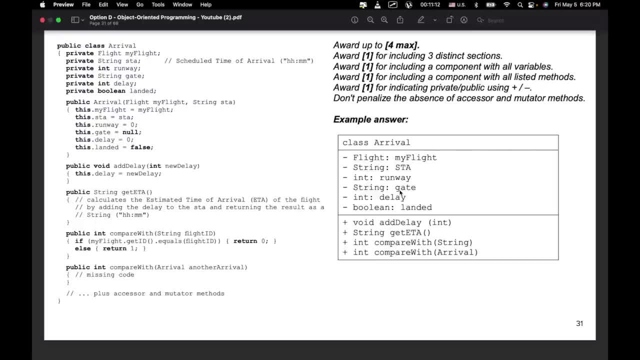 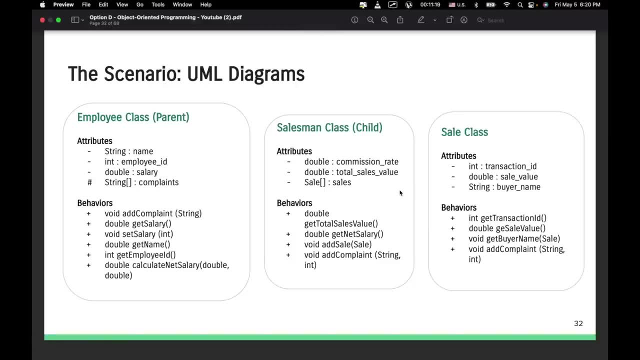 In fact, on the exam you'll be expected to just assume that those exist. Now for our own program, for our scenario. right here these are UML diagrams. So in the employee class we had these four attributes. Three of them are private. 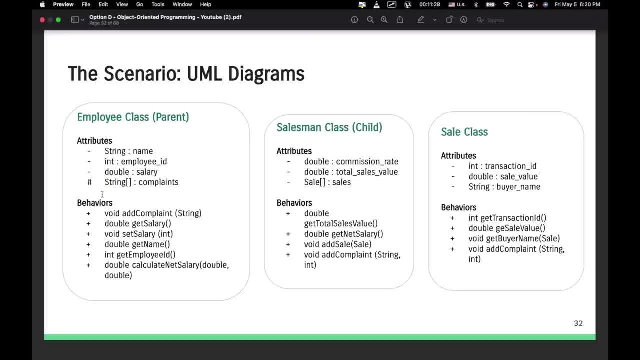 One of them is protected, hence the hashtag. And we had all these public methods. These are pretty run of the mill. Just kind of illustrates as a whole what our program looks like. Now here's an example of a diagram. We haven't really drawn one for our own class. 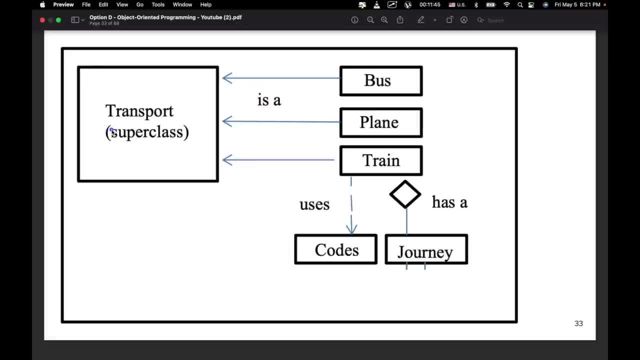 But right here we have a transport superclass And we have is a right here. So this is our diagram, This is our transport class And we have these arrows pointing towards it, because bus, plane and train are all subclasses of our transport superclass. 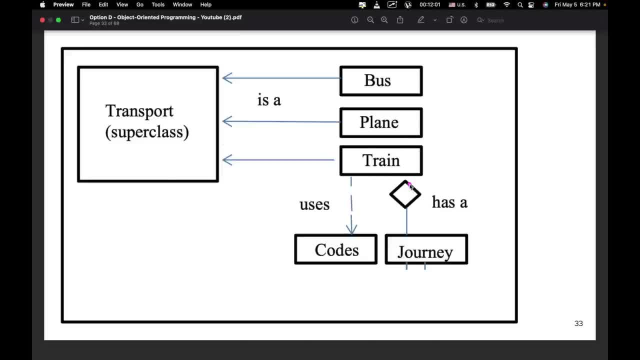 And then we have a train followed with a diamond and an arrow. So the diamond with the has a means that there are many journeys for one train. So there's an aggregate relationship here. So remember on our own program when we had a salesman with many sales. 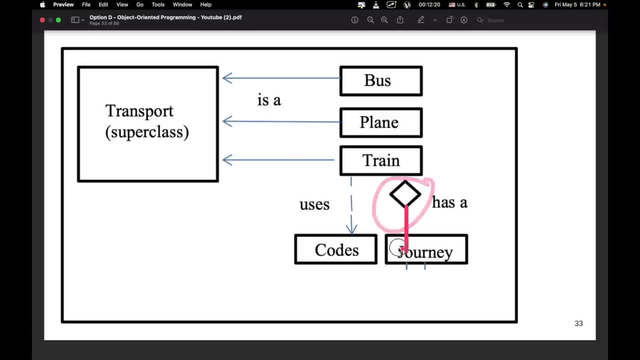 there. we would have salesman right here with a diamond and an arrow pointing to sales And train just uses instances of codes. There's no hierarchical relationship, There's no subclass, superclass or aggregation relationship, But we're just going to have some code objects. 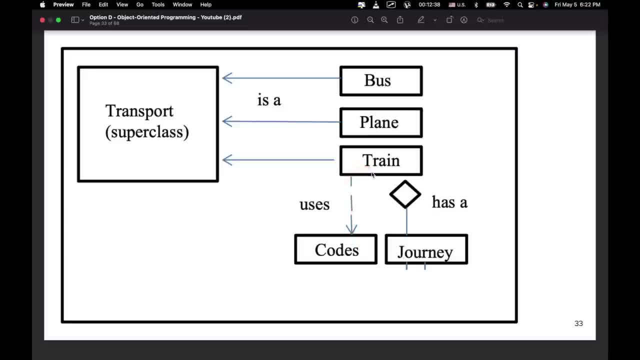 in our train class right here. Or we might just have one code object in our train class And that doesn't mean it's going to be an attribute. That just means we're going to use it in a method, And we'll see more about this in our exam-based example. 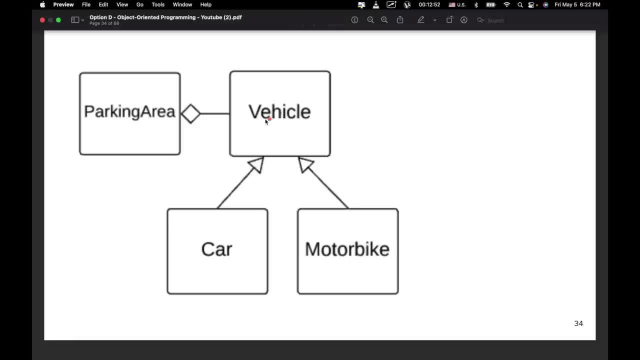 Here's another example right here. So we have a vehicle class- The car and motorbike are subclasses of the superclass- And the vehicle has an aggregate relationship with parking area. Or sorry, I mean parking area has an aggregate relationship with the vehicle. 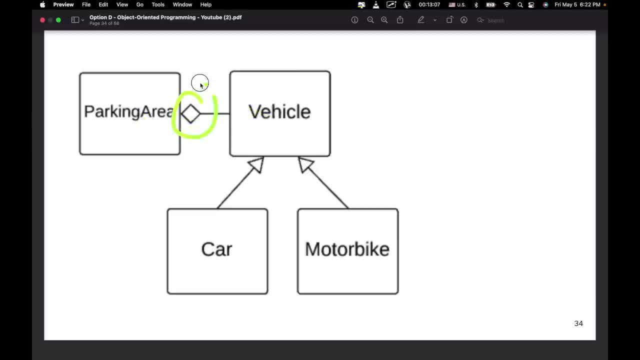 So that means a parking area has many vehicles. That's why we have this diamond and this arrow: The parking area has many vehicles And the vehicle is a superclass to the subclass of car and motorbike. And those are basically relationship diagrams. But let's go ahead and let's draw one. 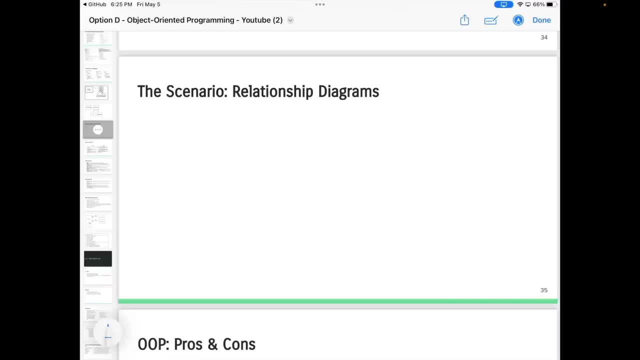 of our own, Okay. so what we're basically going to do right here is we are going to have: Okay, this is my terrible drawing, So you've got an employee class Employee, And then we're going to have our salesman class. 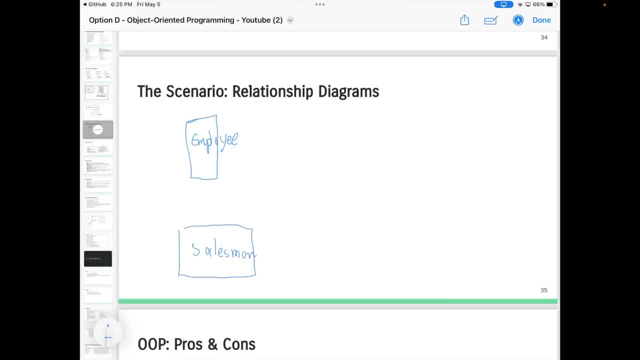 That's going to be pointing up to our employee class, And then our salesman class has many sales, So we're going to have a little diamond there And then that's going to be pointing to our sale class, And that's basically what we have in our own scenario. 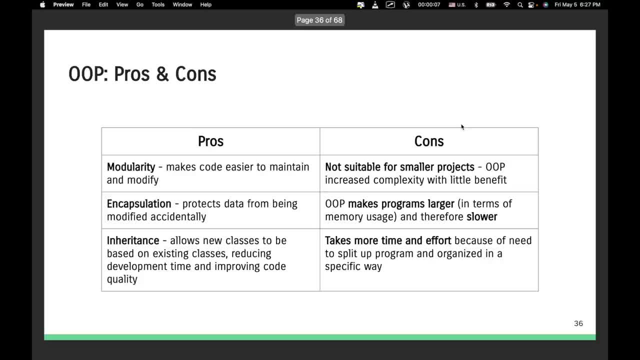 Again, sorry for the terrible drawing. I am far from an artist. Okay, so next, now that we've kind of gone over a lot of the main object-oriented programming concepts, what I want to do is I want to talk about the pros and cons. 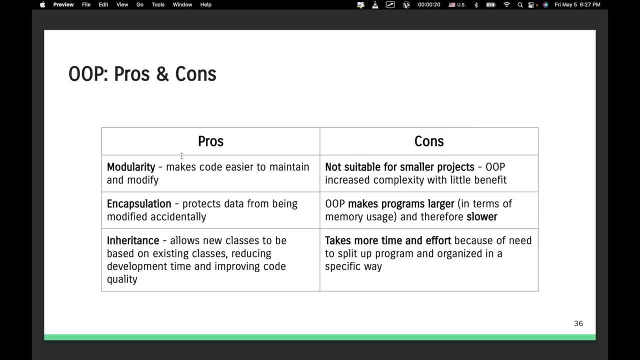 So some of the pros of OOP are: modularity: Code is easier to maintain and modify. There's no encapsulation. You have some protection against data from being modified accidentally through private, protected and public. And inheritance, which allows new classes to be based on existing classes. 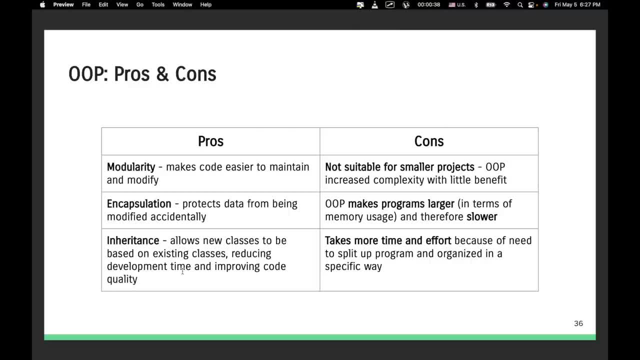 And that means that we can reuse code And we can easily make changes across a wide number of classes. Now, some of the cons are that OOP isn't suitable for smaller projects, So if we're just writing a simple script like just maybe to- I don't know, 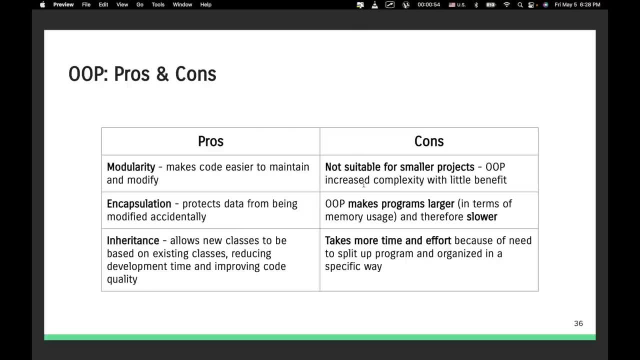 calculate, calculate, sign or something like that. using object-oriented programming would just increase the complexity with no real benefit. Also, object-oriented programmers. object-oriented programs take up more memory and are therefore slower. And finally, just this whole process of modularity takes more time and effort. 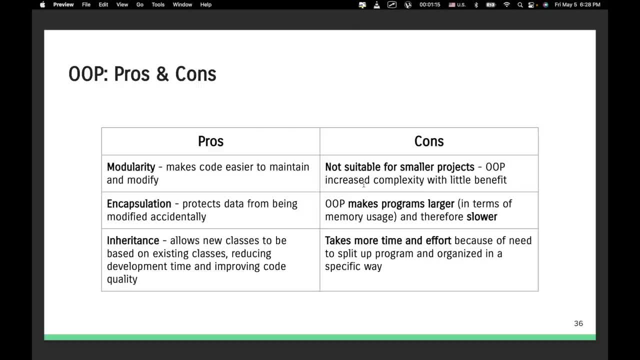 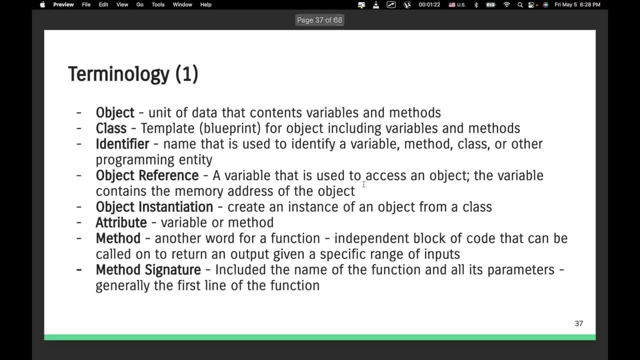 Like, I think the payoff is there, but it is just going to take more time and effort than just writing a program in a more procedural manner without the use of object-oriented programming. All right, So here we have a list of different terms. 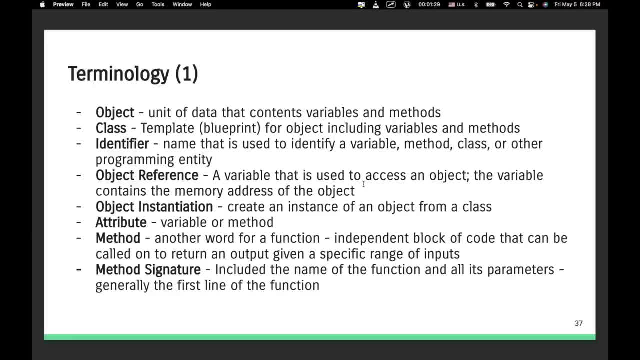 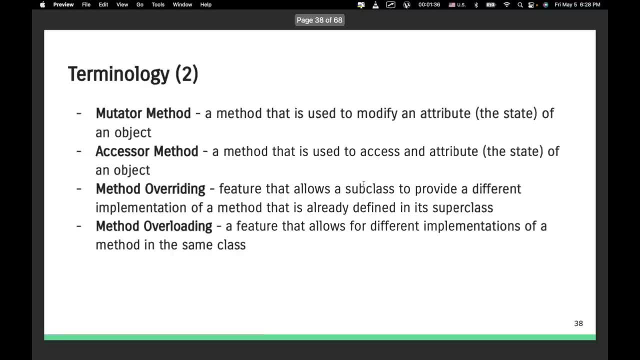 We've gone over all of these. What I'm going to do is I'm going to include this slide, most likely in the description, And you're going to have access to all of these terms. I think the only one I want to go over that we haven't gone over. 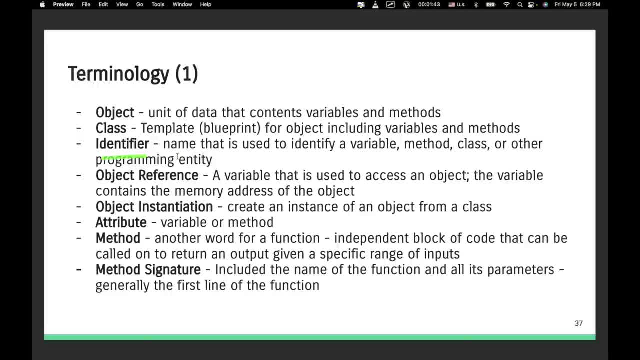 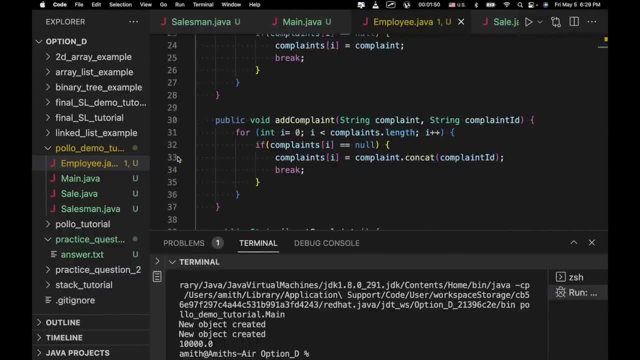 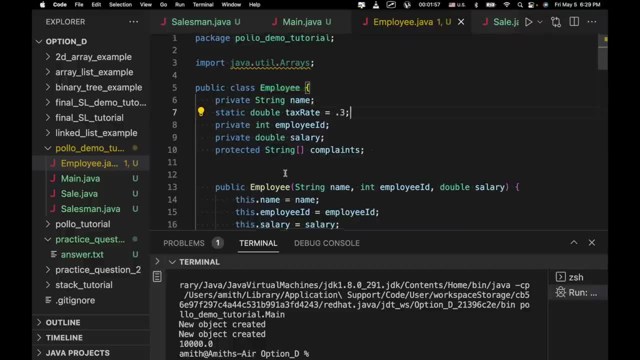 the only two is identifier. Now, identifier is just a name that is used to identify a variable method, class or other programming entity. So, for example, if we're looking at our code right here, name would be identifier, employee would be an identifier. 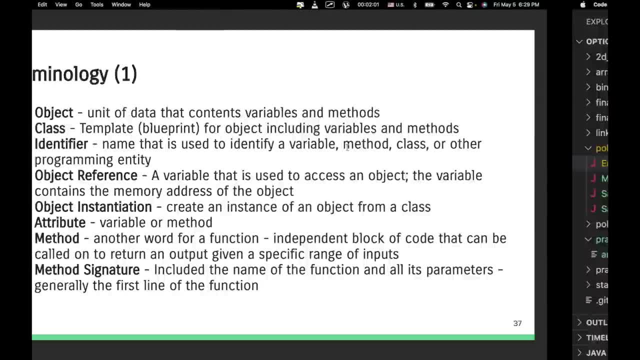 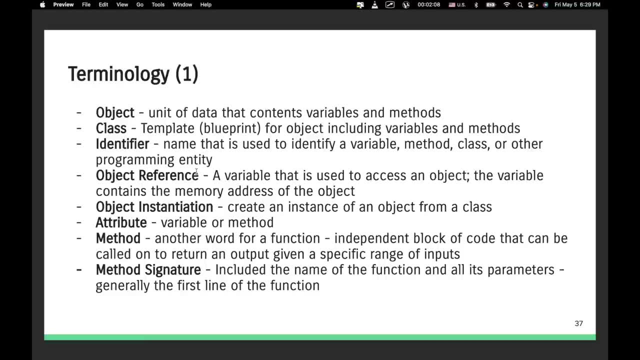 Right here. add complaint would be an identifier. Those are all classified as identifiers. Additional object reference. So when we're talking about object reference, we're talking about a variable that is used to access an object, So that variable contains the memory address of the object. 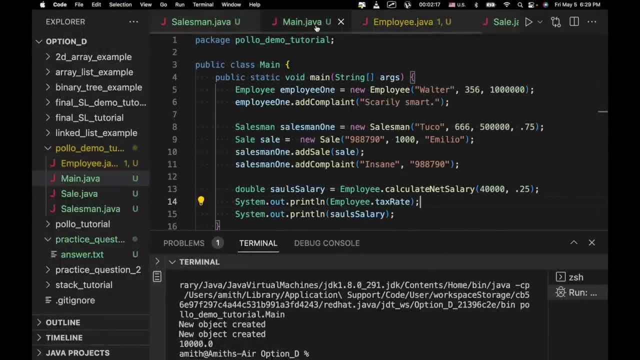 which is the reference. So right here, when we have employee employee1, and that's basically a reference to this employee object, That's an object reference to this object that we've created right here, The other terms we went through in this slideshow. 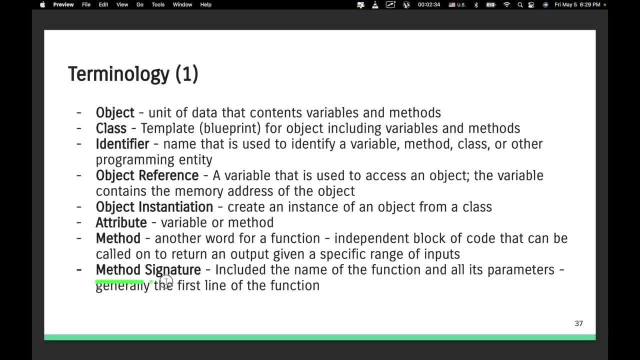 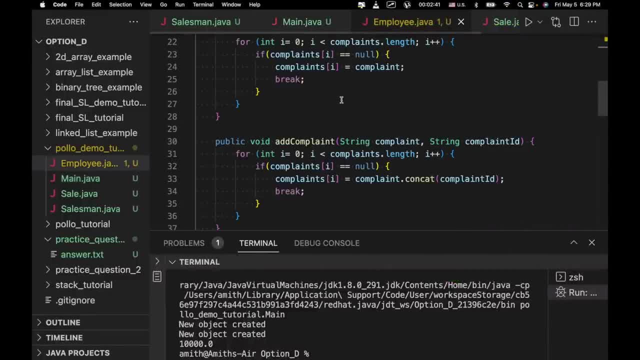 or in this video also, I guess, method signature. So that includes the name of the function and all of its parameters. So right here the method signature would be: let's see an employee. It would actually include this part as well. 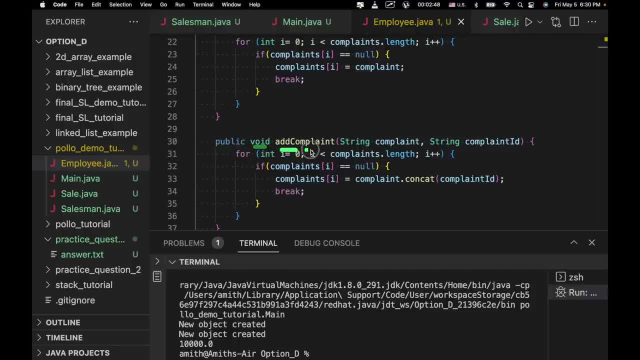 So we'd have public void, the return type, the name of the method and then all the parameters. I mean there are two variations. I've seen definitions include this. I've also seen definitions that just include the name as well as the parameters. 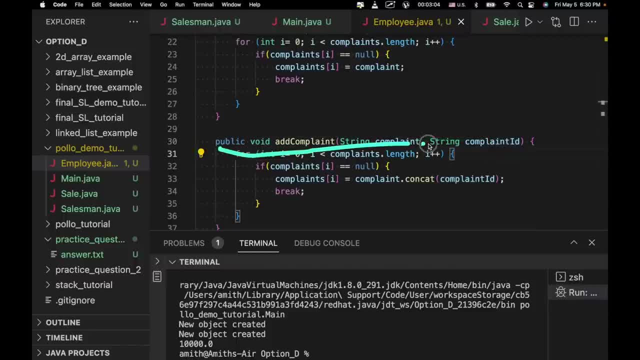 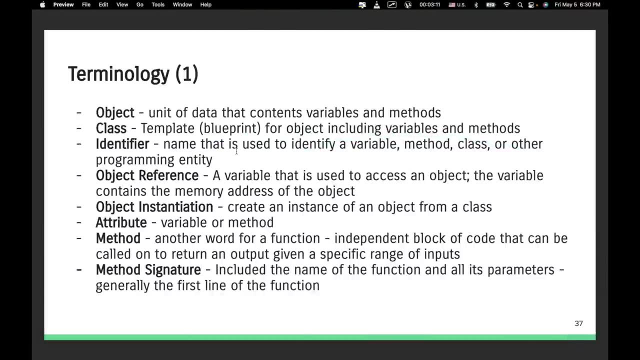 I would say in Java this would make sense to be the method signature. But if anyone's asking you for the method signature, it's not going to hurt to write all of this. These we've all gone over, Okay. so I kind of had a little project planned. 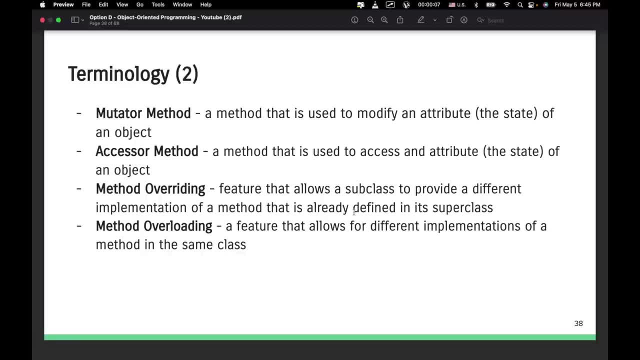 But I think, in the interest of brevity, we're just going to go straight to an example. Basically, I just worked out an example paper too, And I think that'll probably give you more insight into the exam and into these programs in practice than the tedious. 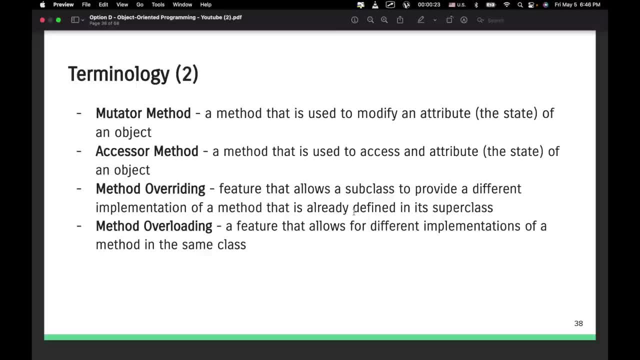 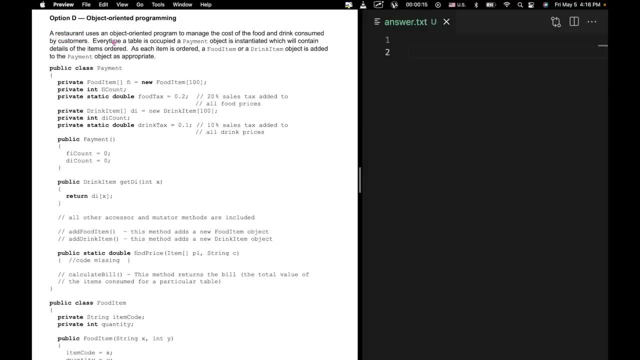 project that I made up would. So let's go ahead and let's get started with that. So right here it says: a restaurant uses an object-oriented program to manage the cost of the food and drink consumed by customers Every time a table is. 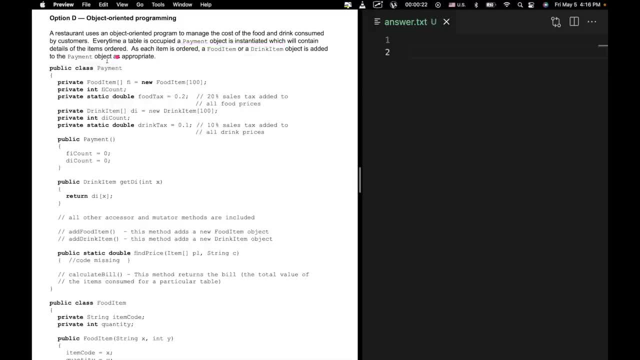 occupied, a payment object is instantiated, Which will contain the details of the items ordered. So, basically, we have a restaurant, we've got tables in that restaurant And every time someone sits down at a table, that is going to be represented by a payment object. 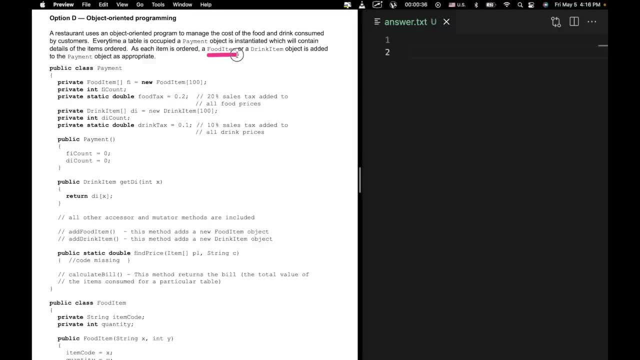 And connected to each payment object is a well. it says, as each item is ordered, a food item or drink item object is added to the payment object as appropriate. So if you look down at the payment class, we actually have an array of food items and we have an array of drink items. 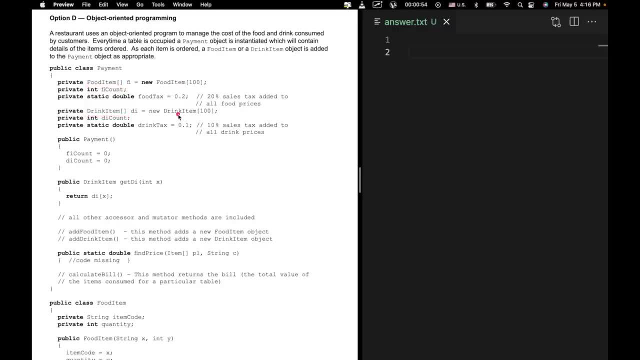 And because these are food item and drink item type, we can assume there's also a food item class and a drink item class. In addition, we have other attributes. So we've got an integer of phi count which presumably keeps track of the number of food items and we have an integer. 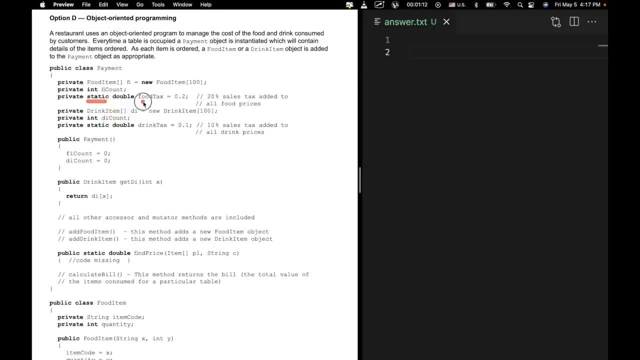 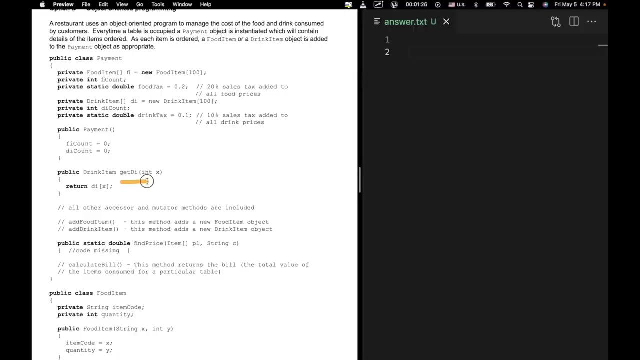 die count, which keeps track of the die items. We also have a static food tax and a static drink tax right here, And we have our constructor, in which the phi count and die count are initialized to zero. Beyond that, we're going to have a get die method. 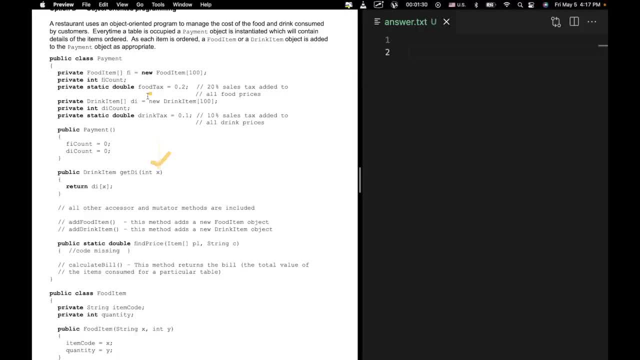 So based on the index entered, we can get a specific drink item And it says all other accessor methods are included. So we have add food item, add drink item and presumably we also have a get phi as well. It also returns a specific item. 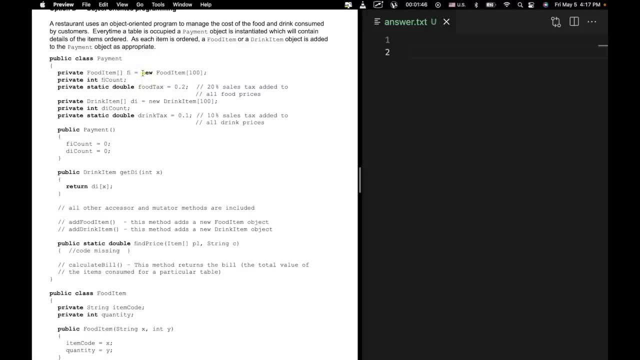 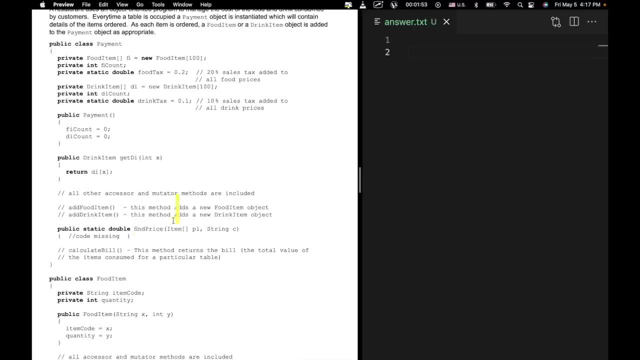 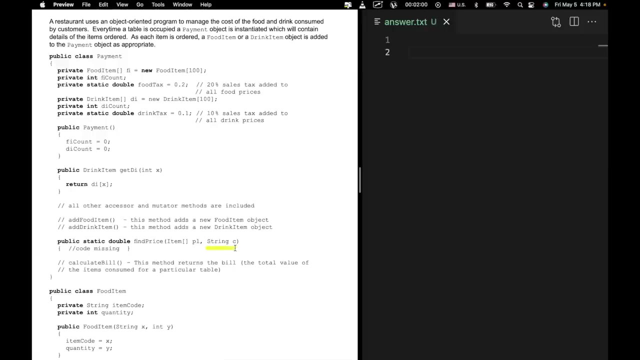 in the phi array. We have another static method here which is find price And that takes an input of items- And I don't know what that is yet. I guess presumably we'll see that later on- And a string c And a calculate. 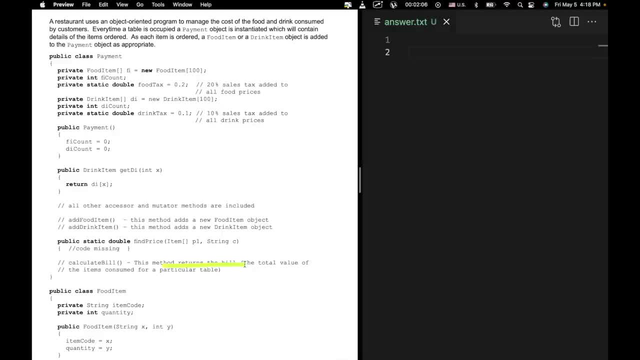 bill item here, which is not as clear, That returns the bill or the total value of the items consumed for a particular table And that's not inside the static method. that's just kinda here which is weird, But anyways, moving on, We also have this is our food item. 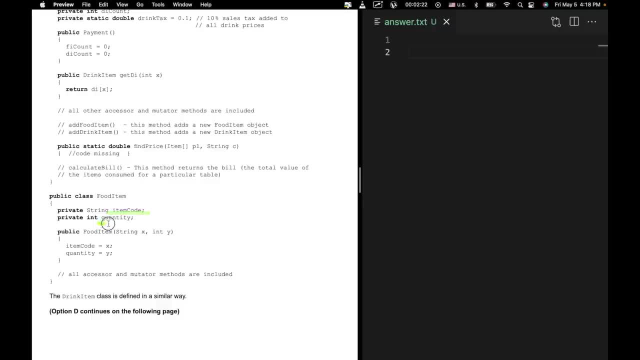 method and we have a item code attribute and a quantity attribute, as well as a constructor, which both of these are initialized to, whatever the, to the input parameters, As well as accessors and mutators, presumably for both of these, And a drink item that is defined. it's basically 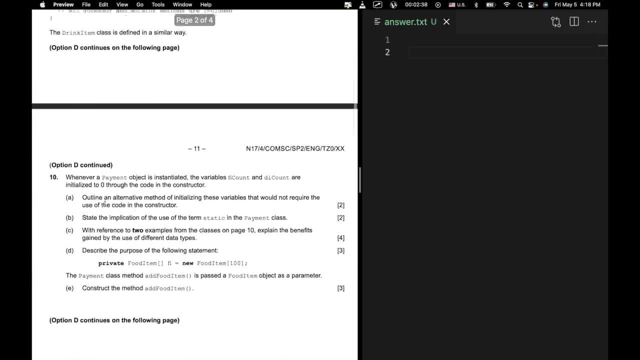 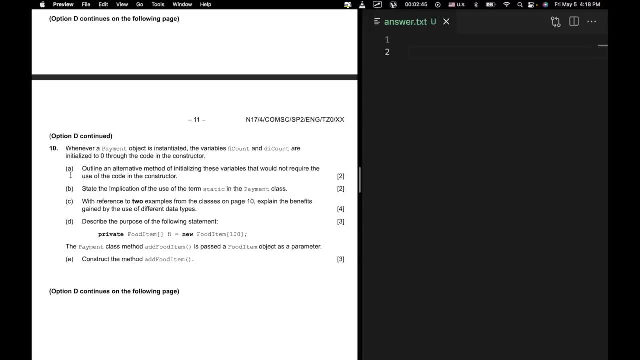 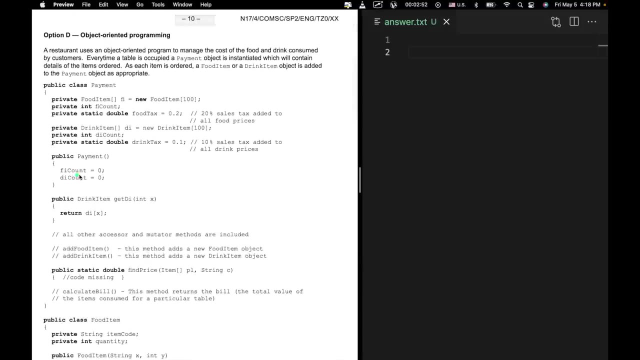 the same thing as this. So, going to our first question, we have A Outline, an alternative method of initializing these variables that would not require the use of the code in the constructor. Now, basically, right here in the constructor, we initialize these to 0. 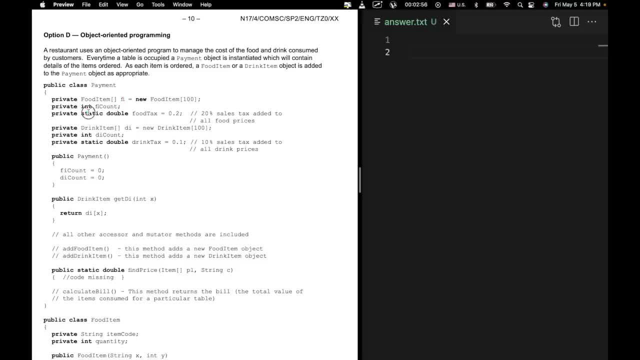 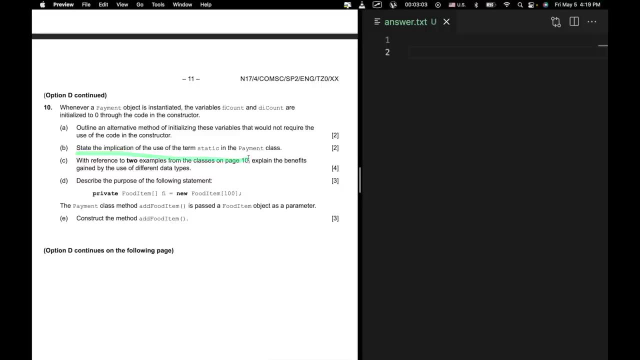 right here. But instead of doing this, we could actually just say phi count equals 0 and die count equals 0, right up here, And that would just be the answer there. Next, to state the implication of the use of the term static in the: 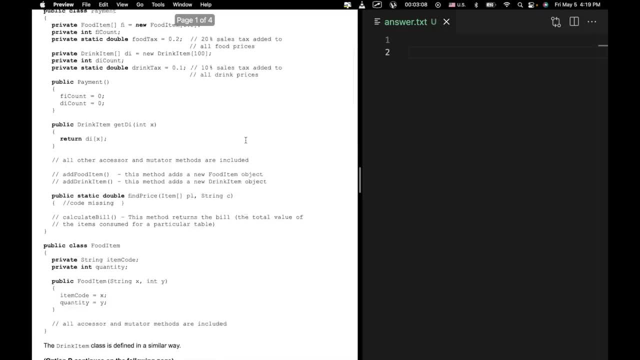 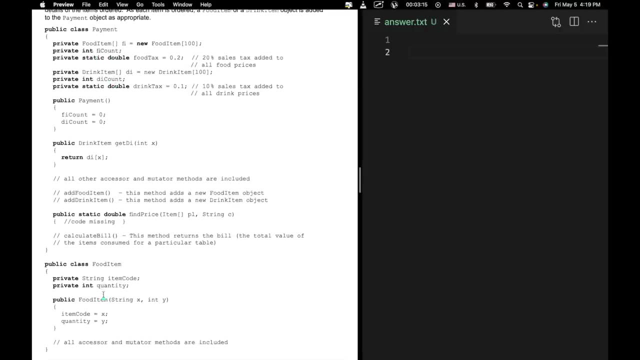 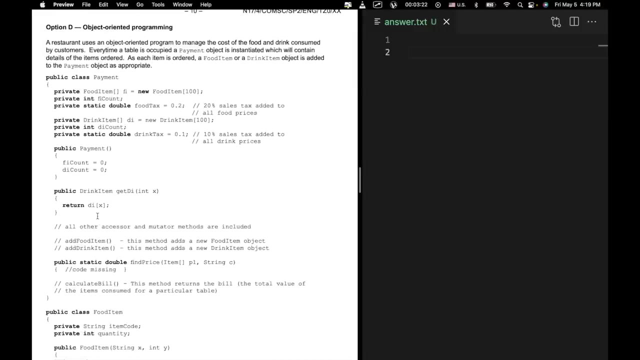 payment class. So right here we have two. we have a static attribute here for food tax and drink tax And we also have a static method right here. So that means that these values can be accessed without instantiating the payment object. So in other words, 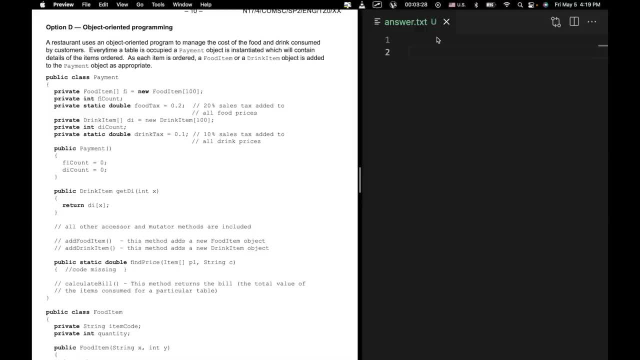 they're the same for all payment objects and they belong to the class, not the object. So in practical terms, if we wanted to access the food tax, we could just, or if we wanted to print it out, we could just do systemoutprintline. 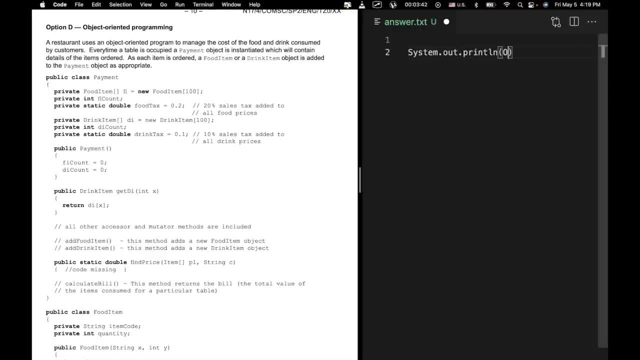 and then we could just do payment, foodtax, and that would be it. Versus for the other attributes we'd have to say payment, payment1.. We'd basically have to instantiate the class. We'd have to create an object So we can do this with a static. 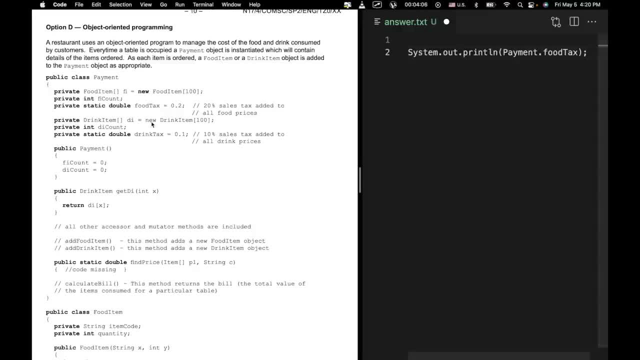 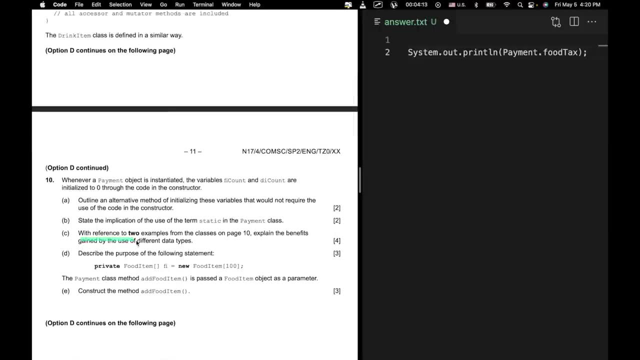 attribute or a method, and we can't do that with a regular attribute or method that's connected to the class. So, with reference to two examples from the class on page 10, explain the benefits gained by the use of different data types. So, 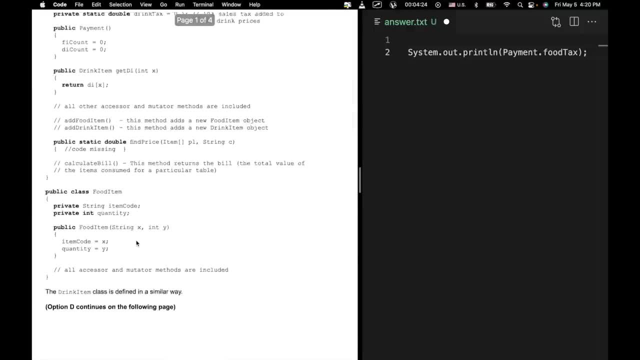 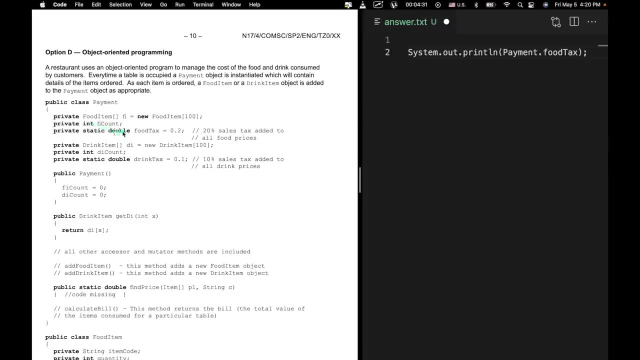 there's a couple of benefits. I would say the biggest distinction right here, the biggest ones that stand out to me, are the these values, the integer and double numerical values, Because unless we have numerical values for these, we can't really do any mathematical. 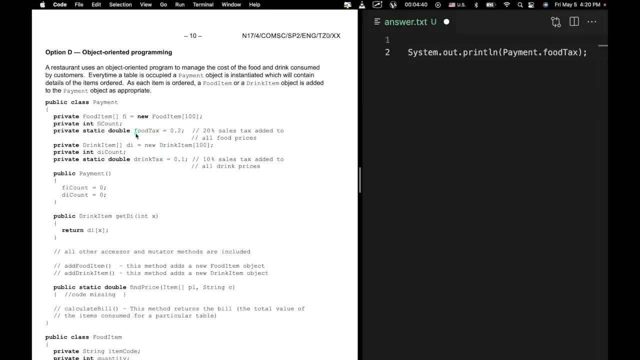 calculations with them, And that's particularly relevant to food tax, because we are going to be doing some multiplication and probably some other arithmetic with these. With phi count specifically, unless this was defined as an integer, we would not really be able to use it as a 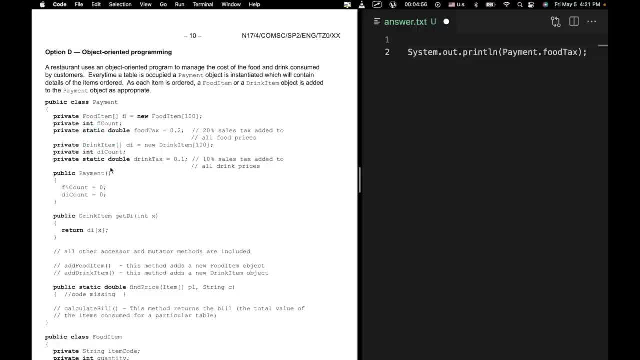 index for our arrays. Moreover, another data type right here would just be these arrays. These are basically arrays of objects, and having that allows us to attach a large number of objects of the same type to a particular class or object, And without doing that, that is simply not possible. 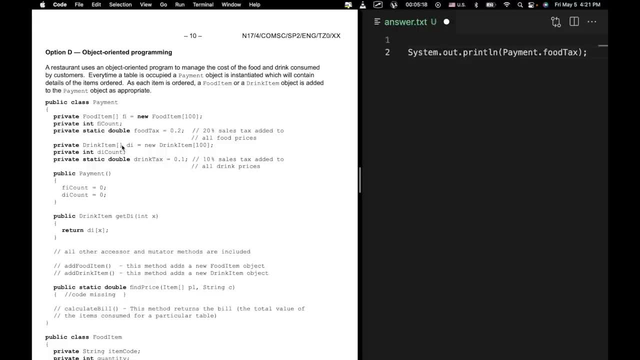 So I guess some other things we can talk about as well is that, depending on the data type that we use, we're using less memory, So an integer is going to take up less memory than a double. That can also have an impact on our program as well. 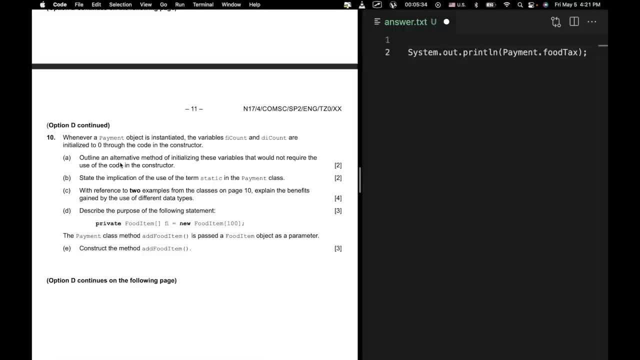 It's the amount of memory that's being used That can be a benefit. Right here it says to describe the purpose of the following statement: Private food item phi equals new food item 100.. Basically, what this is doing is initializing the array of food items. 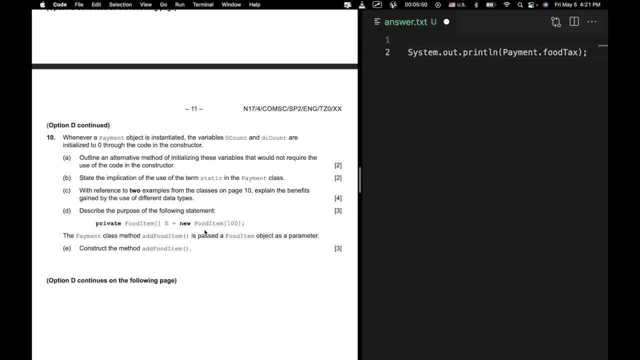 phi with a blank array with 100 items in it. That's basically what it's doing. I can't really think of any other purpose there. I guess the other aspect of this would be the private, The private accessor method right here, And all this means is that 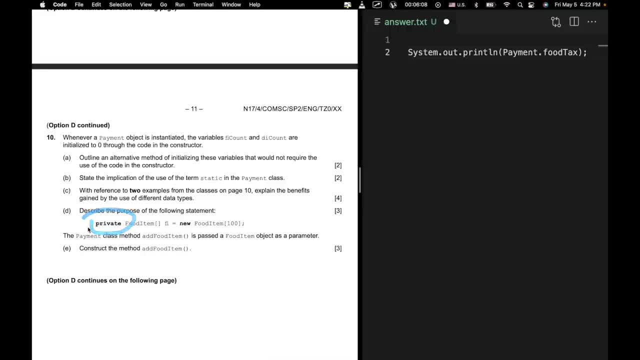 we can't access this attribute outside of an object, So we can't just do paymentphi. That's impossible And additionally it can't be accessed by any subclasses that we have of payment. So if we have any subclasses, like for example, 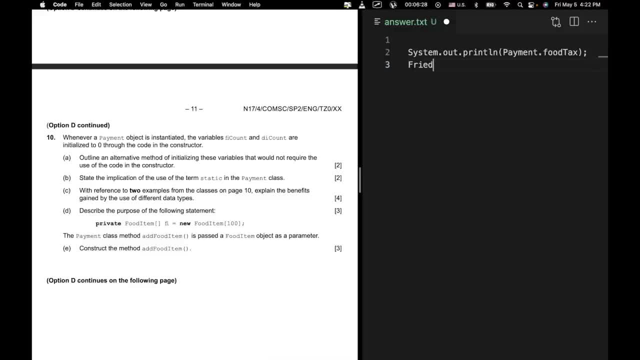 maybe we had friend payment or something like that. we wouldn't be able to access the food item array in that particular class. Right here it says the payment class method. addFoodItem is passed as a food item object, as a parameter. Construct the method. 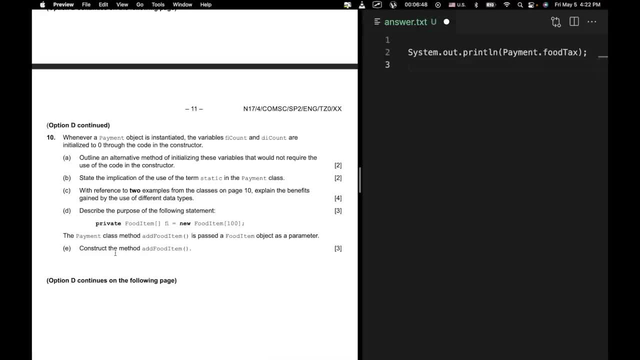 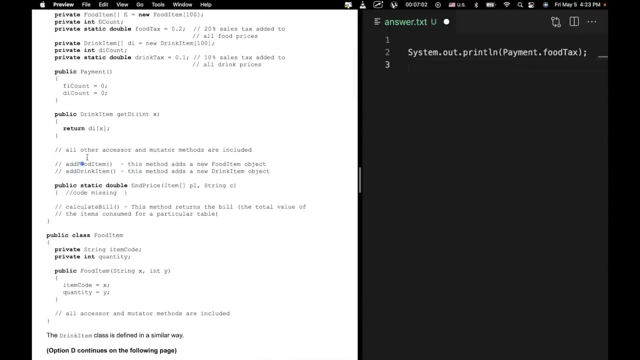 addFoodItem. Okay, so there are a couple of ways to do this. So we want to construct the method foodItem right here, Which is, I guess it was shown right up here. So we have addFoodItem. So if we want to add a new foodItem object, what we're going to do. 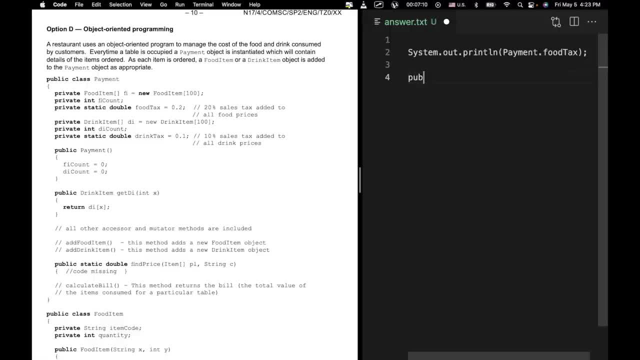 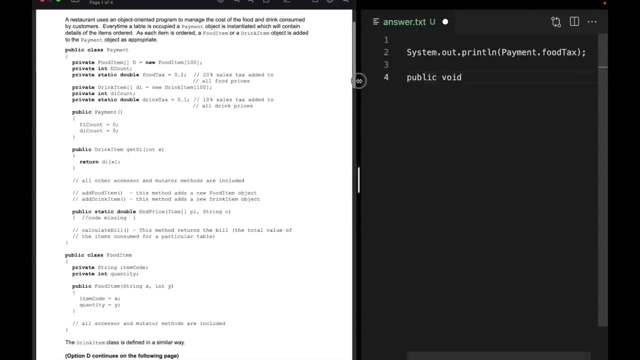 is. we're probably going to say public And it's going to be void, because we're not really returning anything. Just going to move this here a bit. We're going to say public void and then addFoodItem, obviously With a parameter of foodItem of type. 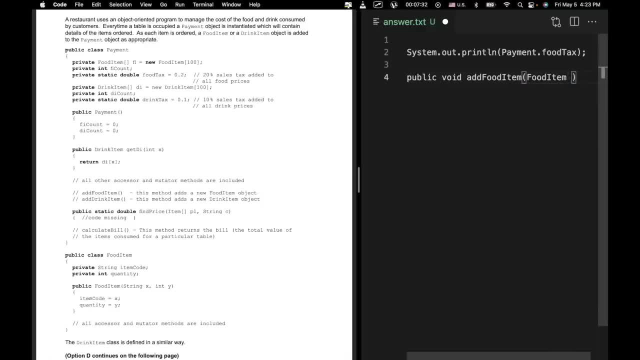 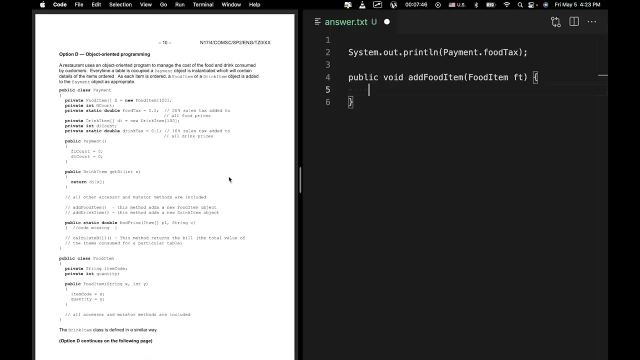 foodItem. We'll just call that ft And yeah, actually I think I will just kind of make this smaller right now. Okay, I think the way what we can use is we have this ficount, So that ficount should be. well, let's see. 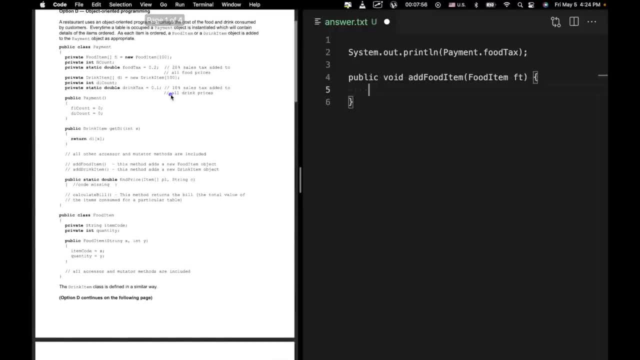 if it gives us any details about it. But the ficount should be like incremented every time we add a new foodItem, And so basically what we can do is we can say fi ficount equals ft, Because basically let's say that we add. 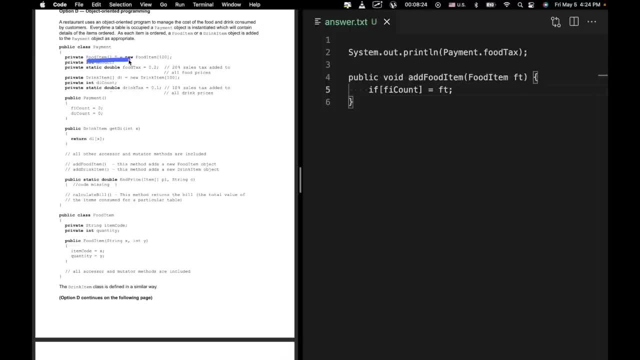 a foodItem to this particular array. That means we're going to increment ficount by one And the index zero is going to be occupied in the foodItem array, Which means that ficount, which means that fi1, is going to be available. 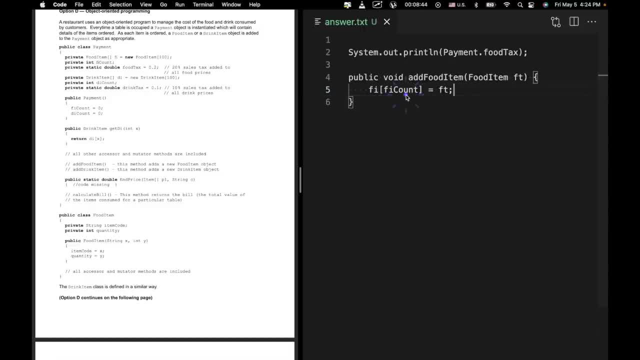 So this actually pretty much works, allows us to put the foodItem in the next available index in our array, And we also want to increment ficount once we've done that. That's how we're going to add a foodItem to our fi. 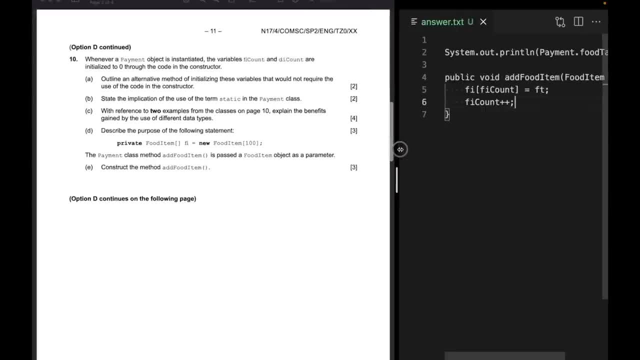 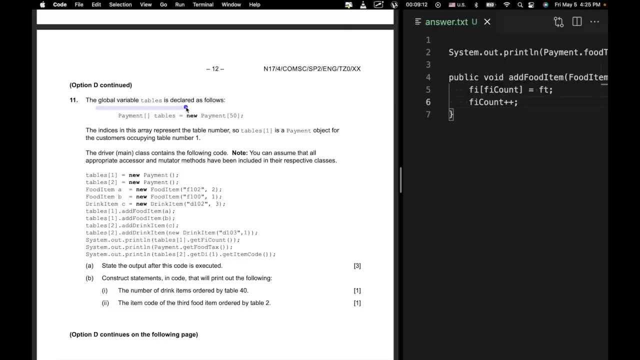 foodItem array. So that's actually the first part. That's number 10. right there, Let's move down to number 11.. So right here it says: the global variable tables is declared as follows: So you've got a payment array called tables. 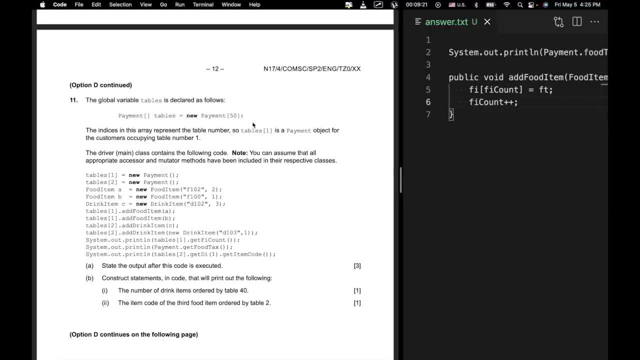 with 50, basically 50 elements in it And this is going to be a blank array And by global variable. this means this is going to be declared probably in a main method, So it's going to be declared outside of a particular class. 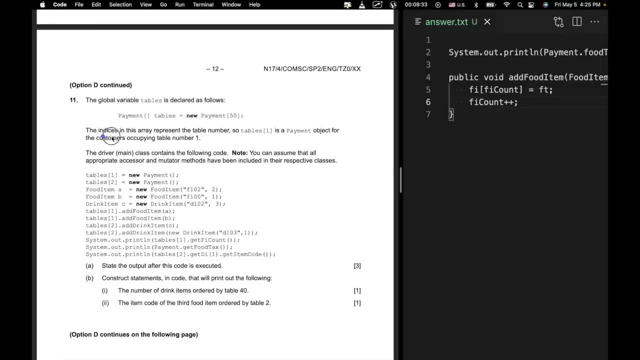 and it's just going to be there. Now. the indices in this array represent the table number, so tables1 is a payment object for the customers occupying table number 1.. Now the driver, the main class, which is what also contains this, contains the: 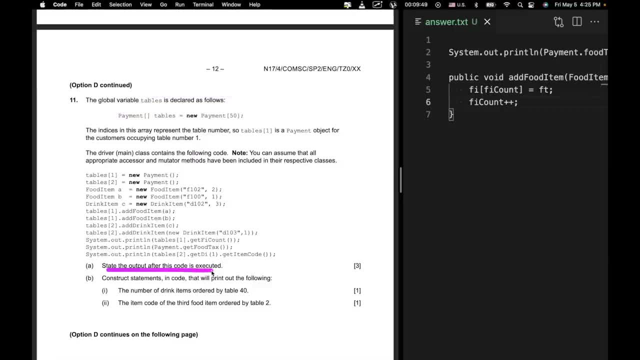 following code State the output after this code is executed: Okay, so right here, let's just walk through what this code is going to do. So we're going to have tables1 and tables2.. So we're going to have new payment objects. 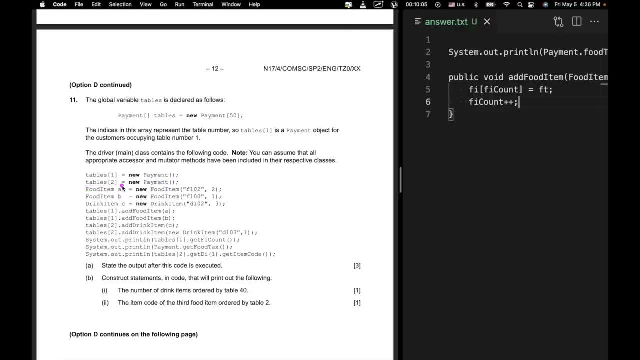 there, And then we're creating two food items right here and then one drink item. So we are adding. so basically adding these two food items to table1.. This drink item to table2.. And we're actually creating a new drink item. 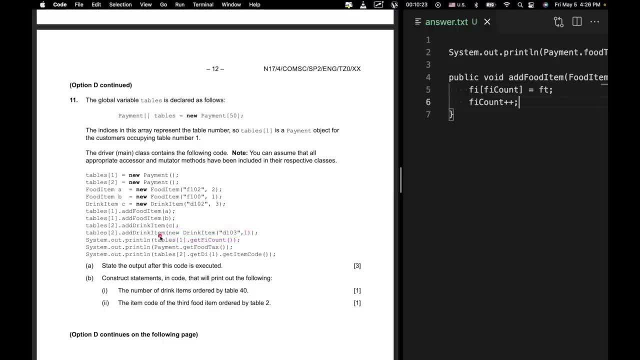 right here inside these parentheses, And then we're going to immediately add that to table2.. So table1 is going to have two food items and table2 is going to have two drink items, including this one and one just created or instantiated right here in the parentheses. 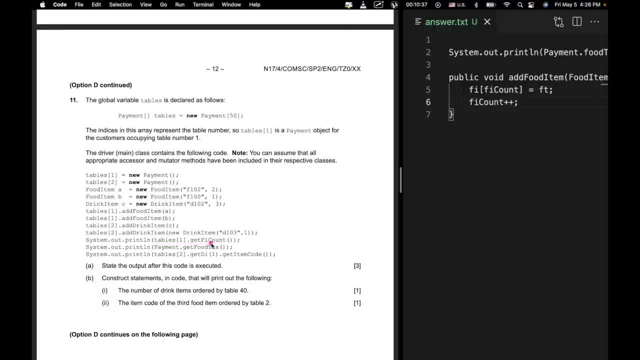 So if we do table1 dot getFiCount, we're going to have, we're going to have. so the first time we add this we'll have 1.. And the next time we add this we'll have 2.. So we should print out right here for this one. 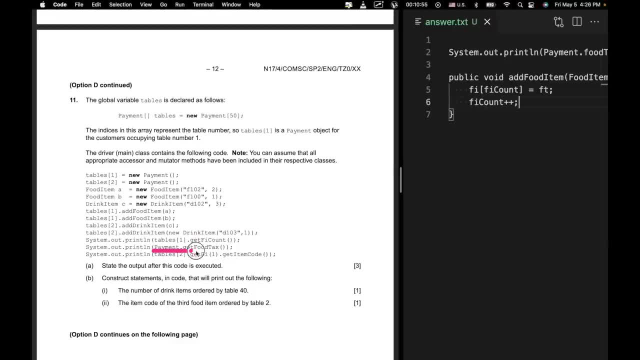 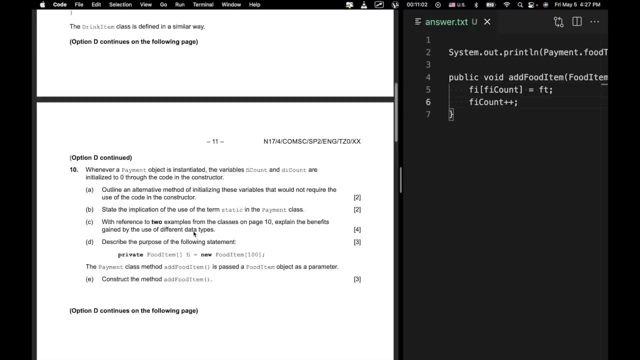 2.. And then right here it says paymentgetFoodTax. So food tax, I believe right up here, was set to .2.. So that's just going to be .2.. So we're going to have 2 for this line, or for 2 for this line, we'll have 2.. 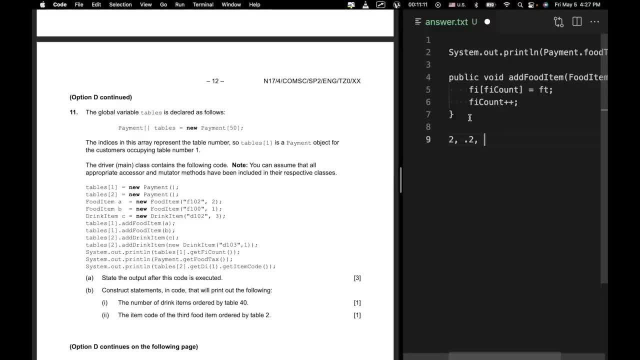 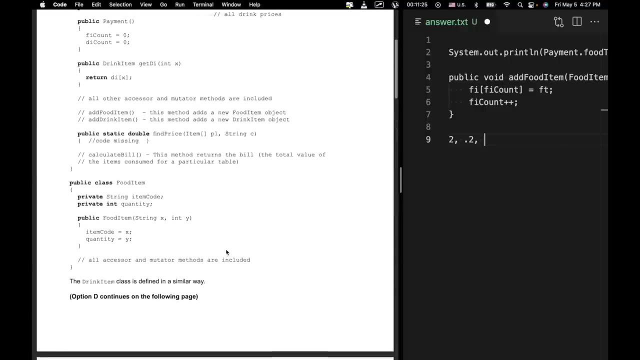 .2. And then it says right here: systemoutprintLine: tables2.getDie1- getItemCode. So if you look back up here to our getDie method and that's on tables2, getDie is going to allow an index input and then we're going to get the drinkItem at that index. 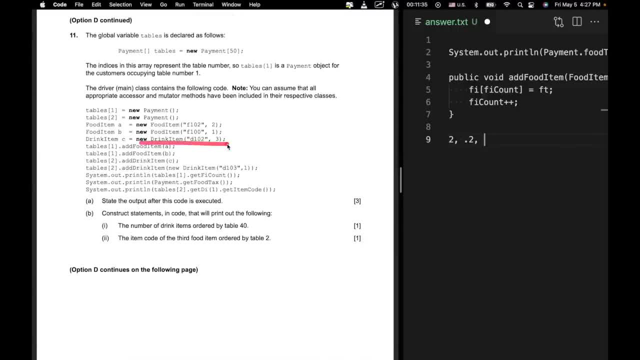 So, if you look at this right here, this drinkItem would have been at index 0 in the drinkItems array And this one right here would have been at index 1 in the drinkItems array. So, and if this one is at index 1, which is right here- 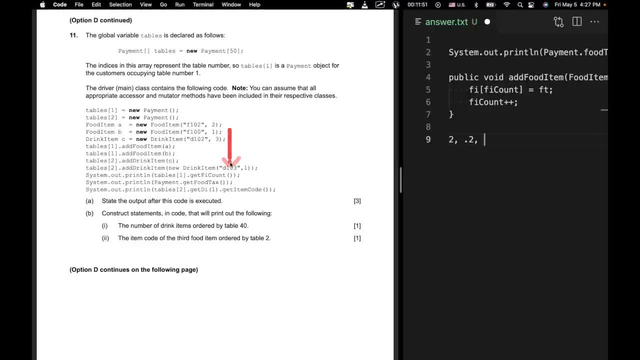 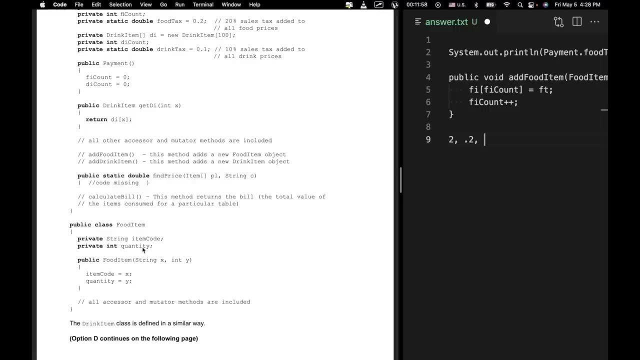 this is going to be the item code, remember, Because if we go back to that method up here, for that method, well, okay, so for that method actually. well, I guess this is foodItem but drinkItem has the same. 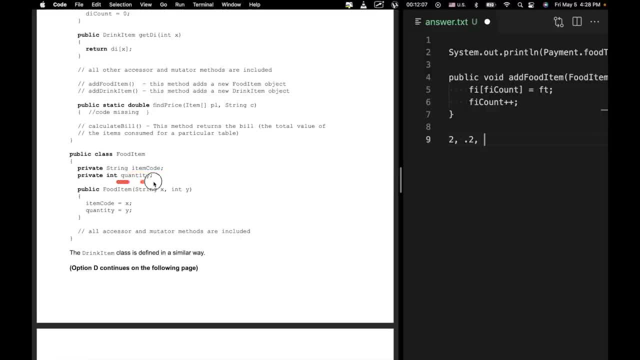 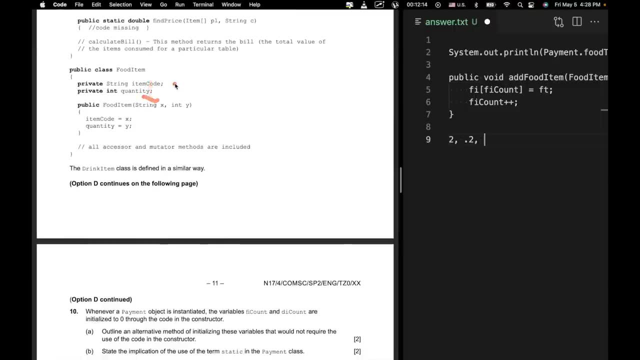 We have an attribute itemCode that we're inputting and then we have an attribute quantity that we're inputting. So the first one is going to be itemCode right here and the second one is going to be quantity right here. So that means, if we go down, 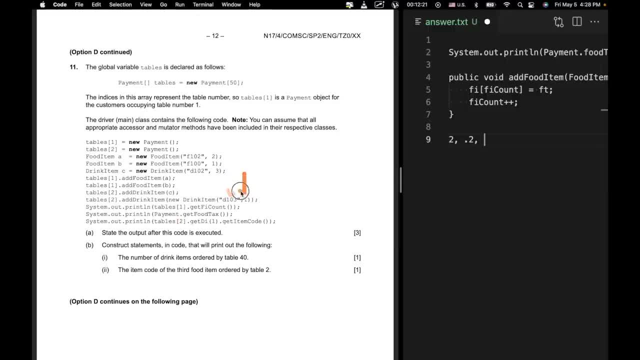 right here. this would have been the itemCode and this would have been the quantity. So if we do getItemCode on this particular item, which is at index 1, then we would just be getting D103.. So that's going to be. 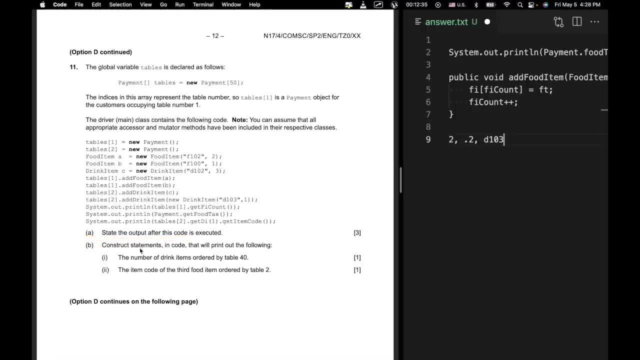 the answer to A. Now it says: construct statements in code that will print out the following: Number of drinkItems ordered by table 40, and the itemCode of the third foodItem ordered by table 2.. Alright, so if these are going to print out the following, 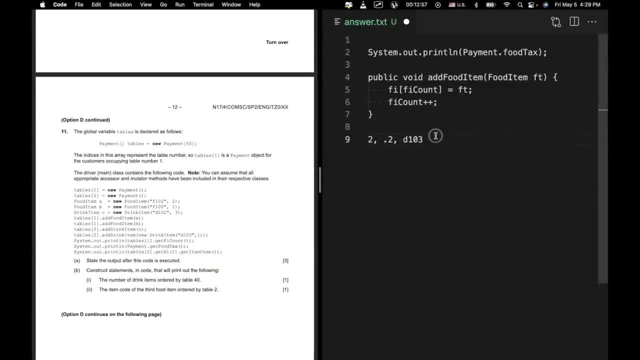 then we're going to have systemoutprintln, systemoutprintln, systemoutprintln, and we're going to have ordered by table 40.. ordered by table 40.. So right here it says that tables1 is for customers occupying table 1.. So for table 40,, 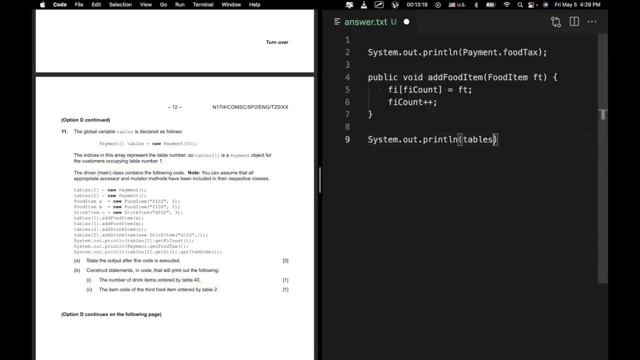 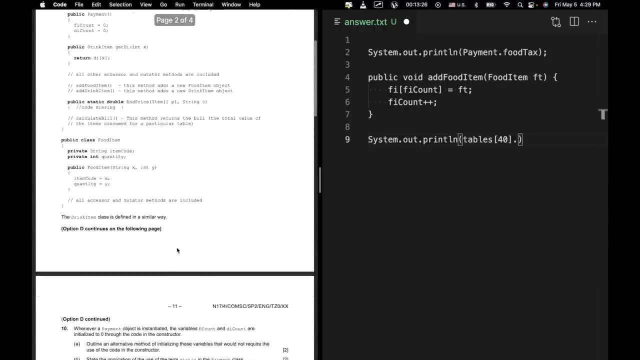 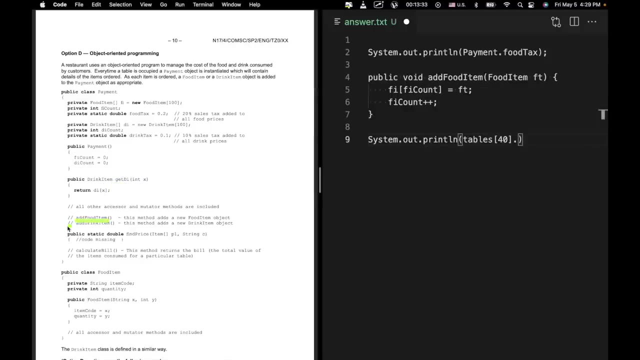 that means we're going to have tables 40. We want to get the number of drinks. If we go back up here, we had a getDie, So this is getting a specific drink And we have addFoodItem and addDrinkItem. 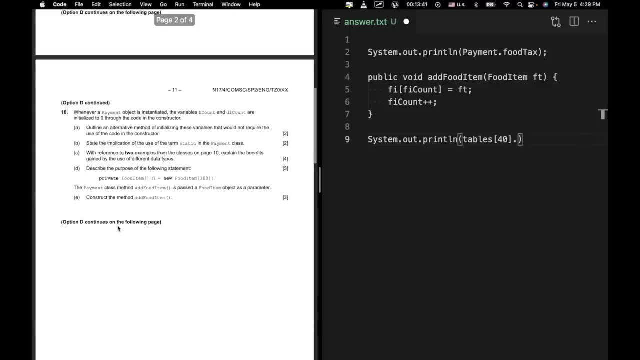 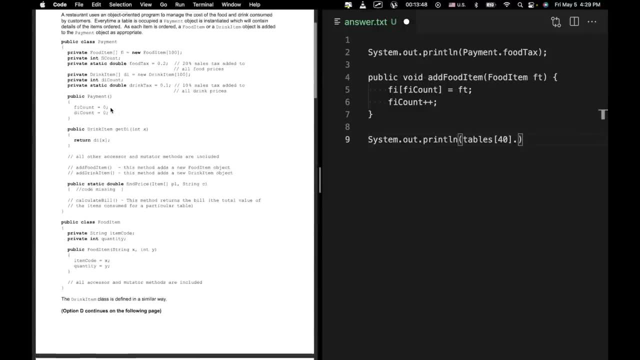 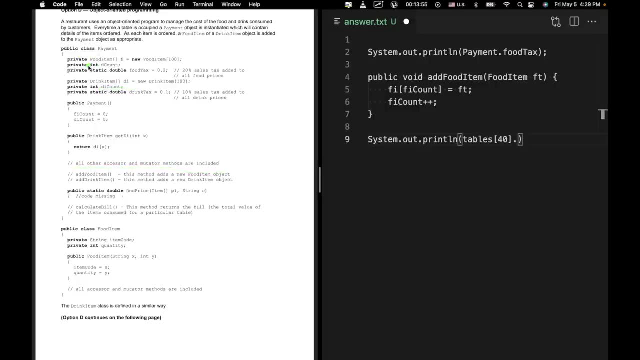 And if we want to get the number so right here- it said the number of drinkItems- that means that we probably want to get the dieCount right here- And if we have all of their accessor and mutator methods- and this is private- 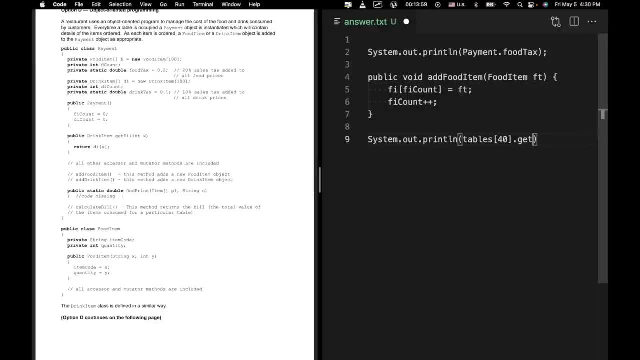 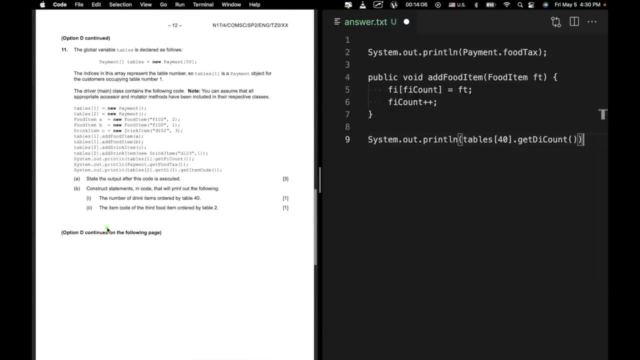 that means we're probably going to have a getDieCount method that's going to allow us to do that. So that's going to be the answer to that one. Now, right here it says the item code. We want to get the item code of the third. 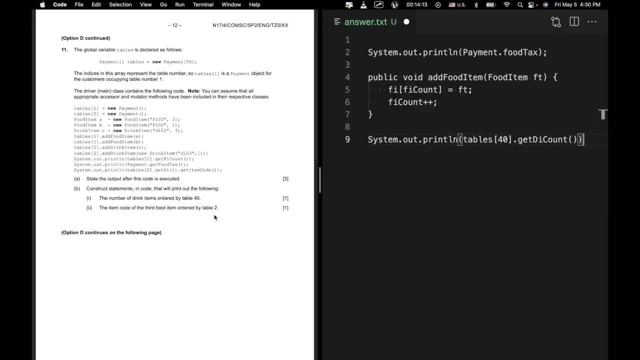 food item ordered by table 2.. So if we want to get the third food item ordered by table 2, that means that we're going to do systemoutprintln, systemoutprintln, We're going to go to tables2.. I'm actually going to put this right down here. 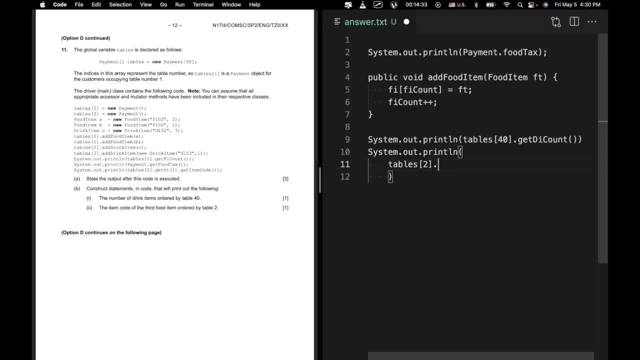 just so it's easier to see And we're going to. so if that's the third, so we want to get that third food item. So if we have to, so in order to get food items, we need to do as we saw. 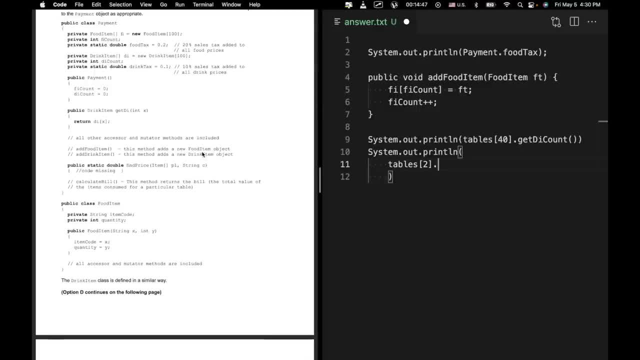 right up here. we're going to have a. we're going to have, if we have an addFoodItem, we're going to have a getFoodItem and addDrinkItem class Or addFoodItem and getDrinkItems method, rather. 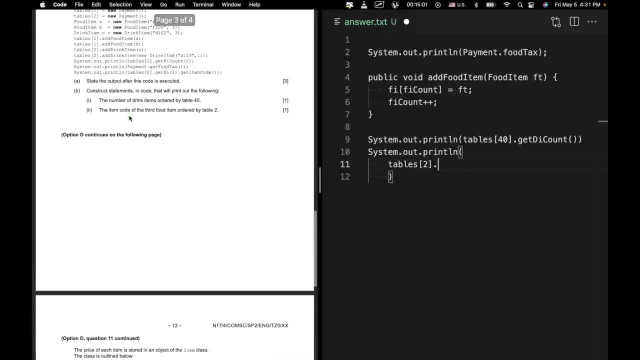 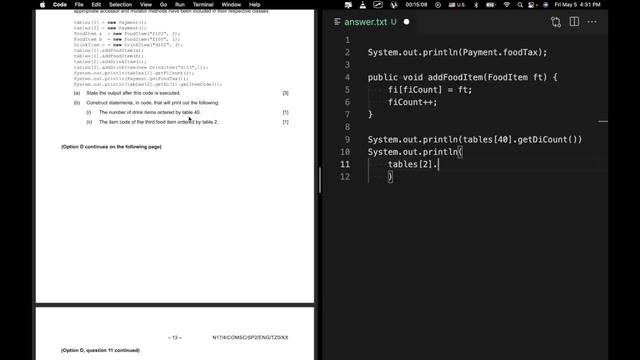 However, we're talking about the third item, right? So the third food item. so that means the index. it's going to be an index of 2 in the food items array, So we can do tables2, and then similar to getDie. 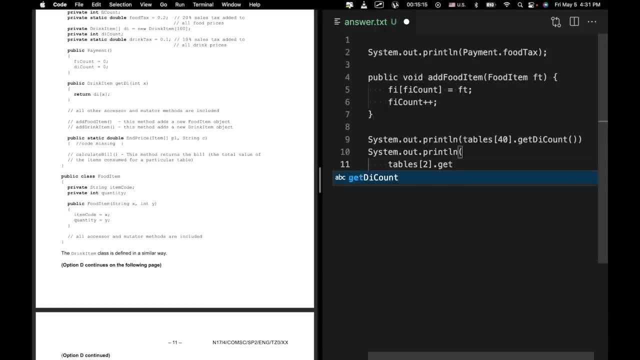 right here. we're probably going to have a getFi index2 and then we want to. if we getFi, that means we're going to get a food item and we want to get the item code, so it's going to be getItemCode. 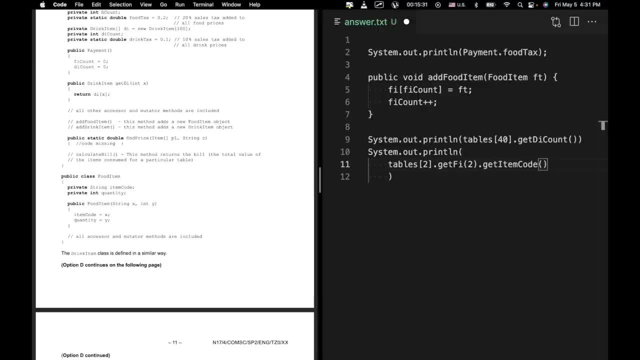 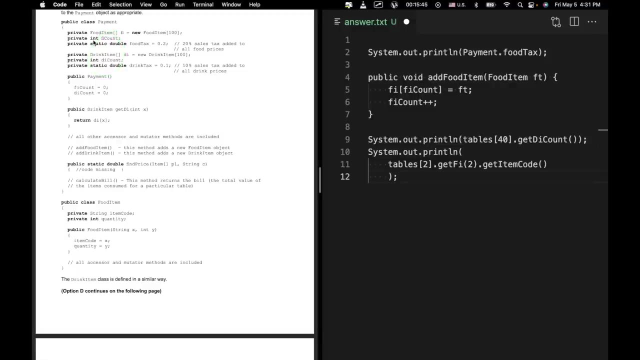 Now I just want to point out to the fact that there is a lot of assumptions here about what methods are here and what aren't, If you have variables, if you have any of these variable attributes except for the static ones. sorry, I can't talk today. 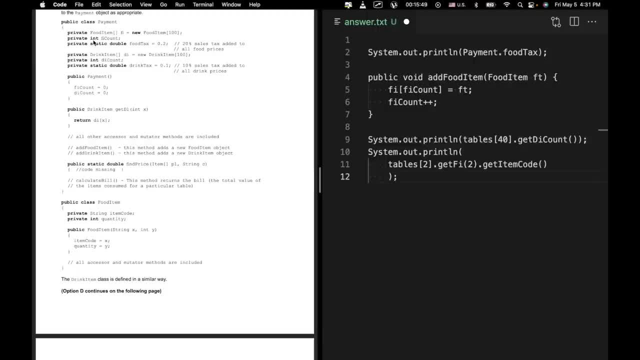 except for the static ones. then you're going to have a get and set method for those, and if you've got any methods right here with arrays, you're going to have an add method to add an object to them and you're going to have a get method. 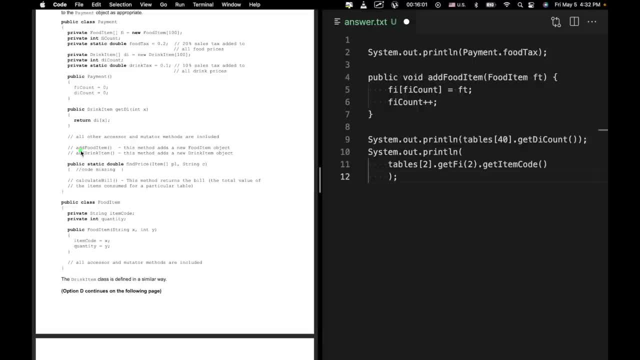 to get, probably get a specific item from them. In this case it's getDie or getFi. but you're going to have both of those things, either to get all of them or to get the item in a particular index. So you can just kind of assume that. when it says: 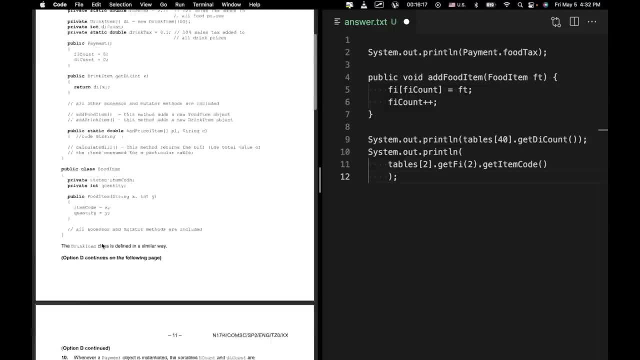 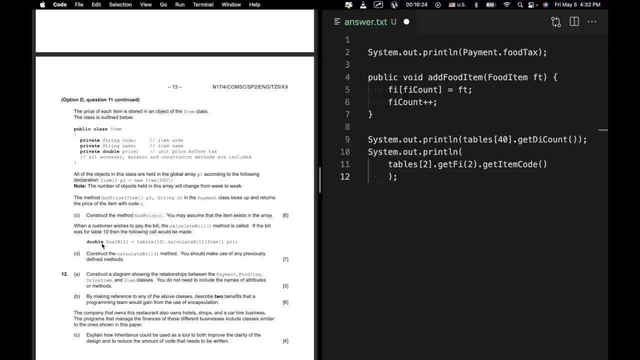 all their accessor and mutator methods are included. I know that might be confusing, but that's kind of how it works. Okay, so this is still question 11. So it says the price of each item is stored in an object of the item class. Now, if you don't remember the item class, 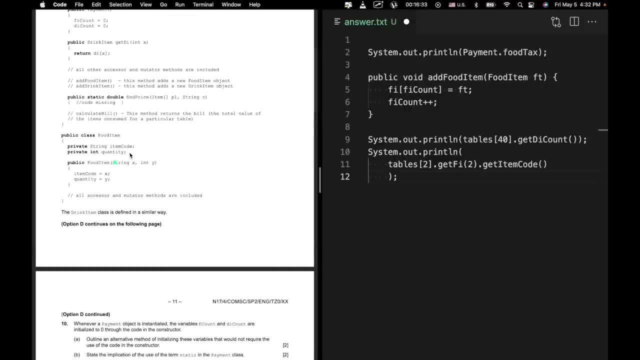 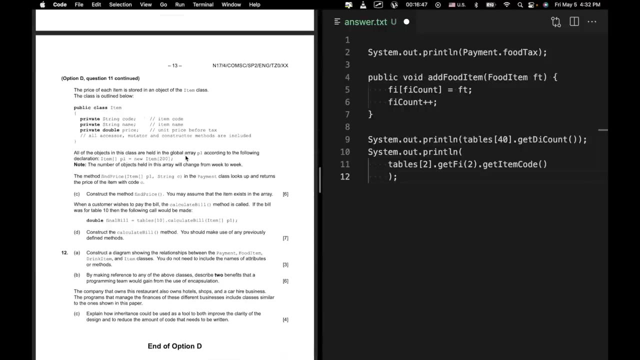 that was right here on this static method, right here. So we had findPrice item, we had an item array called pl and a string c and we didn't really know what that was, but I guess we're going to find out now. So right here it says: 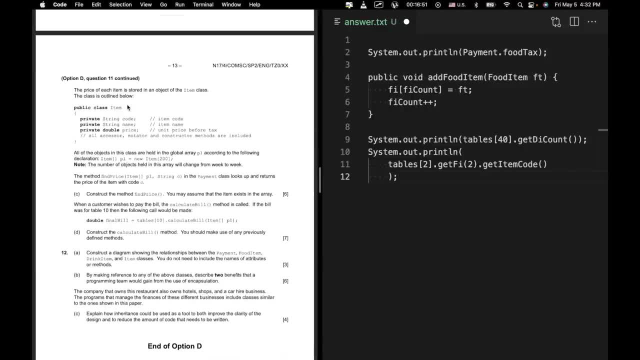 the price of each item is stored in an object of the item class. The class is outlined below. We have public class item and on that we've got three attributes. We've got string, we've got code name and price, two of which are strings. 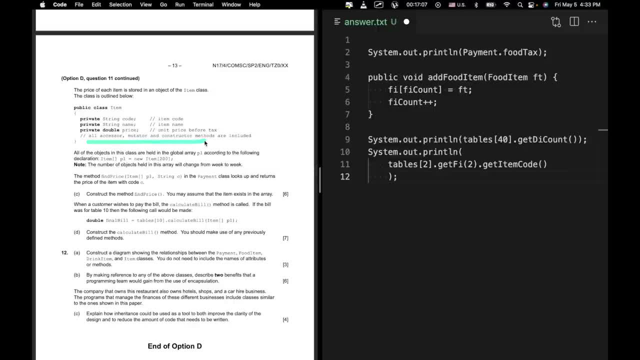 and one of which is the price. All of the accessor, mutator and constructor methods are included. I assume the constructor methods are initializing all of these. So it says all the objects in the class are held in the global array pl. according to the following declaration, item pl equals: 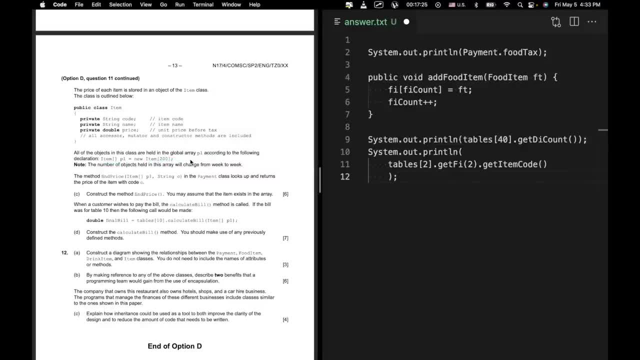 new item 200, which means we've got an array potentially with 200 elements. The number of objects held in this array will change from week to week. The method findPrice, item pl, string c in the payment class looks up and returns the price of the item with code c. 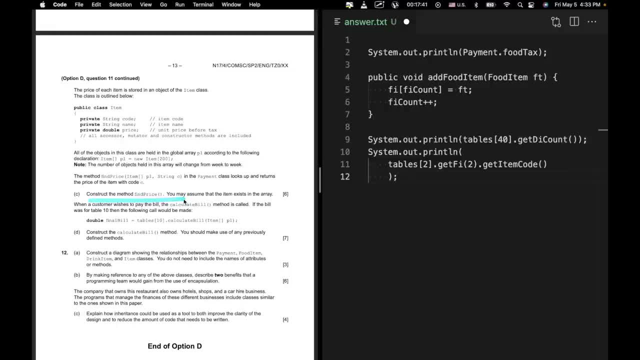 Construct the method findPrice. you may assume that the item exists in the array. Alright, so basically, what we're going to do is we're going to start with the method definition, So we're going to have basically returning a price and that the price right here is known to be double. 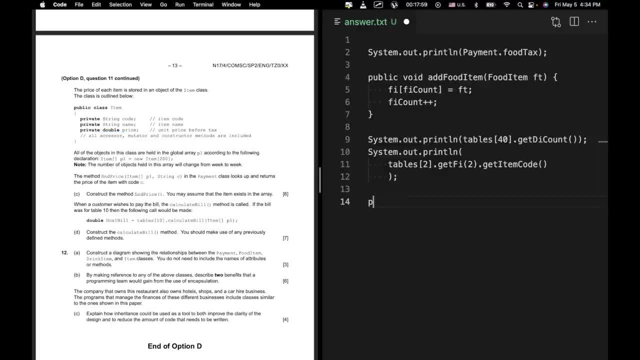 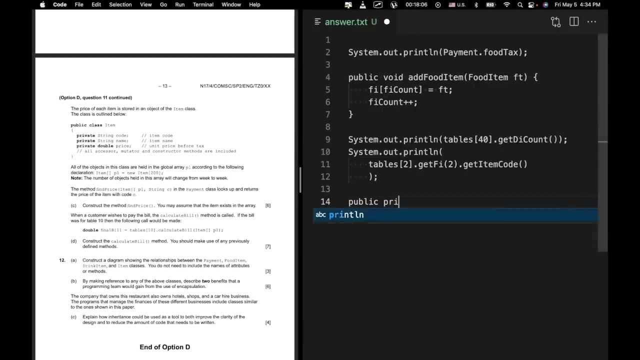 So we can say public- I'm just going to go ahead and make this a bit smaller here- price: public, double findPrice, item p, string c: That's going to be our method definition, Alright. And now we want to go through this array and we want to find the particular. 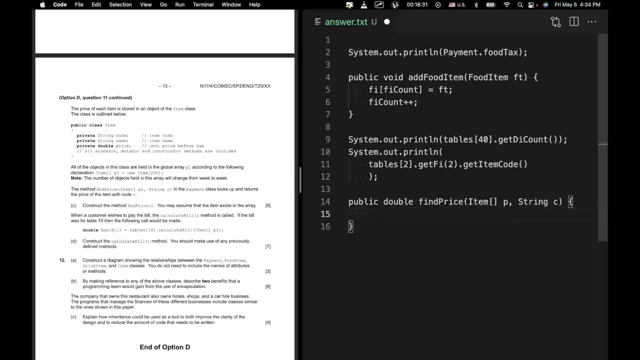 item that matches the item code. So what we can do is we can say 4 i equals 0 i is less than p dot length i plus plus. That's going to be our loop right there, initializing 0 and then continuing until we get to the 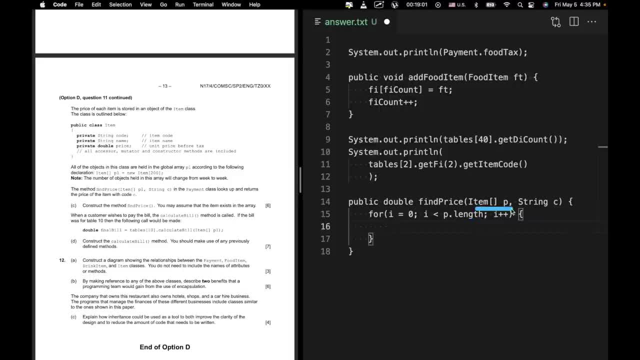 right before, until we get to the length of the array. if p i dot get, let's say it's probably going to be get code, get code equals c, c, then we're just going to go ahead and I think we're going to return p i dot. 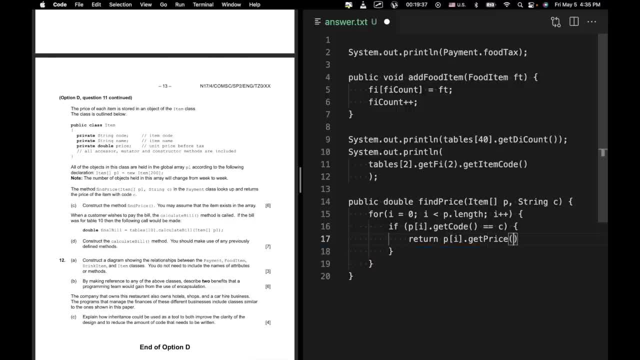 get price and we can do return, because as soon as we find it we want to return that value and we don't really need to do, we don't really want to get anything else. when we do this return right here it will. it will end the execution of the function. 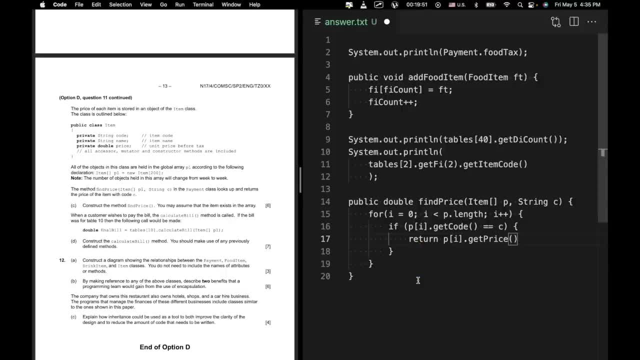 so basically, exit is out of the function, so that's that's probably a good way to do it. there's obviously other ways to to do this. let's see if there's any other particular. okay. it says the number of objects held in this array will change from week to week. 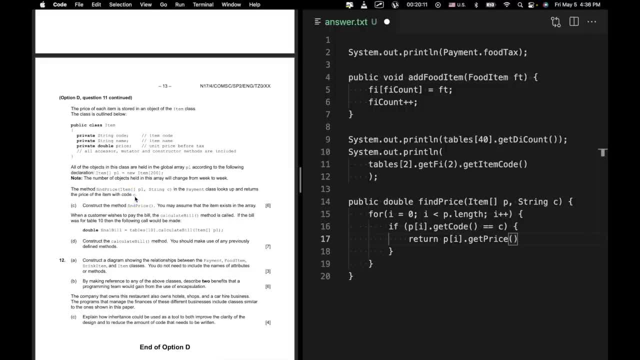 looks up and returns the price. now there are a few other things that we could do if we really wanted to. I mean, if so, if you wanted to do this, if you wanted to check all 200 entries, then we could do that. we could just say, well, yeah, if you want to check through all, 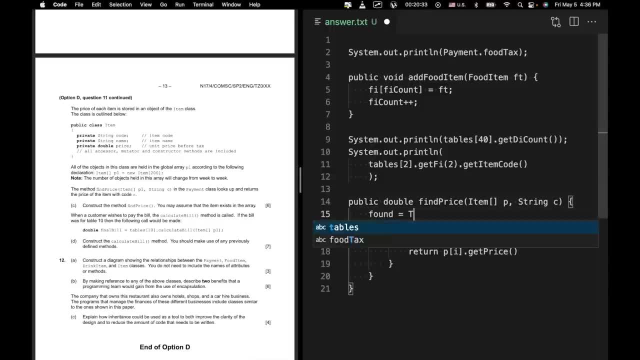 200, we would just say: found equals true and price equals zero, and then we could just do: price equals p of i dot get price, and then after the for loop we would just return price. so it's another. it's another variation that I just mentioned, because in the mark scheme, for some reason, 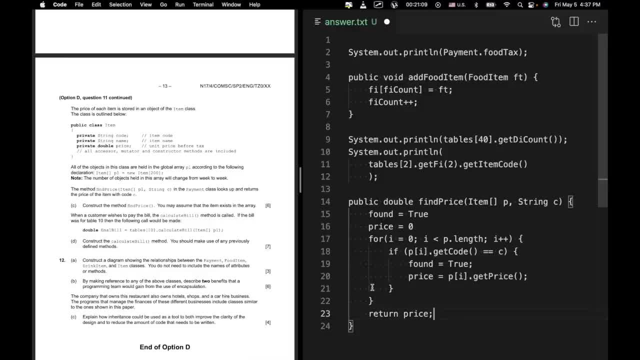 it's it to check all 200 items, but either one- I mean like they're both- they both accomplish the task okay. so let's kind of let's go back to the exam and let's move on. I'm gonna zoom in a little bit right there. 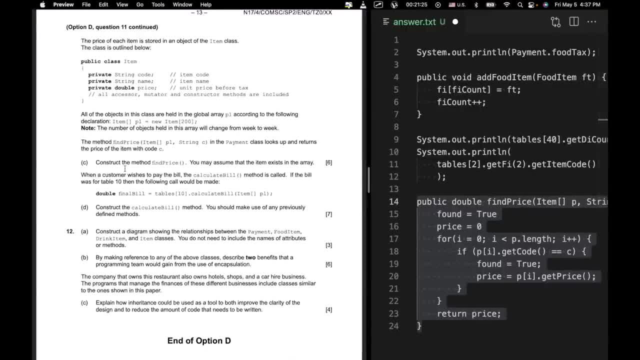 okay, so we constructed the find price method. now it says when a customer wishes to pay the bill, the calculate bill method is called. if the bill was for table 10, then the following call would be made: so table is 10 dot. calculate bill, item pl. so this global like item. 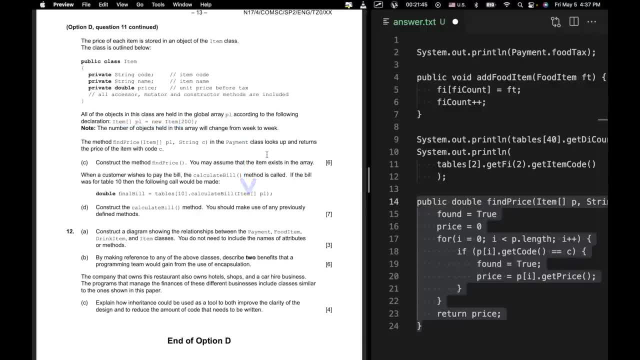 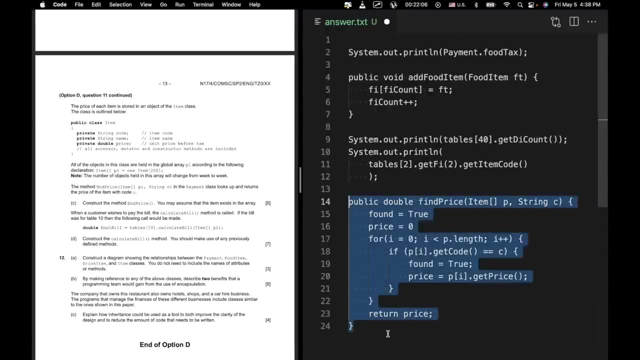 array is going to be put in here so that we can get the prices of whatever items that the particular table has ordered, and so we need to calculate, or we need to construct the calculate bill method. so let's go ahead and let's do that, and we're going to start by creating the method. 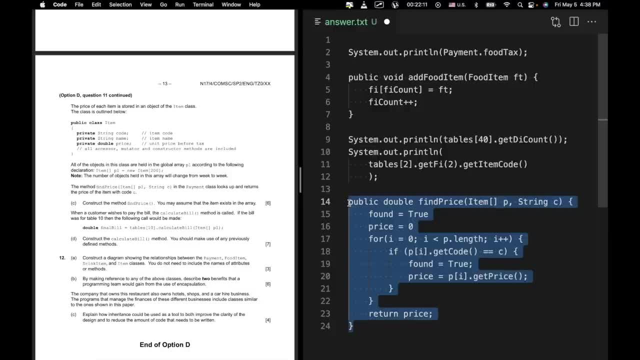 definition. we're going to say calculate bill- well, look, so we're going to be returning a double, something of double data type. so we're going to say public double, calculate bill, and then item pl, and this is going to be on a on this particular class, right here. so we're going to go right back up here. 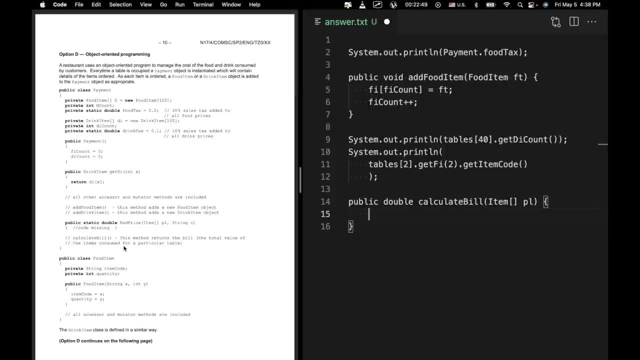 so right here we have calculate bill and okay, so we're also going to have access to all of these different methods right here. so there's a few things that i think i want to do. what i want to do is i want to go through every single food item. 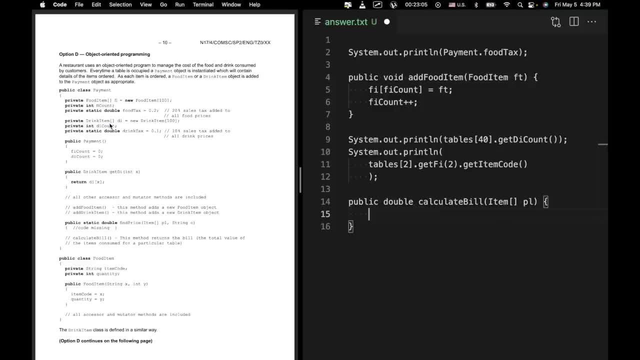 and every single drink item. so i'm going to say four, i'm going to create two loops. i'm going to say four, i equals zero, i is less than phi dot length, i plus plus, plus um, and i'm going to go, i'm just going to get every single. 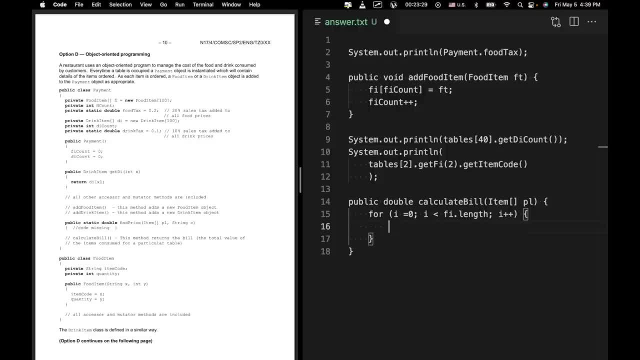 item. so i'm going to say, um, okay, how do i want to do this? so, right here, let's see what else do we have right here, okay, so every food item has an item code and i think we want to use that item code in our, in our. well, obviously, we're going to use that in. 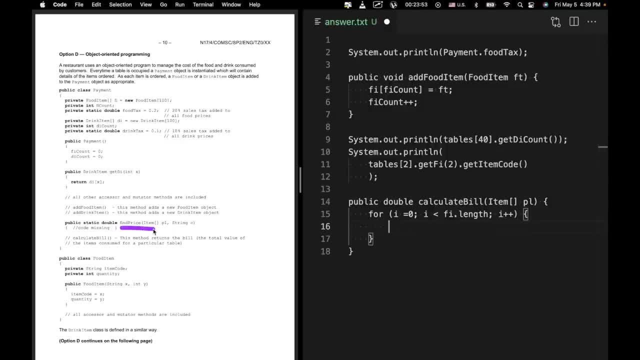 a particular method, um, but also one thing to keep keep in mind is we're going to have access to our find price method, so actually i'm going to copy paste this. i'm going to make sure that we still have that um, and it may not be completely. 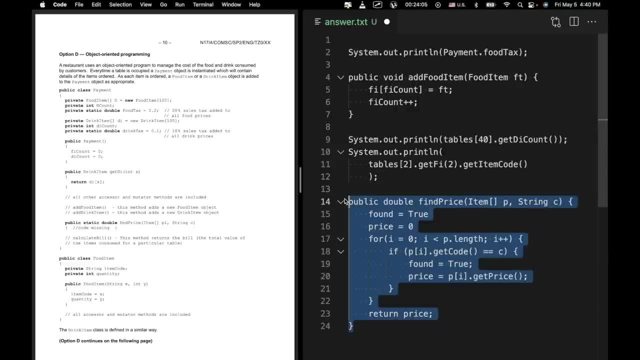 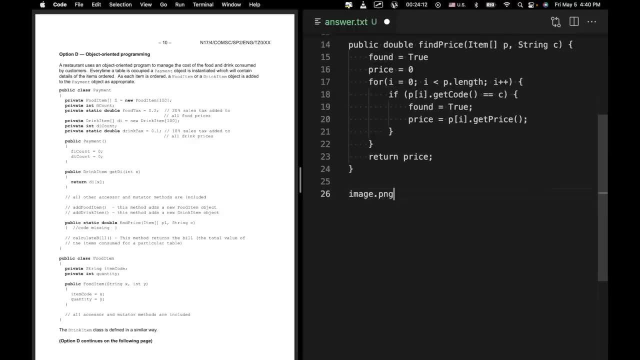 clear, but any of these questions, if you have previously written a different method, then you can actually make use of that in subsequent questions. so we're going to leave that right up there. then we're going to paste what we have, um, and i guess i need to rewrite that. 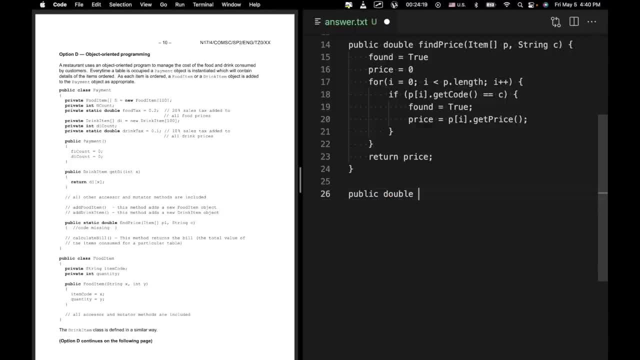 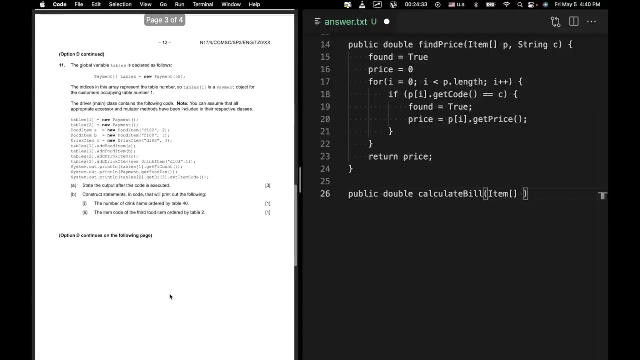 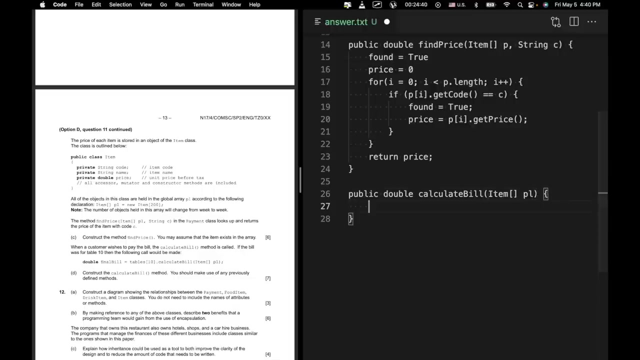 so we're going to do public double. let's see, calculate or find: yeah, calculate bill. then we had item uh c. let's go down here make sure that's what it was, or it might have been item p, item pl. let's go back to creating our array. we'll say for: 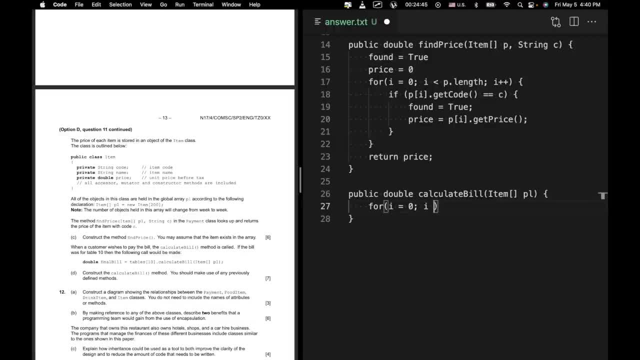 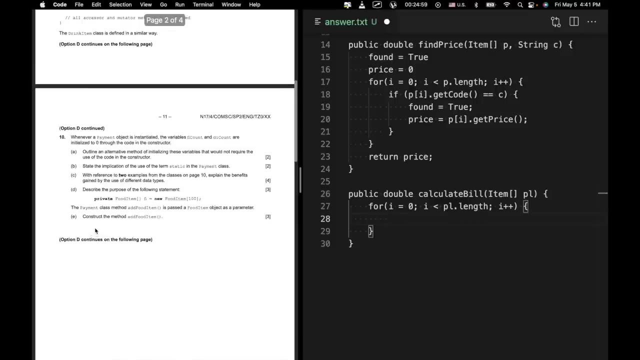 i equals zero, uh i is less than uh pllength, and i plus plus. and then we're going to go and we're going to say: let's see, we have a food item tax as well. we take into account, um, but we'll go back right up here and we 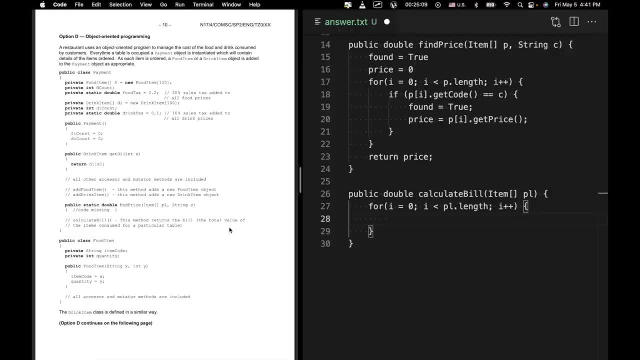 will start? we will start by getting the prices of all of the different items. so i'm going to create- i want to say like okay, well, right, i'm going to create a methods like double food. we'll say food total equals zero. okay, and we're going to do for each of these. 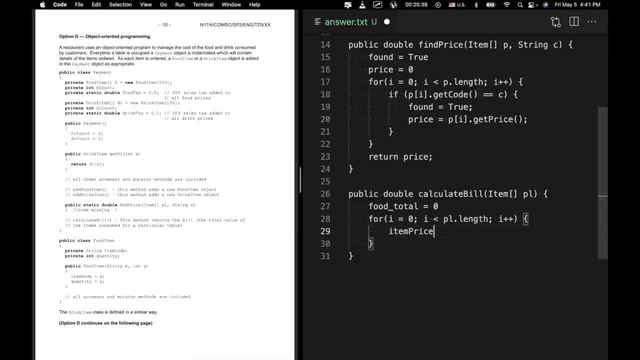 we're going to say item price equals. well, we want to get the item code first, right. so for each, for each one of the food items right here, we're going to say item code uh equals. we're going to have phi. i dot get item code because 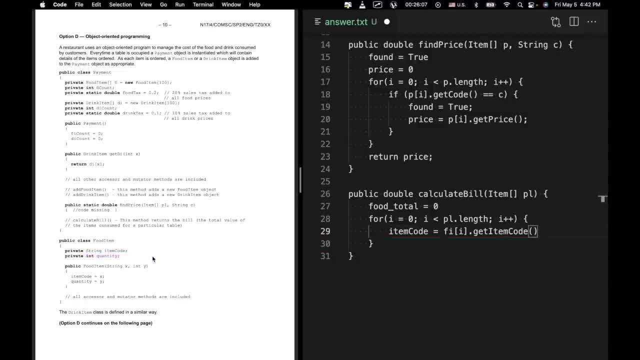 that's going to be the accessor that corresponds to this particular object. and then we're going to use um, find, we're going to say, uh, price, item price. we'll just say food. i'm just going to make this clear because we're going to do this. 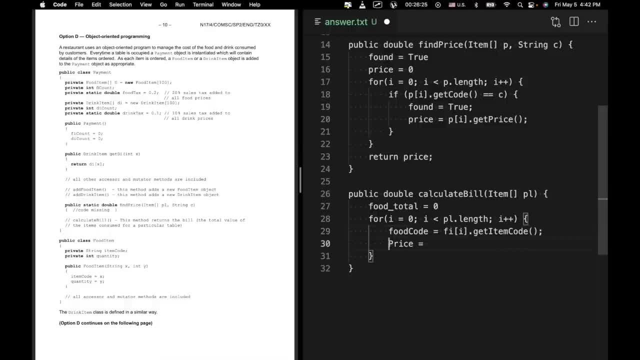 with drinks too. so we'll say: food code, uh, food price equals, because we've gotten the item code. so then we can use our find price right here and that's going to return our price. so we can say: um, find price, uh, pl, and then food code. 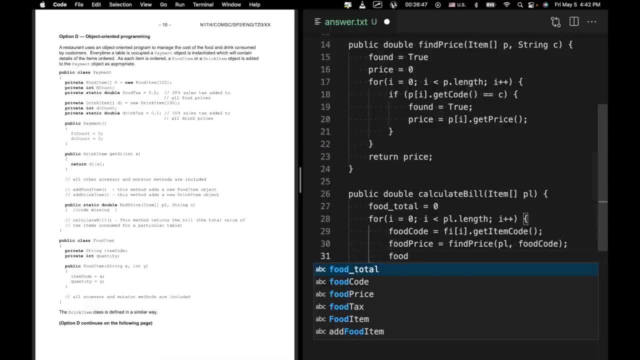 and then we're going to say, uh, food total, um equals food price times one plus our food tax. because you want to increase the value of each one by 0.2, so we'll say one plus, uh, food tax. okay, so, so far, so good. well, okay, we want to do food. 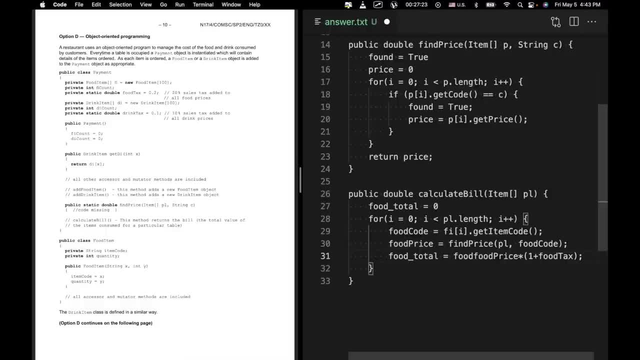 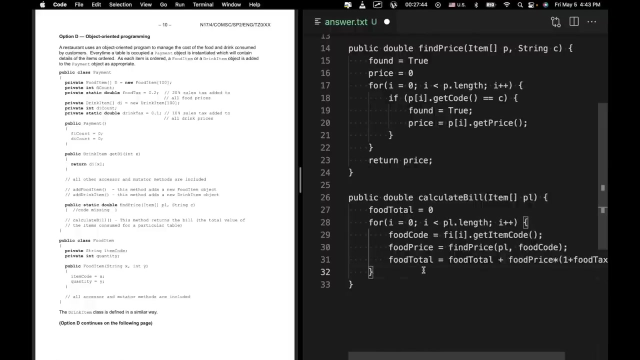 food total because we want to add our existing total. actually, i'm going to write that with the correct um camel case notation: equals food total. there we go, okay, so we can do that, and then we can do the exact same thing, basically for um. well, although this shouldn't be pllength. 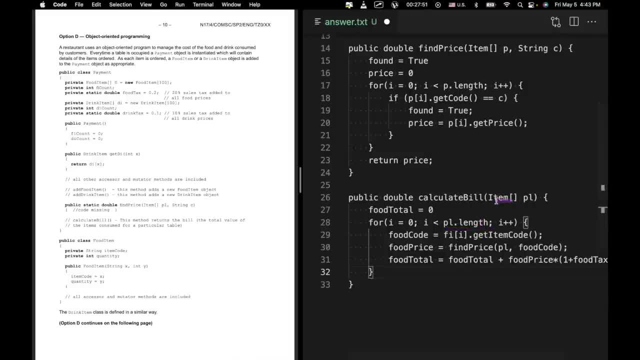 right here. that's a mistake, because pl corresponds to items. so i think this is actually just going to be phi count, or we could even do, we could do philength, but we'll just do phi count because we've already got that from right here. and now what we're going to do. 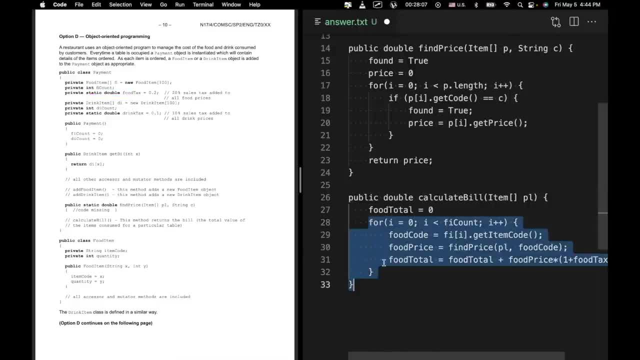 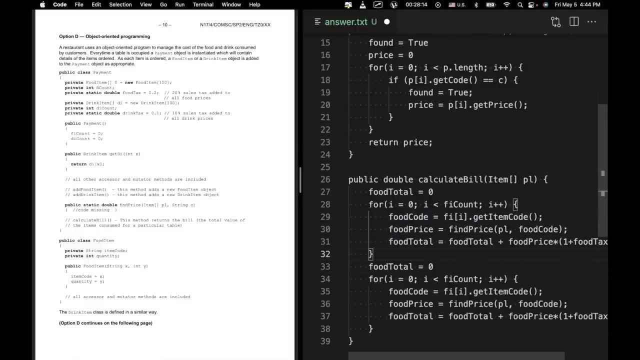 is we're going to go. i'm just going to copy this: like this isn't good programming practice really, but like then there's a better way to do this that uses less code, but for just for keeping things simple, because the process is the same for both of them. 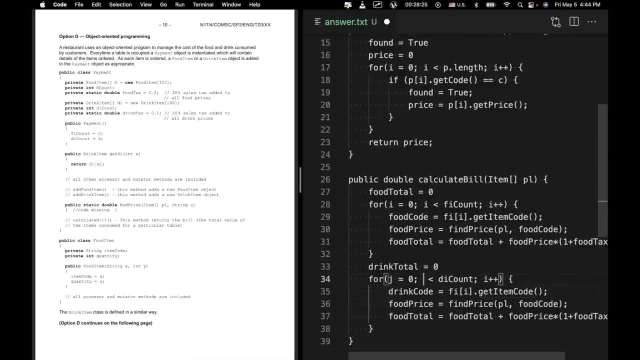 um, and i don't even really need to change the names of these because of scoping like this i only exists within this block of code and this j only exists within this block of code. but we'll just do it just to keep things clear. get die. 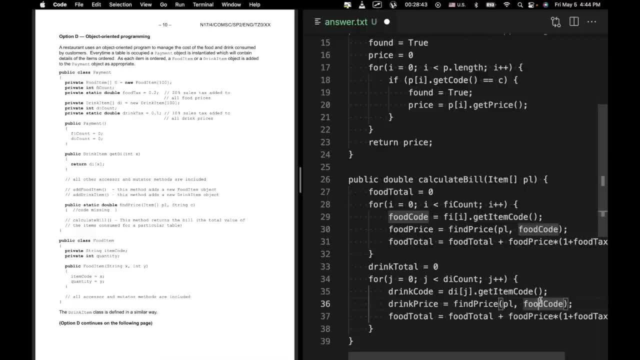 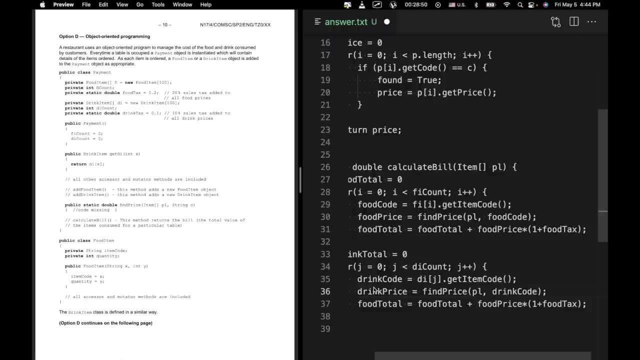 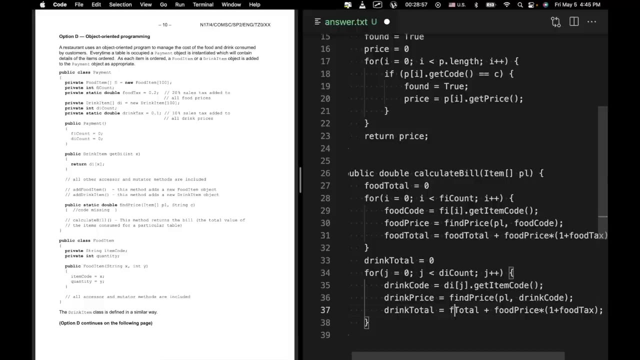 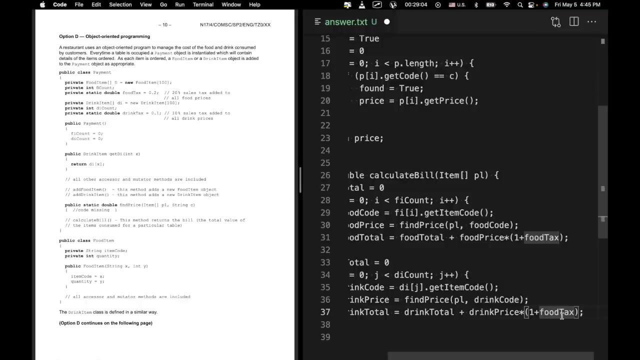 drink price: uh, drink code, and i'll just move this over to steam a little bit and then we're going to change this to drink total: uh, drink total plus drink price for that particular item: times one plus drink tax, because drink tax is different. drink tax is only 0.1. 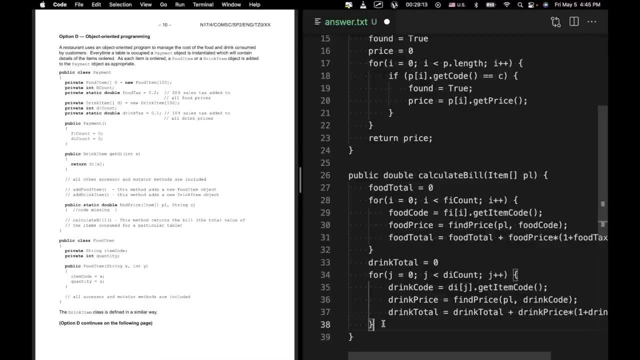 and then we can say that the total- uh, okay, i guess i made a mistake right here. um, so right here i forgot to leave out the quantity. so each of these right here is going to have a. it's going to have a specific quantity, so it's not just going to be one of those items. 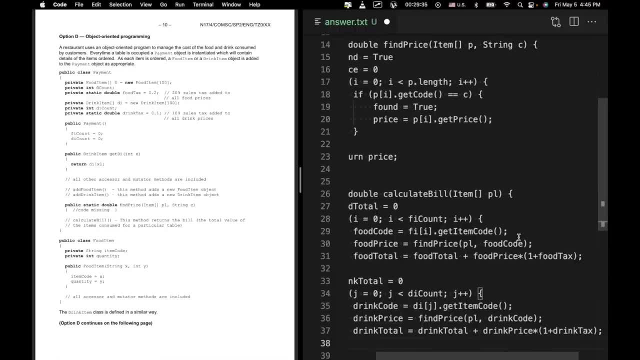 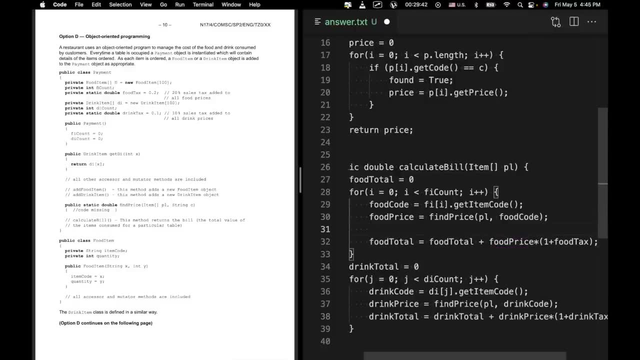 it's going to be how many ever um of those items there are. so just food price isn't enough. um, i guess we can say uh food total. now we already have food total um food order. uh total equals food price. uh times um times food times. f i, i. 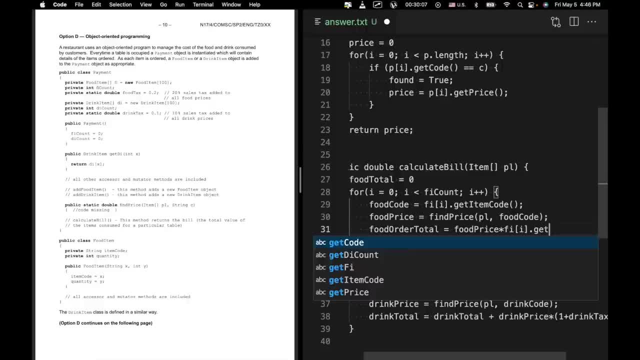 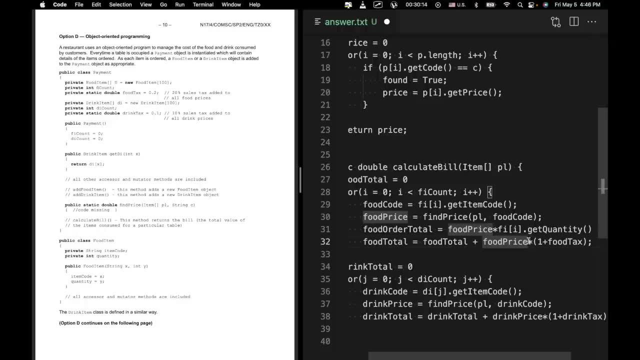 dot get quantity and then we will have food order total right here, because each food item it could have multiple. it sounds really unintuitive. actually, now that i think about it, it have multiple things associated with it. um, so for example, you might order three beers and then three vodkas and then 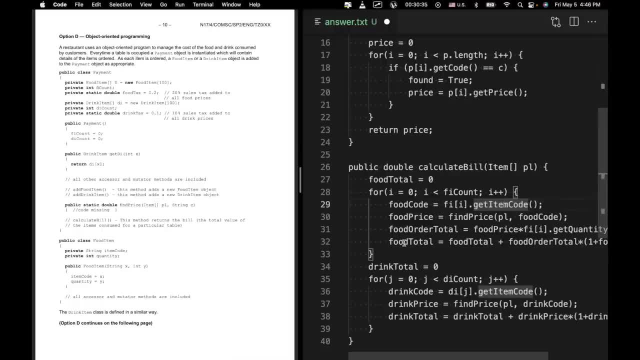 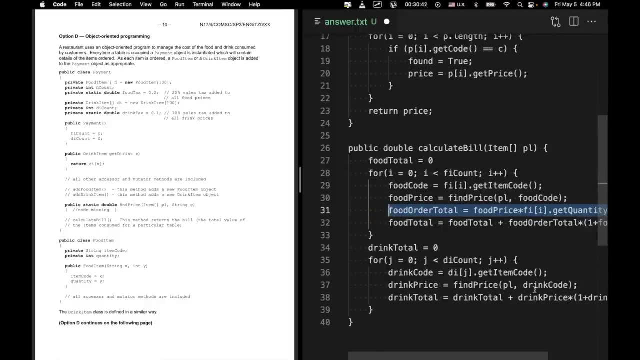 three wines, although we'd probably be really drunk by the end of that, um, so i'm going to do the same thing right down here, just to take that into account. that really, like that's kind of weird the way it's, it's like it is, but yeah, i guess. 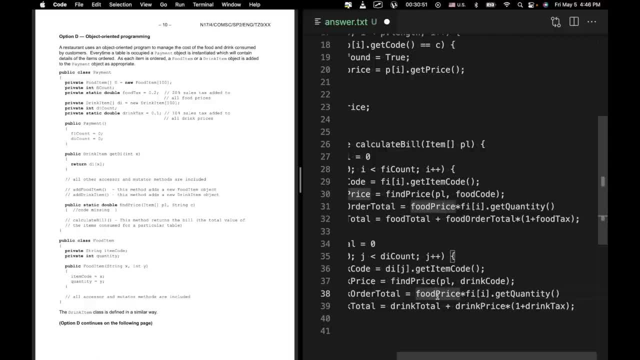 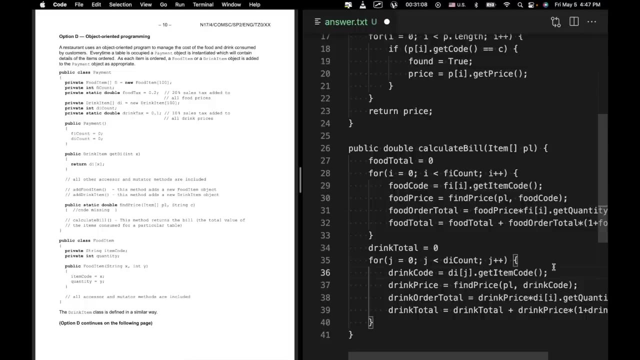 we order more than one of a particular item, so maybe not that weird. we'll say: drink price: uh, times d, i dot get quantity. okay, hmm, cool, looks good, all right. so now that we've done that, um, i'm just going to say: uh, actually i need to initialize this right here. 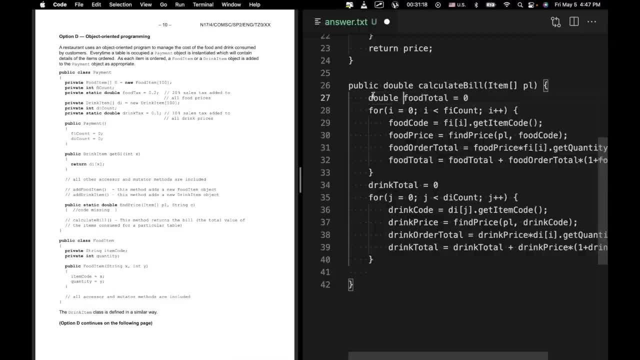 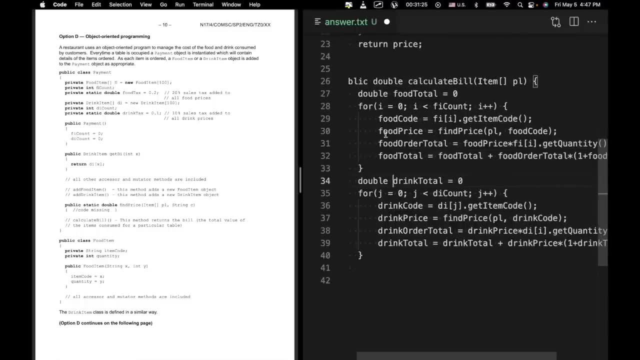 i'm going to say double food total actually. yeah, it's going to be a double right there and double drink total as well. um, um, okay, and right here i need string food code. uh, double food price. i guess i kind of forgot about this because we don't really 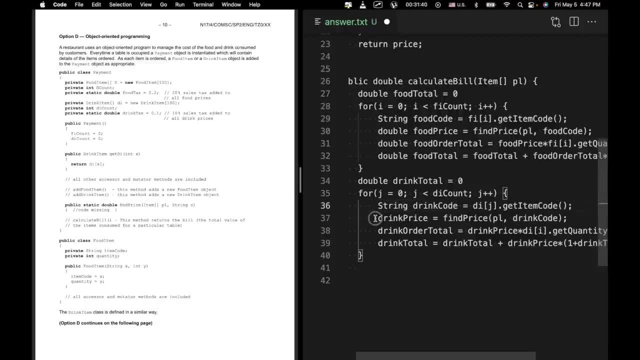 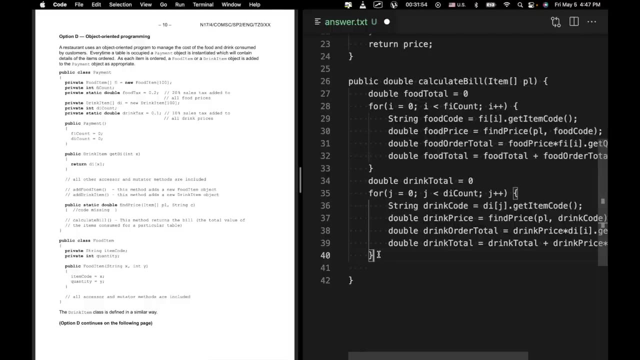 have to do this in python. but hey, we're doing java right now and we're going to have double and double drink, total right here. okay, um, and you do really need to get all of that right. so now that we've got that, we can say, uh, double total. 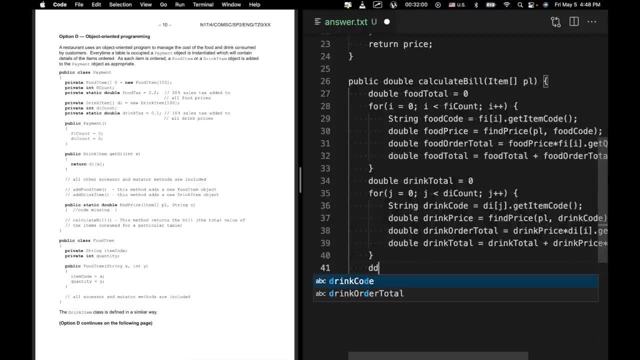 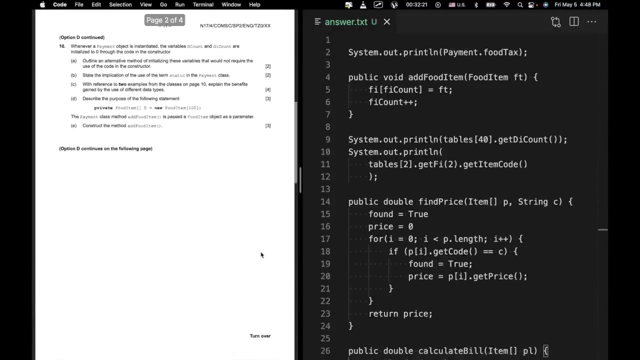 or actually we can just return. oh, i'm just going to make this like as clear as possible. we'll say: double total equals food total, uh plus drink total, and then return total. okay, so that was pretty long, but i think that's the last coding question, um. 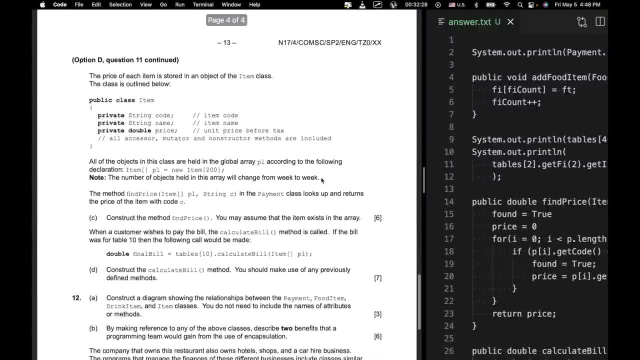 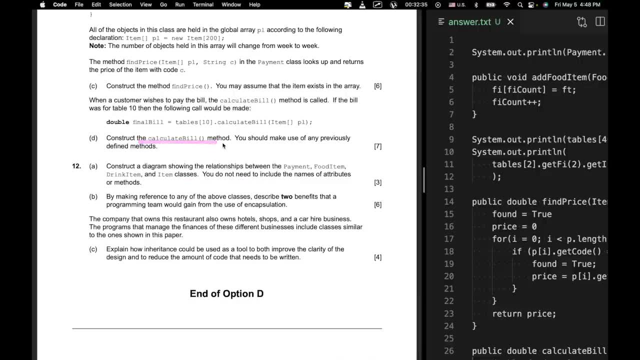 okay, so we're going to go back down to 12 right here, and we did actually successfully complete, uh, that particular question. oh so that was actually still 11, so now 12 is kind of more theory. it says: construct a diagram showing the relationships between the payment food. 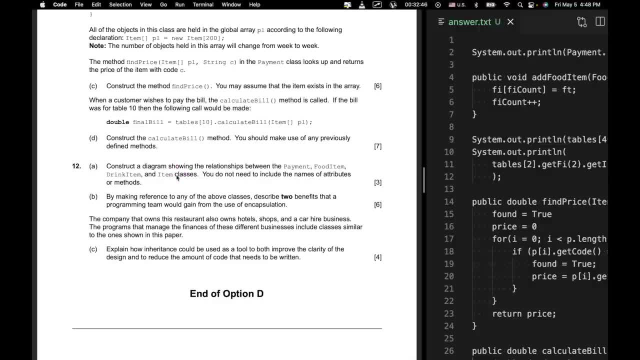 item drink item and item classes. now this is kind of drawing. drawing diagrams showing the relationships is something that you have to do on a lot of the uh different uh option d paper. you've had to do in a lot of different option d papers so you should know how to do it. 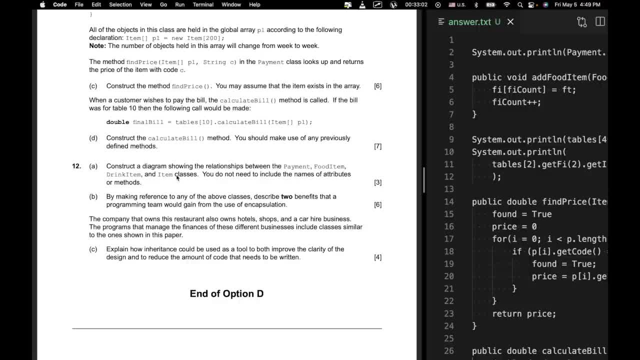 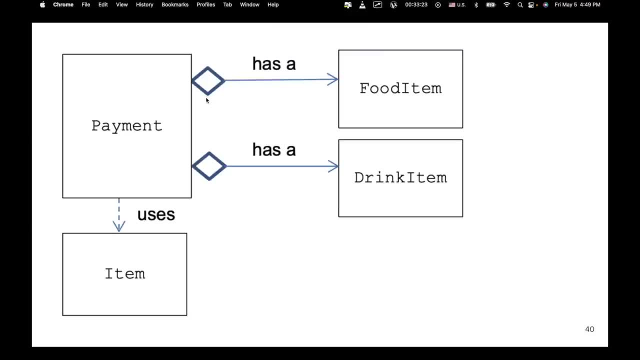 we're going to look at a. we've already seen some diagrams, but we're just going to look at the answer. real quick, um to, just so i can kind of illustrate what this is supposed to look like. okay, so right here. remember payment has. it says has a, but this diamond means 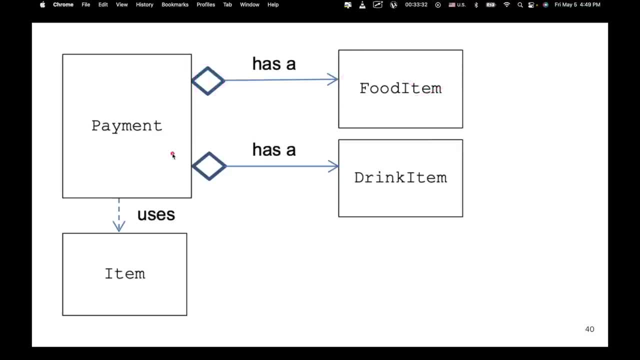 that there are multiple of these food items associated with payment. uh, payment also has multiple drink items. so we have a diamond, we have has a, and then we have an arrow to drink item and then we can just say that payment uses item, because item is not subclass, it's not really in the hierarchy. 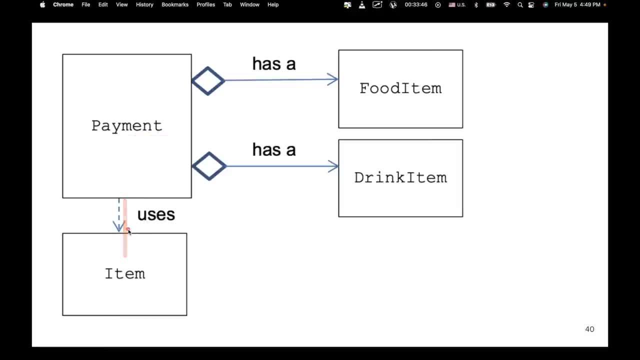 but payment is just making use of item objects. so we have what the payment object uses, which is items, in that static method, and then we have what it has, which is multiple food items, multiple being denoted by the diamond, multiple drink items with multiple drink items, or multiple again. 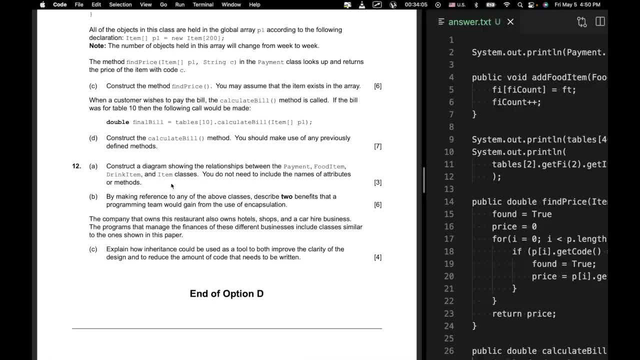 being denoted by the diamond right here. so now it says, by making reference to any of the above classes, describe two benefits that a programming team would gain from the use of encapsulated. so what encapsulation basically means is one having, um having all the attributes and methods. 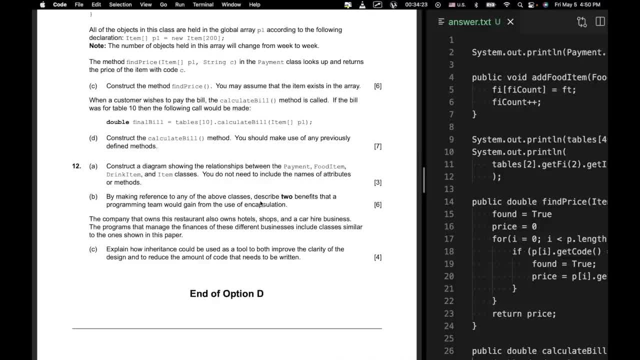 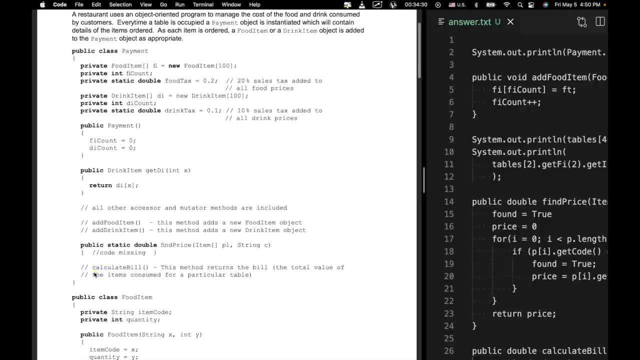 all together in one object, um, and that's useful because that means that we can actually go up here and, for example, if we want to get calculate bill, we can make use of all the other attributes in this object and aggregate them in order to be able to. 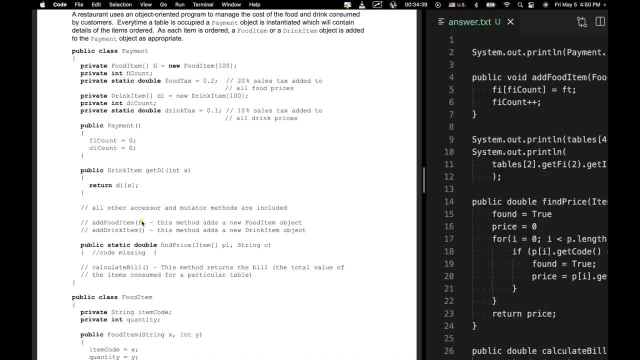 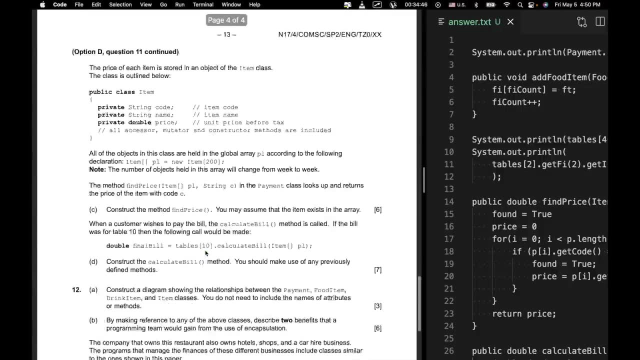 uh, find the bill in conjunction with another method that we have, which is find price. so it just basically means being able to have those all in one place and be able to make use of them to do complex calculations is one benefit, i would say another benefit is: 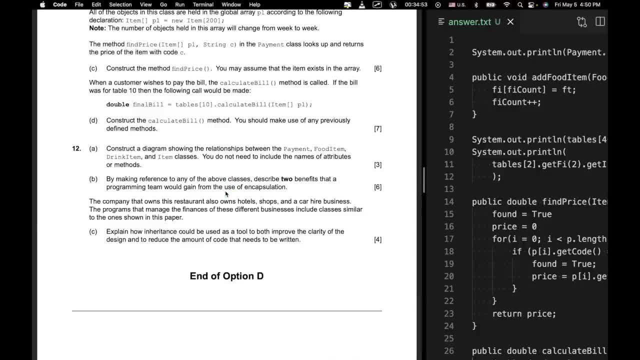 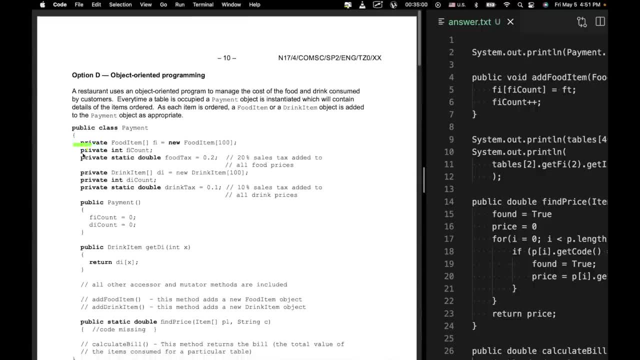 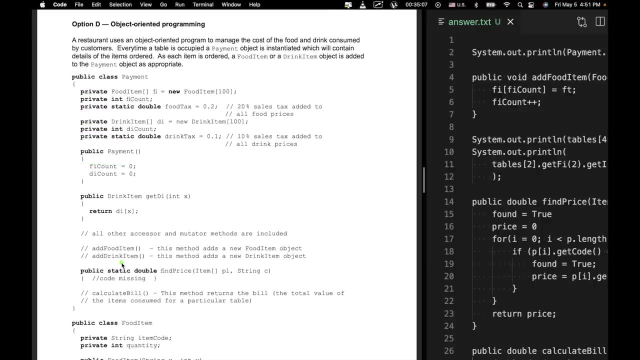 to the other use of encapsulation, which is um, those accessor methods. right so, because um these? right here, because these are private. this means that if we want, we can control exactly how they're used through our um accessor or, more importantly, mutator methods. so, for example, right here, 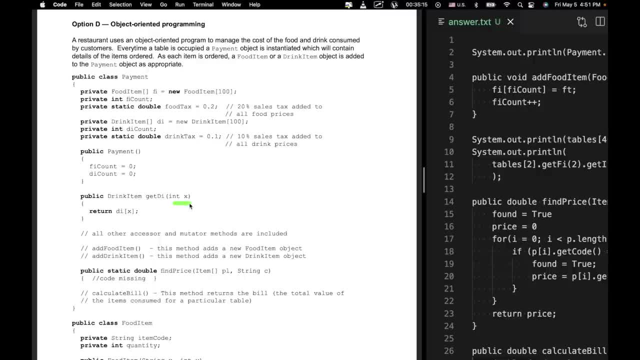 um, if we wanted to have a specific criteria for the indices- we want to make sure someone's putting in a valid index- we could do that. so, basically, what we can do is we can use accessor methods which are a component of encapsulation, in order to make sure that only those values are being edited. 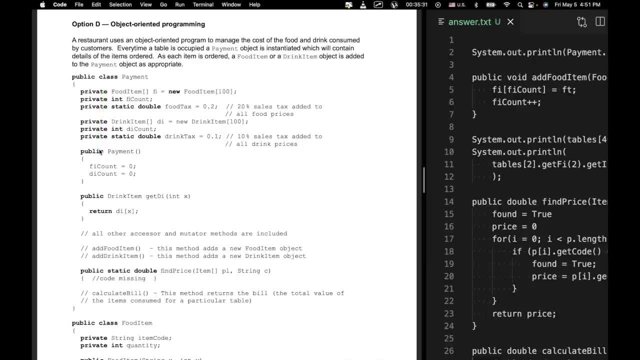 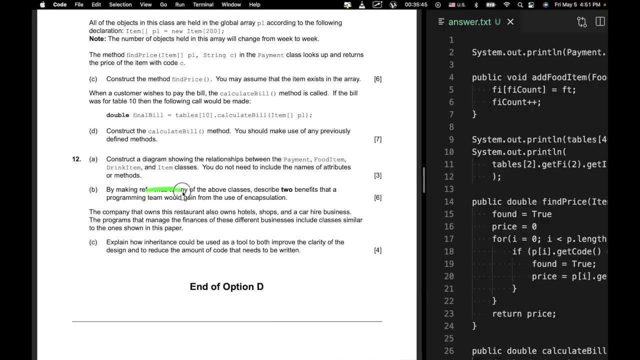 that we want to be edited- uh, from outside the object and then also control how they can be edited? uh, by forcing other programmers to use accessor and mutator methods. and now, let's see, it says by making reference to any of the above classes. okay, so we already just did that. 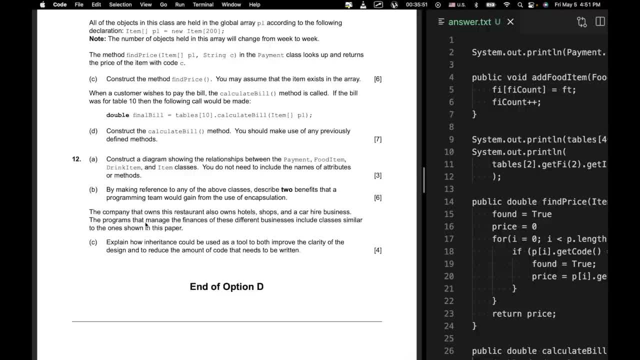 it says the company owns this restaurant. who owns this restaurant also owns hotels, shops and a car hire business. programs that manage the finances of these different businesses include classes similar to the ones shown in this paper. explain how inheritance could be used as a tool to both improve the clarity and the 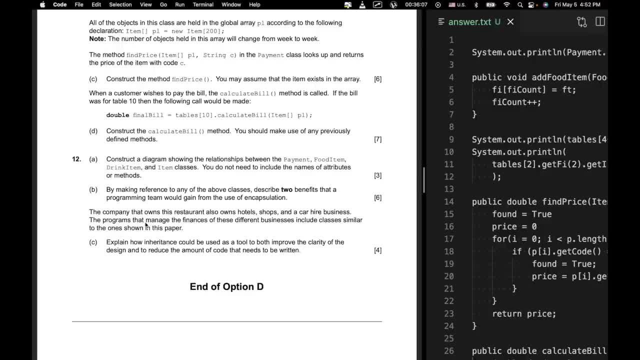 design um and to reduce the amount of code that needs to be written um. so probably what i would do is i would create a generic payment class and remember the payment class actually corresponded to tables, um, but i would have um in hotels- it'd probably be hotel rooms. 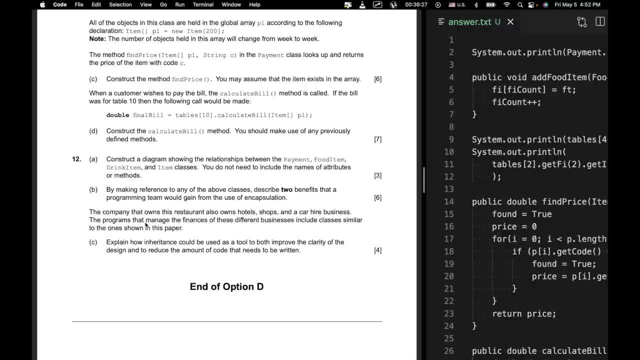 um, in shops that'd probably be probably just a customer and in a car hire business that'd probably be a car and i think they would all share. um, they could all share a payment class. i mean, obviously, that payment class wouldn't have pay, wouldn't have payment or drink. 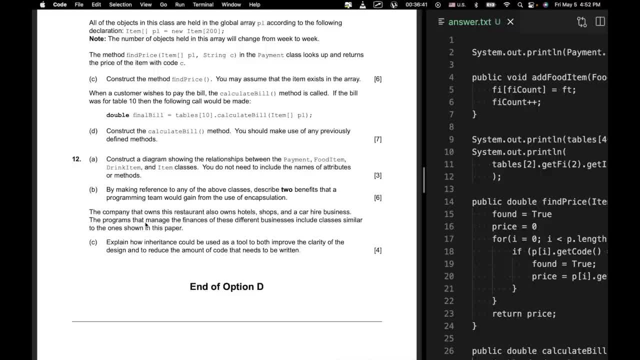 items, but it might just have price or it might have the quantity of units, um. so that could be one way in which inheritance could be utilized, or so we could have a generic payment class and we could have on the different types of goods being sold in each one of. 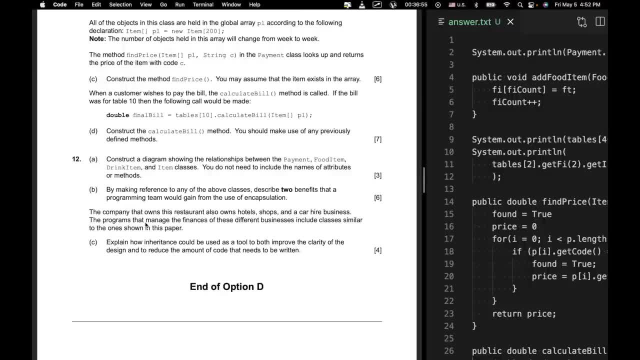 these um different places inherit from that payment class and have their own attributes and methods assigned to it. that also means that we wouldn't need to write the code in a payment class over again. we could just write the code once and share it between these different subclasses. 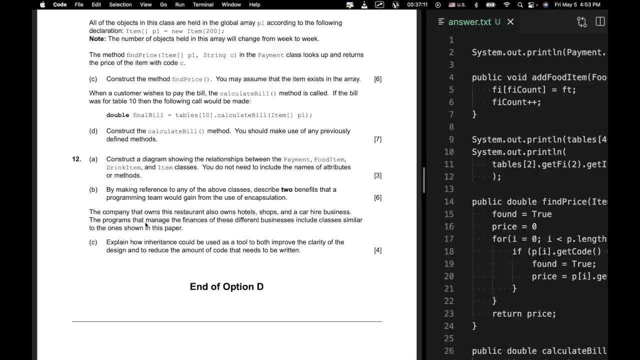 um, i think that it's probably the most, um, significant way. uh, we could also well- i guess static methods or attributes don't really play into that- but yeah, just this idea of having a generic payment class and then having, uh, then having classes associated with the uh specific type. 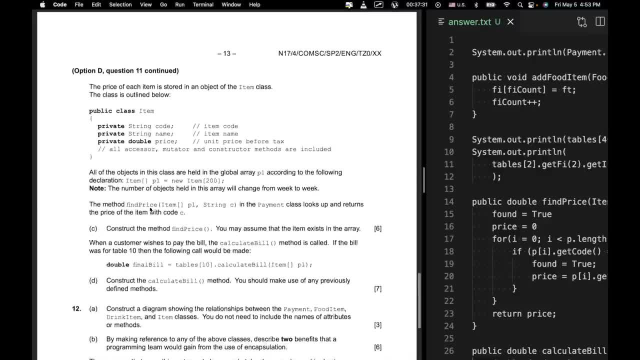 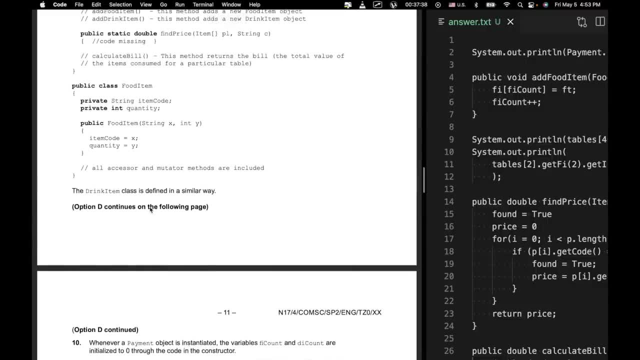 of business anyways. that's, we basically did a whole option d paper. i was gonna do two of these, but this is running into 37 minutes, so i think we're just gonna stop here. um, i hope that was useful to you, like i know this may be. 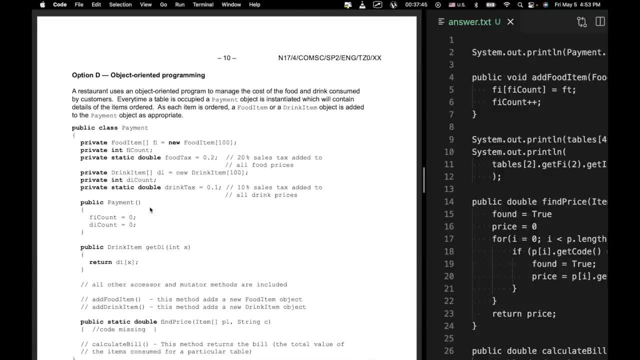 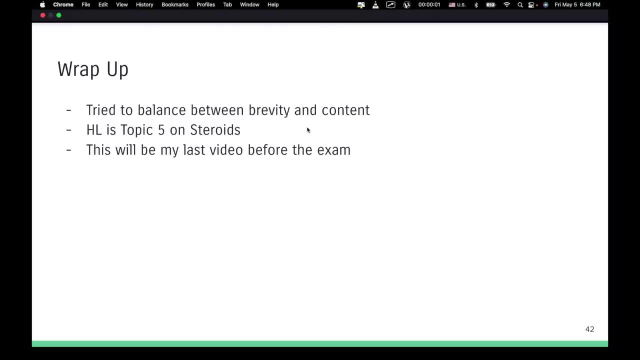 been hard to see. uh, i've never actually done this before, like having a paper on one side and writing code on the other side. hopefully this was of some value to you and i could walk you through some of my logic. okay, guys, so that basically wraps up, um. 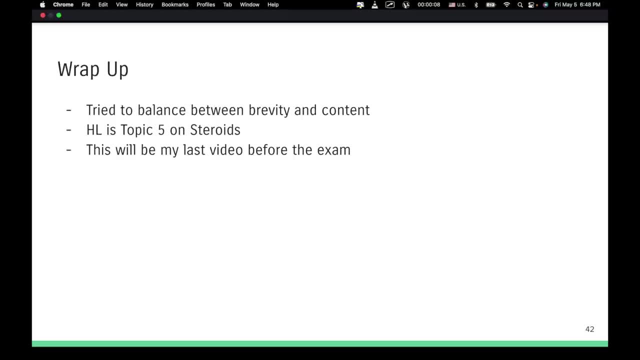 the sl portion of option uh d, like i would have liked to do another exam paper work through and potentially, uh, like a little project. but i really wanted to balance between brevity and content and, um, that's particularly true as i'm putting this out like two or three days before the exam. 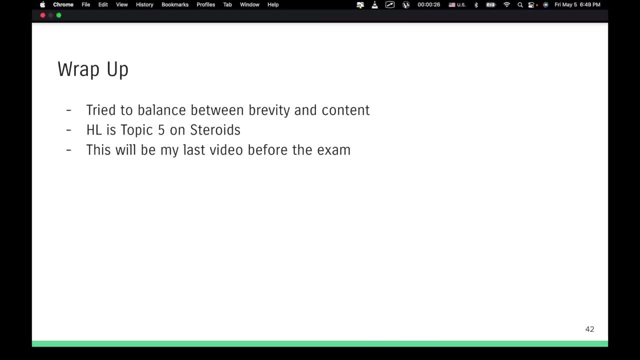 now hl is topic five on steroids. like it's basically taking all the topic five content and then applying it to object oriented programming and i just really don't have time to go through that before the exam. so this will be my last video before the exam. um, for those who will be taking the test,